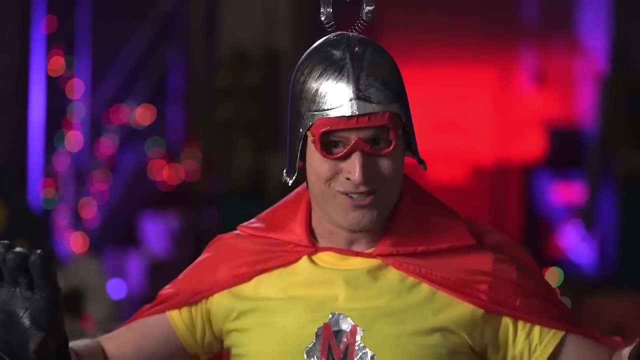 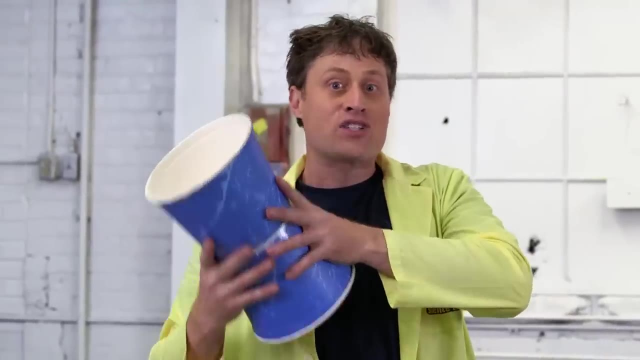 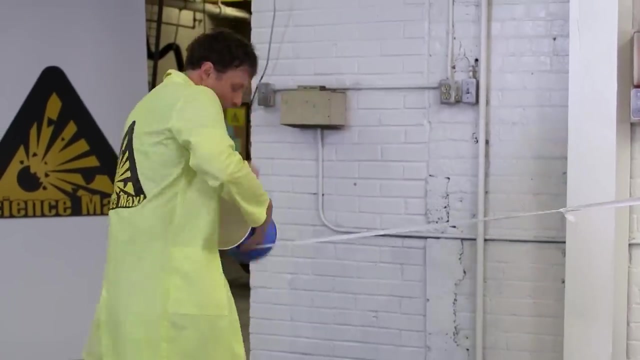 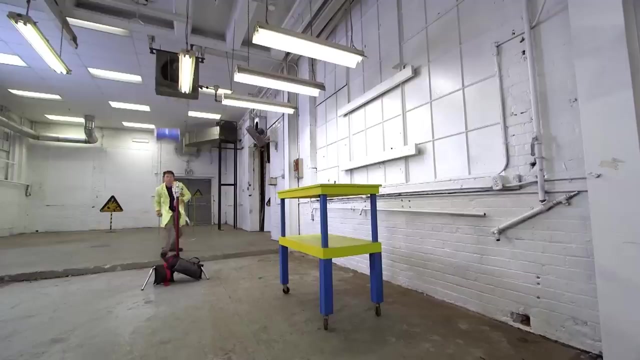 Magnus it out. See how much better that sounds. No, no, no, max, max it out. Check it out. Magnus Flyer 2.0. Stand Elastic Slingshot. Wrap it around. Oh, Remember for the Magnus Effect to work. 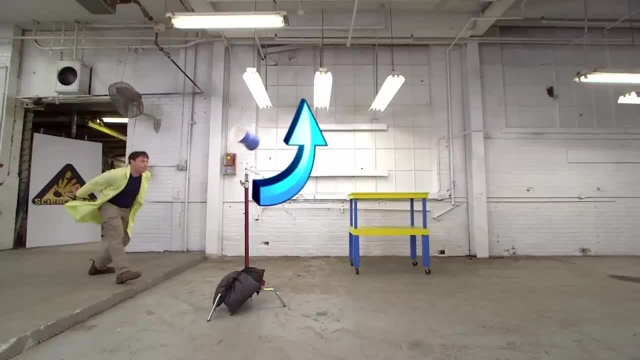 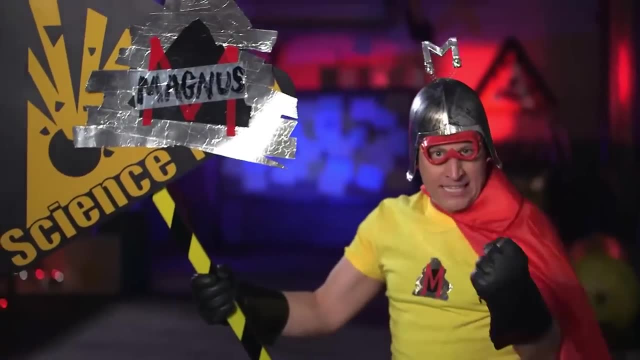 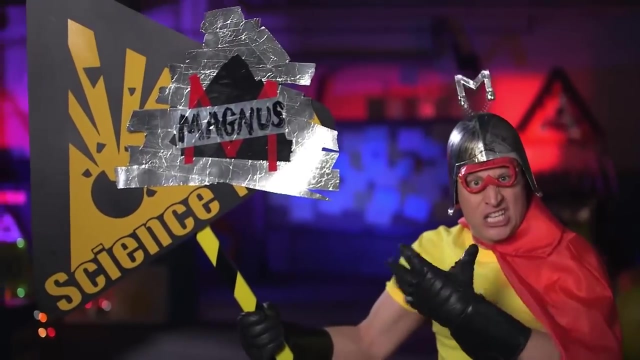 your cups need to be spinning this way, the front side rotating up. Oh, And there you have it, The Magnus Effect. I, Magnus, am now taking over the show. It is now Science Magnus. That is my effect, Slightly improving the name of science TV shows. 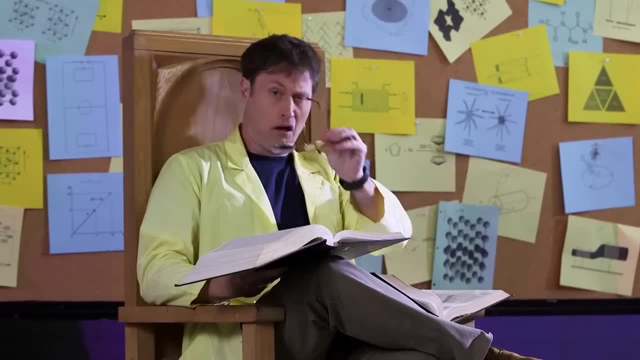 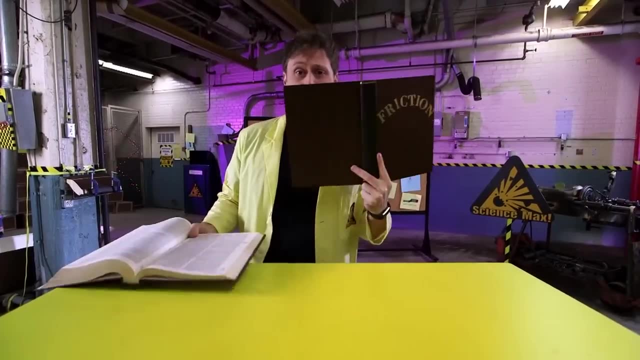 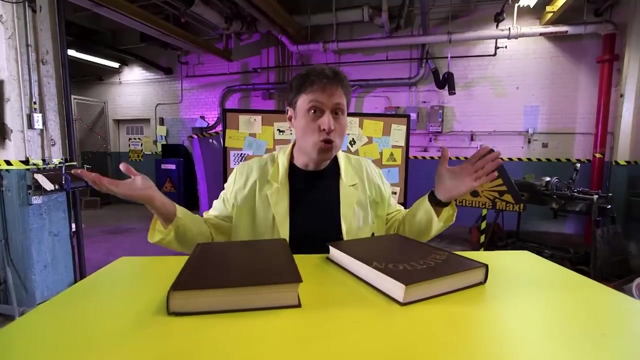 Oh, hello there. Uh, Here's a fun science experiment you can do with science and friction together. Take two books, Put them on top of each other and pull them apart. Ooh, not too much friction, But if you take the books, 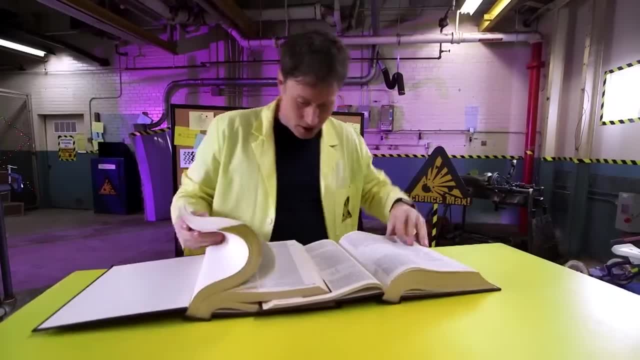 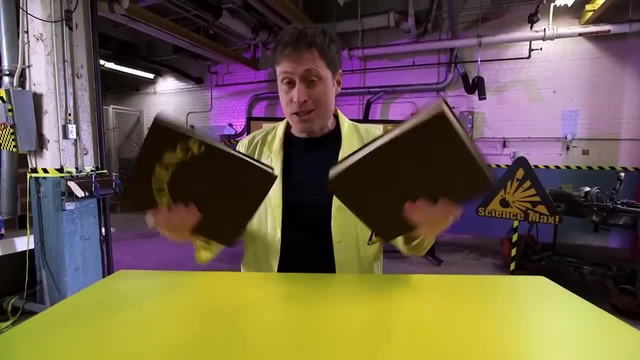 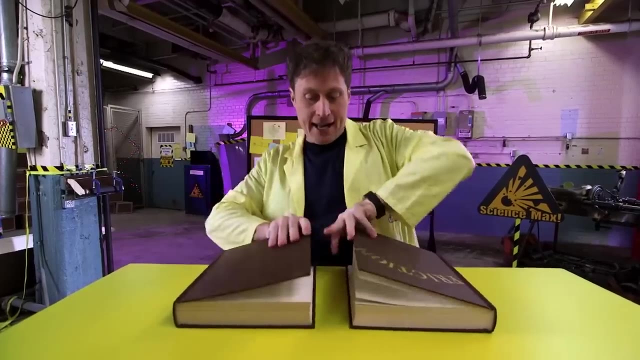 and you interleave some of the pages- maybe three or four parts- and try it again, pull them apart. they're a little harder to pull apart. That's because the friction for more pages touching each other actually starts to add up. So what if we were to take two books? 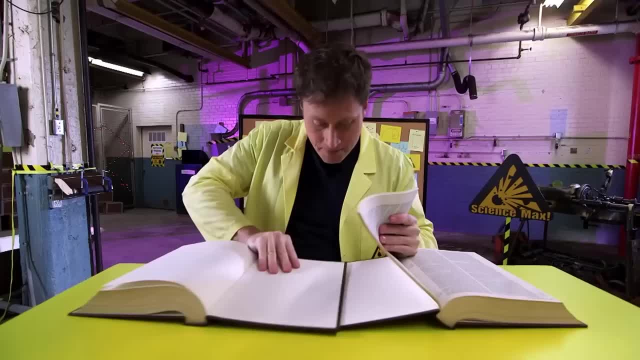 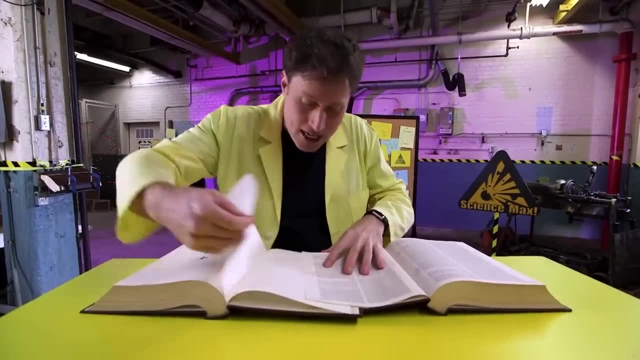 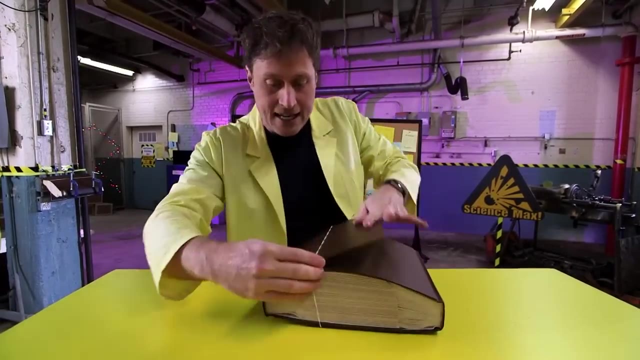 with a lot of pages and very carefully and meticulously take them apart And meticulously take each page individually, one at a time, and overlay each one and go back and forth. These are two books completely shuffled together. The elastic band is actually just to hold the covers together. 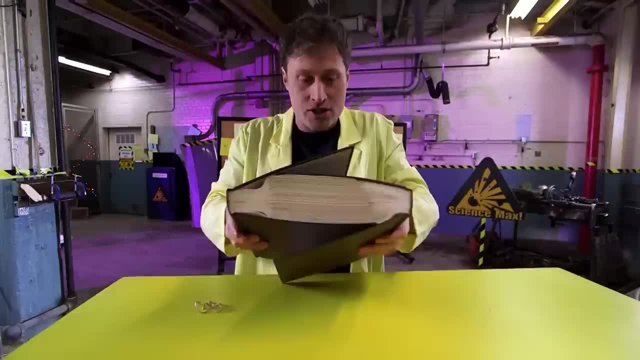 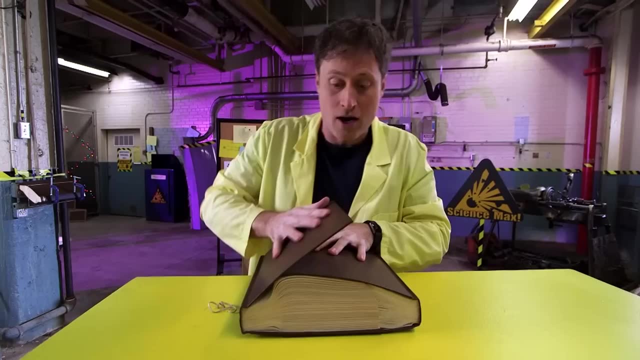 All right. So now, the friction between all of these pages when I try to pull it apart makes it pretty much impossible. Now there's two things going on here. First of all, when you start to pull the books apart, the pages start to stick together. 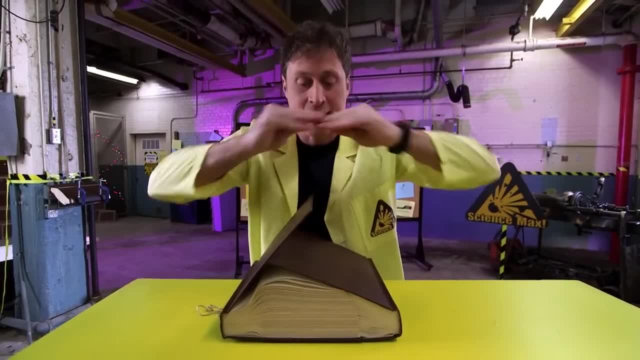 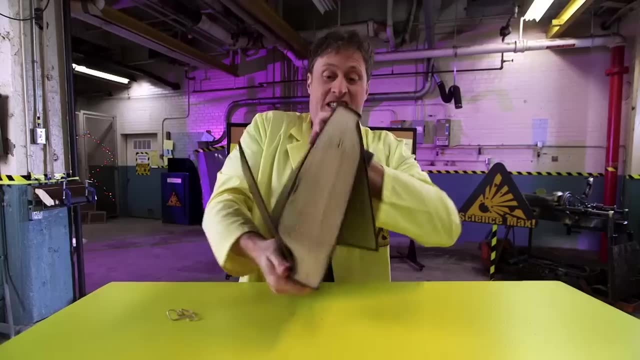 because they squeeze together, because you're pulling and they're squeezing, And the fact that there's so many pages sticking together, the friction builds up to a degree that is actually very impressive, But don't take my word for it. Let's max it out. 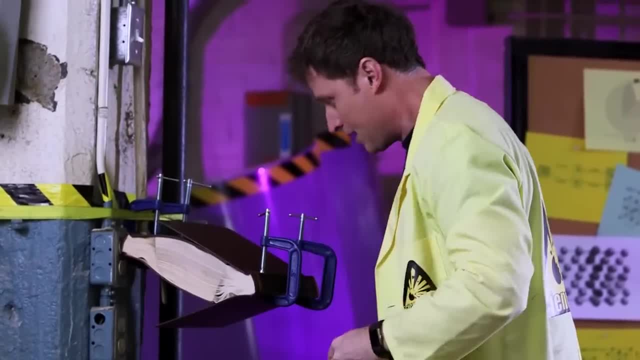 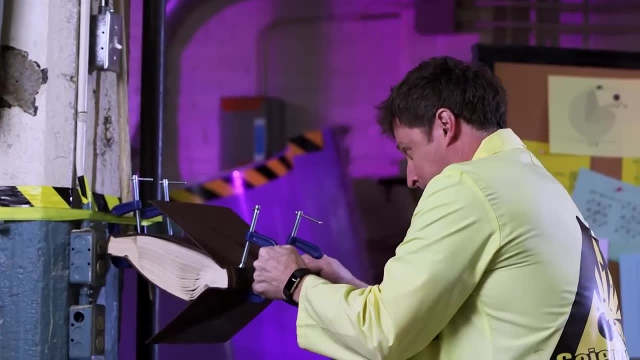 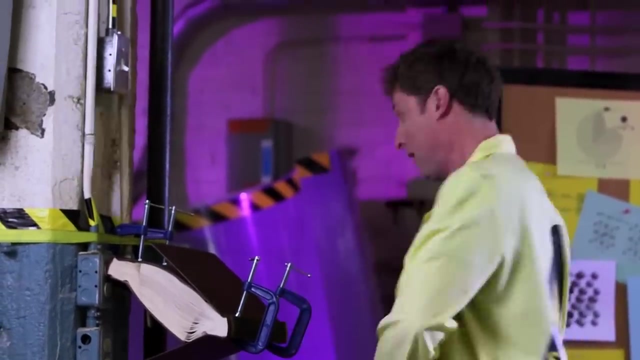 Here is another two books: elastic just to hold the covers, This one clamped to the wall And I'm going to pull this one. Science Still don't believe me? Well, let's max it out some more. Two books, all the pages layered together. 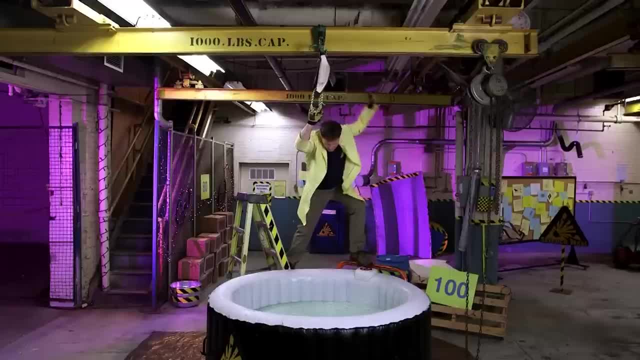 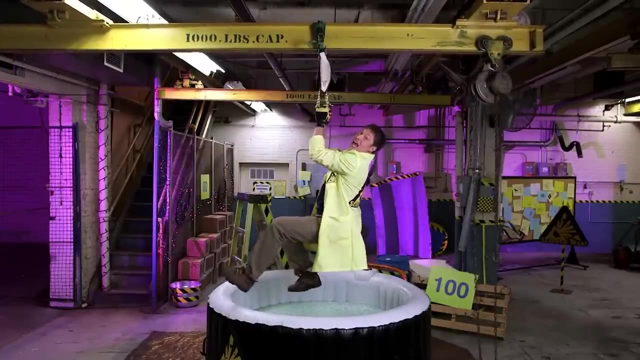 held together only by friction, suspended over a giant vat of slime. Now let's see how much faith I have in science: Friction, yeah, Okay, Okay, Oh, no, Okay now to get down. Okay, hold on. 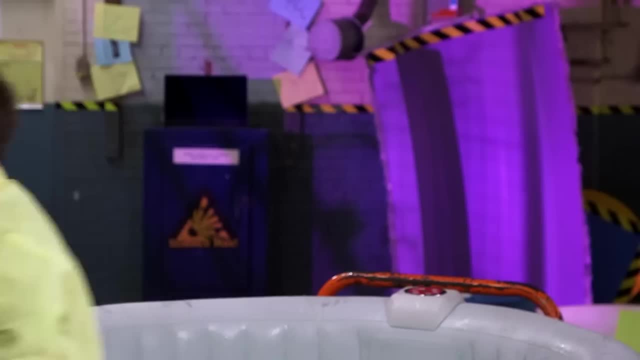 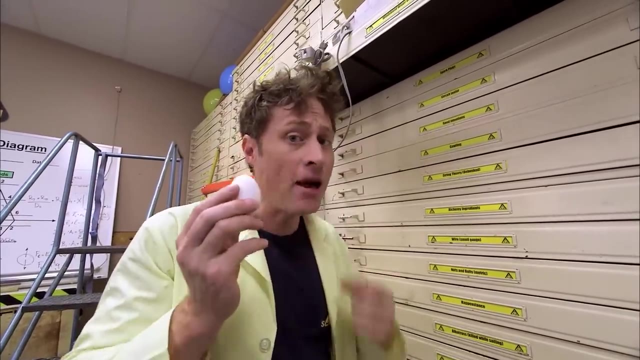 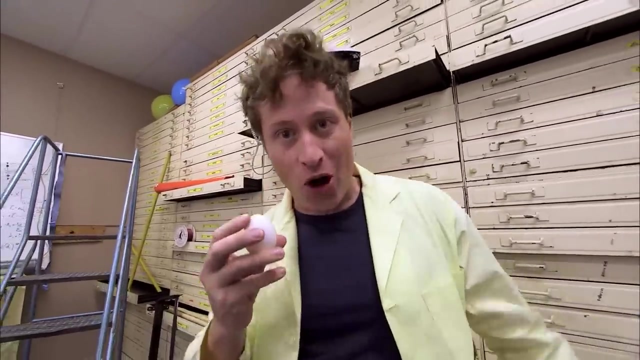 Science, That was close. Oops, An egg. Now you might think of eggs as kind of flimsy and they do break pretty easily. but eggs, Eggs- are actually stronger than you think. It's because they're well egg-shaped. 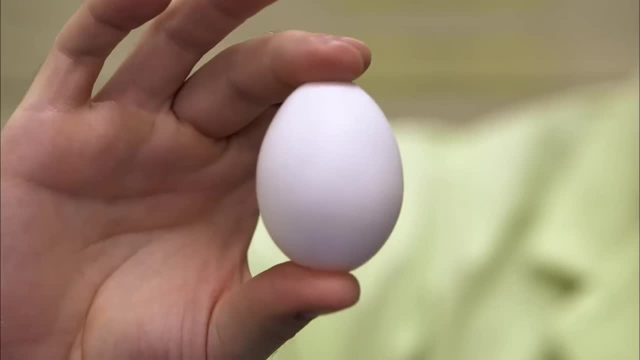 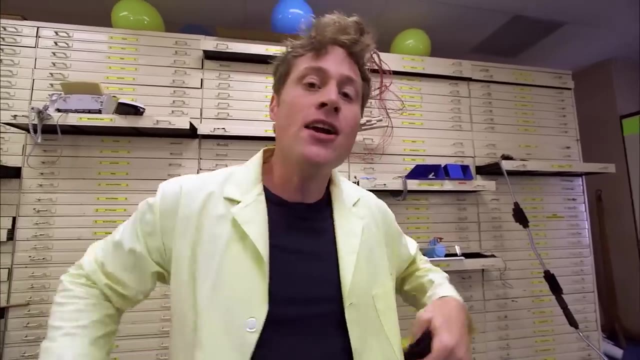 You see, the top of the egg is like a little bit of an arch and the bottom of the egg is also like an arch, and arches distribute the weight just like they do in a bridge. Here's how you can experiment with how strong eggs are. 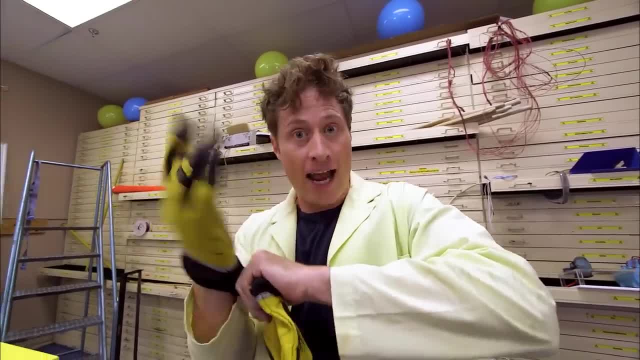 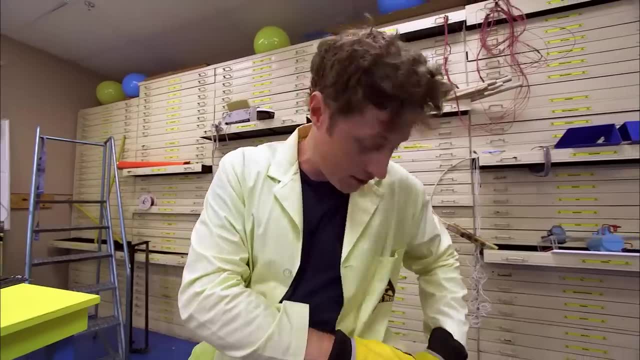 First, you want to get a pair of gloves to protect your hands from the shell, just in case anything goes wrong. You should also tell an adult that you're doing this experiment, because if it does go wrong, you're going to have some mess to explain. 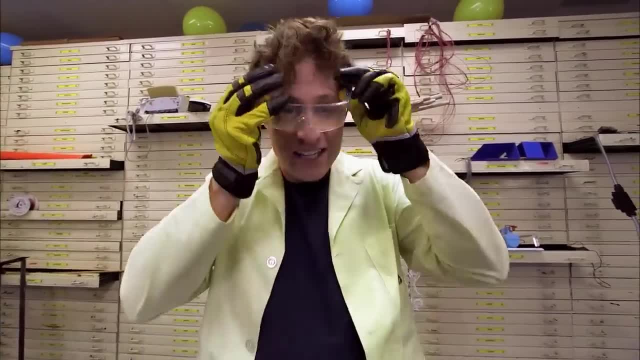 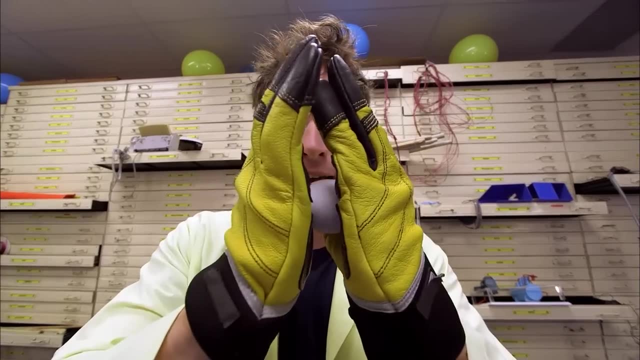 And also you should probably put on some safety glasses. Now here's what you do: Take your egg and carefully put it in your palm, just like that, and put it against your other palm and you're going to push in directly on either side of the egg. 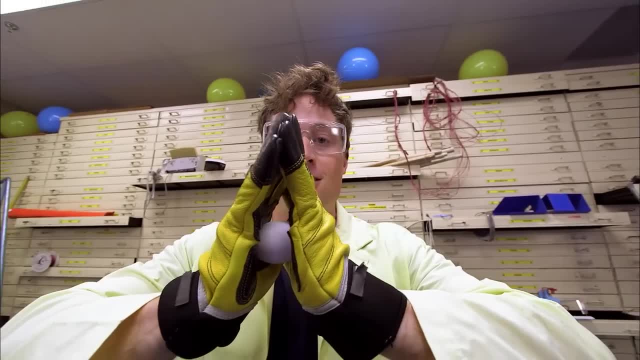 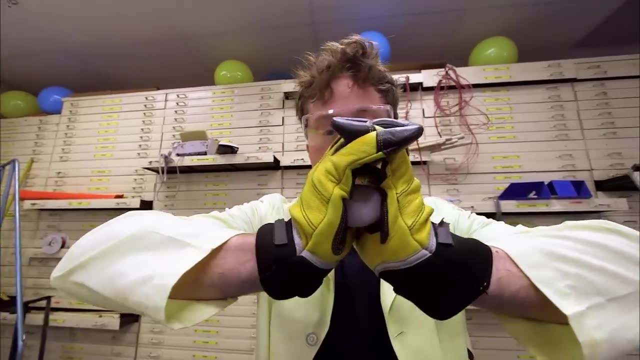 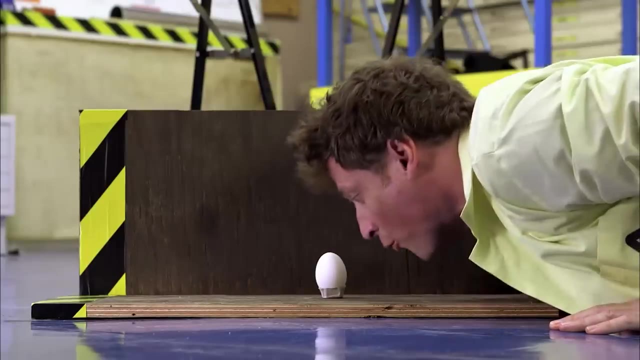 Start pushing harder and harder. You can even lace your fingers and press even harder and if you do it right, the egg won't break. Pretty amazing, right? So just how much weight does an egg hold? Can one egg support my entire weight? 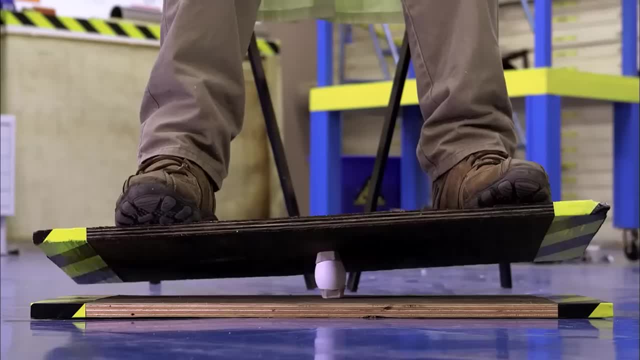 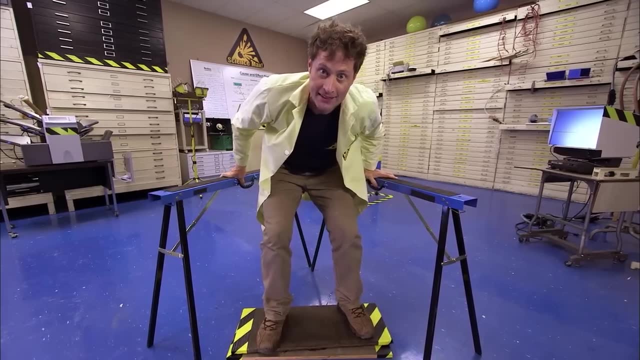 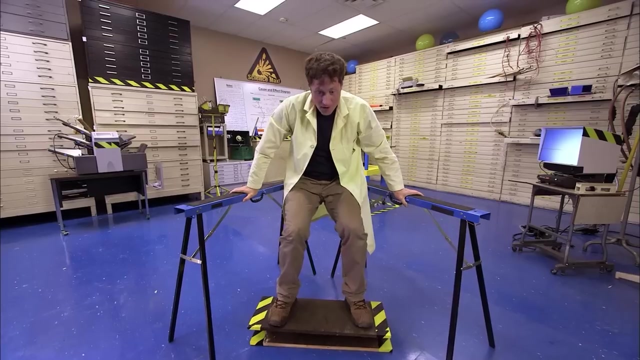 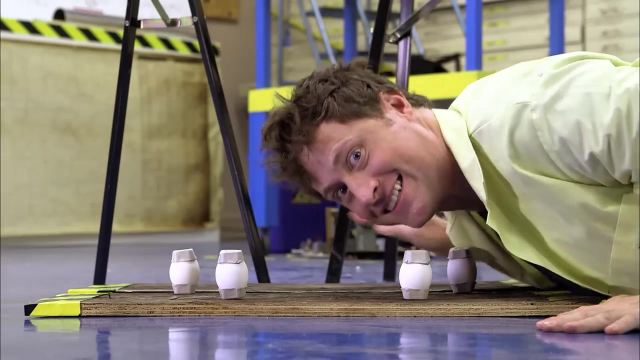 Let's find out. I'm going to lift my weight up like this and lower myself down and No, Cannot hold my weight. Can my weight be supported by two eggs? Uh, nope, Phil's weight, Four eggs, Oh. 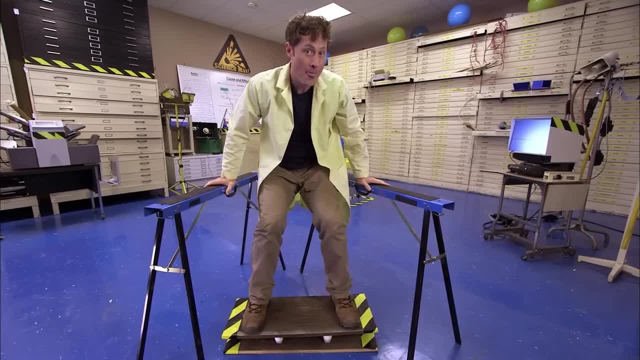 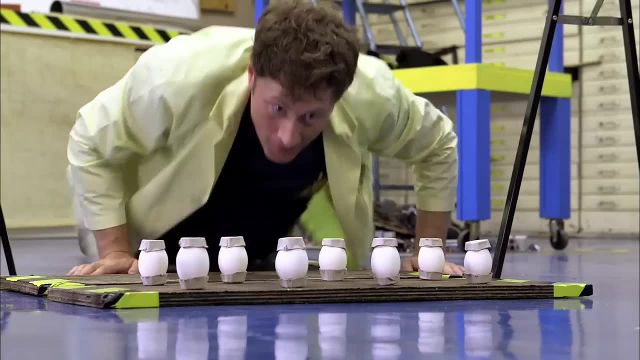 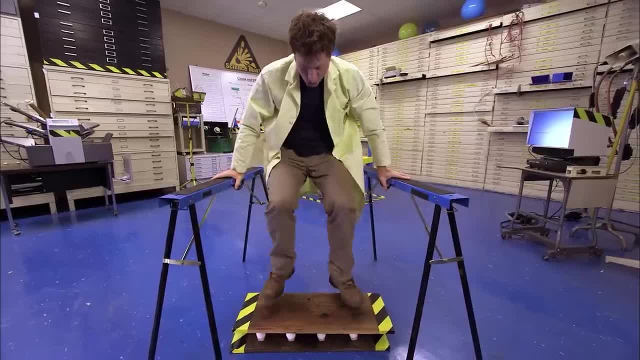 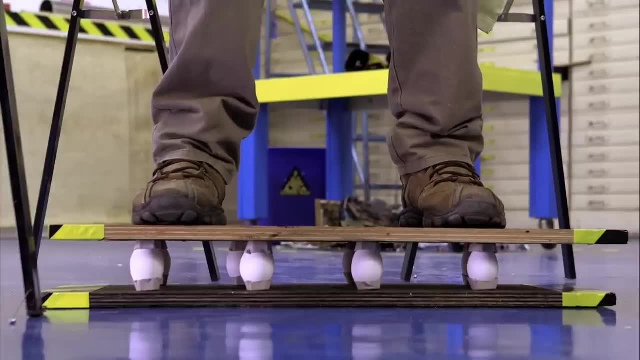 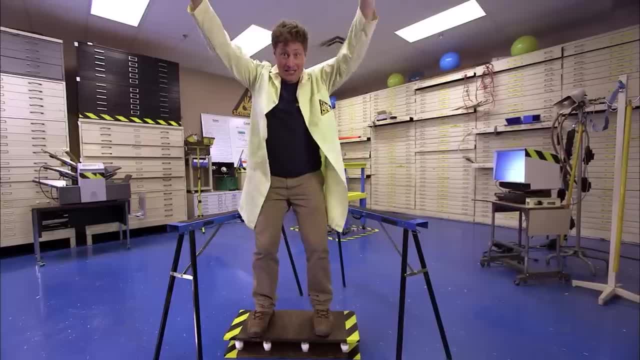 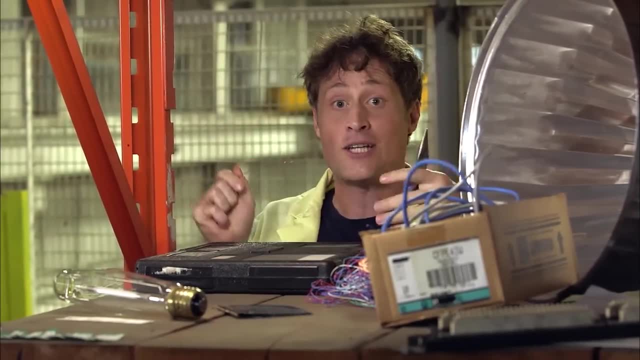 Ah, Oh, My weight can be supported by just eight eggs. Science, Careful Tires, Battery, Copper wire. Now, if you've already done the electromagnet experiment, here is another experiment that uses all the same materials, plus these. 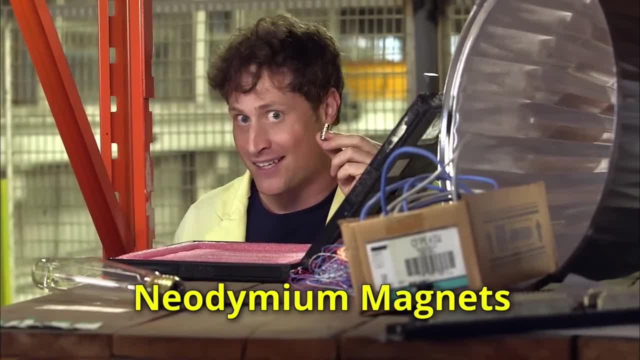 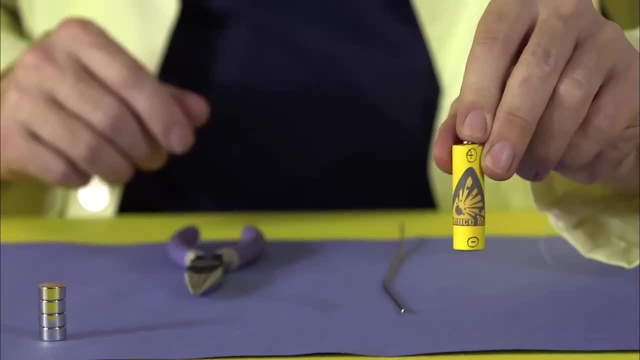 Neodymium magnets, some of the strongest magnets you can get. So what does the mom do with her embryo? Here's what you need: A battery, some neodymium magnets the same diameter as your battery, copper wire and some pliers. 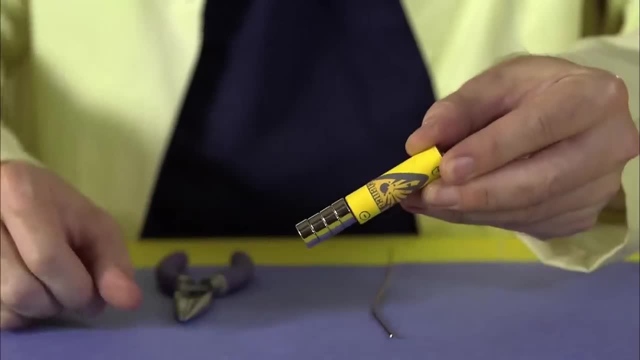 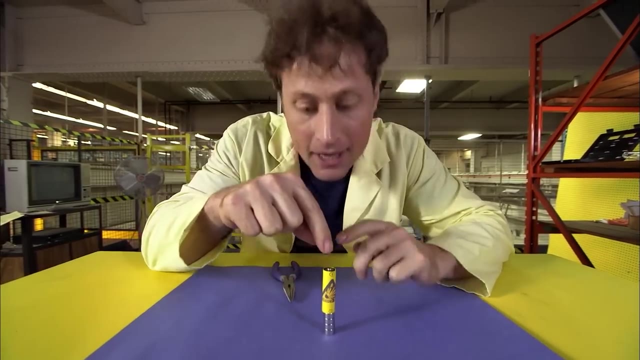 So here's what you do. First thing is you put the batteries and the magnets together like that. Then what you wanna do is bend the wire so it's touching the top of the battery and goes around the battery and then touches the magnets at the bottom. 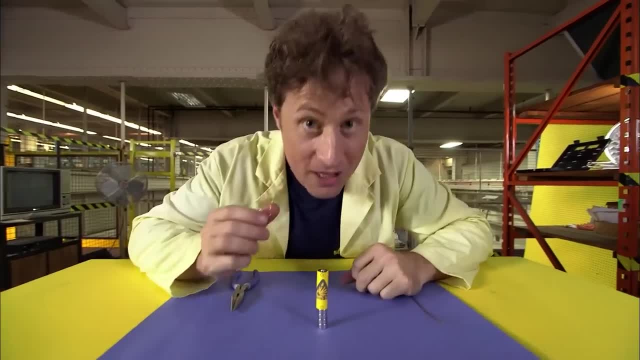 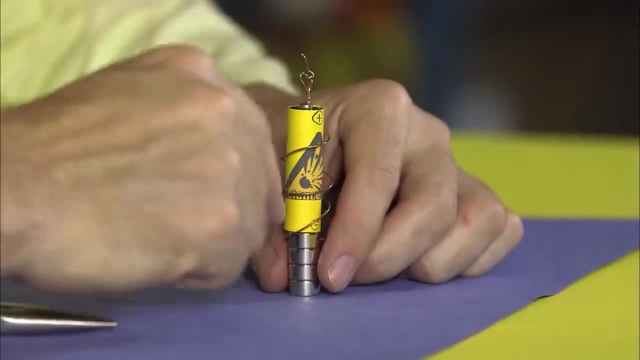 Here's what that might look like. I say might because you can do any shape you want. I've made a coil here and if you put it over the battery you'll see it only touches the very top of the battery and the magnets at the bottom. 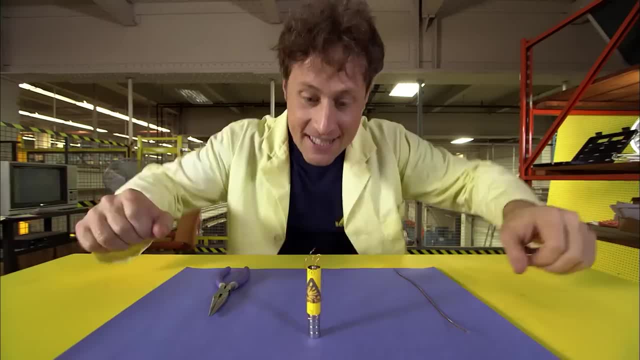 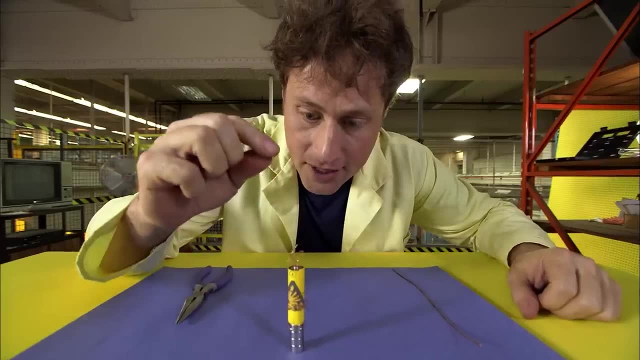 And if I let it go, it spins. It's a homopolar motor. What happens is the battery sends an electric current through the copper wire and that turns it into an electromagnet, which is attracted to the magnets at the bottom and it spins. 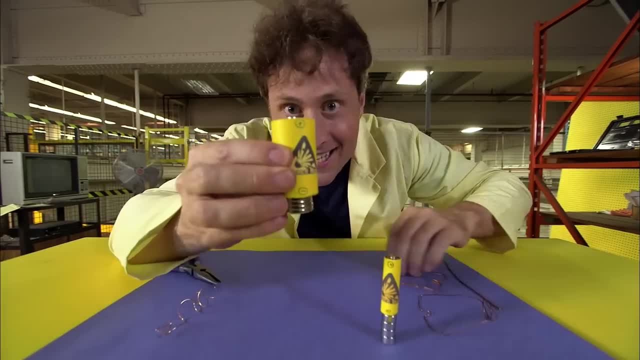 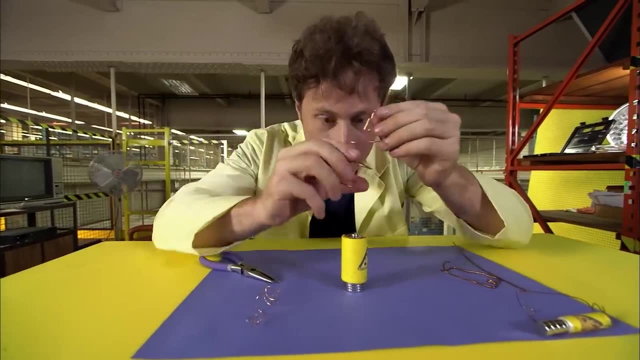 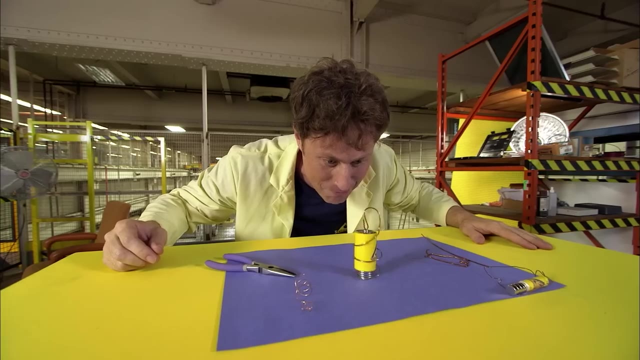 So now let's max it out. Ha ha, a D cell battery, which is larger, and of course larger neodymium magnets. and you do the same thing: Make a coil that only touches the battery at the top and at the magnet, and ha ha, it spins. 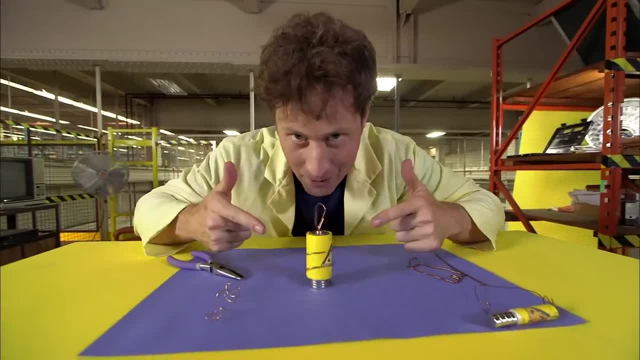 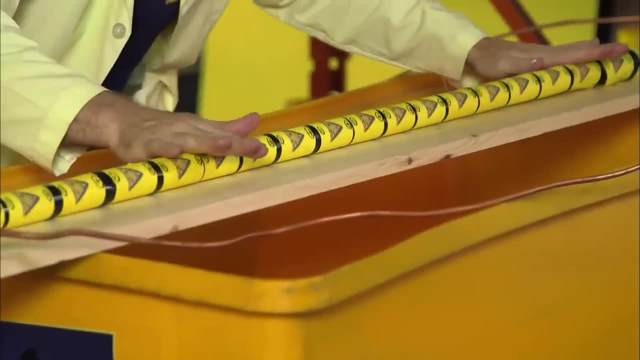 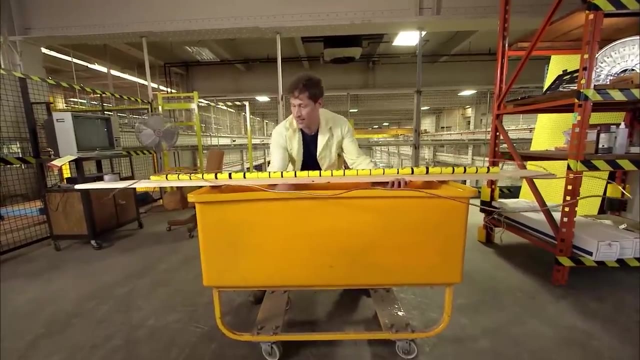 Max out homopolar motor. But don't worry, this is not the biggest size we're gonna do. Come on, ha ha ha. maxed out homopolar motor. I have 27 D cell batteries, a giant copper tube and a neodymium magnet, so I'm just gonna. 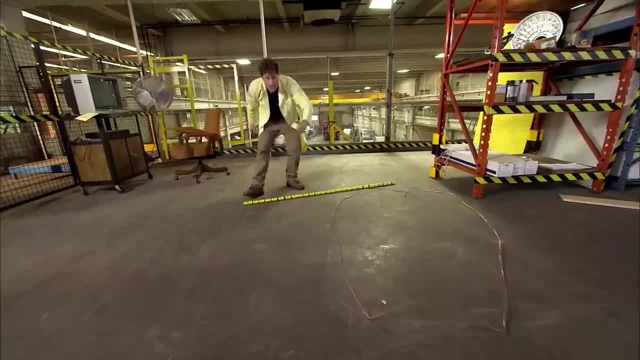 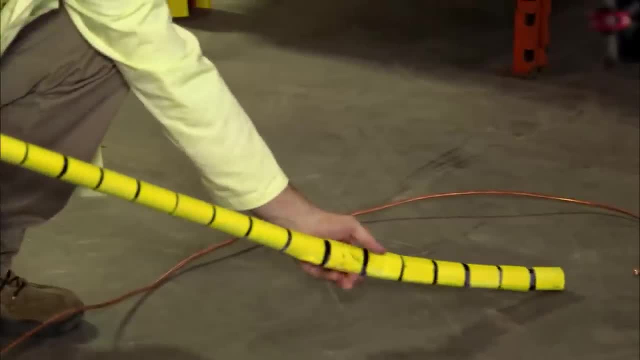 get rid of that. put this down, Okay, so the first thing I do is attach the neodymium magnet to the batteries, and I've got all the batteries taped together here, so they'll sort of stand up like like this: ha. 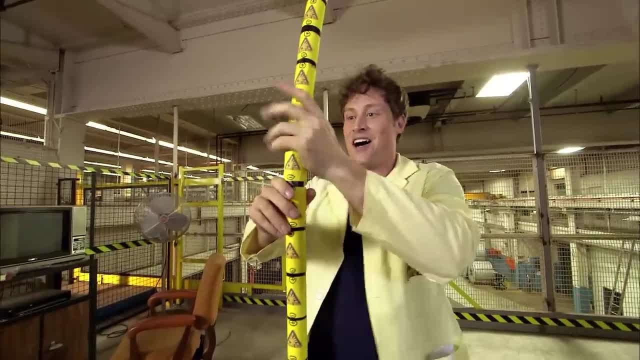 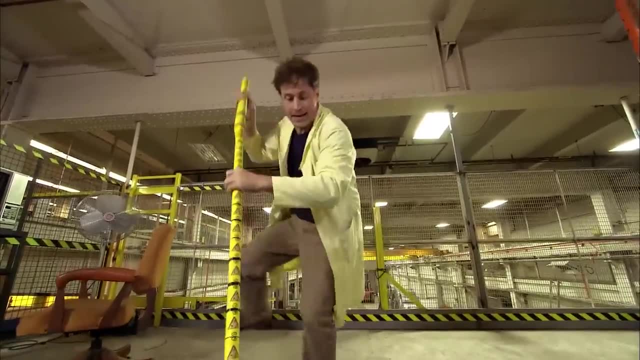 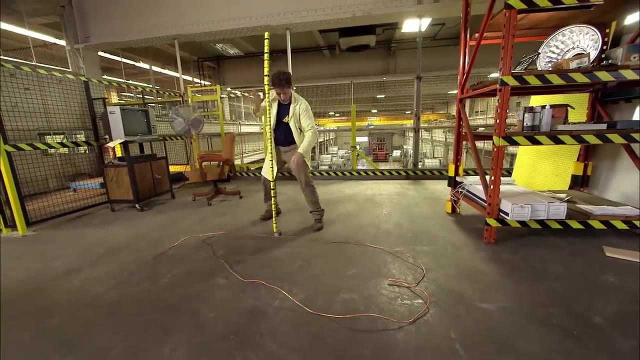 Ha, ha, ha, ha ha. giant stack of D cell batteries. Okay, now what I do is I take the copper, I take the copper coil. um, I need to get, I need to get. okay, hold on, hold on, I got this. 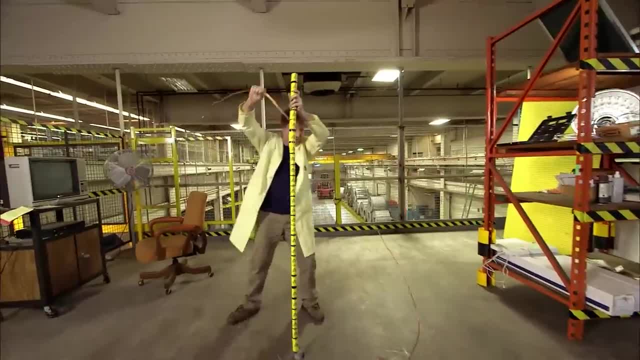 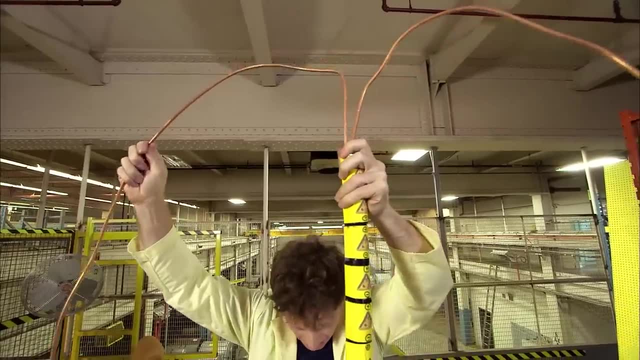 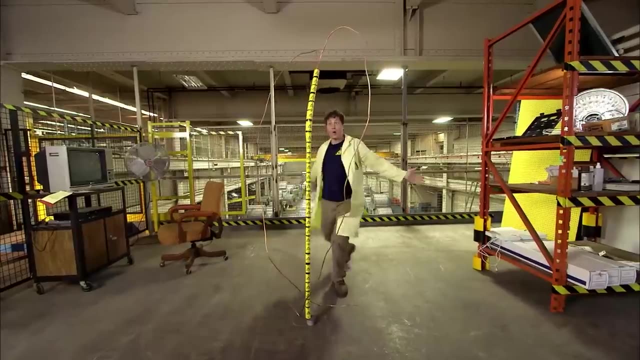 I just need to get the copper coil in. Ha ha, ha ha, I did it. Okay, so I take the copper and I put it on top of the D cell batteries, like this, and then I let it go. Let it go. Nope, whoa homopolar motor. 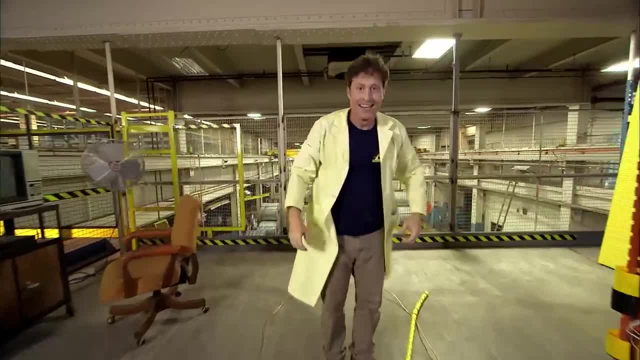 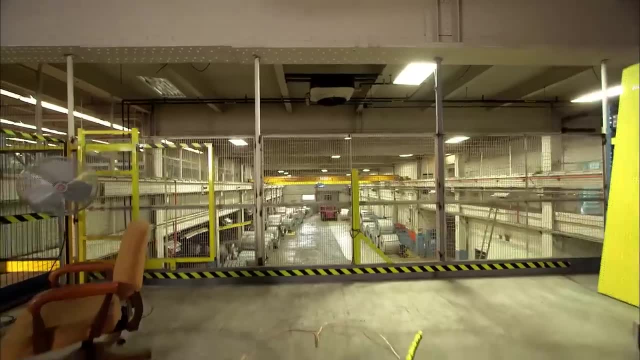 Okay, so that didn't work, but that's okay. I like it when it doesn't work, cause that's science. It's not science if it works perfectly every time. I mean you gotta have some room for improvement. Science. 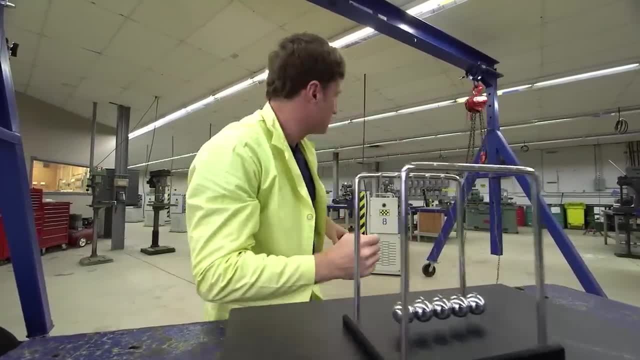 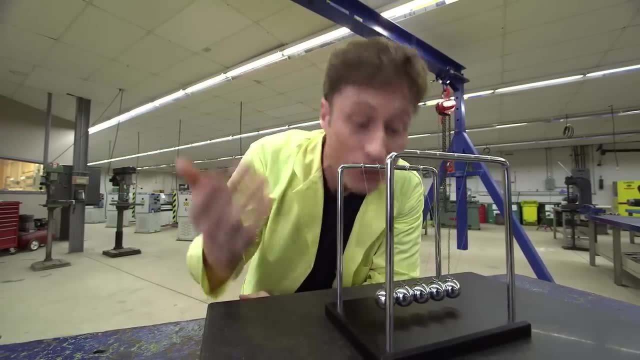 Whoa. Okay, This. this is Newton's cradle and it's a really cool toy that demonstrates all kinds of laws of motion, including Newton's cradle, Including Newton's third law- Newton's third law. What you do is you pull this one ball out. 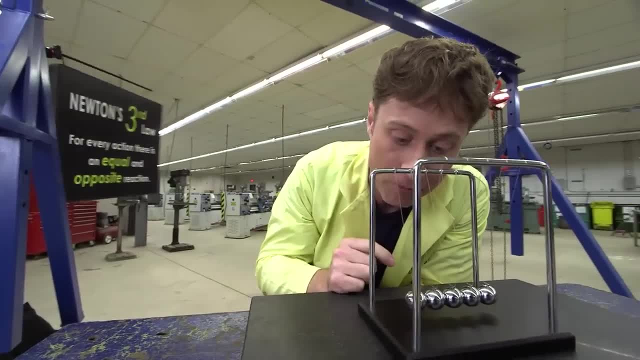 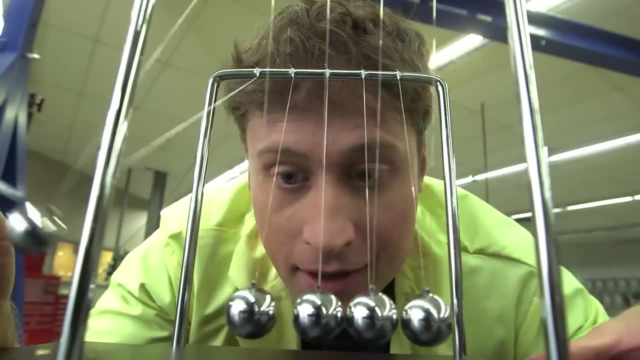 and when it hits these balls, they exert force on that ball to make it stop moving, but it exerts force on these balls which travels through the balls and makes this one on the end fly out like that. Now there's a lot going on here, but you can really see. 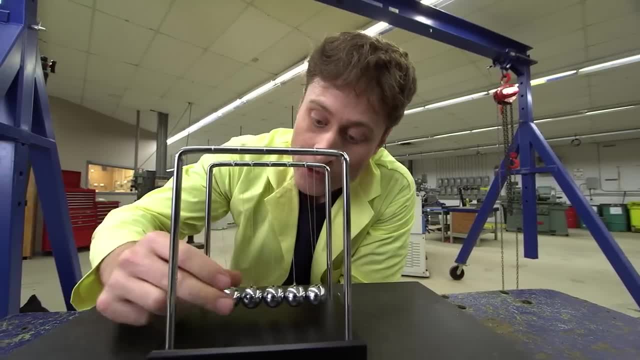 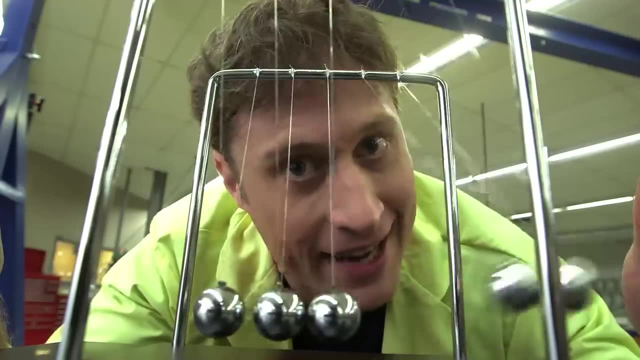 how the force is equal, that you put in and you get out. if you use two balls, I swing two balls up and two balls go out. that side Isn't that cool. Now, it wouldn't be science max unless we maxed it out. so come on. 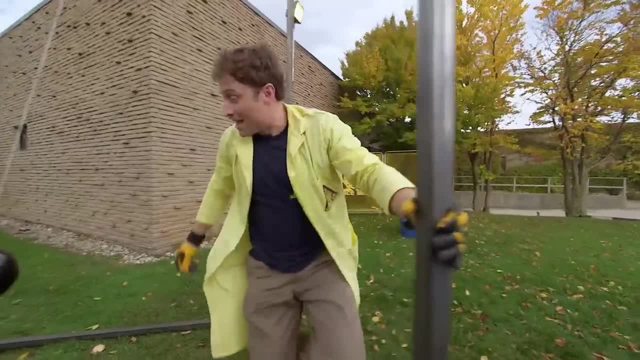 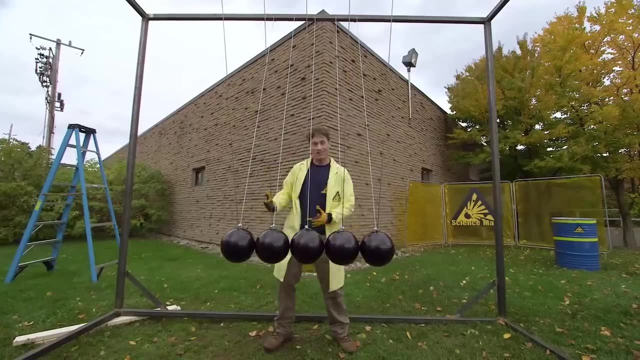 Whoa, okay, This is one we built out of bowling balls, Bowling balls, bowling balls instead of smaller balls, And I think it's gonna work the same way. Let's find out, You throw one out and and yeah, it works the same. 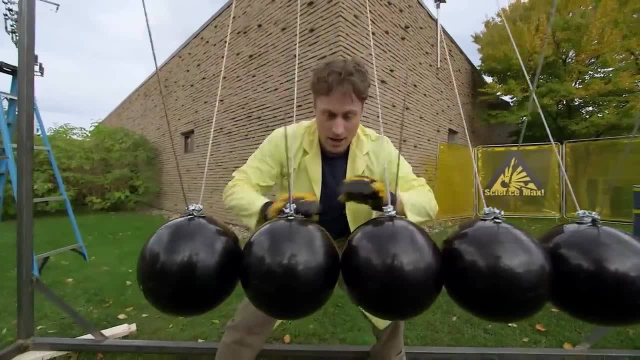 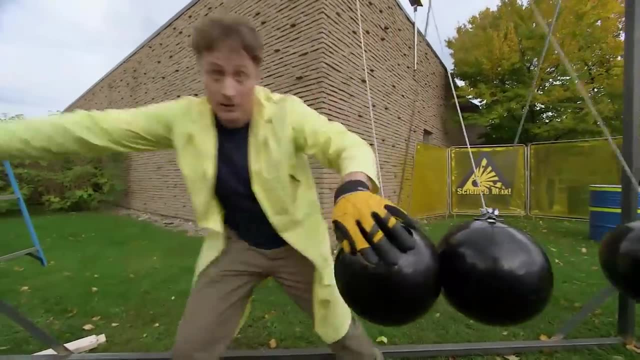 Okay, now let's try it with two balls. Okay, ready, Wait, wait, wait, wait. And two balls throw them out And two balls on that side. All right, so there you have it, Newton's Third Law. 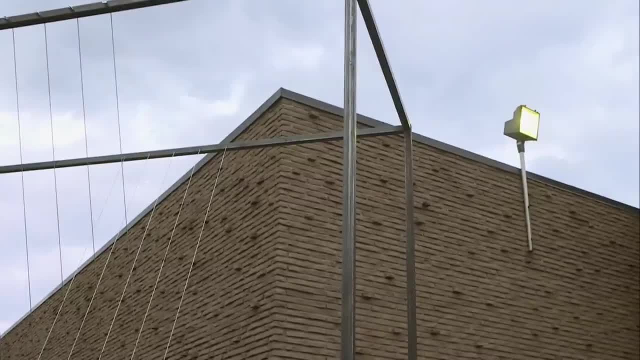 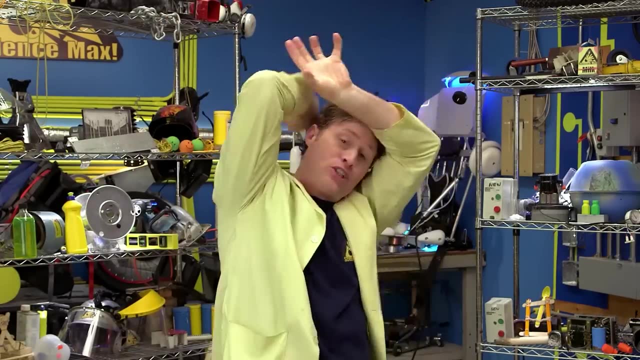 Oh, Ah. Newton's Third Law: For every action there is an equal and opposite reaction. Help, I'm being crushed by all this pressure. A whole kilogram is being pushed down on every square centimeter of my body. 103 kilopascals, ah. 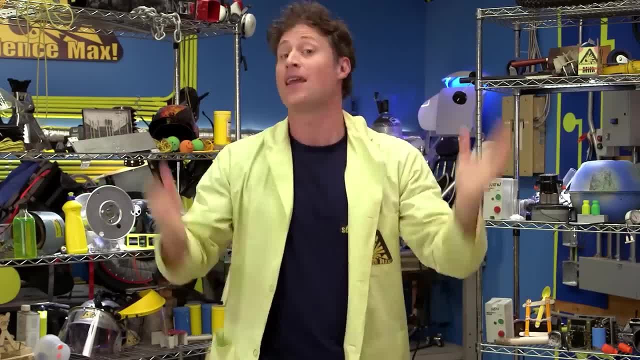 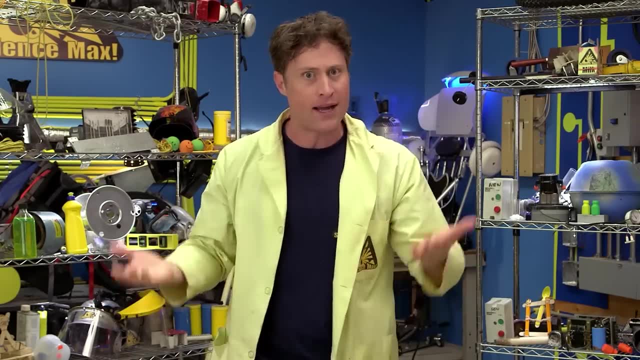 Actually, one kilogram for every square centimeter on your body is the exact kind of pressure that you and I are under at all times every day. We don't notice it because we're used to it, but it sounds like a lot, doesn't it? 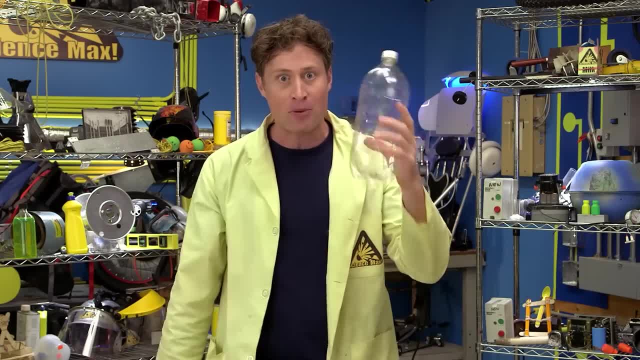 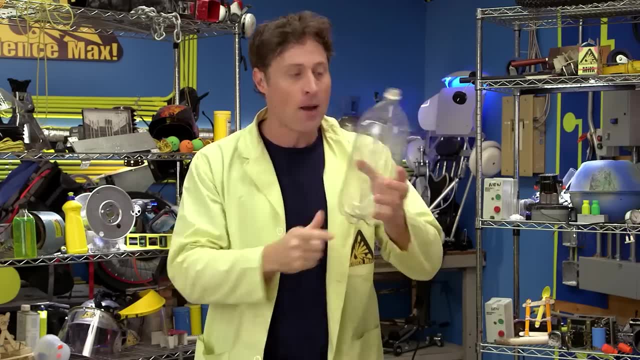 Well it is. Here's an experiment you can do with a plastic bottle. Say, at room temperature there are 10 million air molecules in here. doesn't really matter how many, but we'll say there's 10 million at normal room temperature. 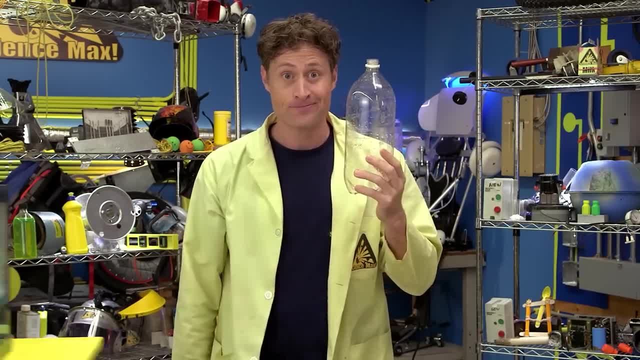 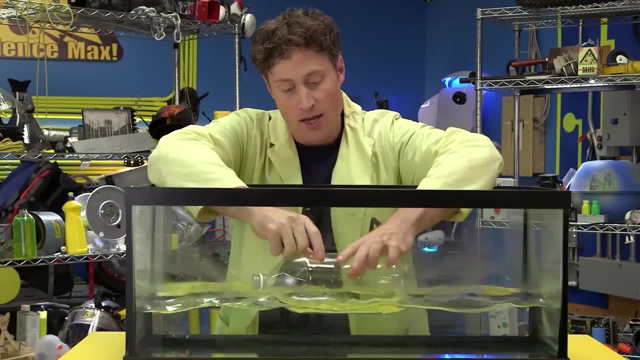 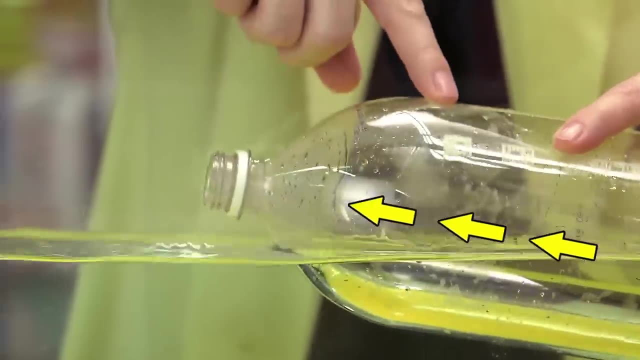 What happens if I heat up the air inside this bottle? This is warm water. What I'm trying to do is heat up the air inside the bottle because the air molecules, when they get hotter, move faster and need more room. So the 10 million air molecules are starting to escape out. 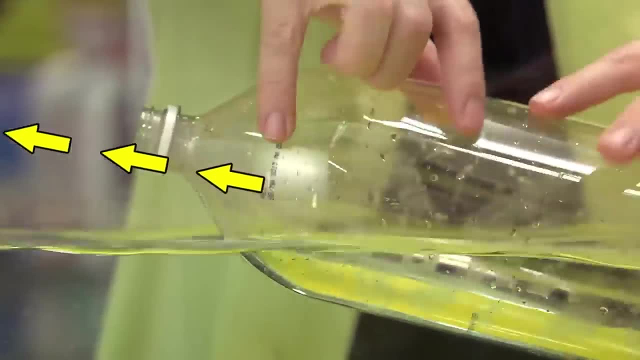 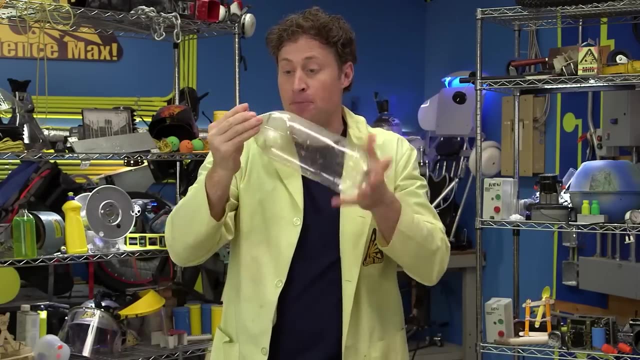 the mouth of the bottle and reducing the number of air molecules inside. And now I take the bottle out and cap it, Because the air molecules heated up and speeded up. they needed more room. Now there's less of them in the bottle. 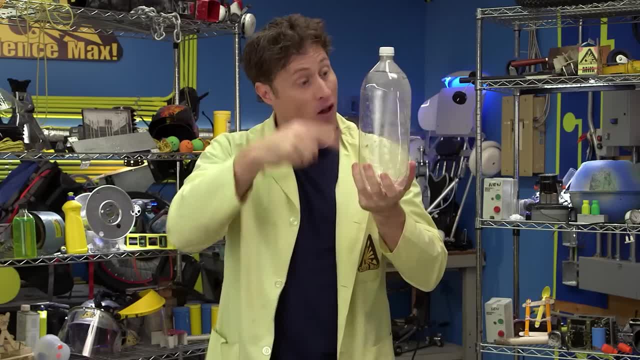 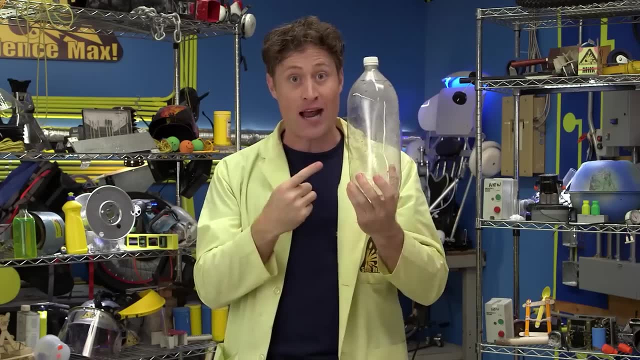 There's about 4 million air molecules inside this bottle, but they're all hot air molecules and they have a higher pressure and you don't notice it because the air out here isn't crushing the bottle. But watch what happens if I cool the air inside the bottle. 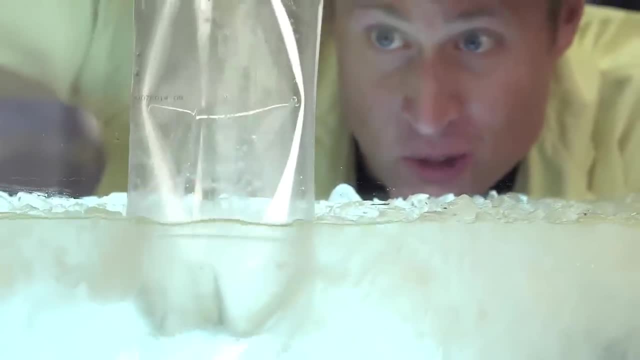 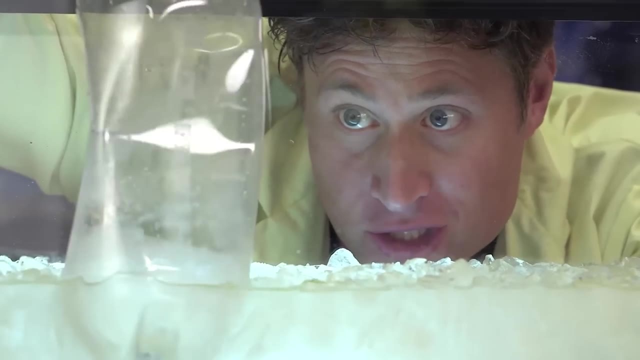 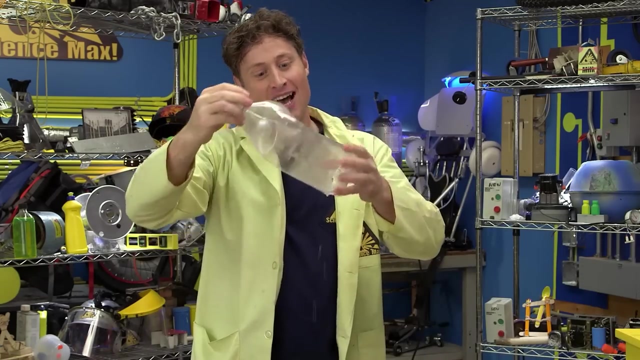 This is ice water. So what's happening now is the molecules are slowing down and they need less space, So they need less room, and they're being crushed by the pressure on the outside of the bottle. It has been crushed because the colder air molecules 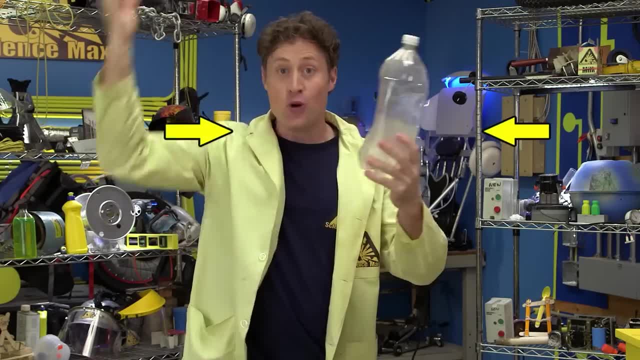 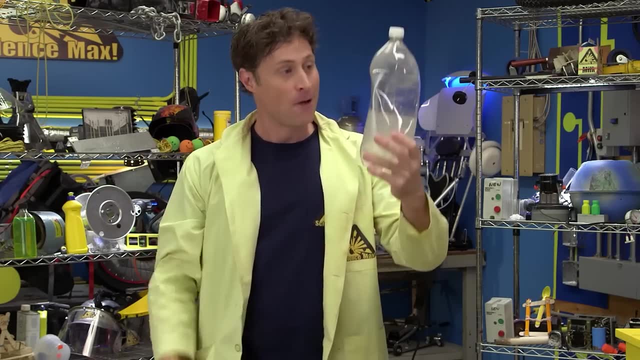 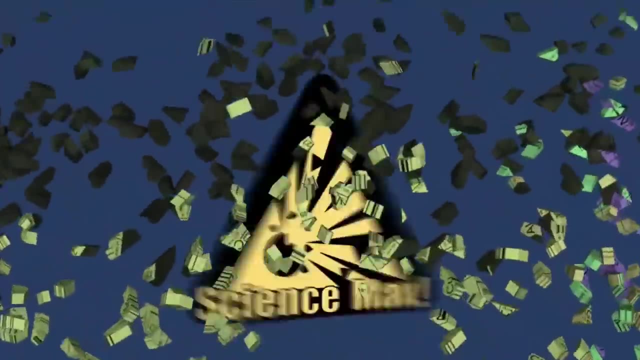 don't need the same kind of room as the hot air molecules. the room temperature air has crushed the bottle. The air inside has a lower pressure than the air outside. Pretty amazing. Even more amazing when we max it out: This is a steel drum. 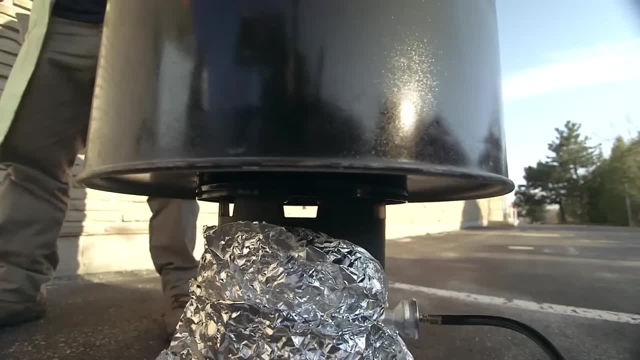 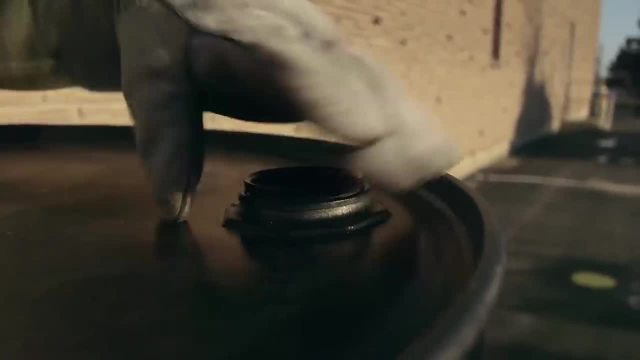 What we've done is we've put some water in it and we're heating it up to boiling, so there's nothing but hot air inside the drum. This is an airtight cap which we use to seal the drum, And now we cool the drum off. 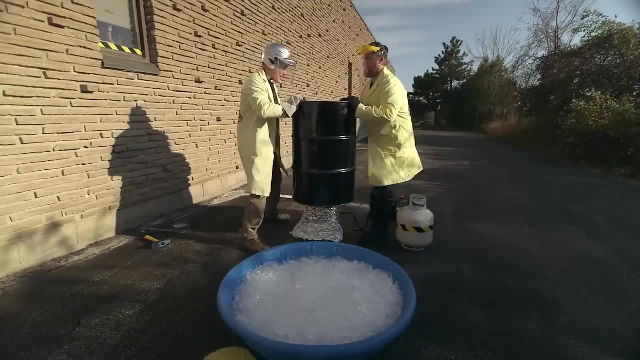 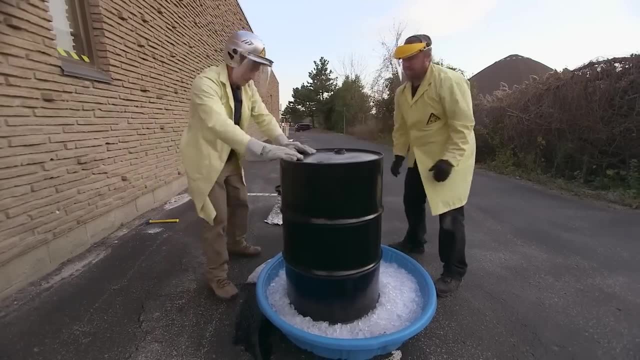 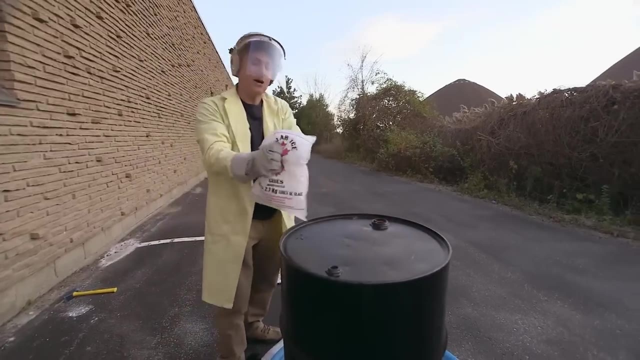 Hey, Trevor, give me a hand Ready. One, two, three, you lift. That's good, This pool is filled with ice. What we're doing now is cooling off the steel drum, which will cool off the air inside it. 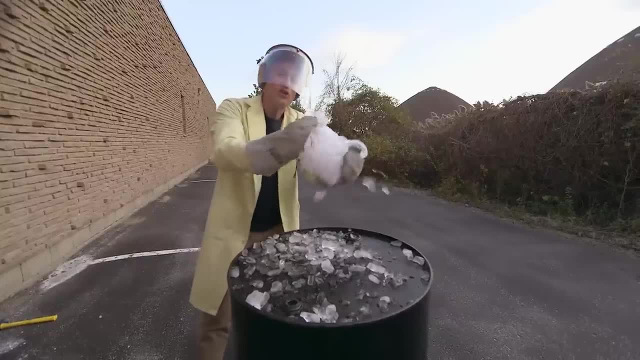 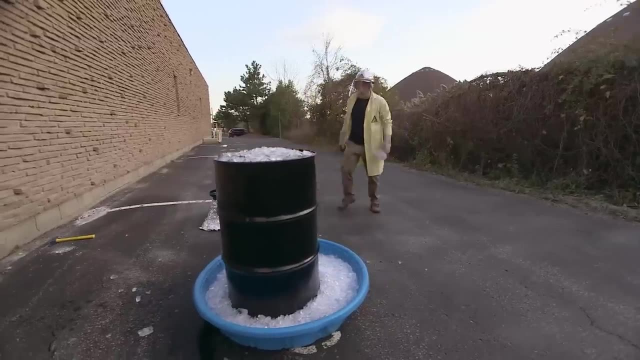 Which means eventually, the air inside the steel drum will be a much lower pressure than the air outside the steel drum. Because the steel drum has a lot more volume than a two-litre pop bottle, it takes a lot longer for the air to cool down. 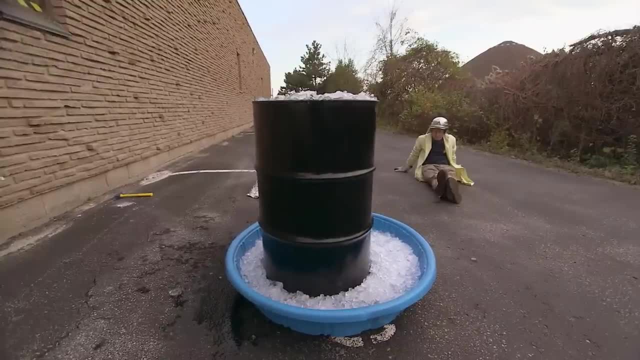 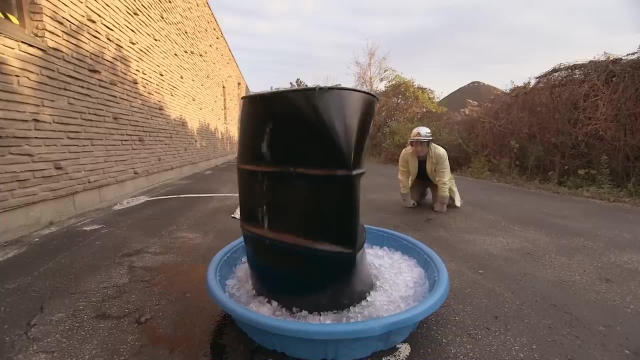 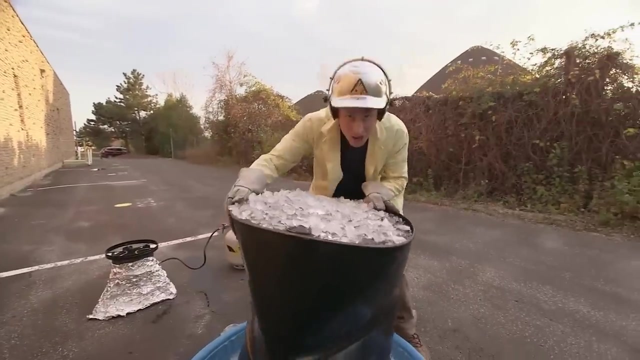 The other thing to think about is that it's a steel drum. I could stand on it and it wouldn't even dent. But sure enough, after a few minutes- Whoa, Check it out- The barrel has totally crushed. The low-pressure air inside the barrel wasn't enough. 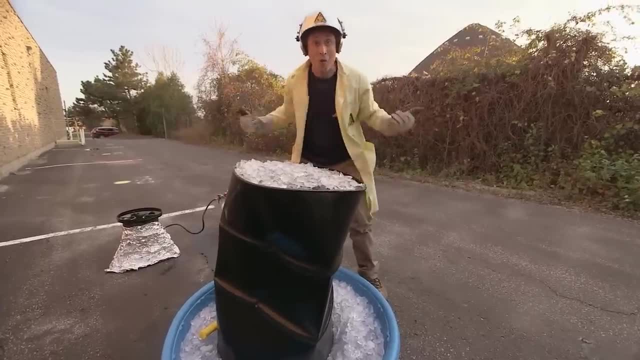 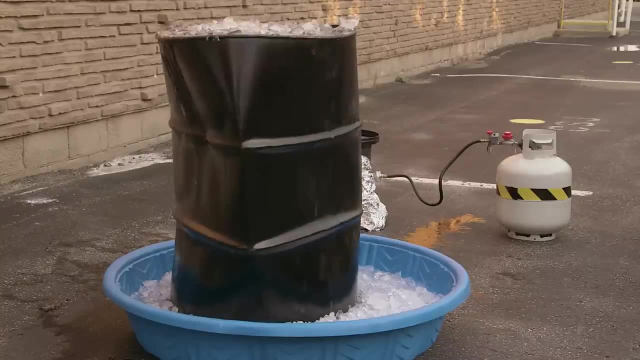 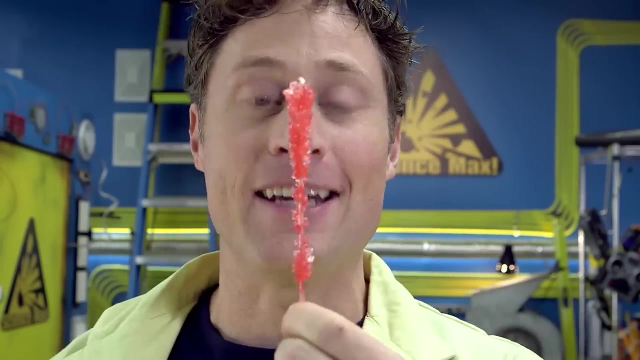 to withstand the force of the regular air pressure that you and I walk through every day. The air pressure all around us is enough to crush a steel drum. How cool is that? Mmm, this science is delicious. This is rock candy. It's basically crystallized sugar. 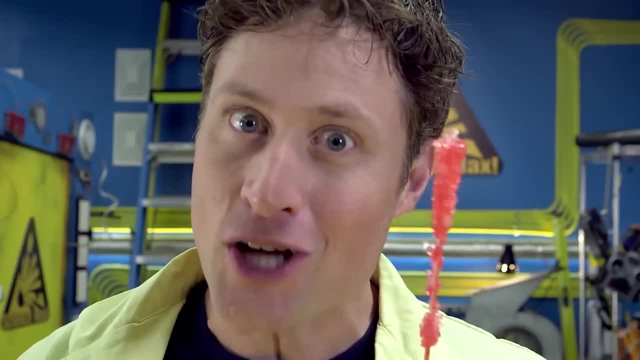 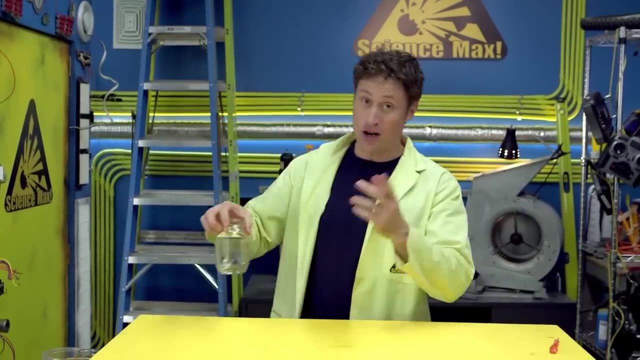 And you make it by turning a solid into a liquid and then back to a solid again. Here's how you can make it at home: You need a container that you're not going to need for a while and some water, some sugar. You can use brown or white. 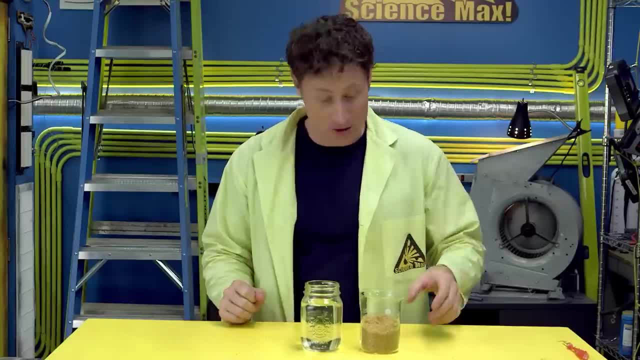 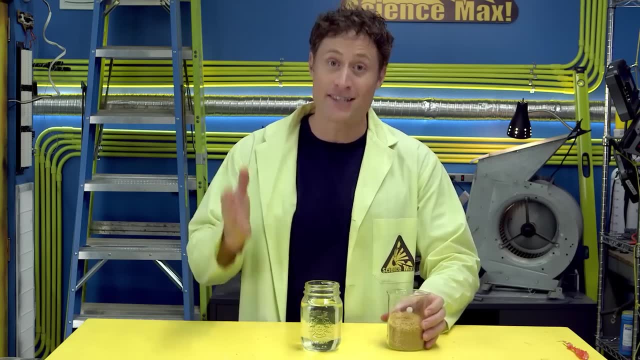 I like to use brown And an adult. Here's why you need an adult. You want to dissolve three cups of sugar into every cup of water And you can't do that unless you heat the water. So get an adult, a saucepan and heat the water up. 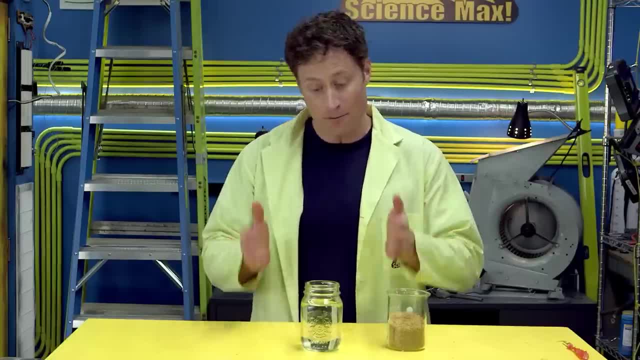 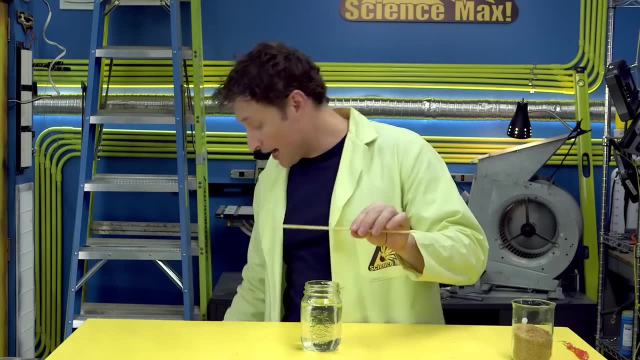 Pour the sugar in and keep stirring until it's all dissolved. Then pour it in your container and let it cool down. Then you'll need A shish kebab skewer, which is something you can get at the grocery store. Cut it down to the right size. 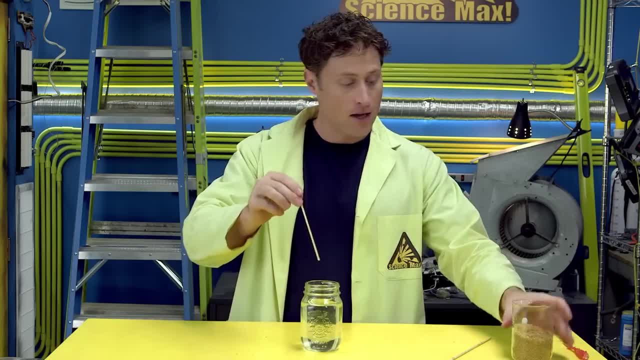 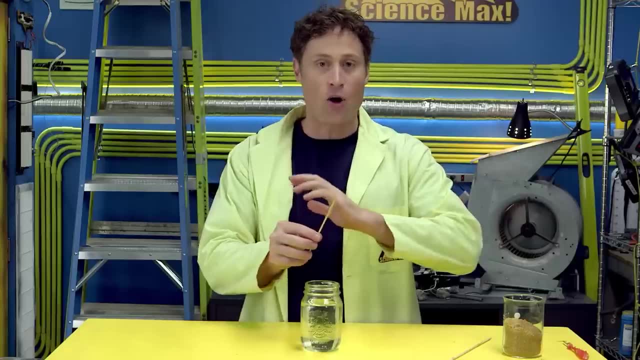 so it fits nicely into your container, And then dunk it in your sugar and get some crystals coated around the stick. These are seed crystals and they get the whole process started, And now you have to wait for these to dry, otherwise they'll just fall off the stick. 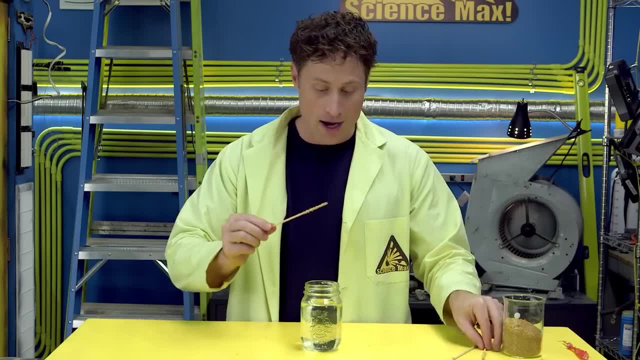 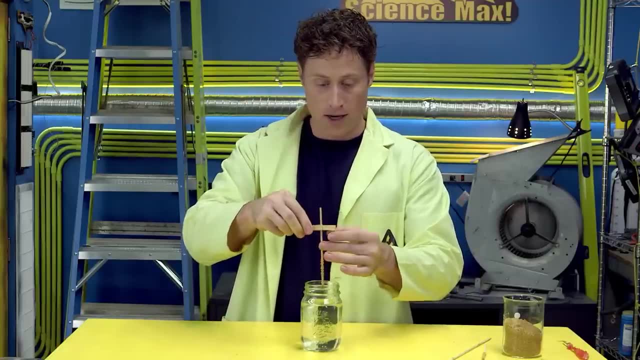 when you put it in the water. So I've got one here that has dried out. You'll also want something to keep it from falling in the top of the container, So I'm going to use a clothespin, Put it in there and dunk it in the container like that. 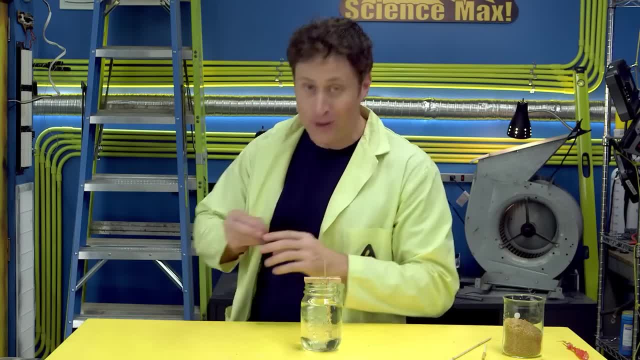 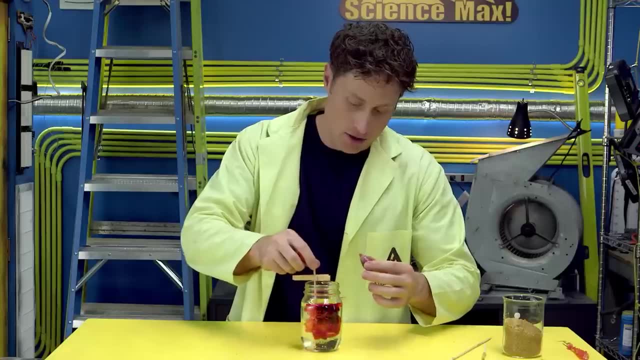 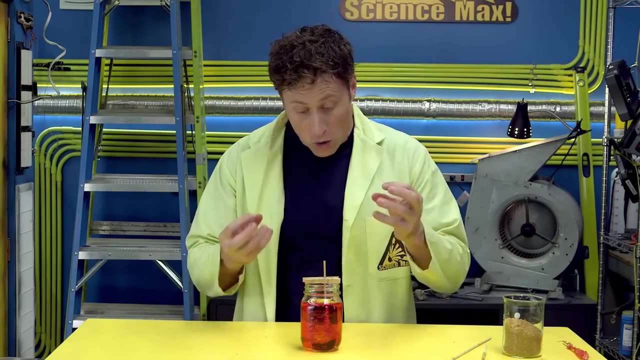 And now for the final step. if you want, you can add food coloring. I like to use red because it reminds me of science, And I'm going to use the stick to actually stir that up a little bit. There we go Now the dissolved sugar crystals in the water. 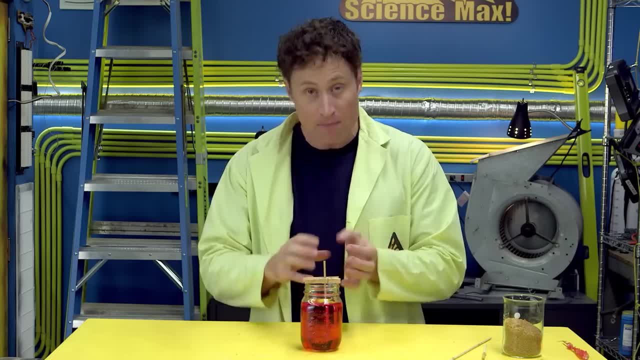 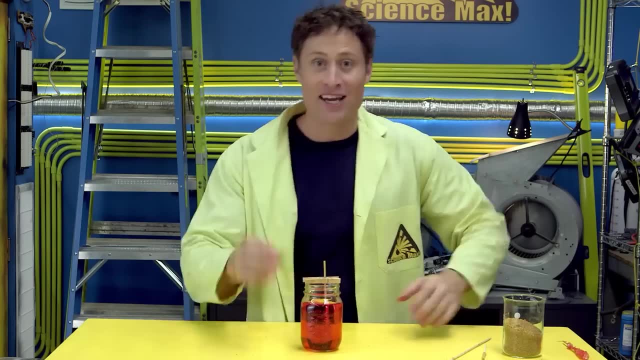 will slowly grow on the crystals that are already attached to the stick and it will eventually grow into a rock candy Pop, But it takes about a week. No, I'm just kidding. I've already got one that's standing by. Here we go. 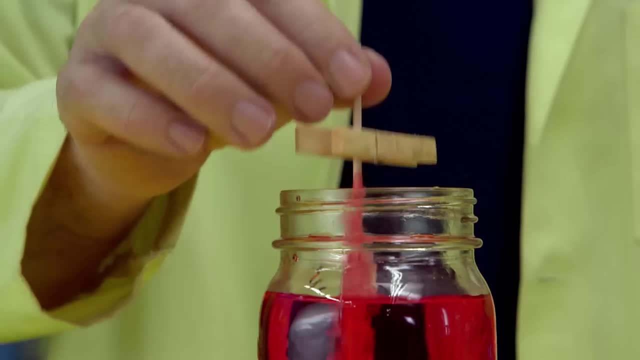 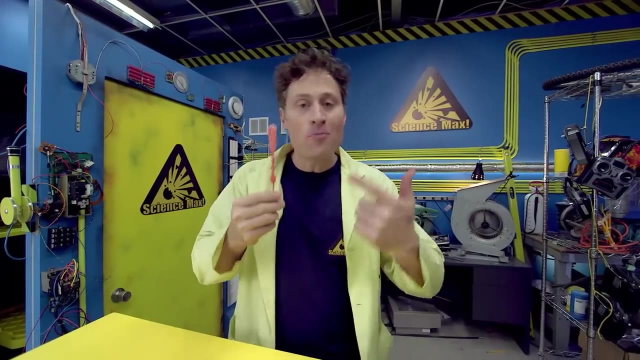 This one has been growing for about seven days And there you go: rock candy, Delicious science. Now how can we make this any better? I mean, it's crystallized sugar. It doesn't get any more maxed out than that, does it? 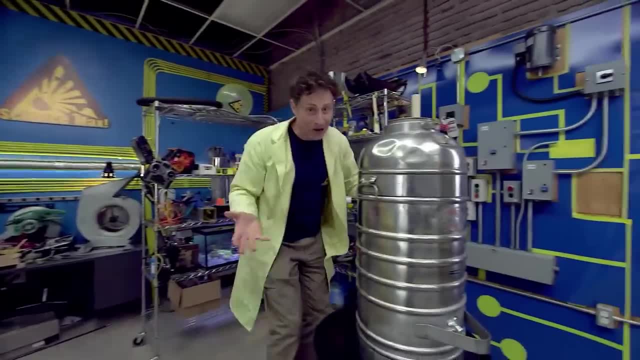 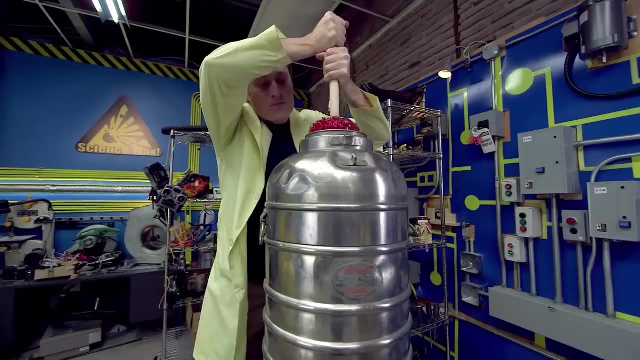 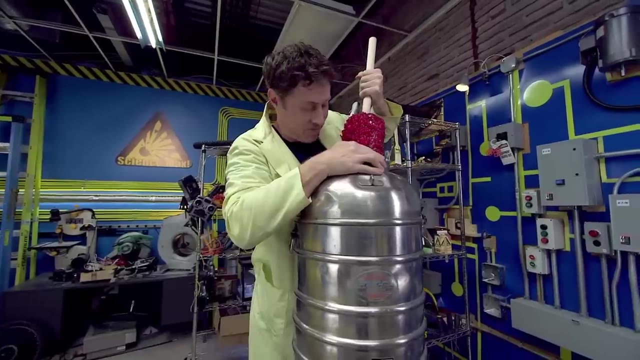 Yeah, it does, Come on. This is a giant container of sugar water and I've been brewing a massive rock candy crystal in it for a while, But it's sort of getting a little bit too big to fit out the top of the container. 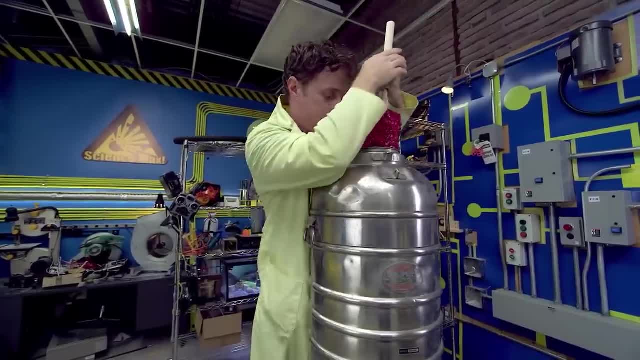 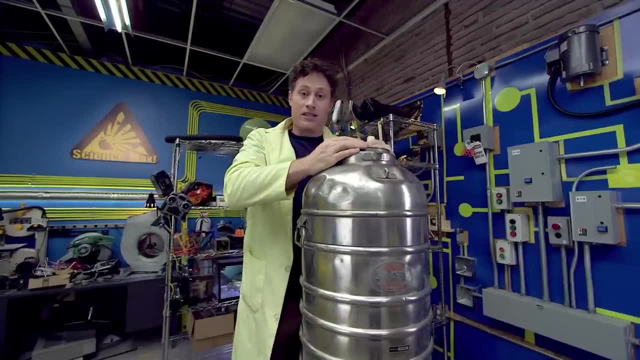 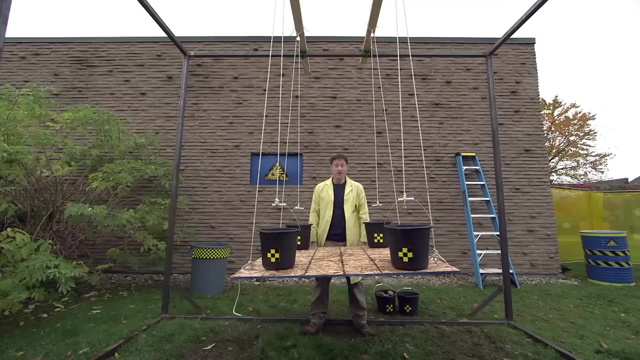 So you know what? I'm just going to put that back in there and chalk that one up to science, Because, well, eating a rock candy crystal that big would definitely not be good for my teeth. So yeah, Yeah, Here is something mind bending you can do with pulleys. 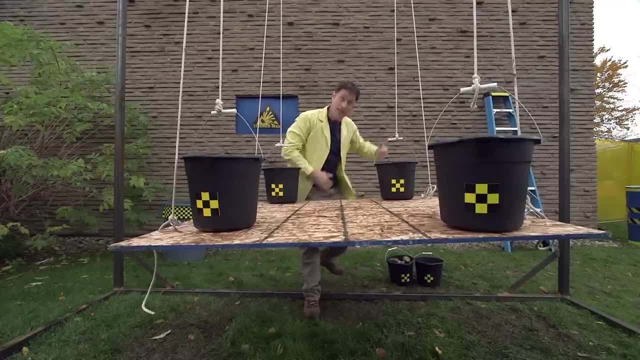 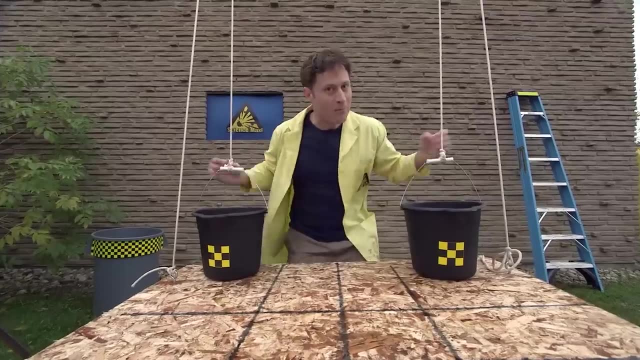 These buckets are attached to the table through a pulley. There's nothing holding this table up except for the weight of the buckets pushing down on the table. So if I took the buckets off the table, the weight of the buckets pulls the table up. 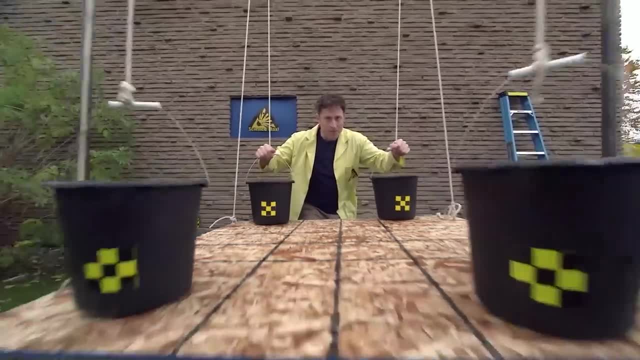 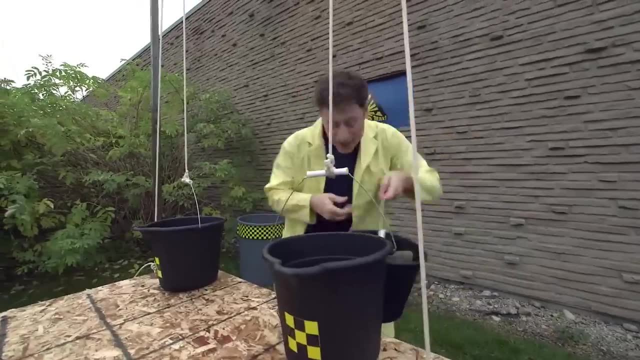 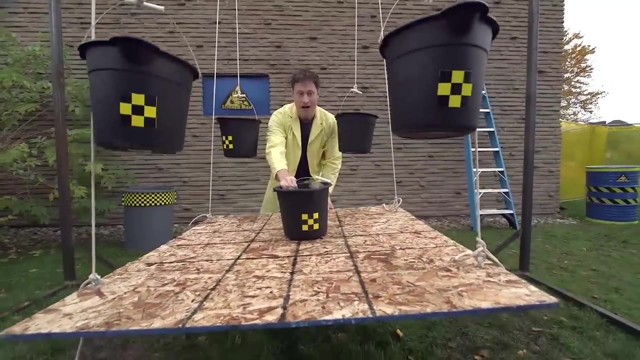 But because the buckets are on the table, everything is in balance, Mind bending, right, OK, wait, it gets better If I took a weight and I put it on the table. the weight of the buckets isn't enough to keep the table up. 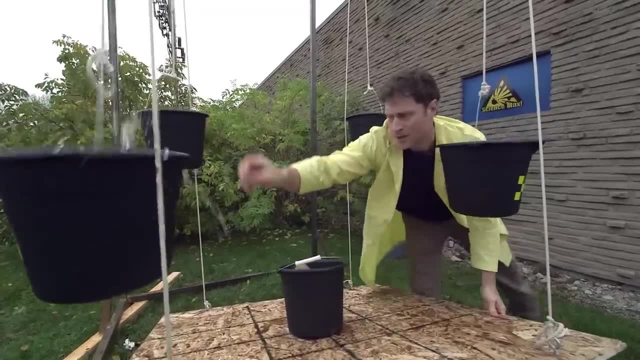 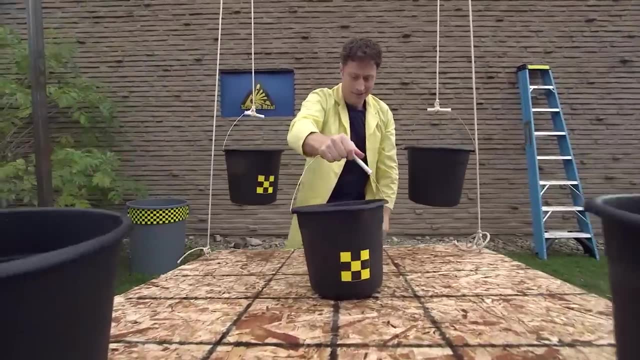 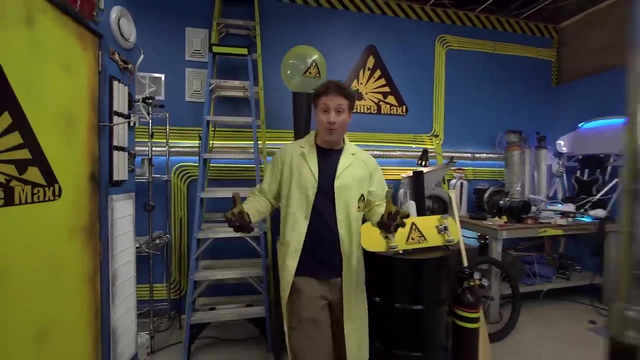 So I have to add more weight to the buckets, so the buckets pull the table up And there you have it. It's weird, It's mind bending. It's science. Today we're combining two different chemicals to create a reaction. Sometimes chemicals can combine in a way. 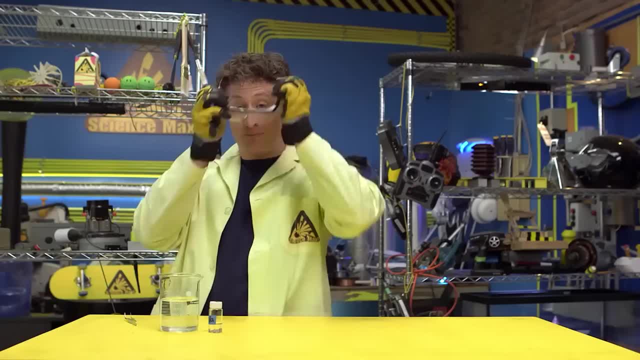 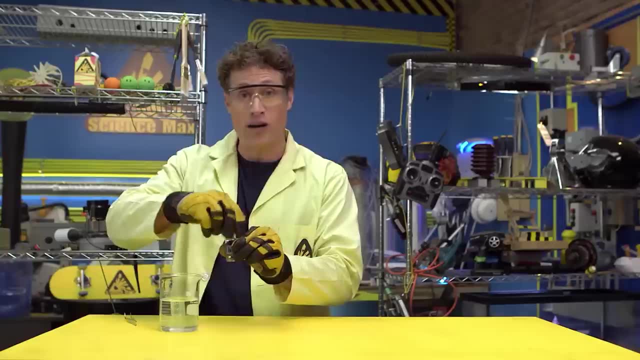 that makes them very different from how they started out. For example, this is sodium or Na on the periodic table Now. the sodium tablets are in mineral oil because sodium reacts very strongly with water, even the water in the air or especially the water in my skin. 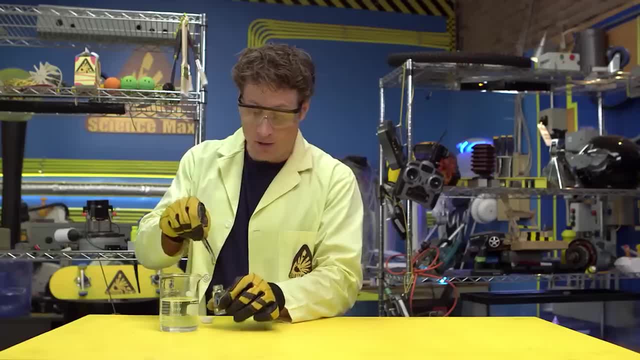 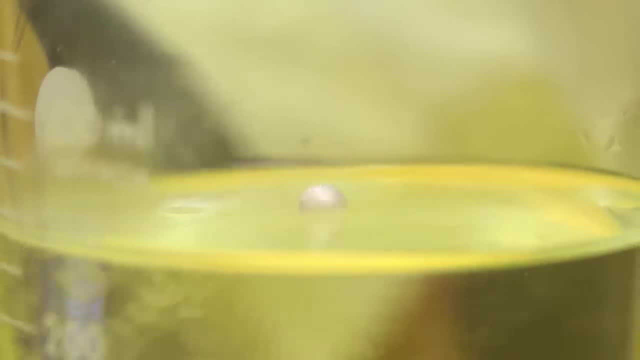 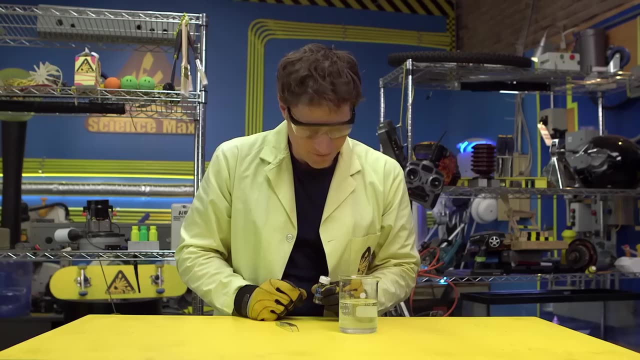 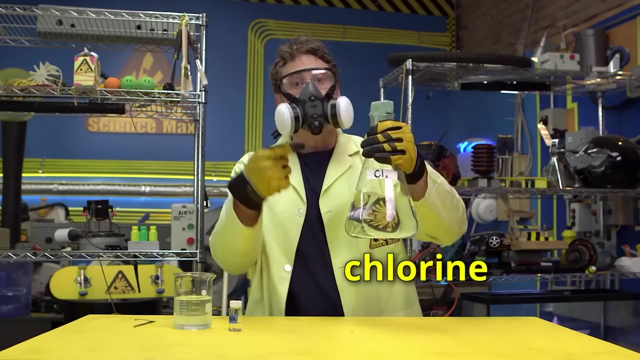 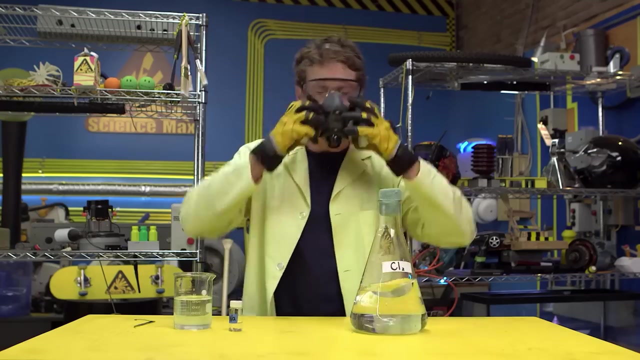 Watch what happens when I drop a sodium tablet into this beaker of water. Very cool and very dangerous. And this is chlorine or Cl on the periodic table. Chlorine gas is very poisonous. So what happens if we combine these two deadly substances? 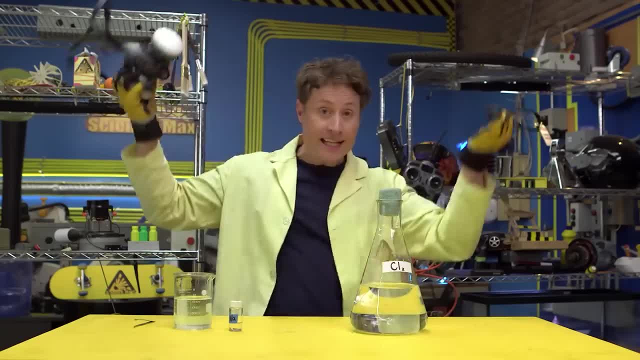 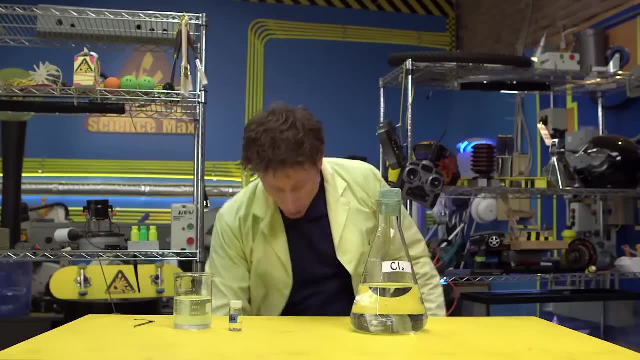 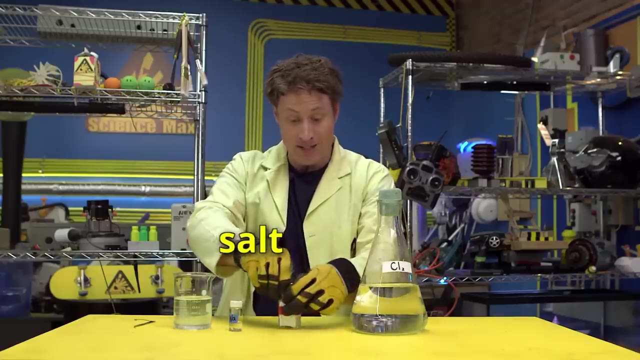 Do we create some sort of super poison? something more deadly than anything else known to science causes fear and chaos in chemistry labs all over the land. No, we create salt: Good old, normal table salt. These two substances combine to make NaCl salt. 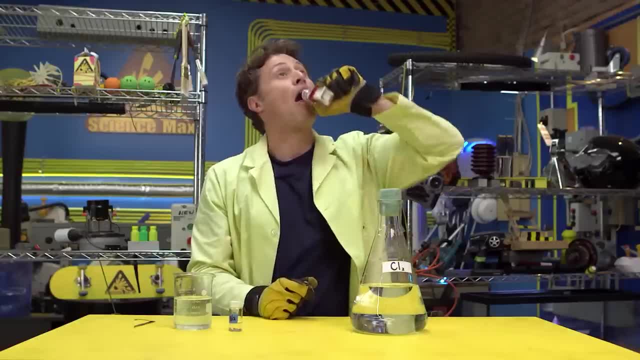 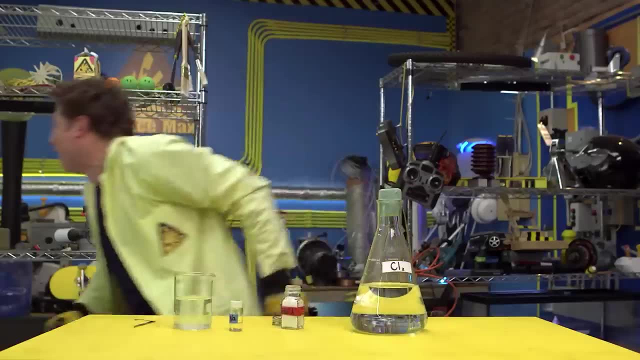 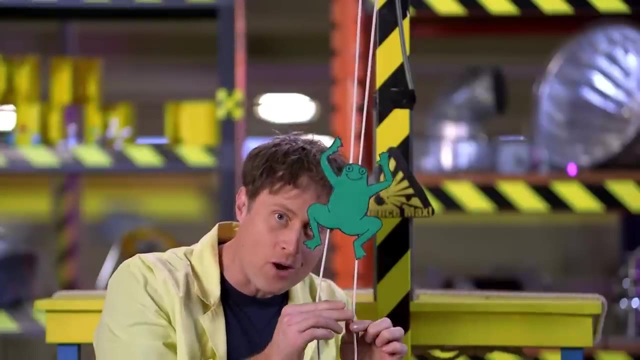 Something completely and totally safe Chemistry. This is a climbing frog. Why does it climb? Because of science. I pull on this rope and then I pull on that rope, and I pull on that rope and that rope, and he climbs up the ropes. 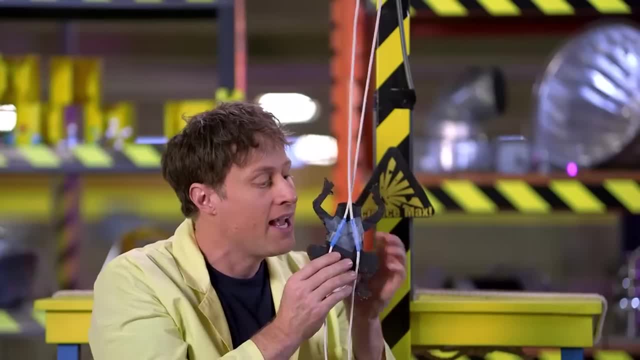 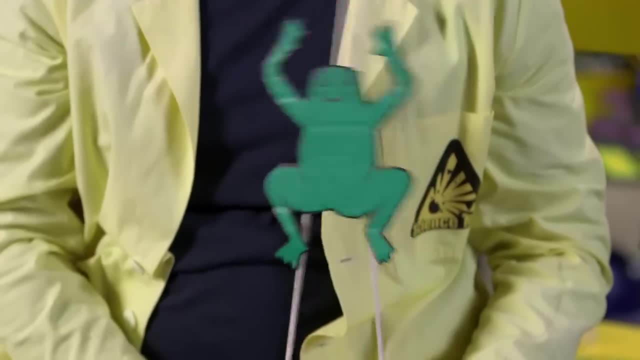 And why? Well, because of friction. The secret is two straws. The straws are pointed away from each other at the bottom. This allows it to climb, thanks to friction. Take a closer look. When I pull on one string, it pulls straight. 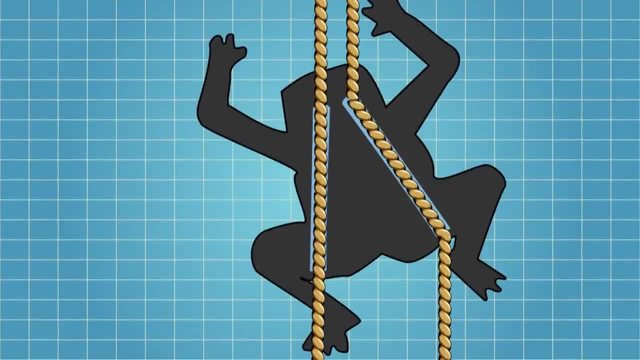 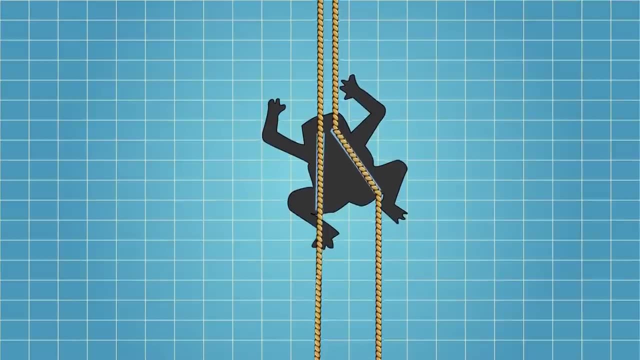 which makes the frog pivot. That string slips through the straw because there's not a lot of friction, But there's lots of friction on the other side because of the angle. So one side of the string goes down, which makes the other go up, which means the frog goes up. 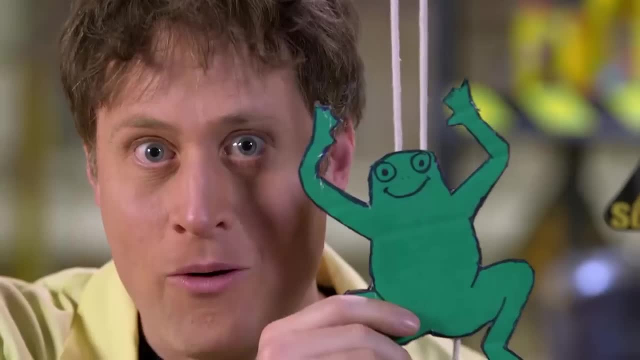 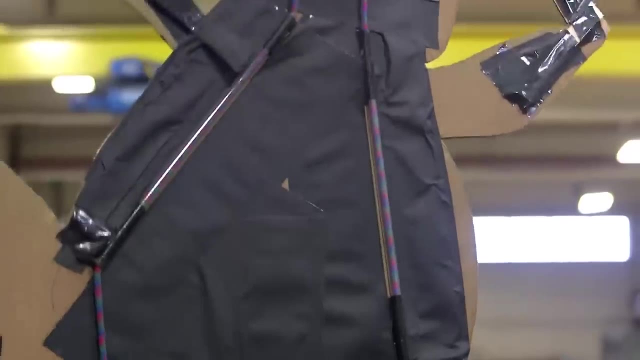 with it, all thanks to friction. So now let's max it out. This is a super maxed out climbing frog, Just like the small version. I have a rope going through two tubes. I pull on one rope and the other holds on by friction. 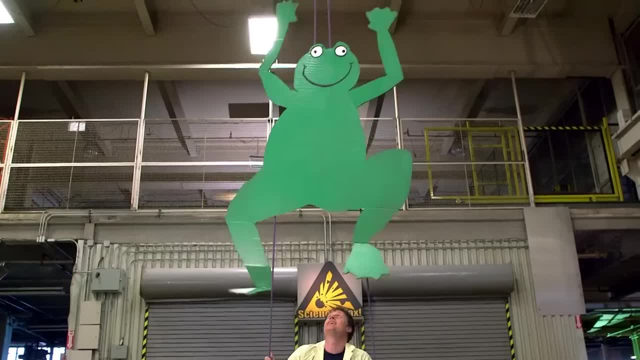 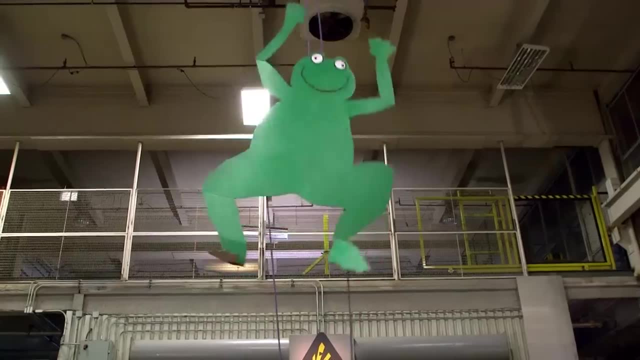 Then I switch And it does work. It's just a lot harder to pull on the ropes, But it does work. It totally works. Whoa, Yes, Whoa There, And then this one, And then that one, And then that one. 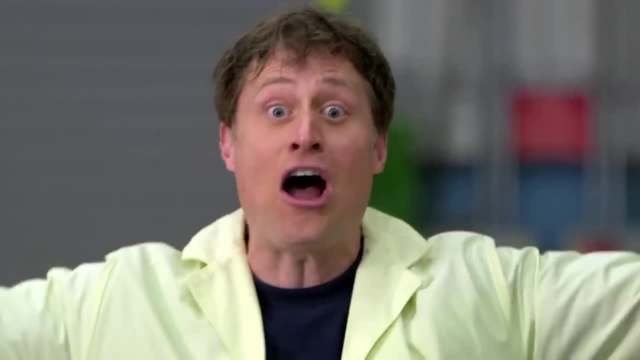 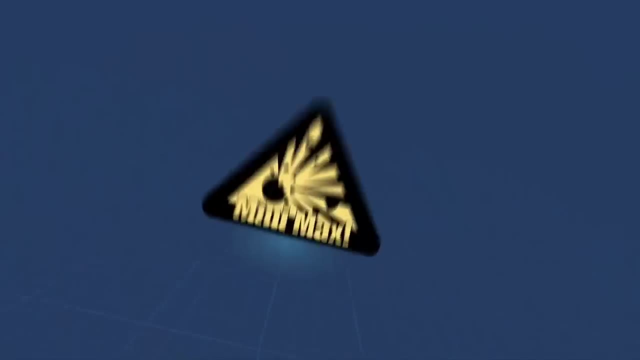 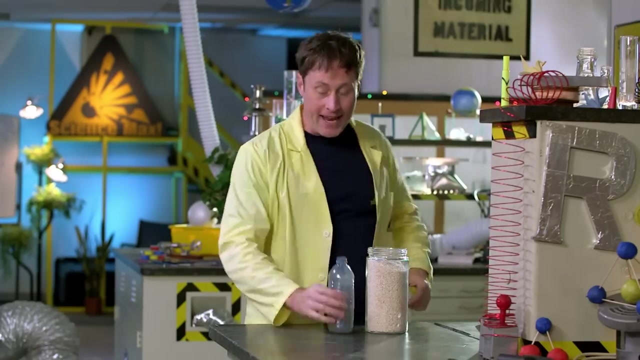 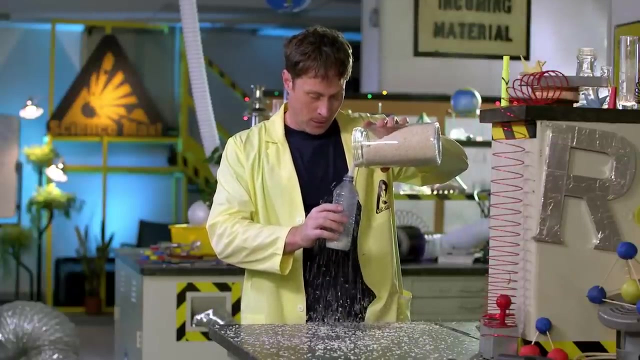 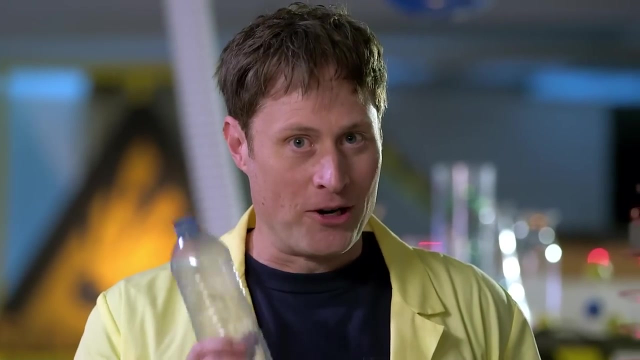 Yeah, A giant climbing frog, All because of friction. Here's another way to defy gravity: using friction. Get a plastic water bottle and fill it with rice, Take two. So get a plastic water bottle and fill it with rice using a funnel. 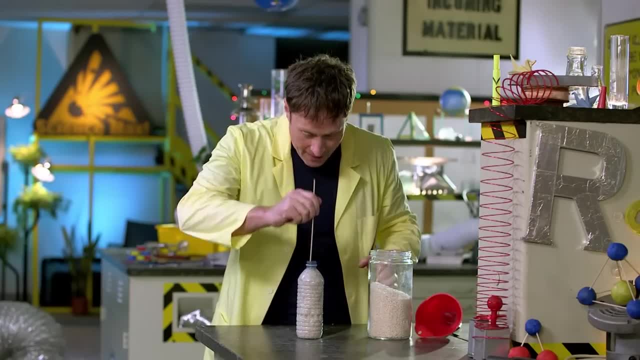 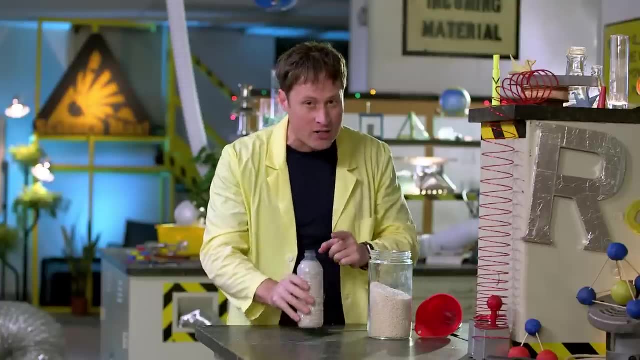 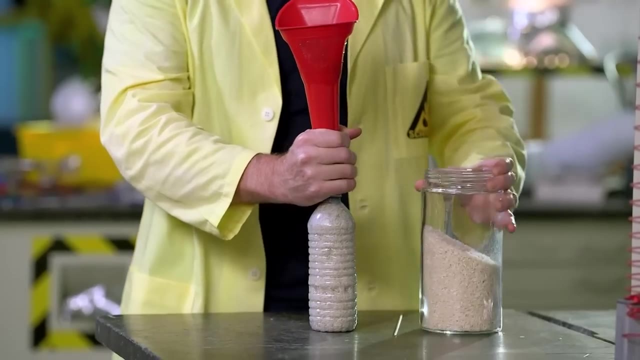 Then take a shish kebab skewer and stick it into the bottle And nothing happens. But if you tap the bottle down, the rice starts to pack in a little bit better. See how the level of rice is lower, Which means you can add more rice. 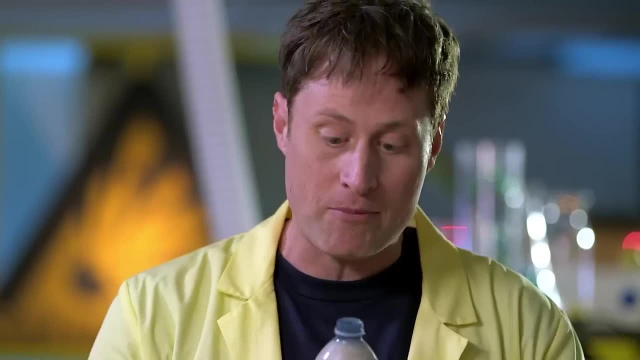 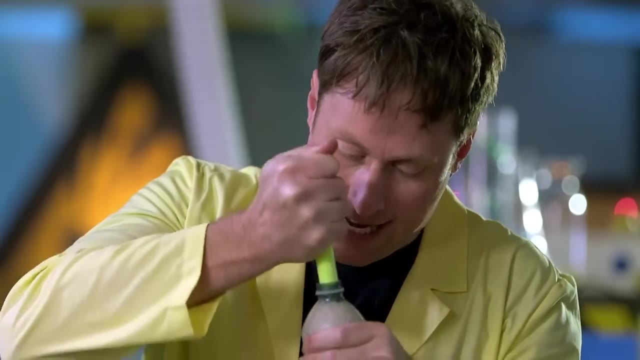 Pack it down even more And you can even use something the same diameter as the mouth of the bottle, like, say, a highlighter, And make sure all the rice is as packed in as you can get it There. Now, the rice is really packed in there. 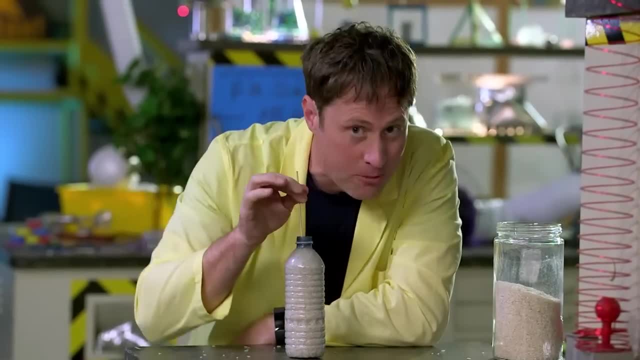 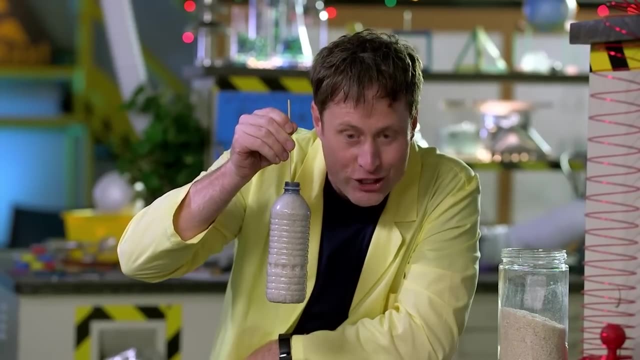 And when I stick the shish kebab skewer in the friction between the pieces of rice and this wood is enough to lift the bottle, The bottle using nothing but friction. Now let's max it out. I filled this 20-liter water cooler jug full of rice. 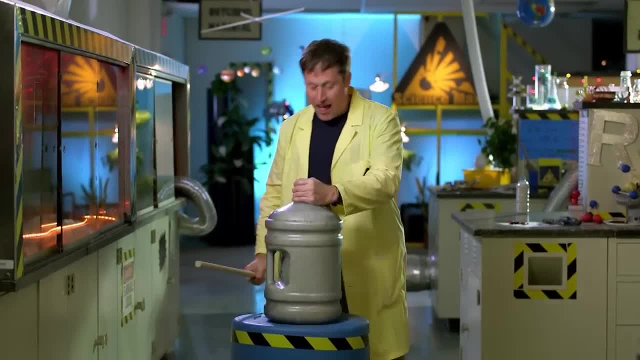 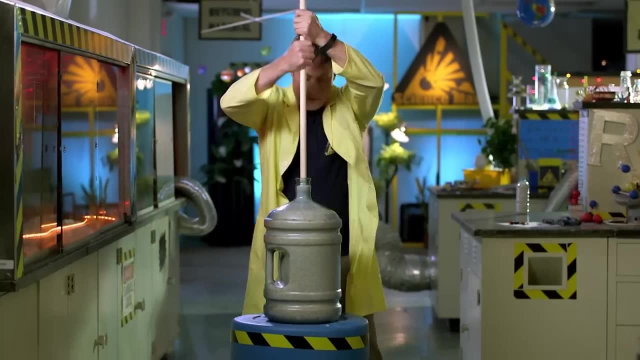 And it's really, it's really heavy. I wanted to see if I could lift it using nothing but friction and this dowel, which is just a round piece of wood. All right, here we go, Ah-ha-ha-ha. 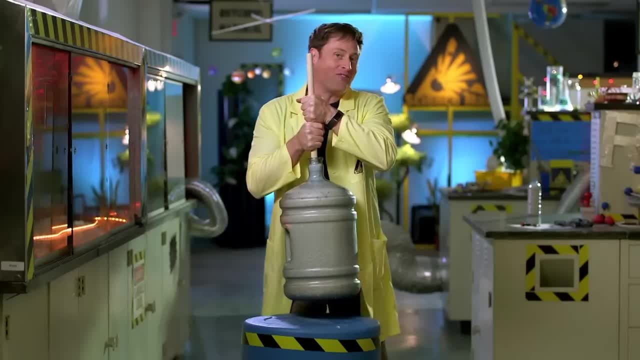 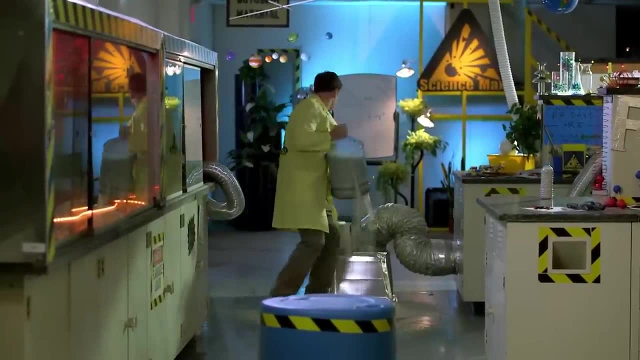 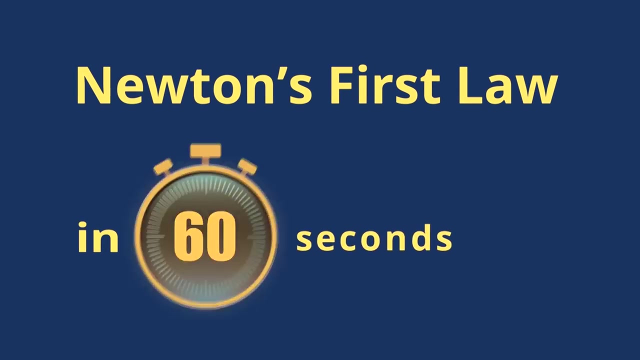 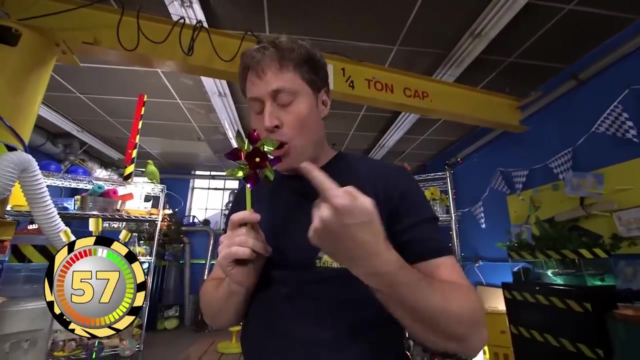 Science. I'd max it out even more, but I don't think I could lift anymore. Ah-ha-ha-ha, It's okay, I could just fit Um Newton's First Law in 60 Seconds. Newton's First Law says an object in motion tends to stay in motion. 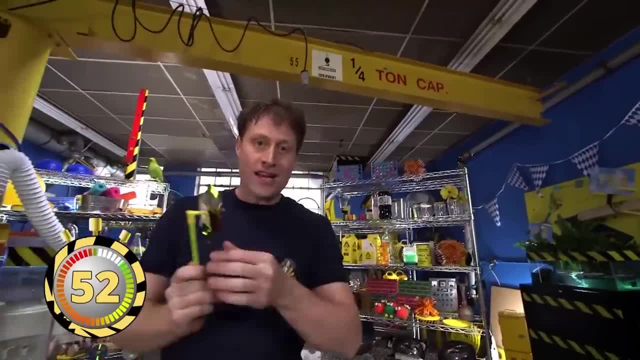 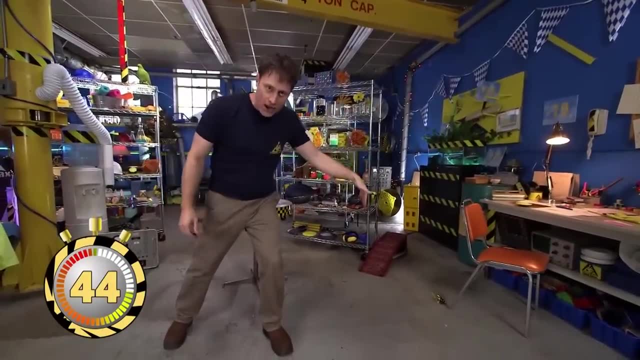 So why don't they See if I was to throw this? It doesn't stay in motion, It doesn't keep going, It slows down and falls to the ground. Well, the whole law states: an object in motion tends to stay in motion. 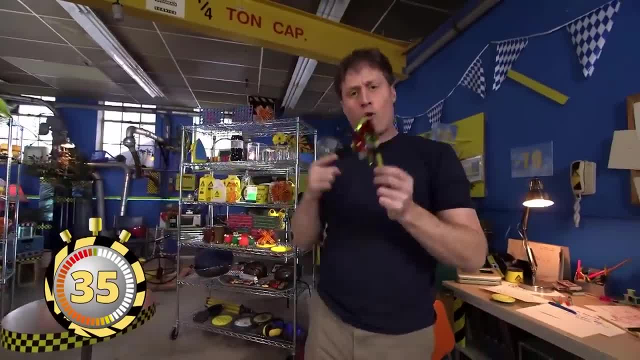 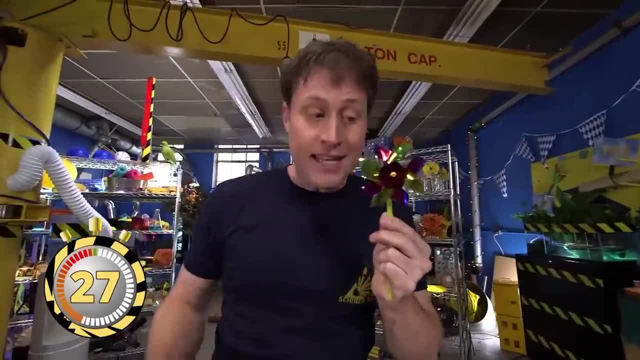 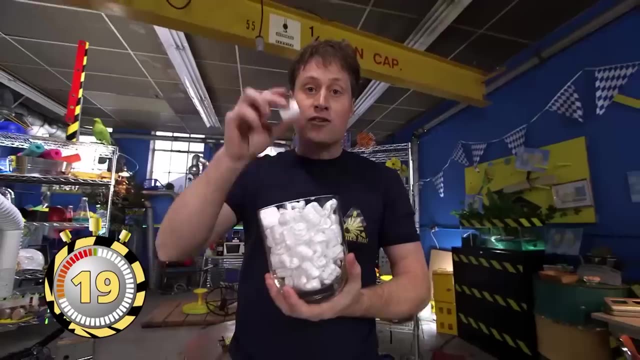 until an external force acts upon it. So what forces are acting upon this? Well, gravity for one, pulling it down towards the ground, and friction, specifically air friction, slowing this down and making it stop. Now, if you were to have something very light with a lot of surface area, 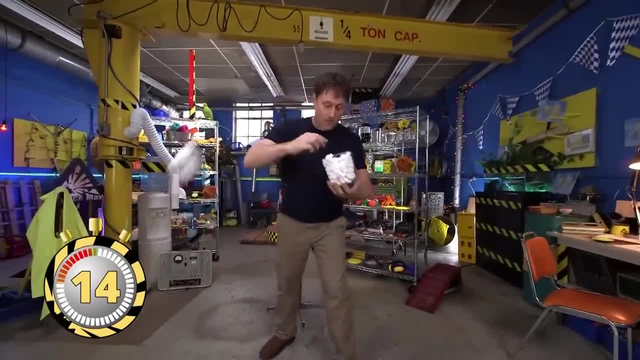 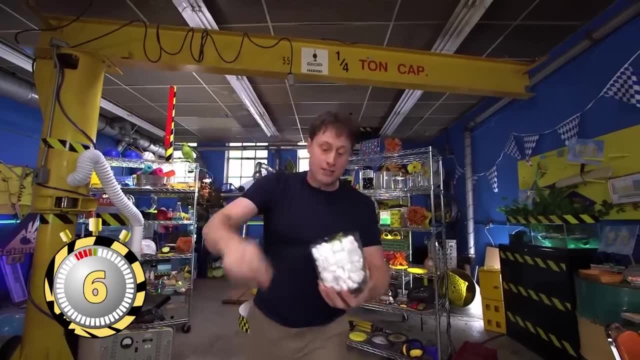 it would really be affected by air friction. You wouldn't be able to throw it very far, Not very far at all, no matter how hard you tried. So there you go. Newton's First Law: An object in motion tends to stay in motion. 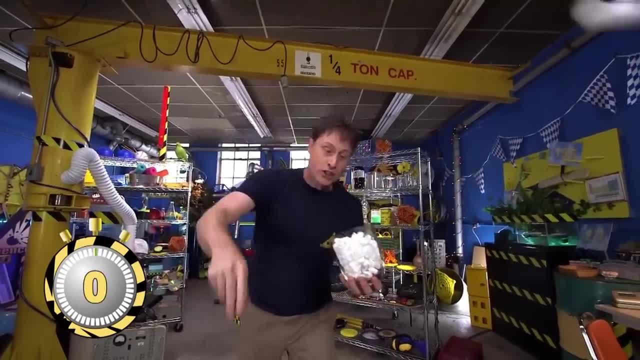 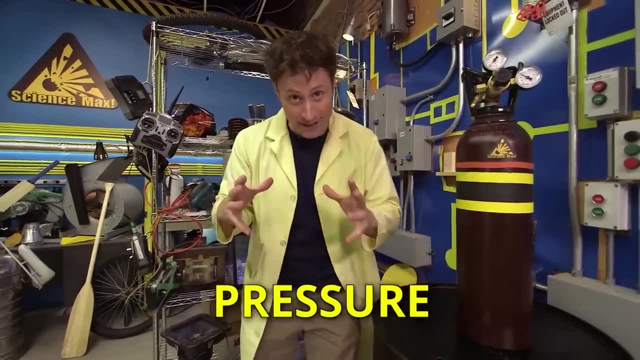 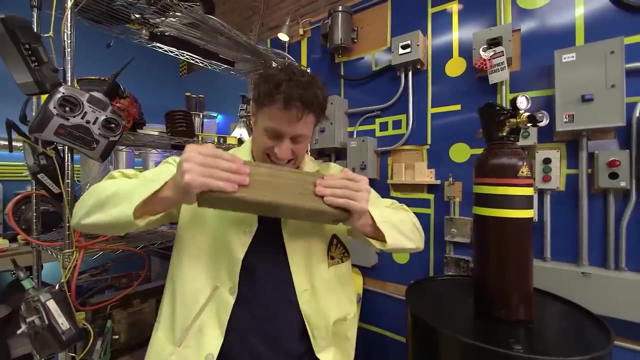 unless it's affected by an external force such as friction, like air friction. So there you go. Pressure happens when you squeeze something or compress it. Solids do not compress very well. I will demonstrate Um Solid Is it compressing. 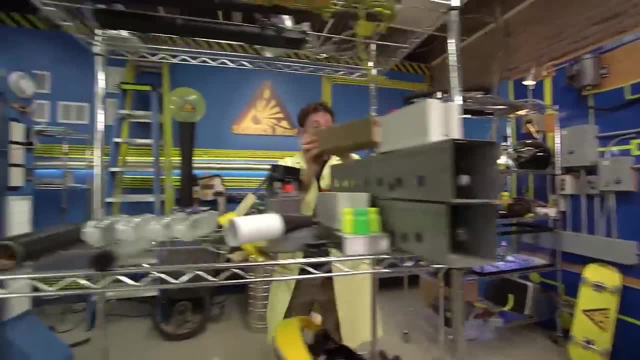 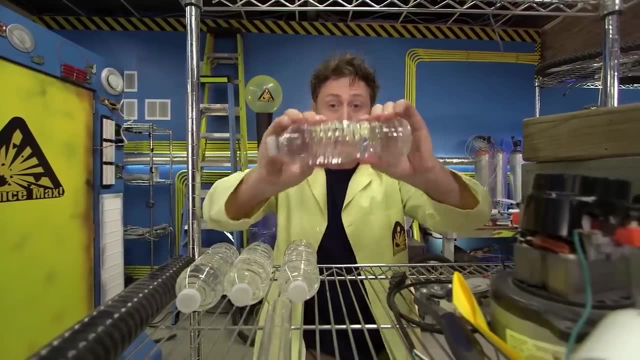 No, okay Liquids don't compress very well either. You can demonstrate this for yourself by getting a plastic water bottle and filling it right to the very top with water and putting on the cap and squeezing. You'll find that you can't really squeeze the bottle very much. 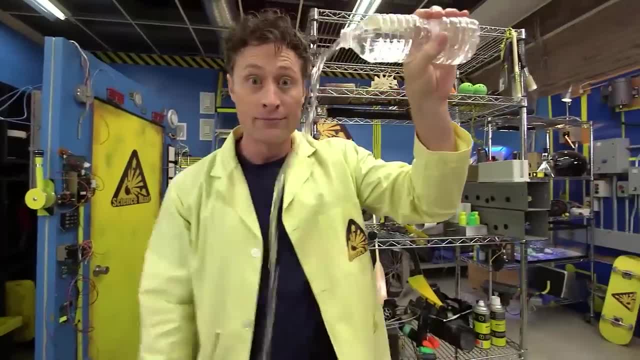 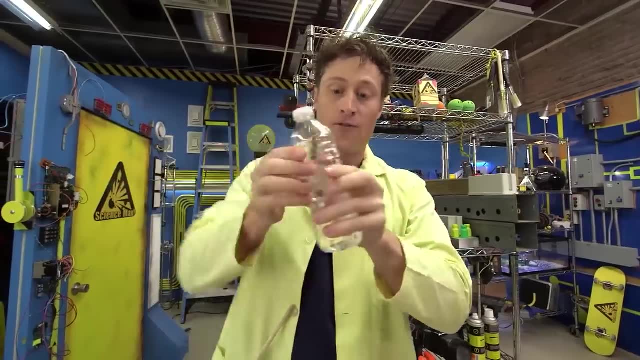 But if you empty out half of the water- No, don't pour it on the floor And then put the cap back on the bottle and try to squeeze it- you'll find that you can squeeze it a lot more. That's because gases. 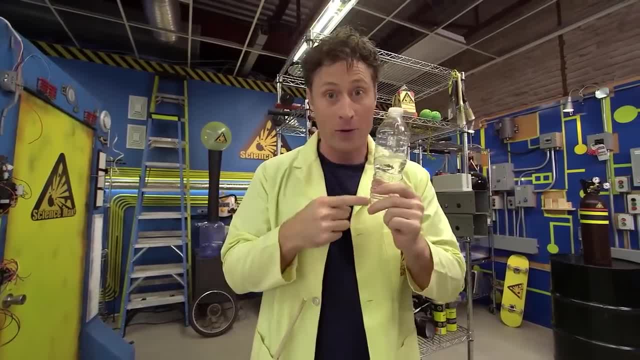 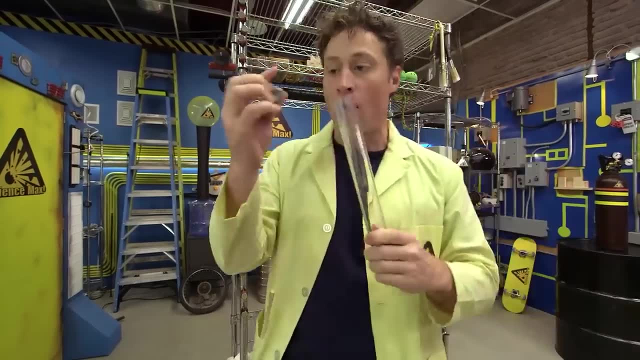 because gases compress much easier than solids or liquids. Here's what's going on. Say: this container is well, any container, And these magnets are air molecules. Now I'm going to put the magnets in pole to pole so they repel each other. 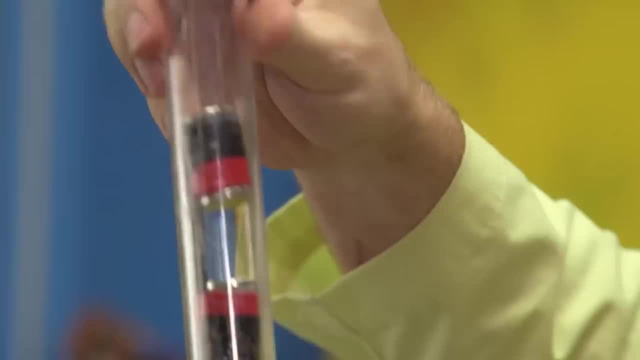 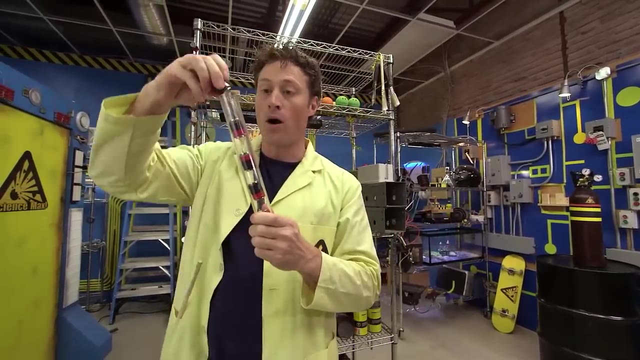 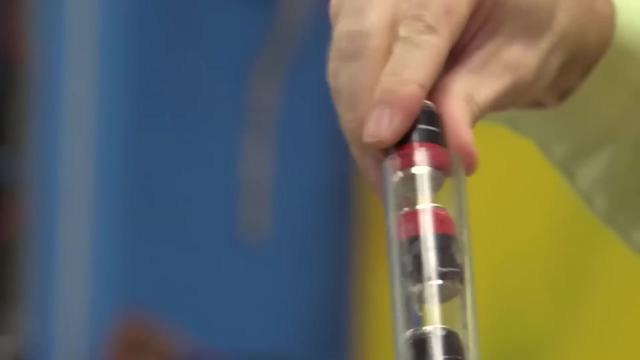 and want to stay a certain distance apart, just like air molecules do. There we go, A container at normal gas pressure. Now watch what happens when I add more gas molecules. They start to get squeezed together, And if I add more, the amount of space that each one gets is less and less. 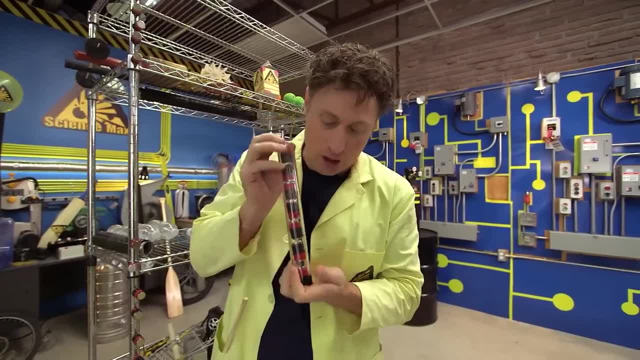 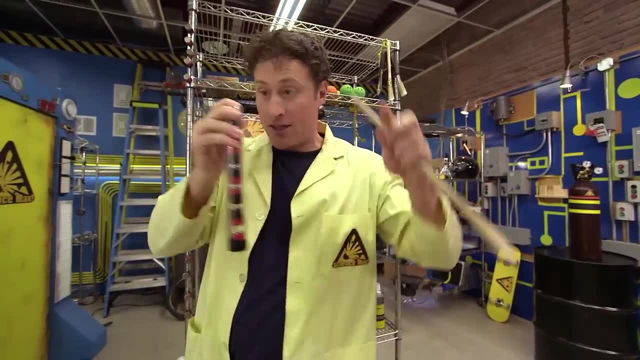 Now this container is under a lot of pressure. These molecules really want to escape through the top of the container but they can't because I'm holding them down. If I took something like this plunger and I pushed them down even more, now they're really under pressure. 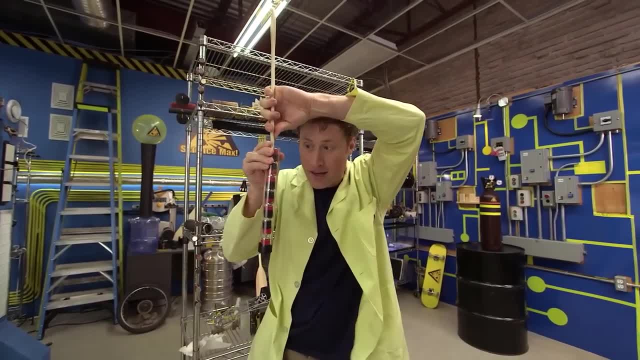 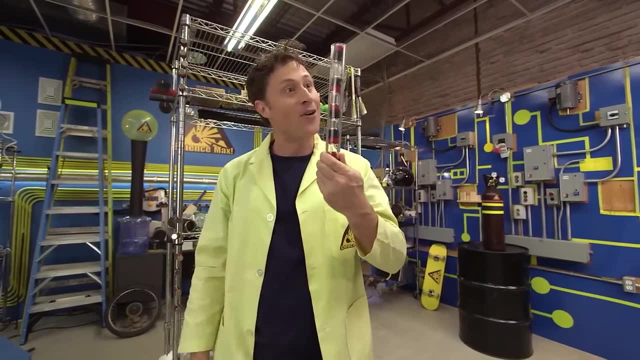 They want to get out, but they can't because I'm holding them in. Now watch what happens when I add more gas molecules. When I let them go, they all pop out the top and the container has returned to normal gas pressure. That's what happens. 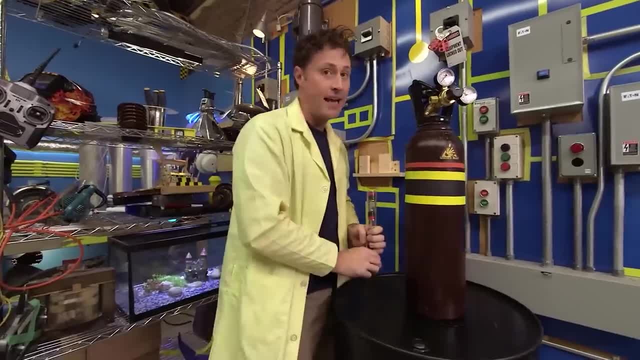 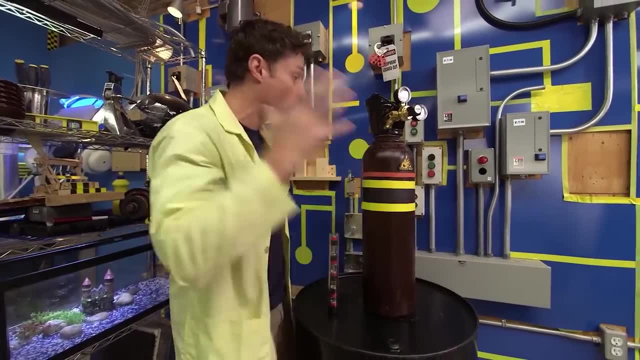 when we put gas in a container like this one. These containers that hold compressed gas are made out of solid steel because you need something really strong, or it might explode if you put too much gas pressure in it. That's why these are only filled up by professionals. 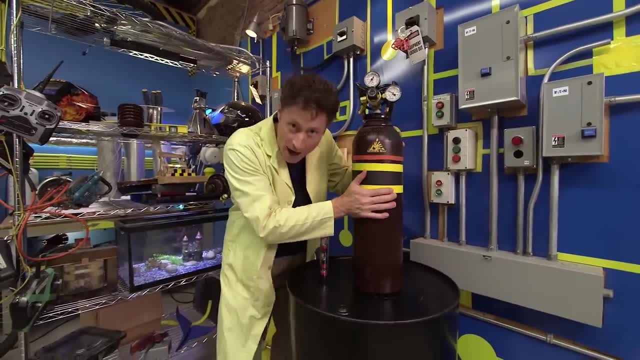 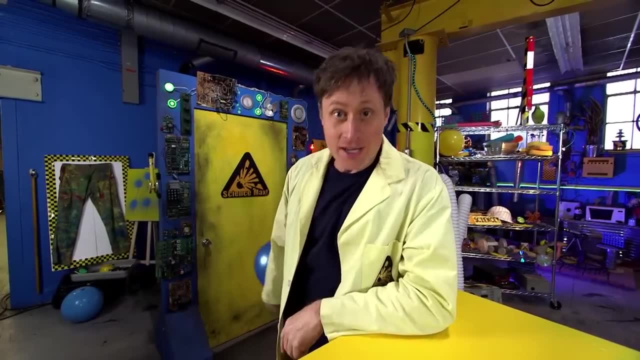 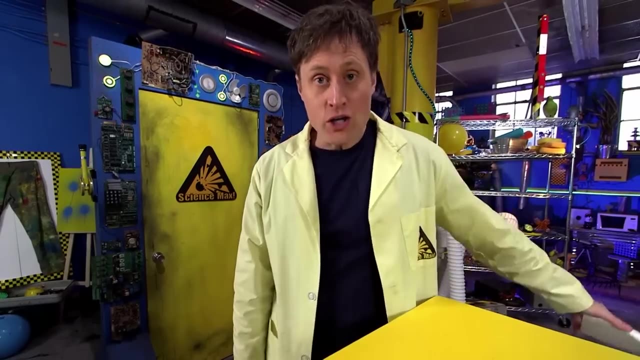 who know exactly how much pressure it can take. And that is the power of pressure. Our maxed-out mousetrap boat isn't the only way to give a boat propulsion. Let's look at another way: using a balloon. Let's make a balloon-powered boat. 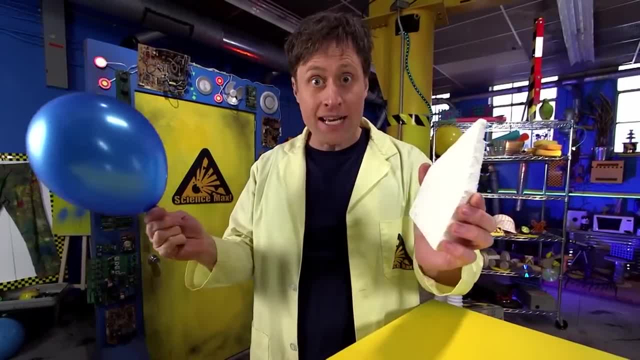 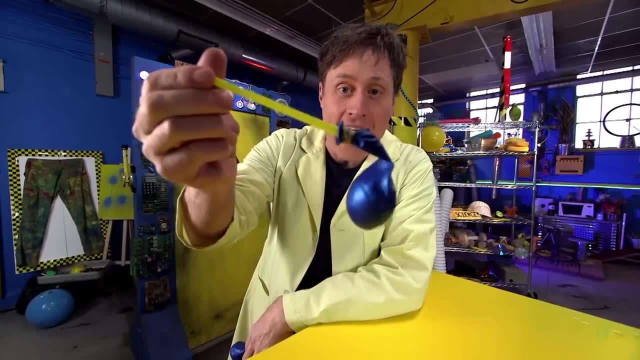 All you need for that is something to be your boat and a balloon. Then you attach them together. Actually, the best way to do it is use a straw and attach the balloon to the straw using an elastic band, And then you attach it to your boat. 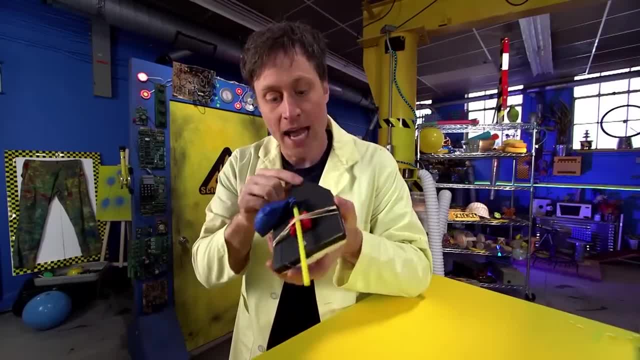 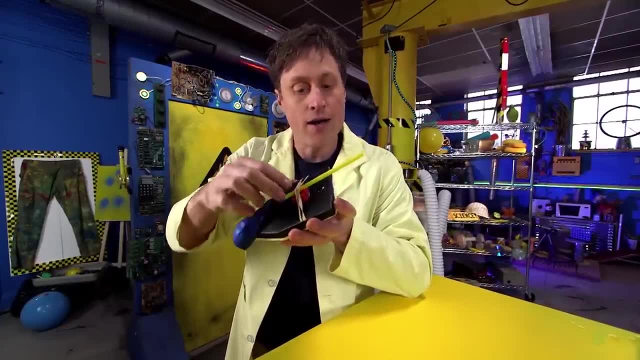 using more elastic bands, just like this: I put a nice tape top on the boat to make it look awesome And I also put a little bit of a riser here using just anything plastic to keep the straw nice and straight. because the question is: 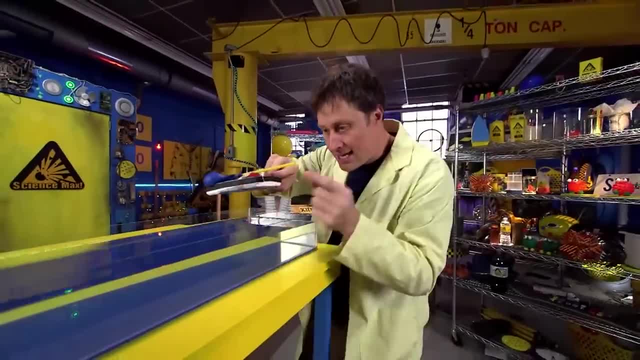 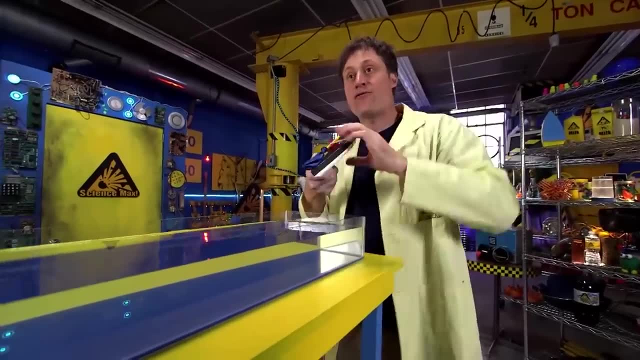 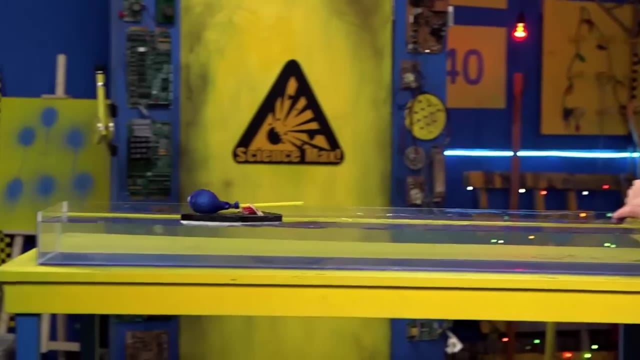 will our balloon-powered boat work better if it's pushing in the air or if it's pushing in the water? Well, let's do a science experiment and find out. First version in the air: Oh, almost all the way. Now let's try it with the straw, like this: 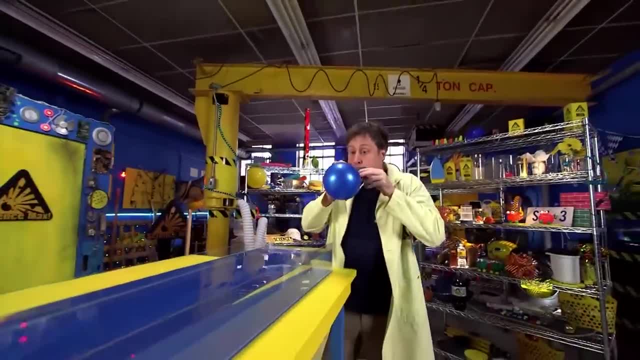 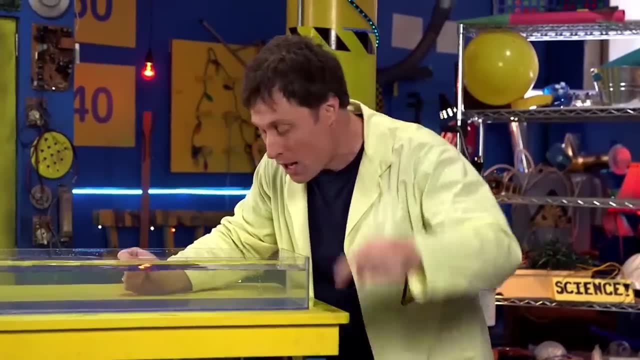 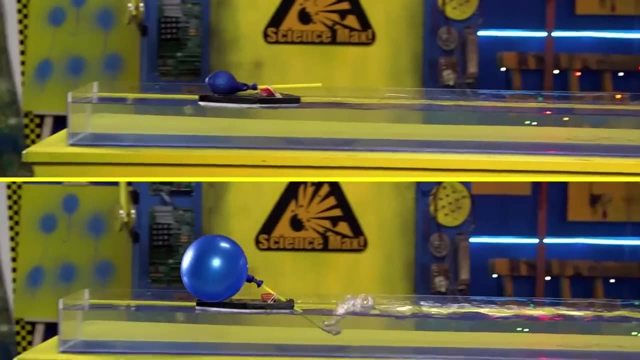 so it pushes into the water. Whoa It works so much better. Why? Because water is denser than air. The air coming out of the straw has to push against something to make the boat move. Water has more mass than air. 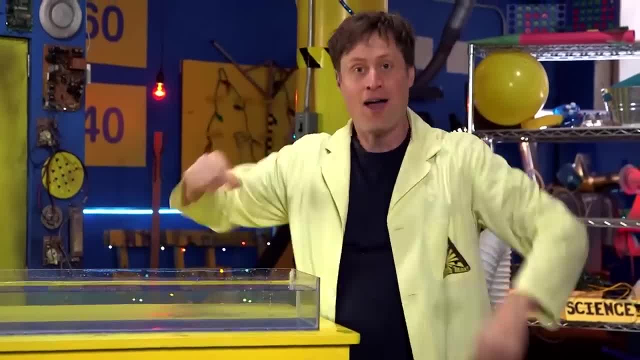 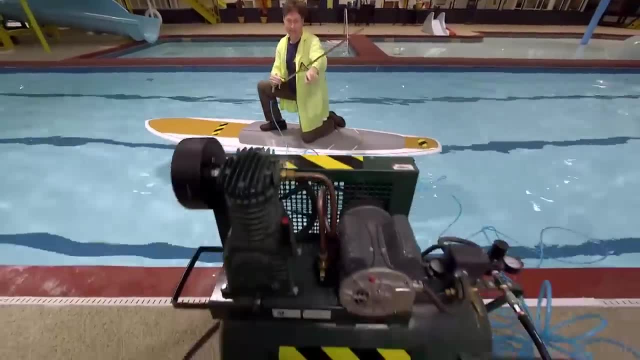 so pushing against water has a better result. Now let's max it out. This is an air compressor. Well, actually that is the air compressor. You see, the engine here pushes air into this tank, which works sort of like the balloon. 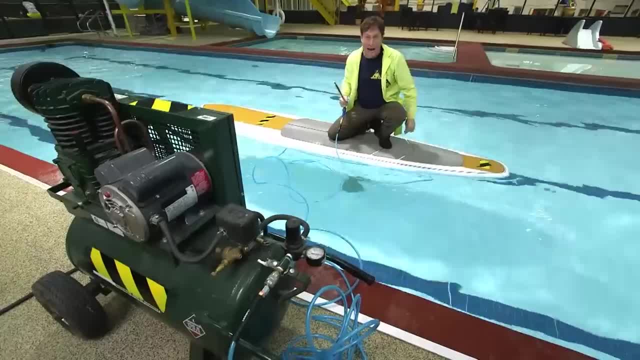 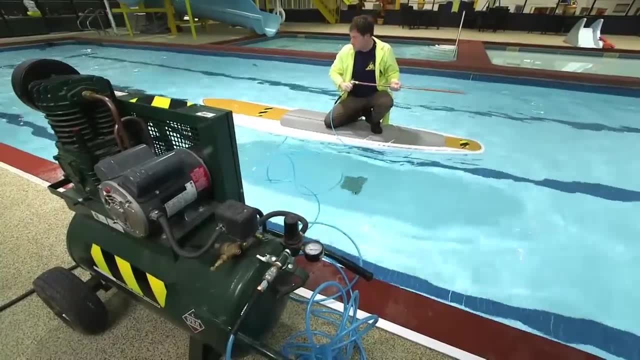 And then it goes out, this long hose which sort of works like a straw. So let's make a maxed-out air-powered boat Ready, Just like the small boat pushing against the air doesn't produce much thrust. Huh, Not so great. 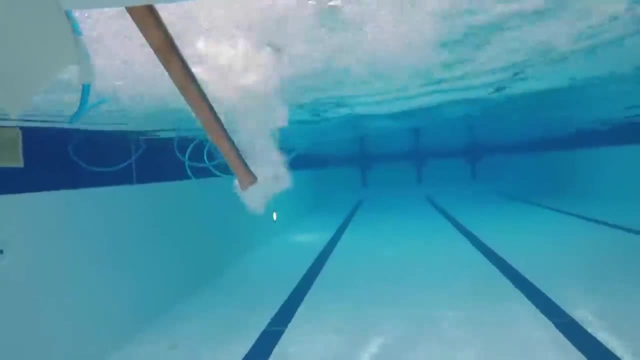 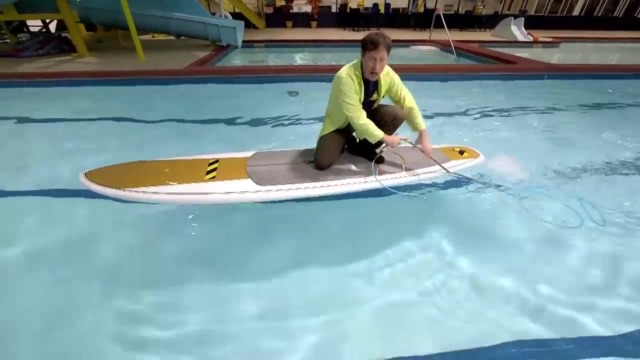 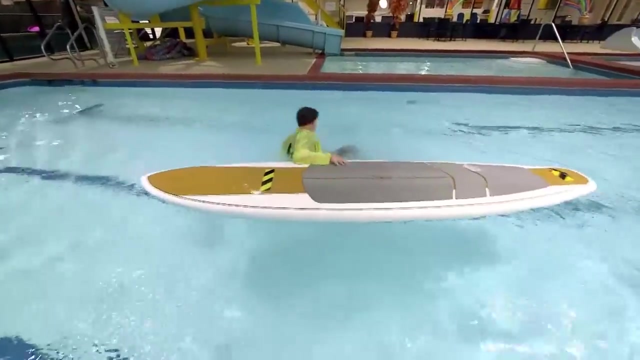 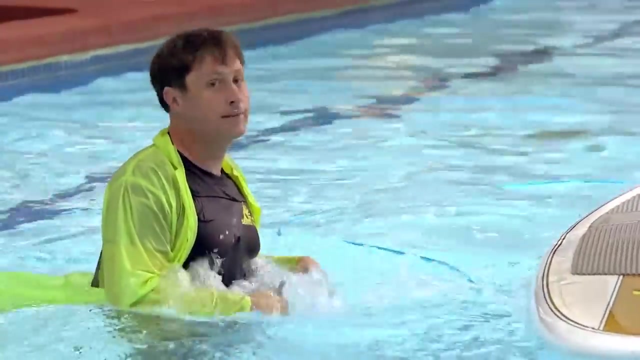 But now let's put it in the water. Pushing against the water gives me much more thrust, because water is more dense than air. Maxed-out air-powered boat. Maxed-out air-powered boat. Yeah, That's not me. This is hydrophobic coating. 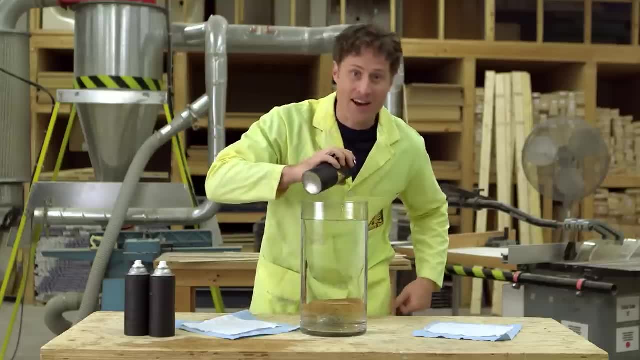 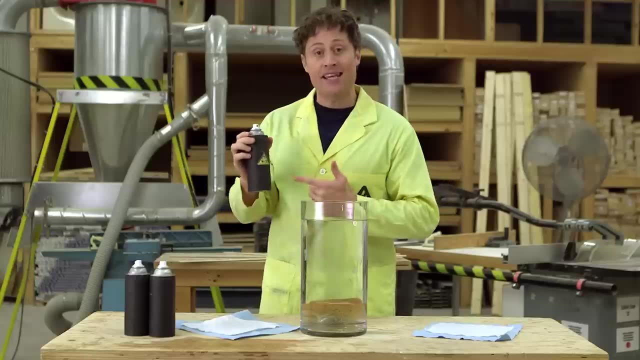 Hydrophobic literally means afraid of water, But it's not actually afraid of water. The chemistry of a hydrophobic coating prevents water molecules from penetrating anything you spray it on. You can get this stuff at the hardware store and, if you want, be science maximites. 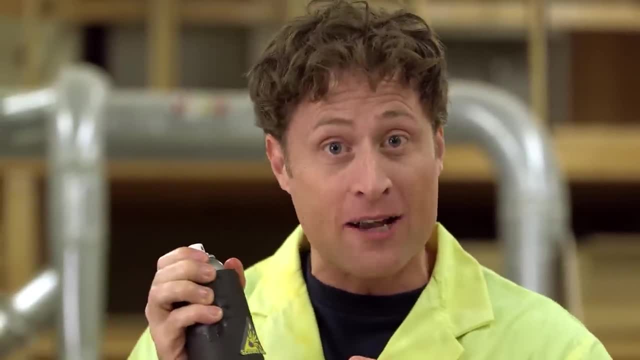 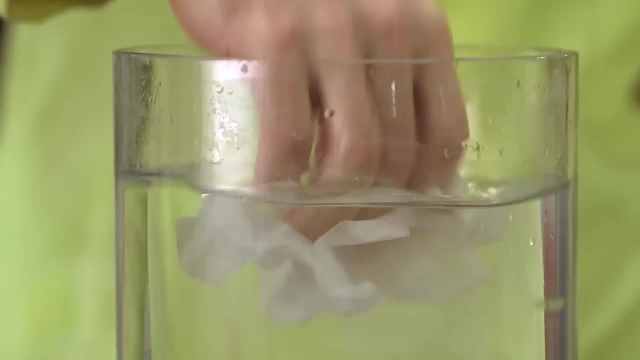 and get an adult and think of the coolest thing you could spray with hydrophobic coating. I like to use things that do not go well when you put them in water, like uh tissue, Yeah, doesn't look great when it gets wet. 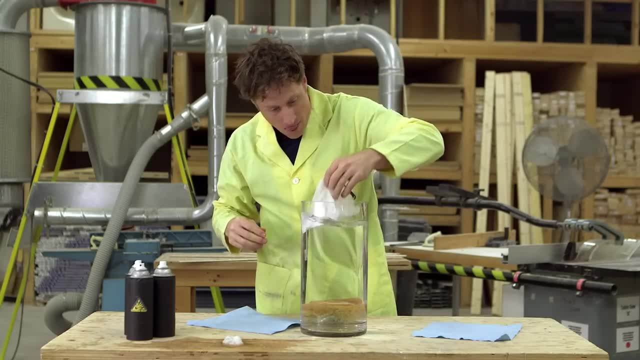 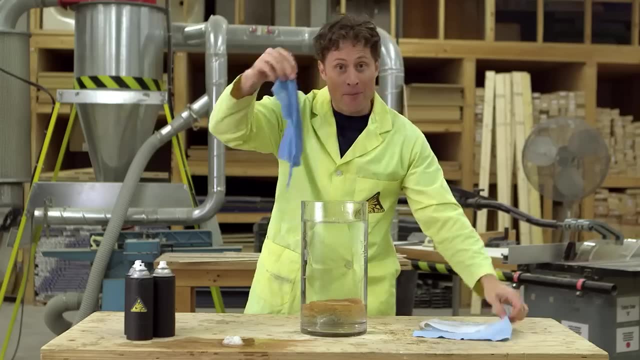 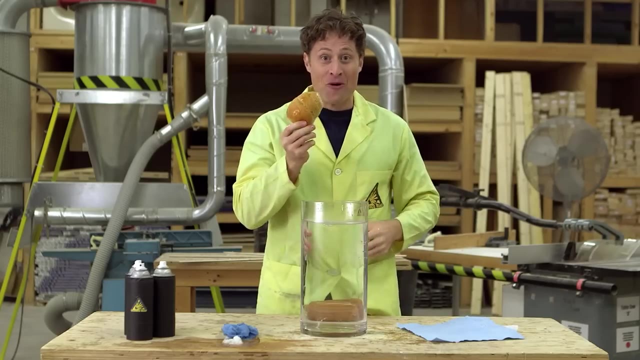 Here's a tissue coated in hydrophobic coating. Huh, Weird. Or it works the same with a paper towel. Paper towel in water. Paper towel covered in hydrophobic coating stays dry. Or how about a dinner roll? Dinner rolls really don't like water. 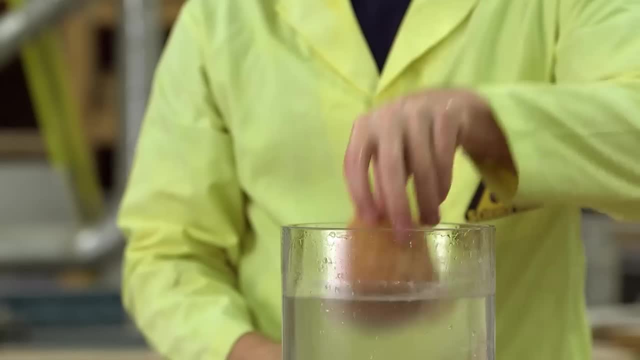 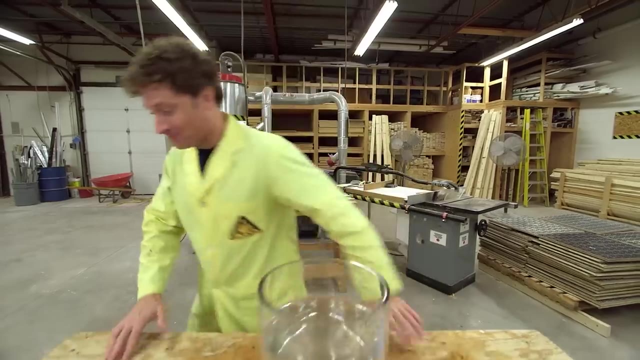 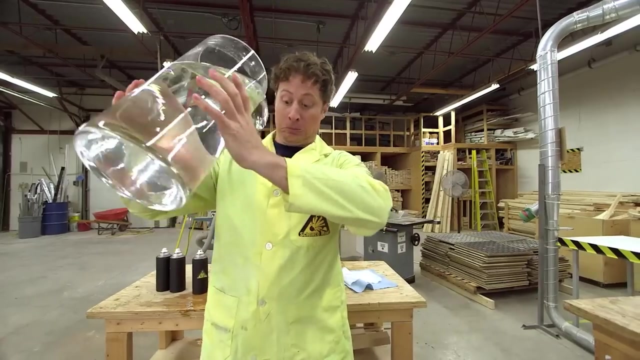 See Gross. But a dinner roll coated in hydrophobic coating- Weird. Just don't eat it. Now it's time to max it out. I have coated half of my lab coat in hydrophobic coating and the other half I have not. 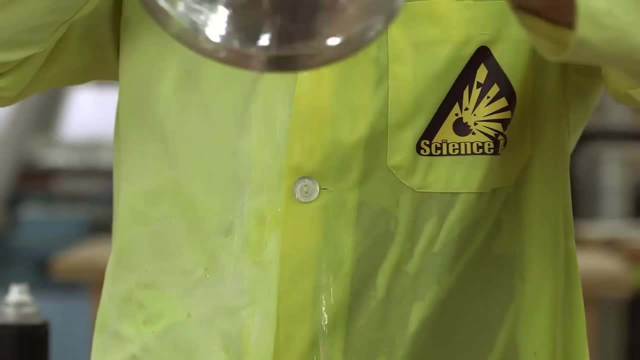 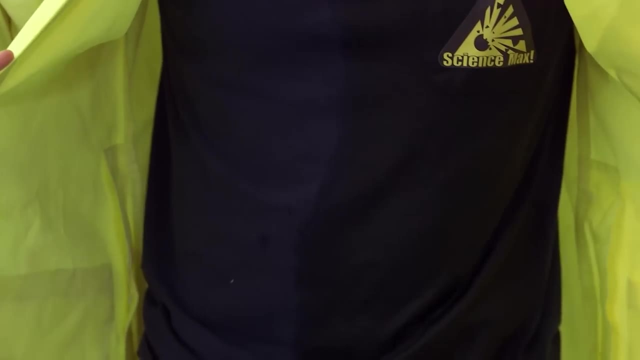 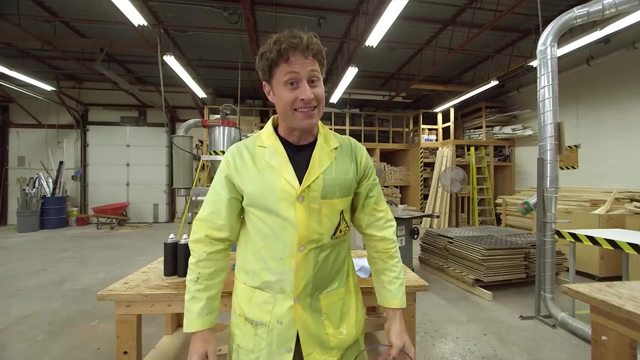 Hydrophobic coating- regular lab coat. Half of me is wet and half of me is dry. What's more, half of my outfit ended up being wet and half dry because the lab coat was protecting my outfit from getting wet. Now it's time to max it out even more. 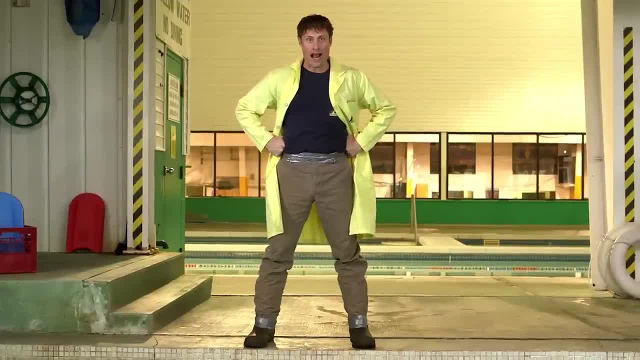 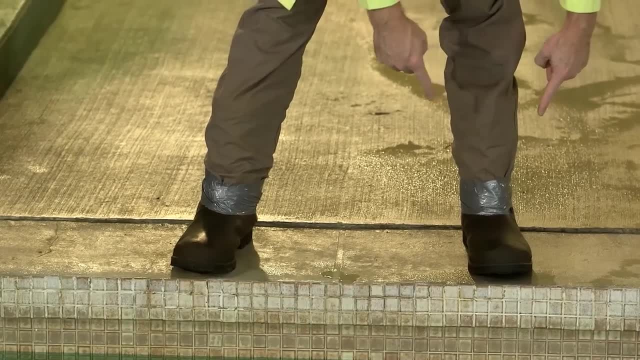 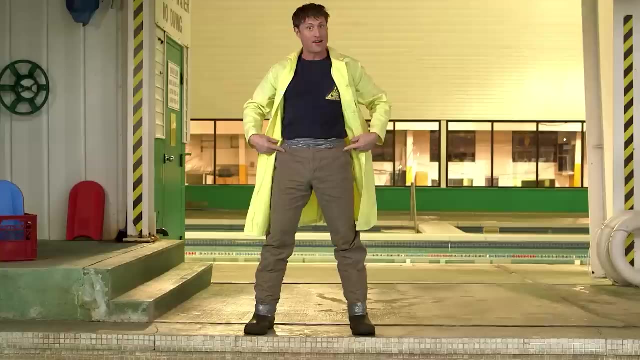 We have coated my entire outfit in hydrophobic spray: My shirt, my pants and my lab coat. The pants have been taped to rubber boots, so no water's getting in there, And my shirt has been taped to my pants, so no water's getting in there. 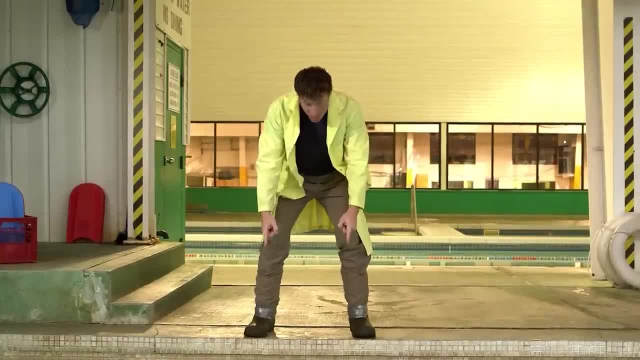 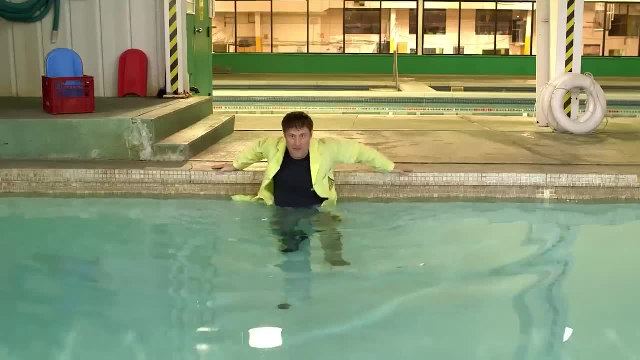 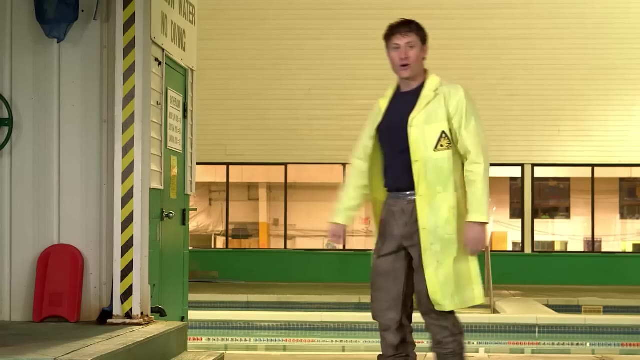 So here's the question: Can I get into the pool and out of the pool and stay dry? Let's find out In the pool, out of the pool, and I'm still mostly dry. Now here's what really happened. I got into the pool and I realized 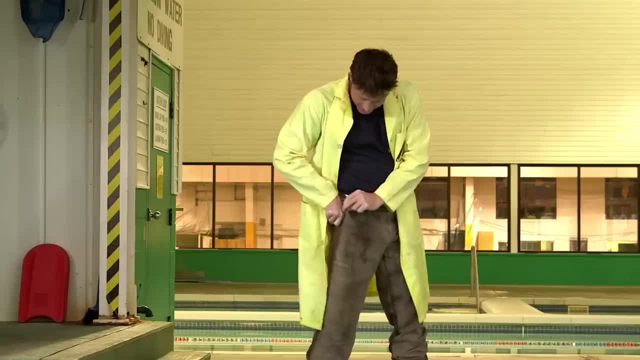 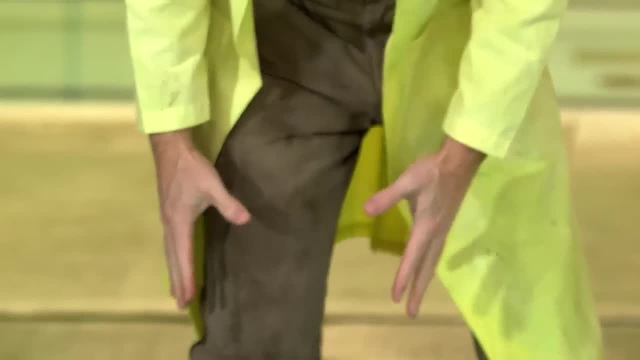 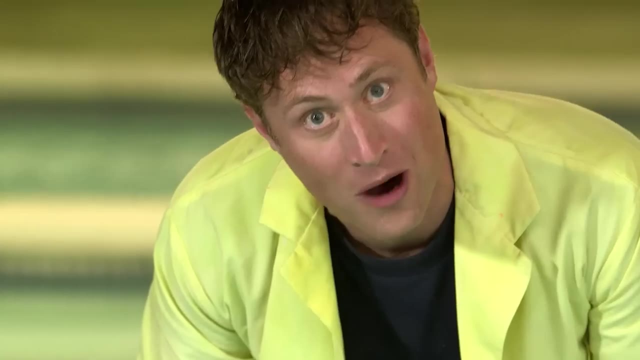 I should have duct taped the pocket, because all the water went in there, down into the rubber boots, started filling up the rubber boots and now my entire leg is full of water because the hydrophobic coating isn't letting it come out. So the hydrophobic coating isn't keeping the water out. 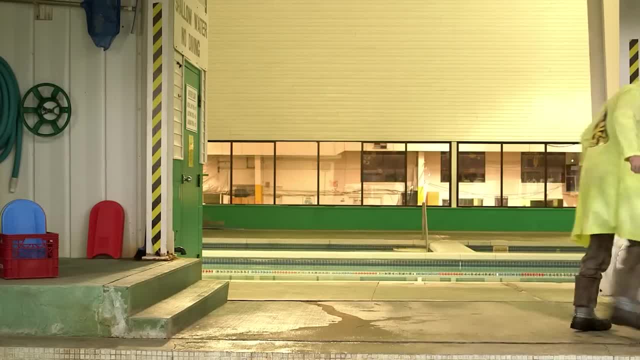 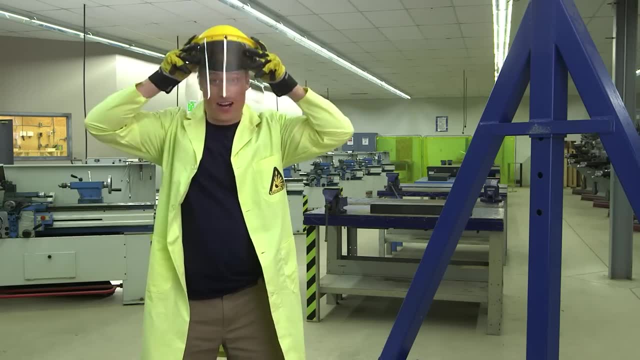 Now it's keeping the water in. Let's take a closer look at Newton's Third Law. Newton's Third Law: For every action, there is an equal and opposite reaction. Okay, All right, let's watch it back When the sign hits me. 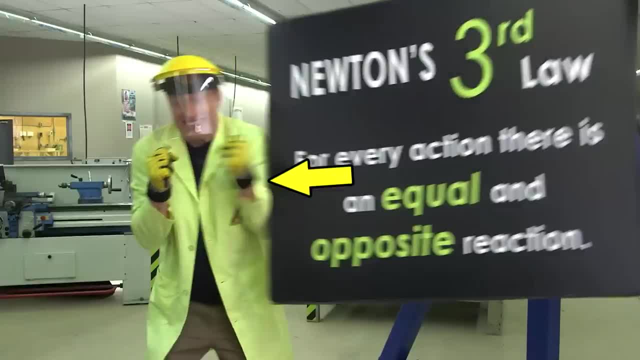 I exert a force on the sign in the opposite direction That makes the sign stop moving. It also exerts an equal force on me, causing me to fly off in two directions. That makes the sign stop moving. That makes the sign stop moving. 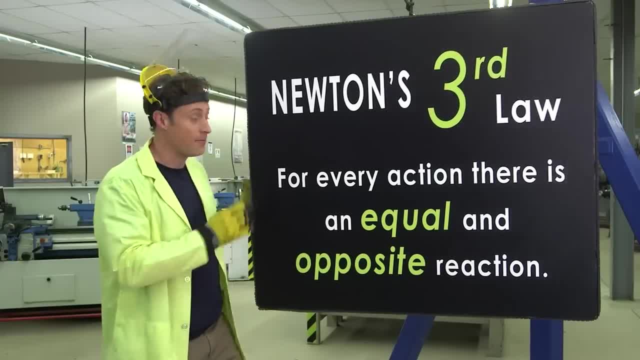 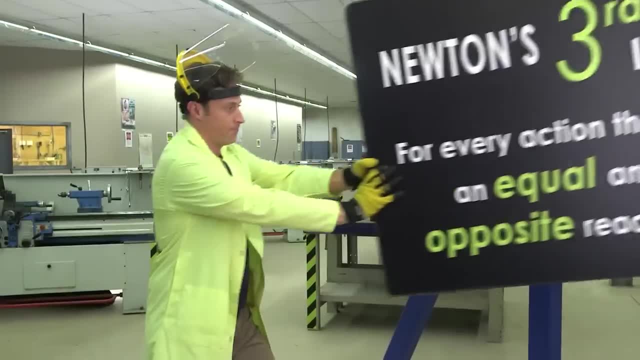 It also makes me to fly off in this direction. Now, if I was to push this sign? I'm not only pushing the sign this way, but my feet are pushing against the ground in the opposite direction. It's um Well, it's really easier to see. 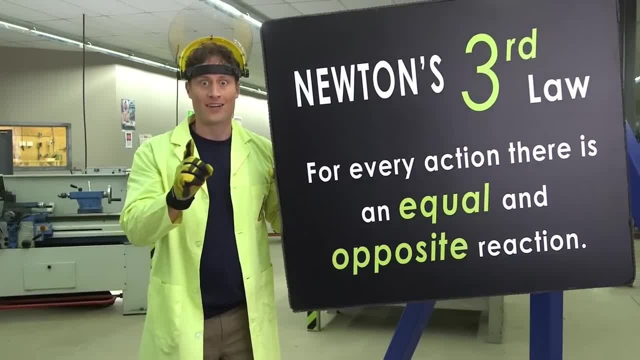 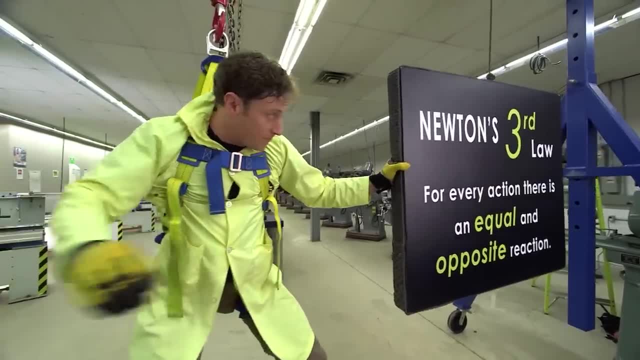 if I'm not standing on the ground. Um, Oh, hold on, Okay. so, Huh, Oh, okay. So now that I'm hanging watch, I push on the sign. but when I exert force on the sign to make it go this way, 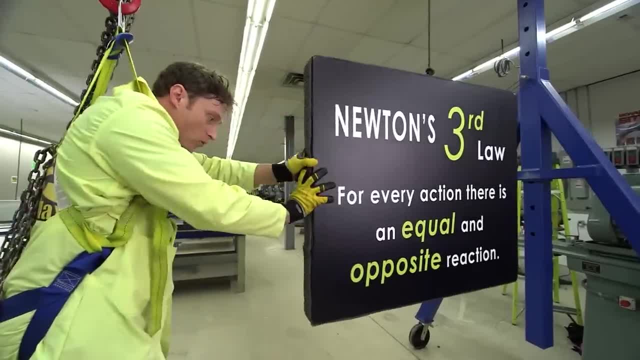 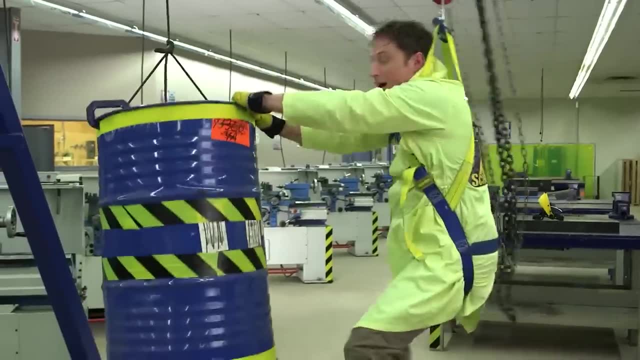 I go that way. Well, actually it doesn't work as well, because the sign isn't as heavy as I am. So wait, I have this over here. This is a barrel and it has stuff in it and it weighs as much as I do. 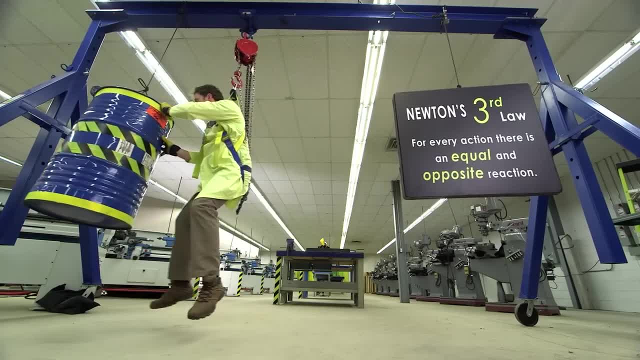 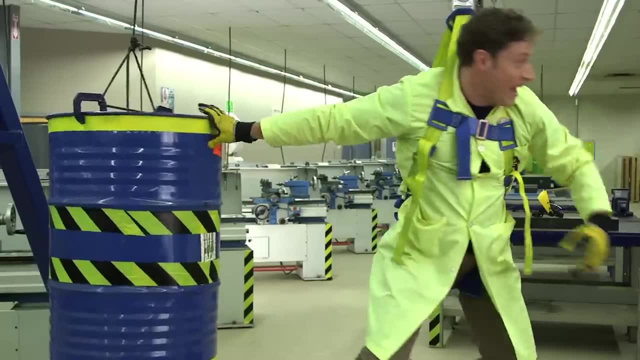 Okay, so watch, If I push on the barrel like that, I go away from it as much as it goes away from me. So there you have it, Newton's Newton's Third. No hold on Newton's Newton's Third Law. 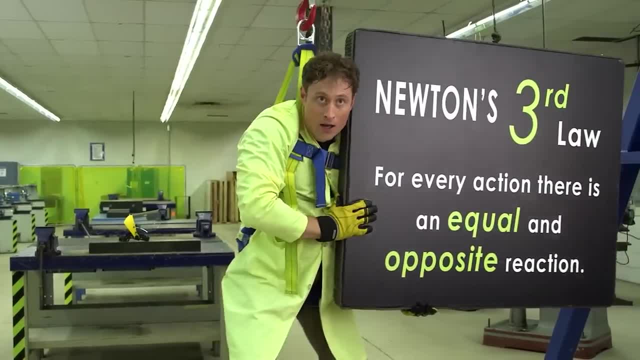 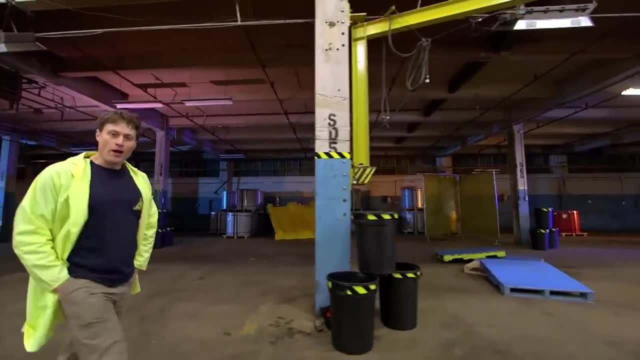 Newton's Third Law. Newton's Third Law, Okay go. Newton's Third Law: For every action, there is an equal and opposite reaction: Inertia. What is it? Well, it's directly related to Newton's First Law of Motion. 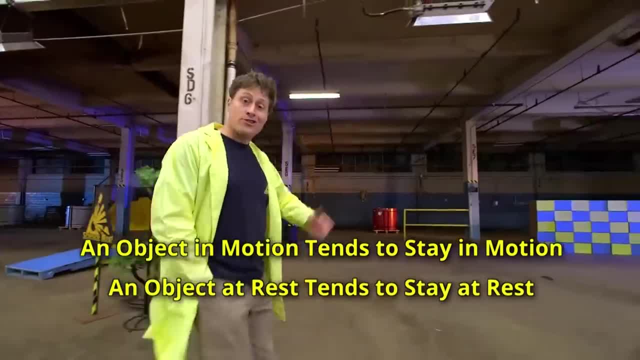 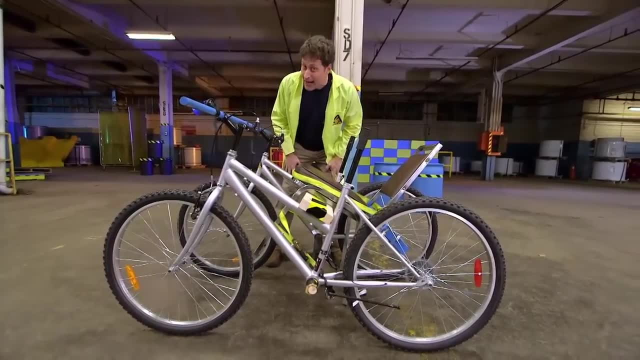 An object in motion tends to stay in motion. An object at rest tends to stay at rest. Let's do an experiment. Here is an object Right now. it's at rest. You might think that means it has no inertia, but that's not true. 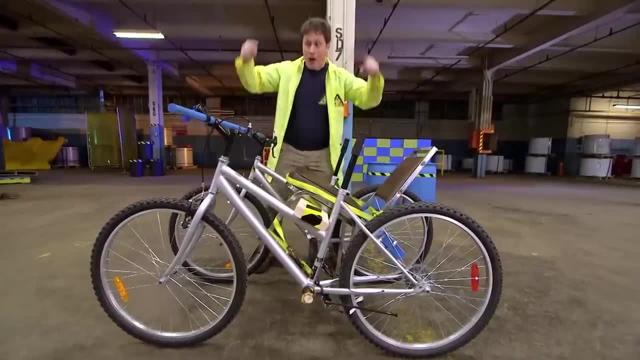 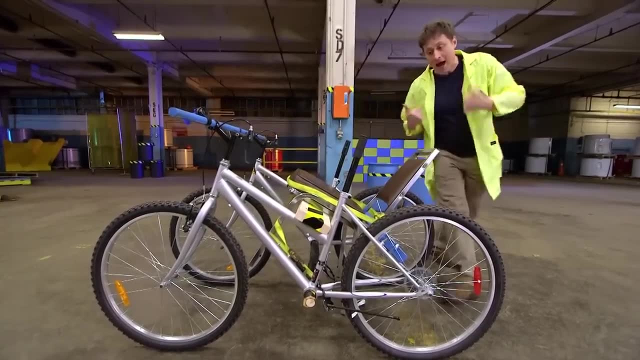 Inertia just means an object's tendency to keep doing what it is doing. Right now it's doing nothing, But if I wanted to overcome its inertia, I would have to put energy in, And now that I have, it is moving on its own. 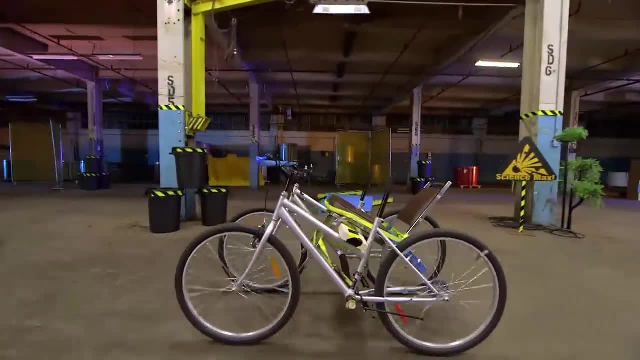 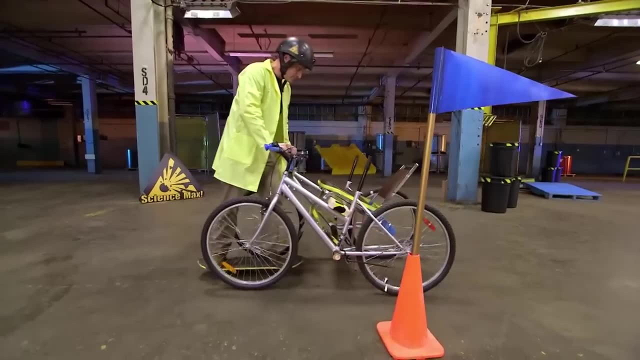 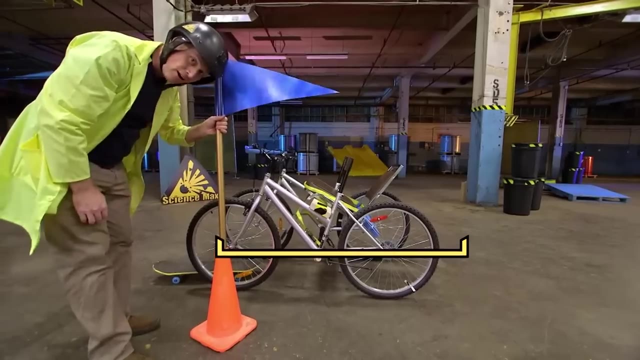 It has inertia. If I wanted to stop it, I would have to overcome its inertia, its tendency to keep moving There, I went exactly that far. Now let's max it out. I'm adding these weights to the cart. 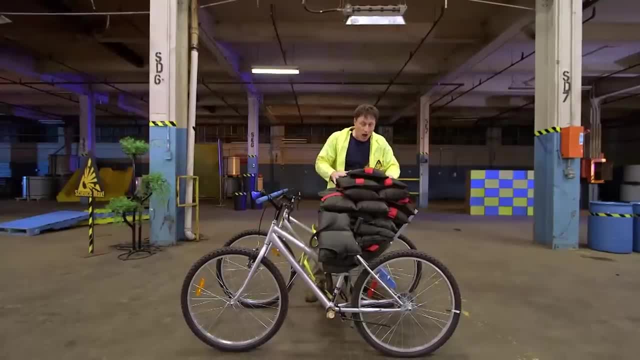 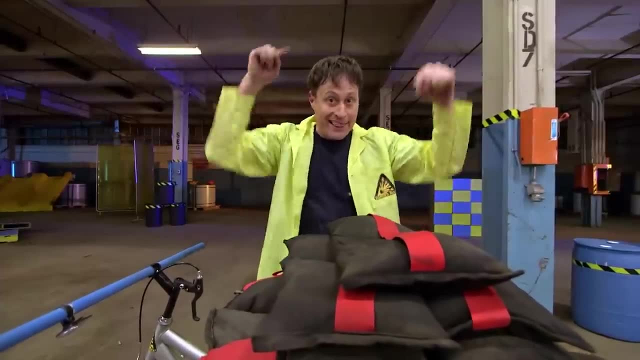 Now it has a lot more mass, which means it has a lot more inertia and its tendency to do nothing. But this time it has a lot more inertia. If I wanted to get it going the same speed as before, I'd have to put in a lot more effort. 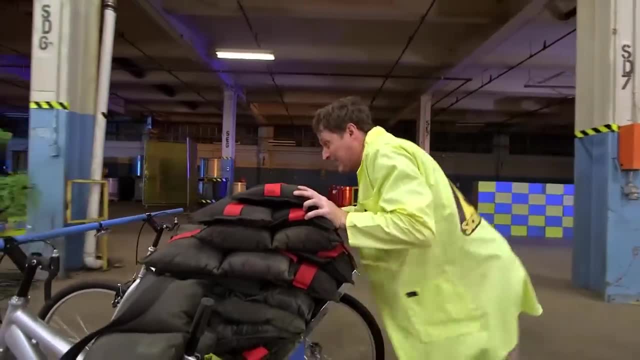 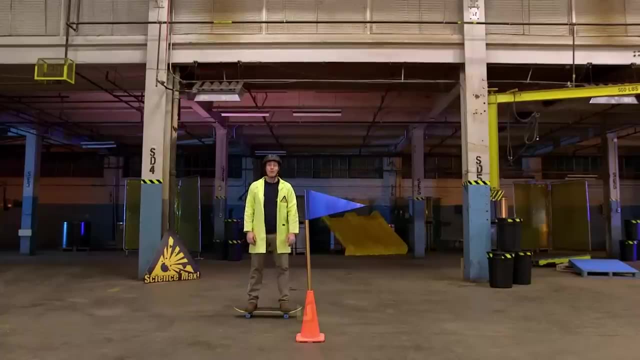 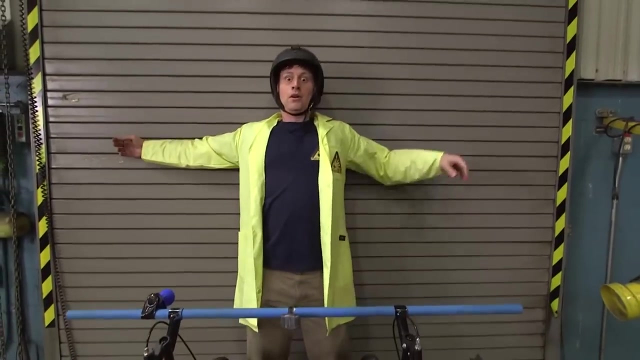 There. Now it's going the same speed as before, but now it has way more inertia, So stop it. and it's going the same speed as before. There It has inertia, so stopping it will be harder. So there you go. 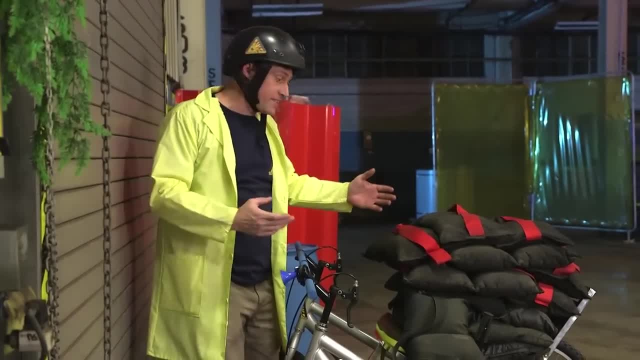 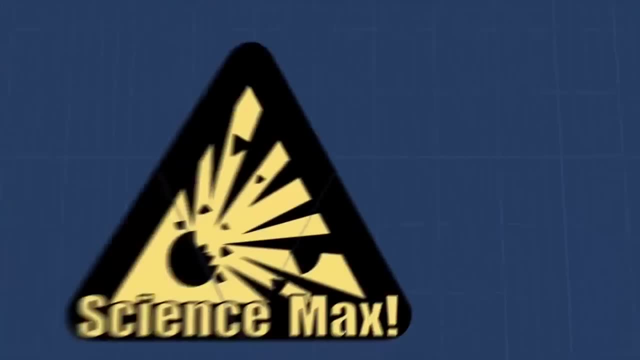 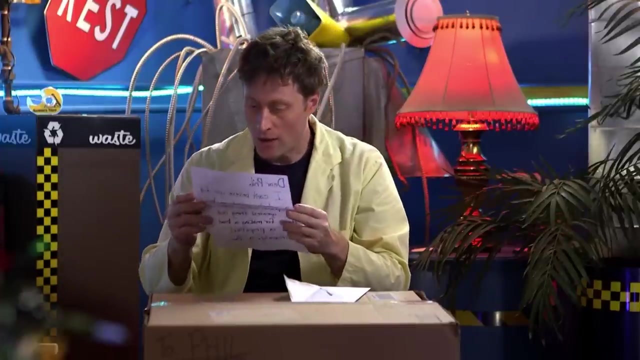 Inertia, A thing's tendency to stay moving or stay still, and the more mass, the more inertia. Dear Phil, I can't believe you did a whole episode on boat propulsion and you didn't use the greatest thing out there for making a boat move. 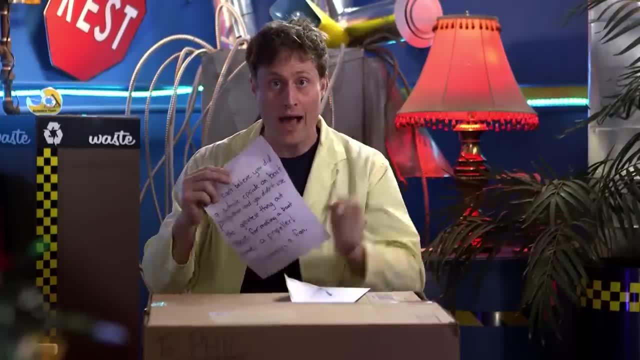 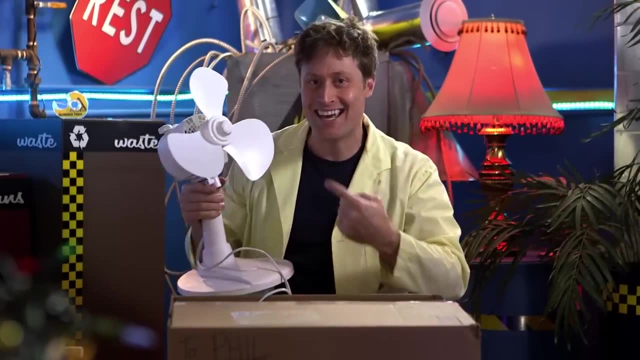 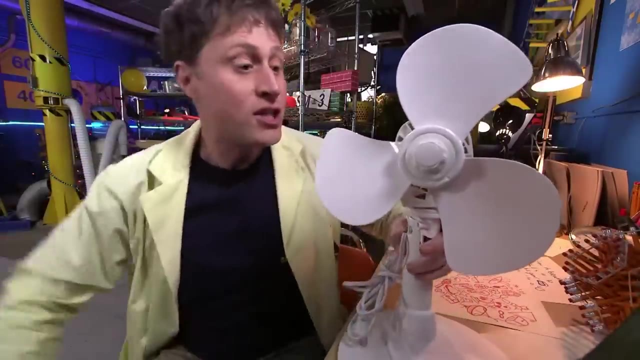 a propeller. Sincerely a fan. Well, let's talk about propellers. Oh, Good thing, this is fan mail. Get it, Because it's a fan. Anyway, A fan pushes air, just like a boat propeller pushes water. 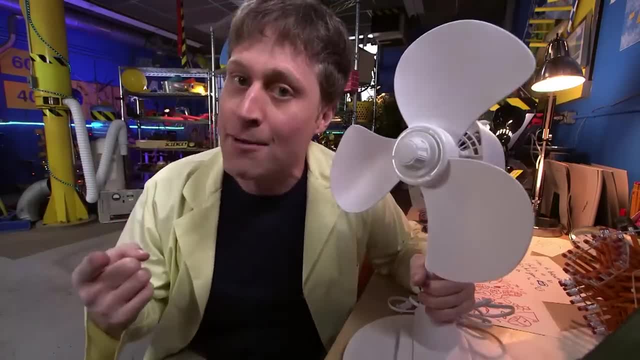 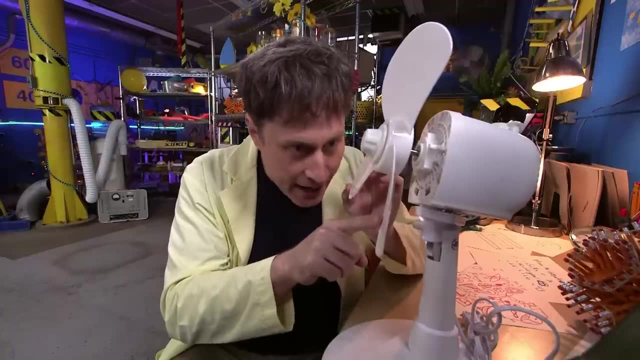 They're both fluids and they behave in the same way. Now, if you look closely at a fan, it's curved on the blades, The air or water is caught under at this side, and then it's pushed out on the curve to make it go that way. 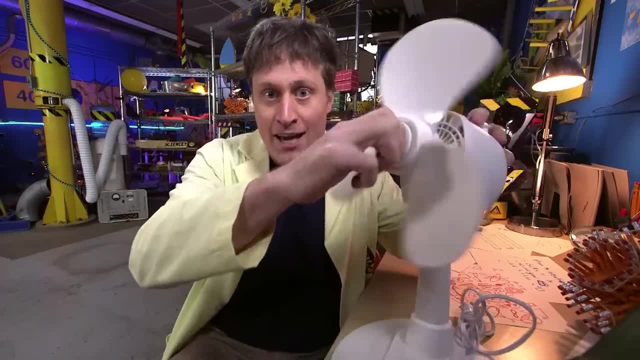 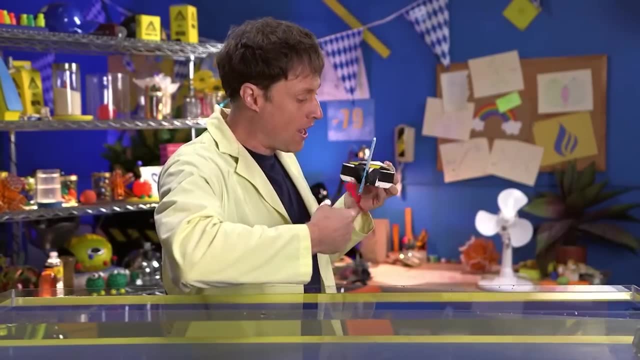 and the faster it spins, the better it works. Now this is a propeller-powered boat, and what you do is wind up the propeller- I have an elastic band here to store the amount of energy I put in- and then you put it in the water. 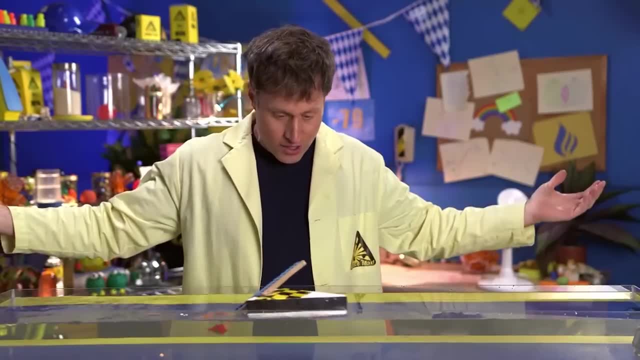 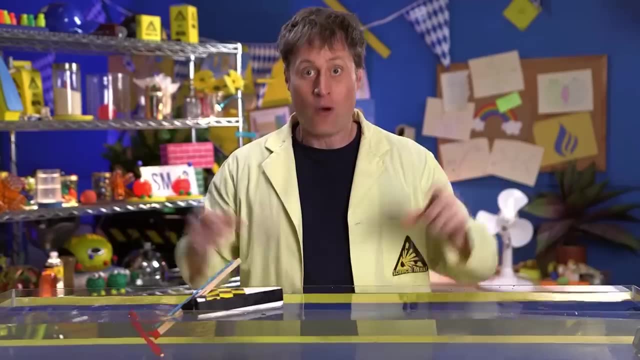 The propeller spins and the boat goes. The boat goes forwards. It's being propelled by the propeller. That's why you call it that Awesome, right? Well, now we'll max it out. This is a drill. It spins. 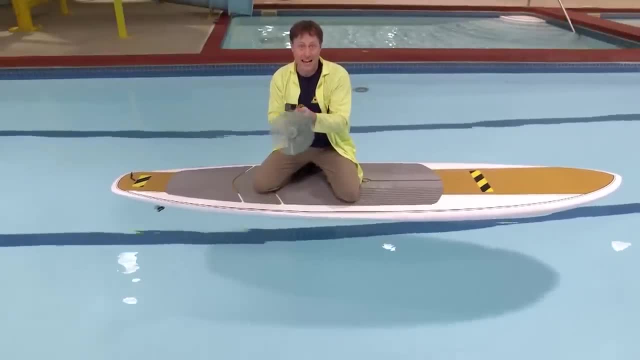 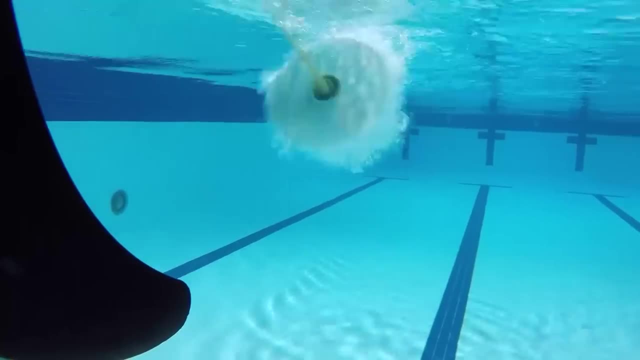 And this is a propeller, and when you put it in the water and spin it, it provides thrust. So let's try it out. Whoa, Remember not to try this at home. I am a trained professional. This is a very small propeller. 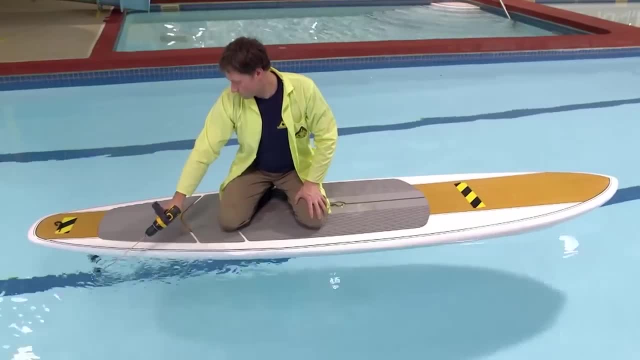 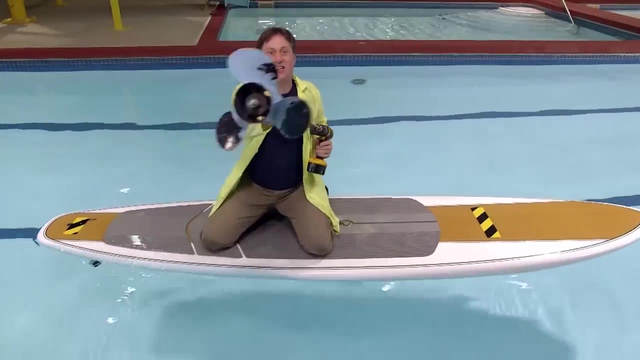 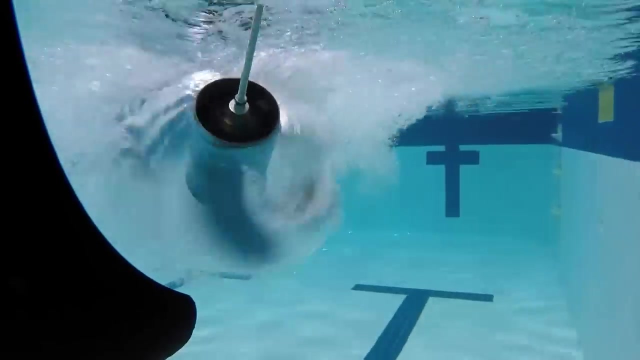 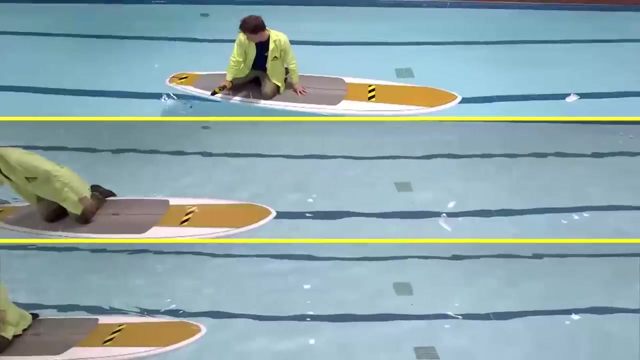 Let's compare This. This is a super-maxed-out propeller. Whoa, Okay, let's try it out. Whoa, Whoa. The larger a propeller is, the more energy you need to turn it and the more propulsion. 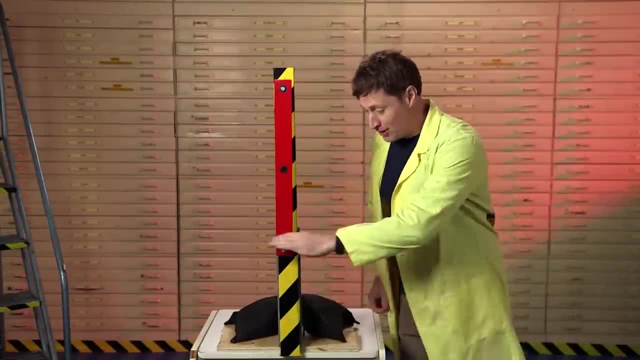 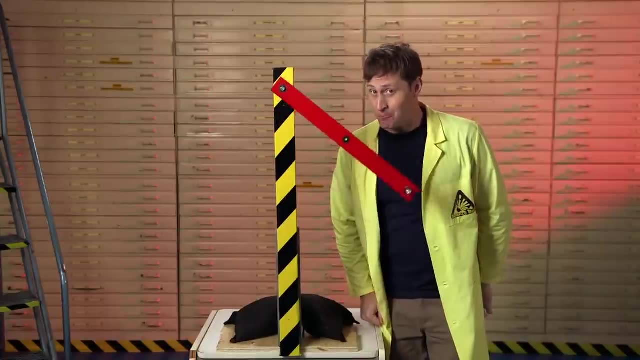 you get out. This is a pendulum. It's a weight that swings. It swings back and forth. Pendulums are pretty simple. It It swings back and forth. Predicting the path of a pendulum: Pretty simple: It's gonna swing back and forth. 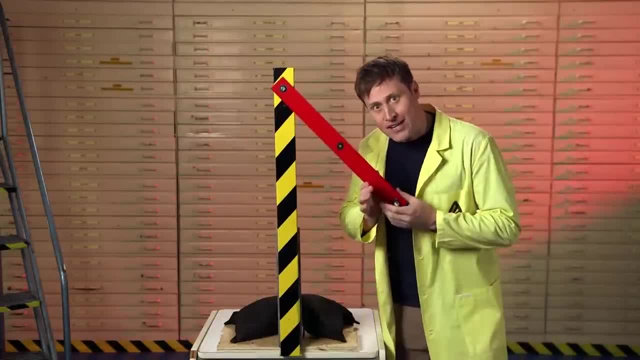 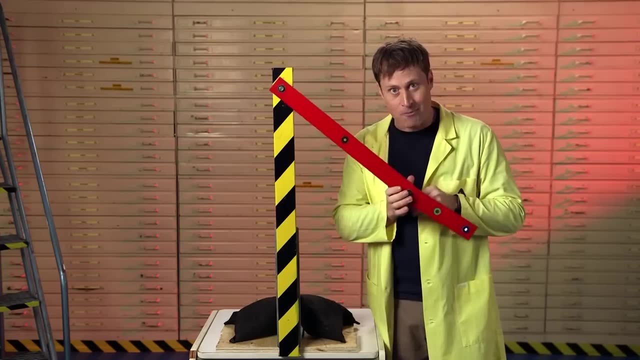 But wait, As I make it so much more complex by adding a pendulum. Now I've got a pendulum down here and that one swings back and forth, and I've got a pendulum up here that swings back and forth. 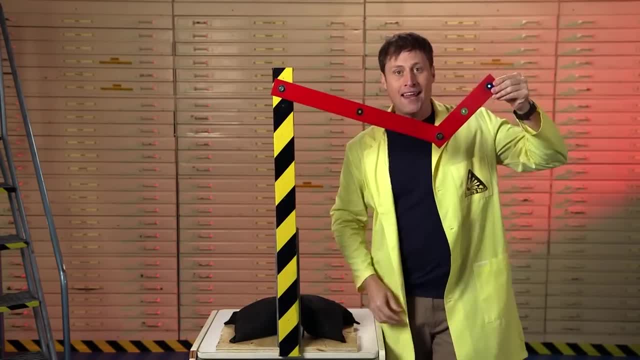 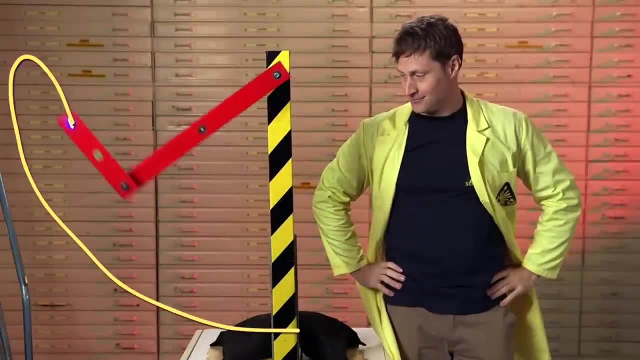 What will happen to this part of the pendulum when I let it go? Can you predict? Let's find out. This is a double pendulum and predicting the path of a double pendulum is really difficult. It's still simple physics. 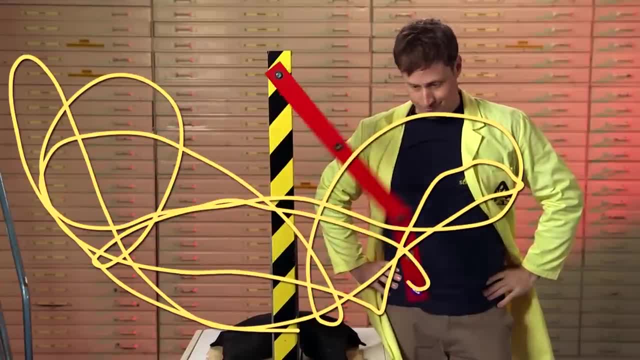 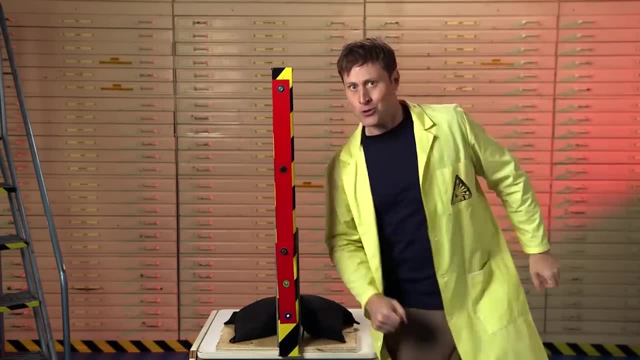 but because there's a moving part attached to a moving part, it makes it way more complex. So the question is: can we max it out even more? Of course you can. These are chaos pendulums. This one's a lever. 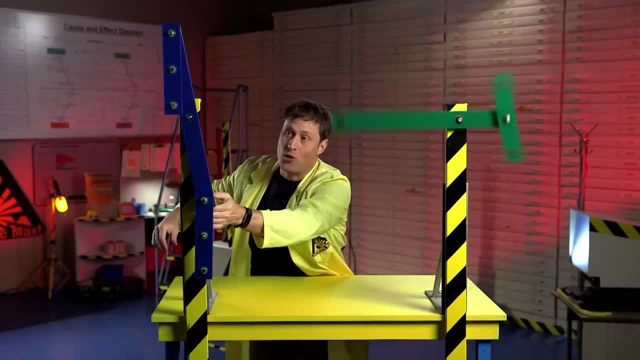 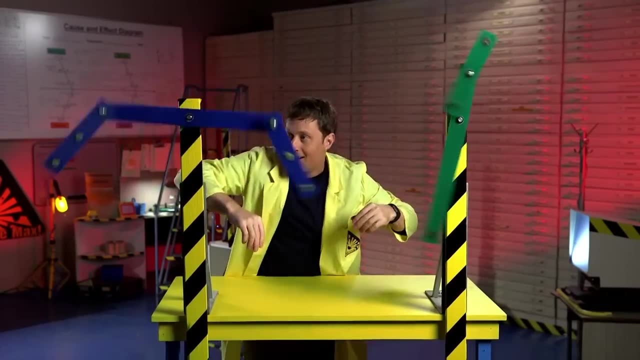 and it's got another lever on the end- Whoa. And this one here is a perfectly balanced lever and it's got a pendulum on either side- Whoa, Whoa. Scientists and engineers have always said that the more moving parts something has. 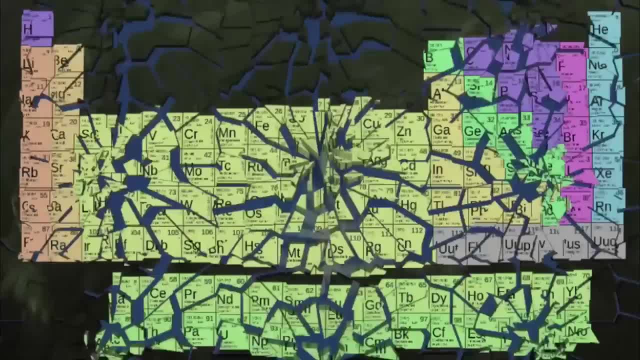 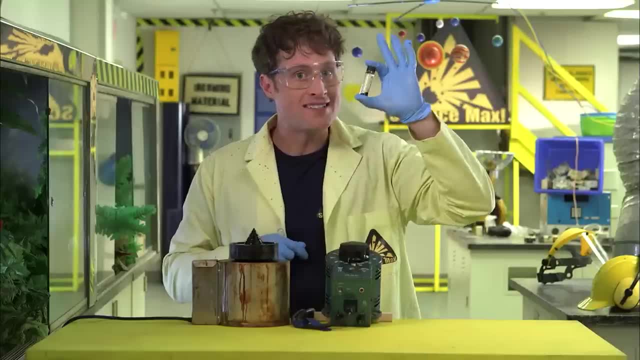 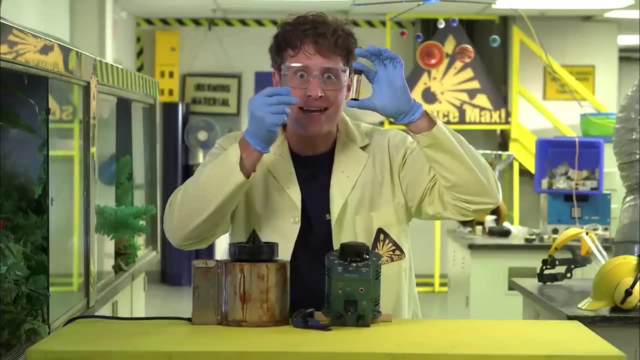 the more complex they are. Science: This is ferrofluid. It is ferromagnetic, which means it's attracted to magnets. And I know what you're thinking. You're thinking it's not that interesting. Well, watch as I put it: next to this magnet. 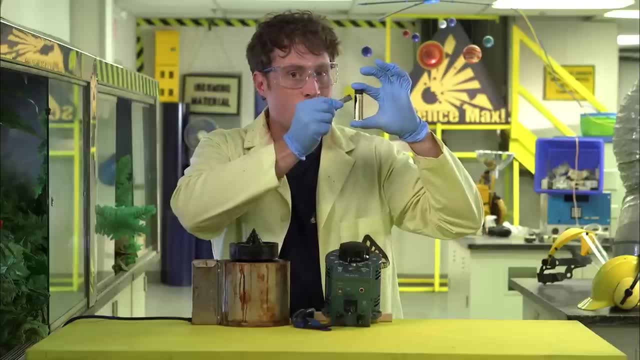 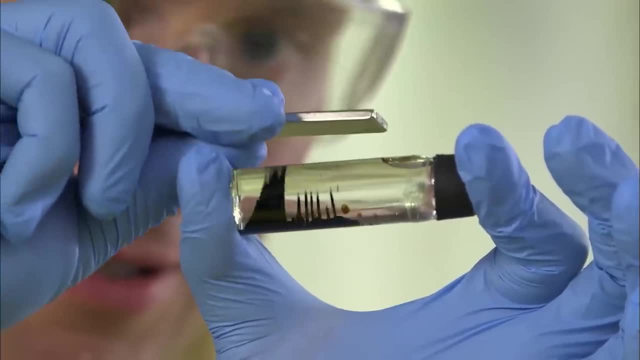 Very interesting And because it's a liquid, it behaves in very interesting ways. Watch this: Unlike most things ferromagnetic like paper clips or iron filings, ferrofluid is a liquid, which means it behaves in a unique way: The spikes it creates. 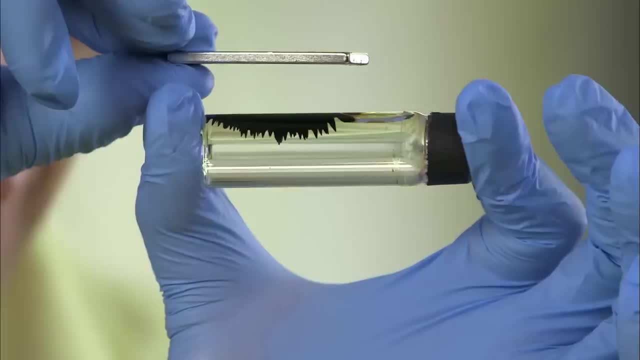 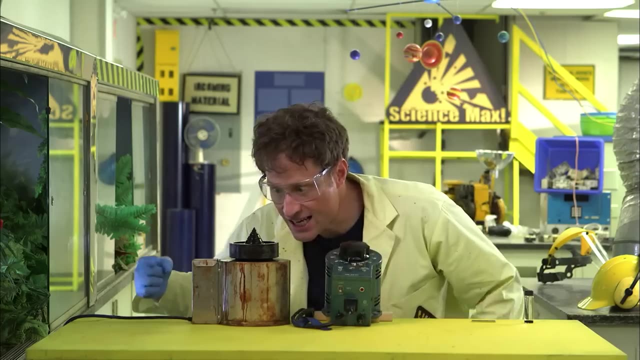 are following the magnetic field lines of the magnet. You can see the magnetic field in 3-D. It's even more impressive when we max it out. This is ferrofluid outside of a glass jar. Now it's sitting in a pool around this electromagnet. 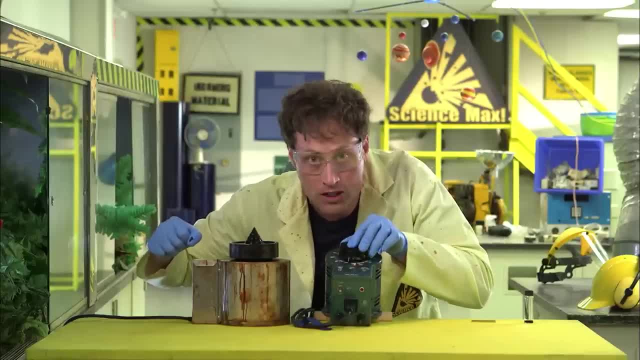 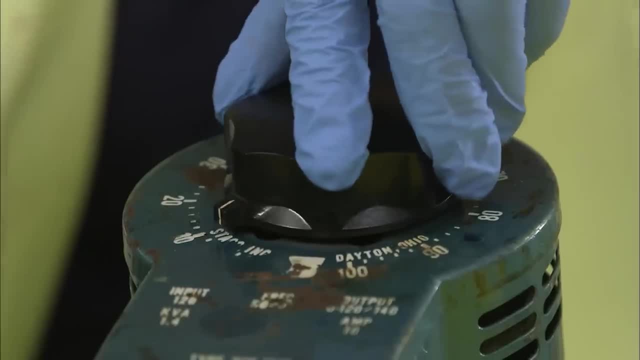 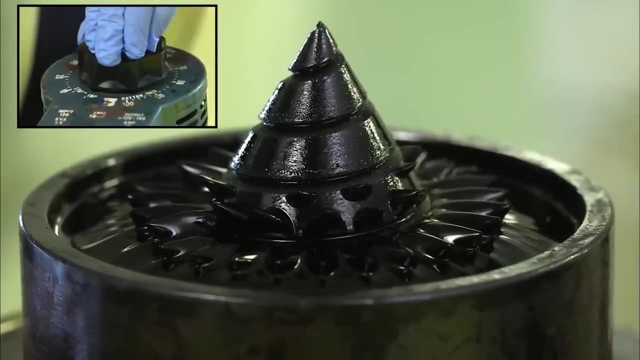 And this is a dial which I can use to change the voltage of the electromagnet, making the magnet stronger. Watch this: Changing the current going to the spiral in the middle turns it into a magnet. The more current I put in, the stronger that magnet becomes. 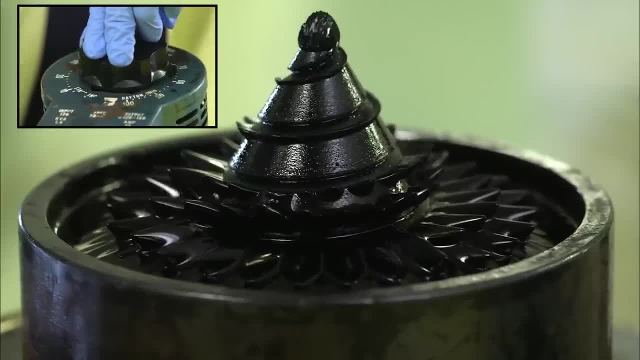 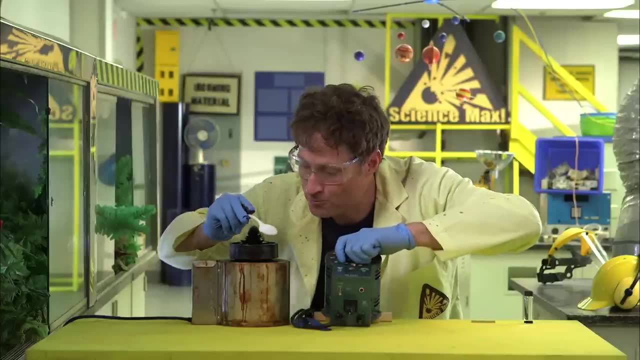 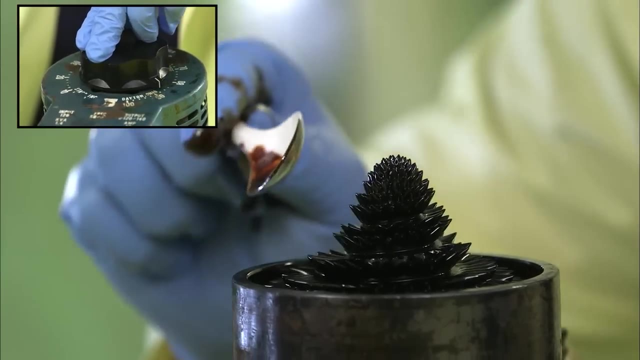 allowing the ferrofluid to climb the spiral to the top. And remember, even though it looks all spiky, it's still a liquid. I will demonstrate with my plastic spoon And watch this. When I turn the magnet off, it stops being spiky. 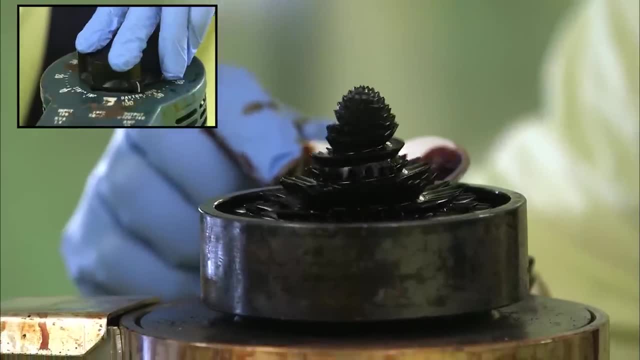 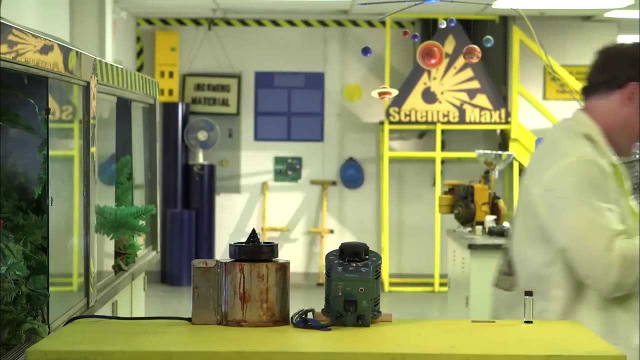 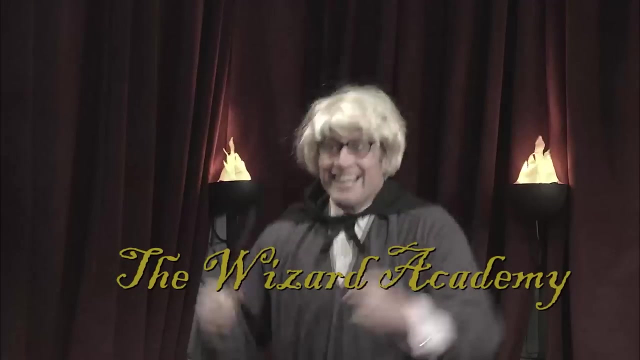 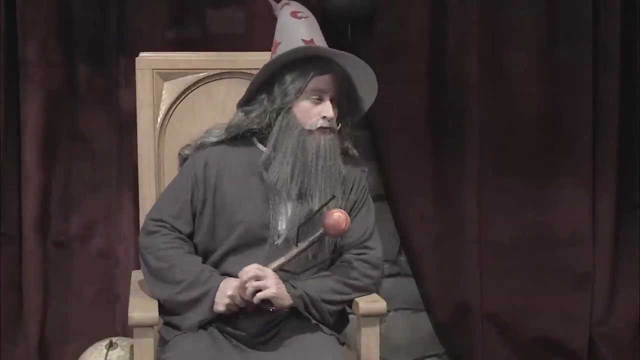 Turn it on, Turn it off. Science, The Wizard Academy. All you have to do is demonstrate true magic And you will be granted entry. Well, Fuzzix, who is the next applicant for the Wizard Academy, Overwhelmo. 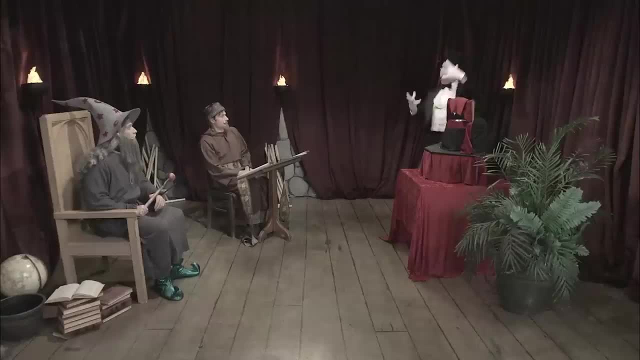 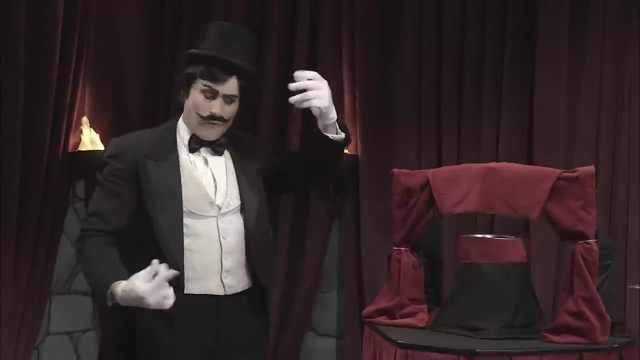 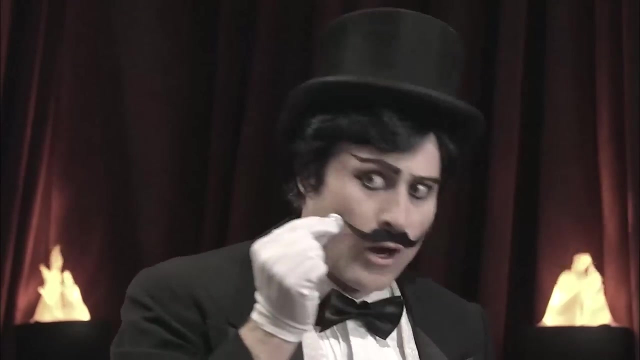 Indeed it is. I Overwhelmo And prepare to be overwhelmed. Would you be flabbergastified if I balanced this coin on its end? Not really no, But would you be impressed if I was to balance this coin on top of this coin? 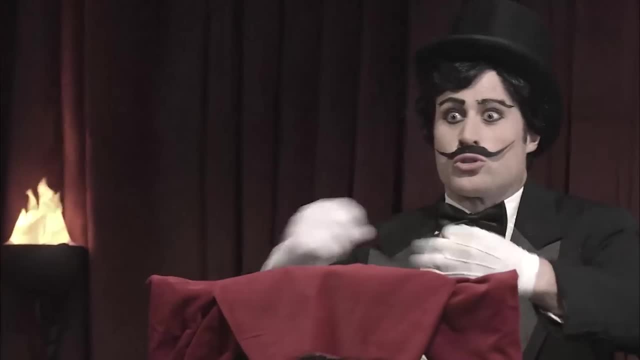 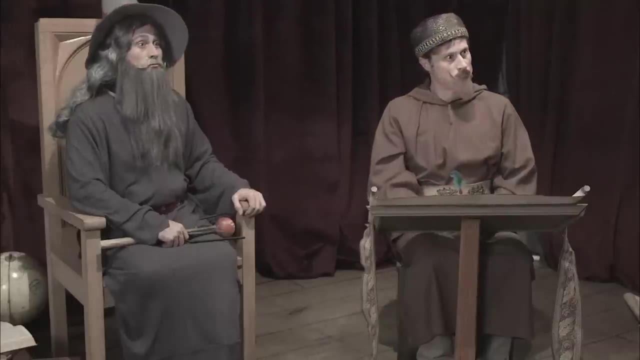 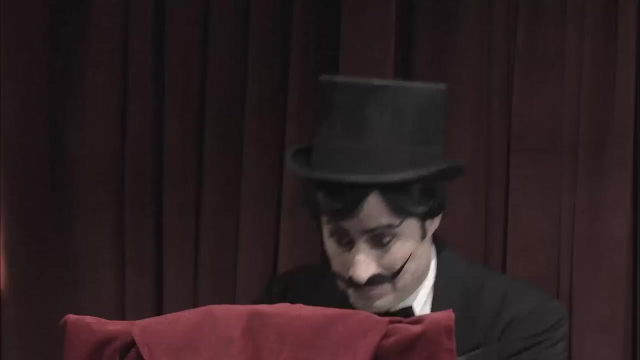 Possibly Prepare to be flustered and stoopified, Stoopy, Stoopy, flustered, As I balance three coins on their ends on top of this glass. Well, that certainly would seem like magic. Let us see, Okay. 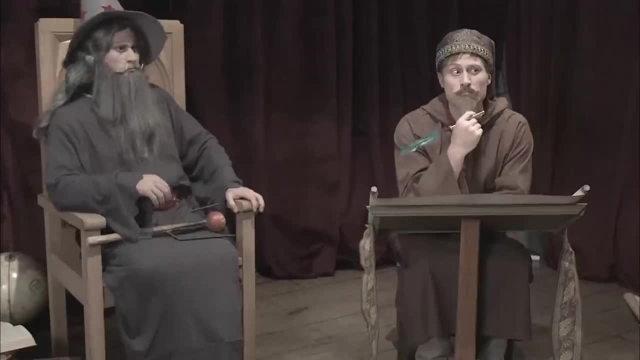 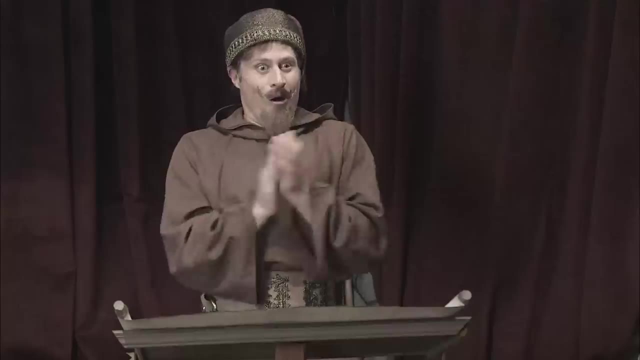 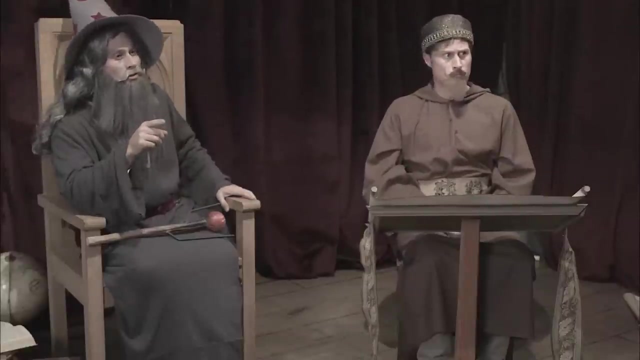 No pressure, Overwhelmo, You can do this. And now I say a magic word. A magic word, And now you must let me into your academy. Wait, What's under the cloth? What? what cloth? This cloth, Nothing. 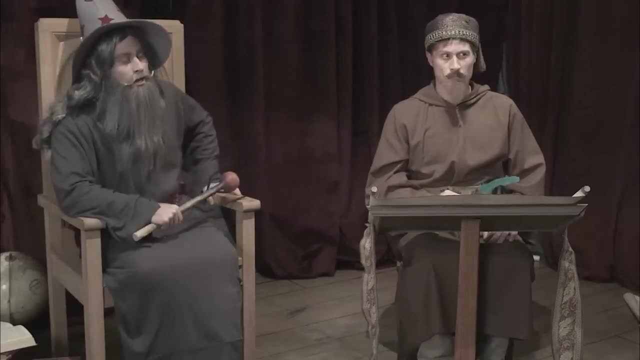 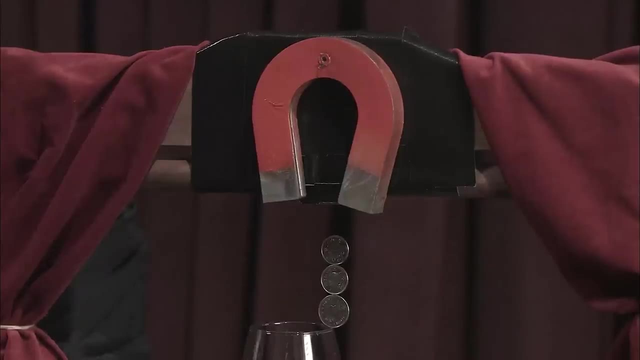 Oh, Is that a magnet? This? No, The pull of the magnet is what's keeping those coins up? The magnet is just strong enough to keep the coins from falling. No, This is set dressing, It's just for. It was a good trick. 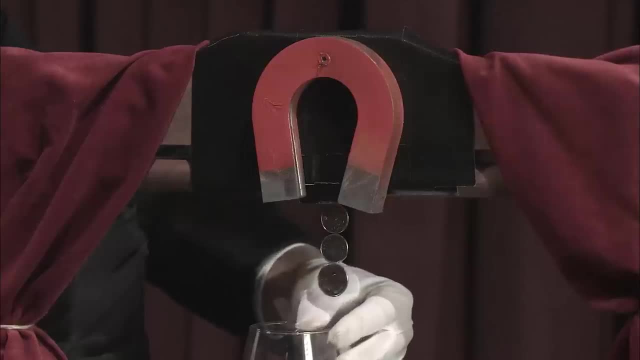 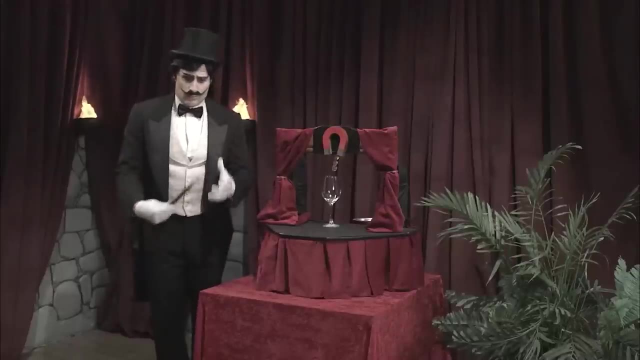 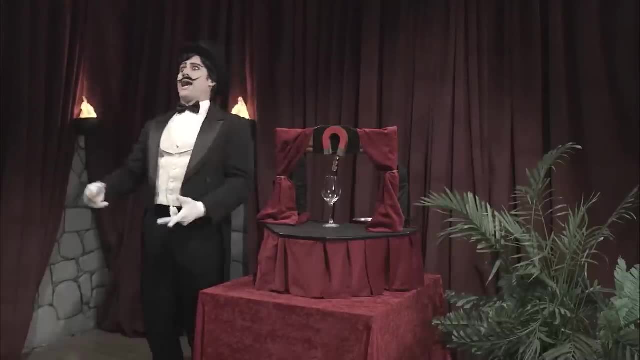 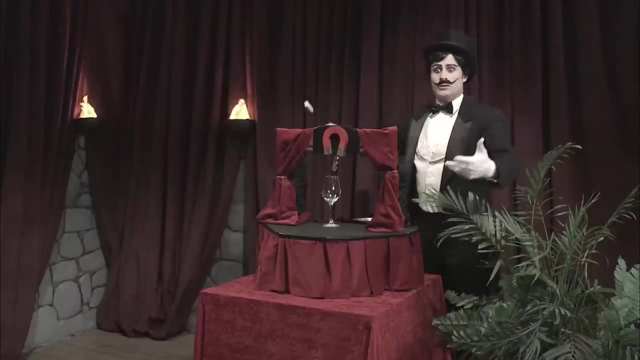 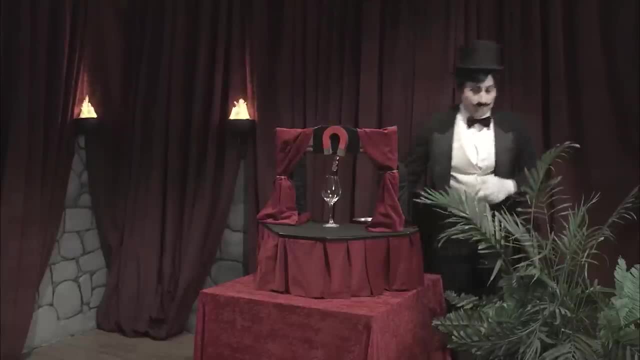 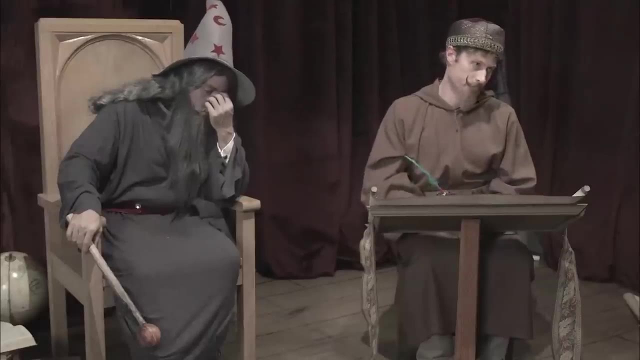 With my magic, you will need at least two pairs of socks, Maybe three Pairs of socks. We can still see you. No, you can't, Mm. A delicious plate of cheese and crackers- My favorite snack. But 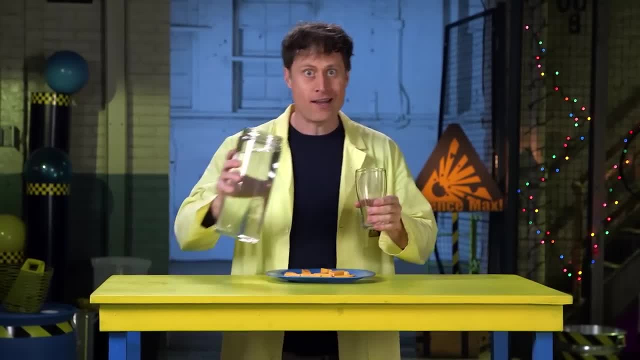 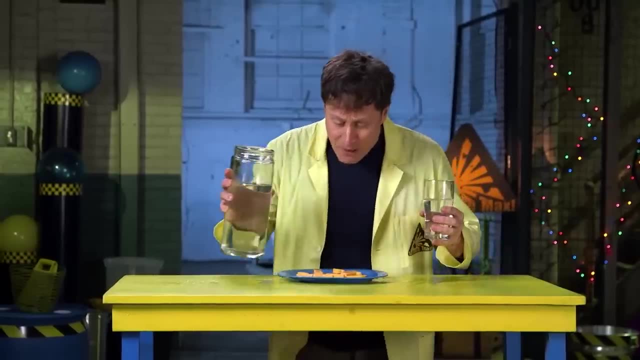 these crackers are pretty salty, So I should probably pour myself a glass of water first. huh, Trev, What? No, My cheese and crackers. Why? Why does this happen? Why does the water stick to the glass? Well, because of science. 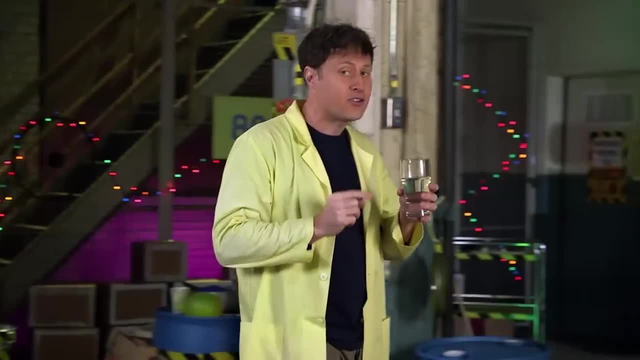 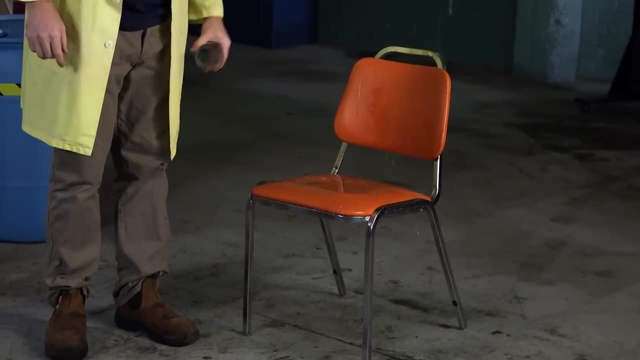 And the reason why it happens gets a little complicated, but it boils down to this one simple thing: Water likes to stick to things. Huh, Did you see? Did you see how it stuck? No, of course you didn't. You know why. 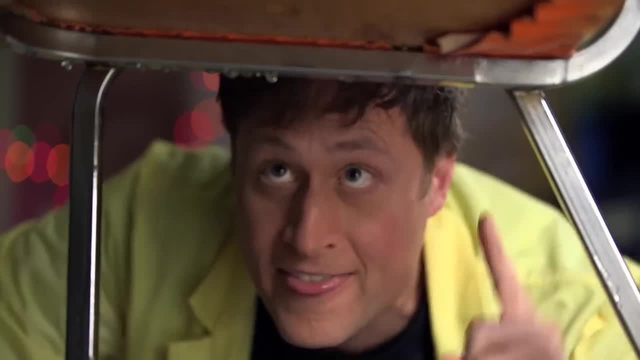 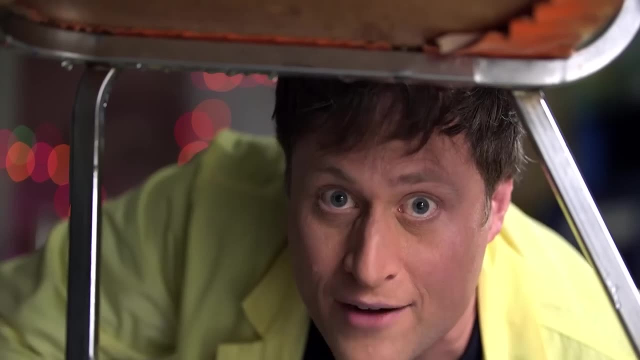 Because it only sticks on a small scale. See those drops of water. That's water sticking to the surface, But it only works when the surface tension of the water is less than the force of gravity, which is why water drops fall when they get bigger. So it sticks to things. That still doesn't explain why you can pour water out of some containers without any drips and other containers make it nearly impossible. Grrr, It's all about the angle. Water will flow very easily when there isn't a large change in direction. 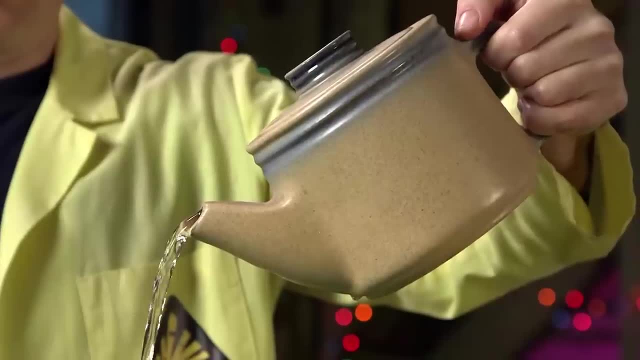 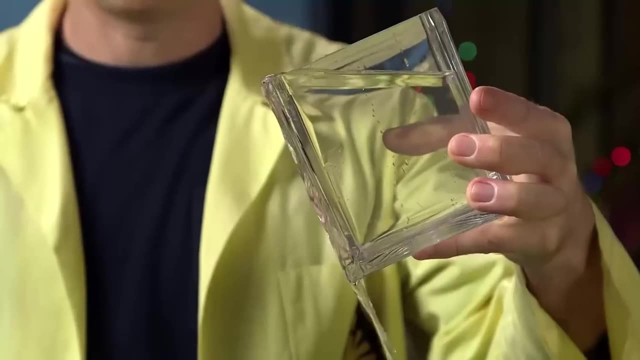 like around the curved top of this glass. But when there's a big change in direction, like at the mouth of this teal, the water can't make that turn as easily. This is also why pouring from a full glass is much messier than one that's less full. 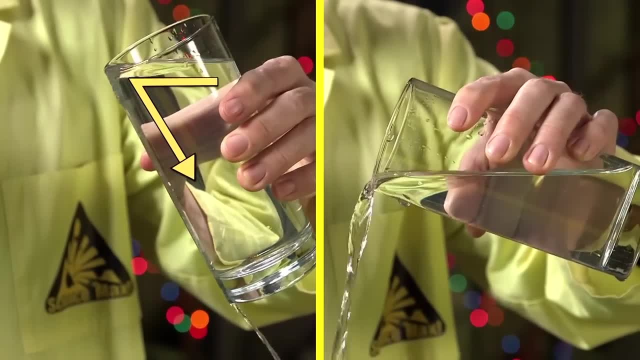 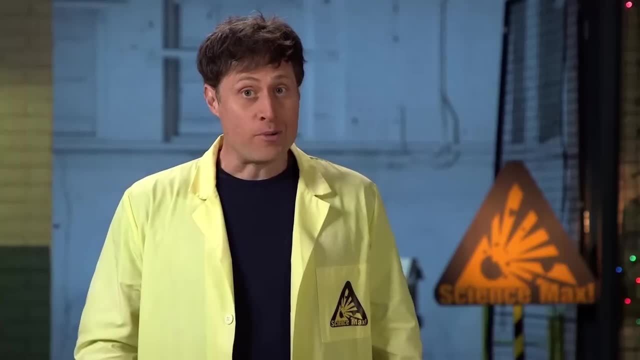 Pouring out of a full glass, the water only needs to change direction this much to flow down the side, But from a half-full glass, the water would need to change direction this much. So all this happens because water likes to stick to things. 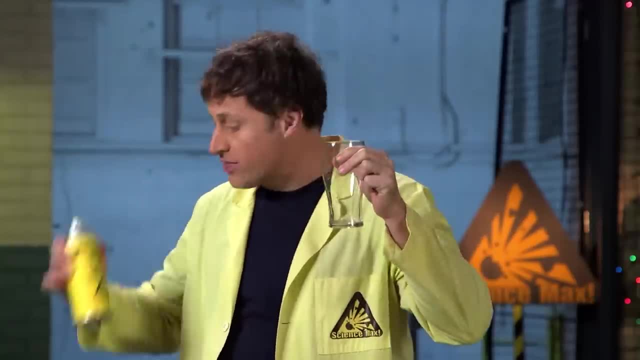 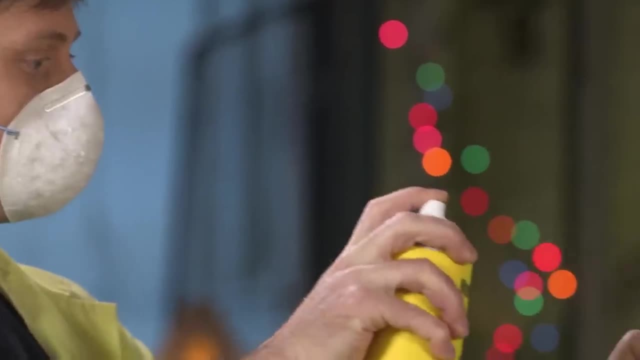 So let's do an experiment and coat this glass with hydrophobic spray. Now, hydrophobic coatings repel water, So if it's repelling the water from the outside of the glass, will we still have the same problem? Well, let's find out. 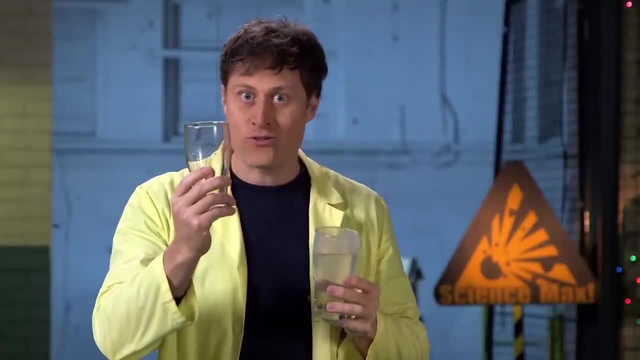 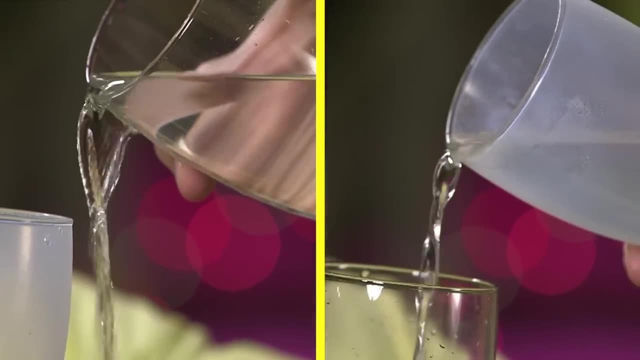 Hydrophobic coated glass, non-hydrophobic coated glass or just regular glass. Water likes to stick to surfaces, but it can't stick to one coated in hydrophobic coating. That's impressive. Should we try something else? Well, that's one way to solve the dribbling glass problem. 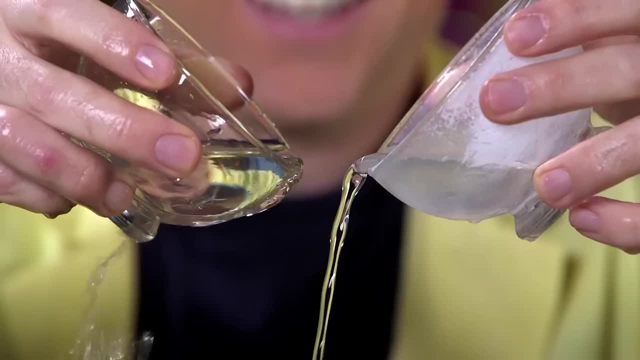 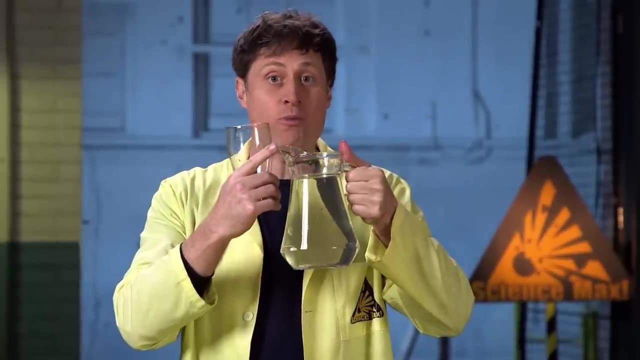 Except you can't coat your glasses at home with hydrophobic coating, because it's not good to eat. The secret is using a container that has a very sharp angle between where you're pouring the water and the underside of the glass, like this jug. 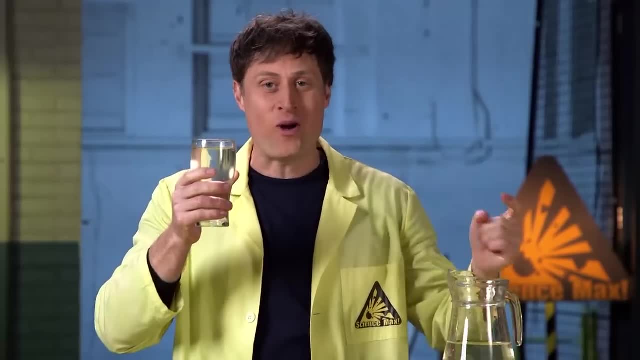 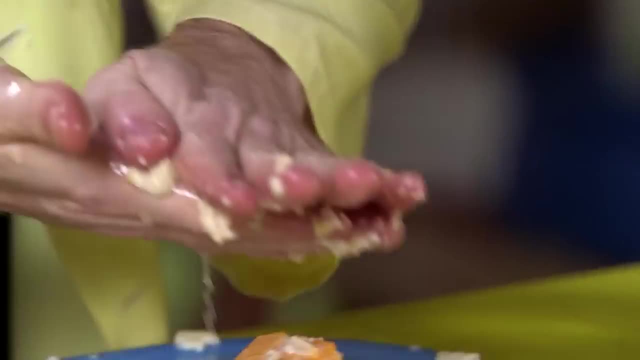 And there you go. Now I can enjoy a nice glass of water with my cheese and crackers. Oh right, I am Wait, hold on, I can re. I will remake the crackers into See. look, see, it's just, it's fine. 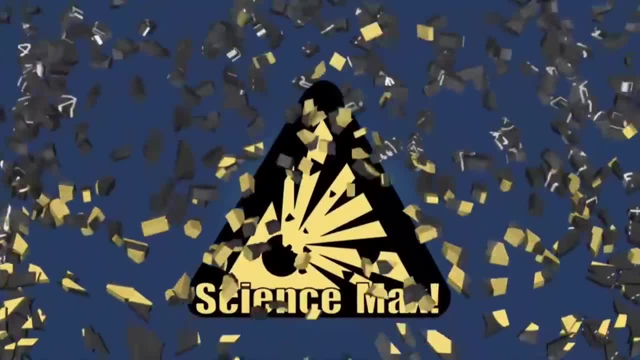 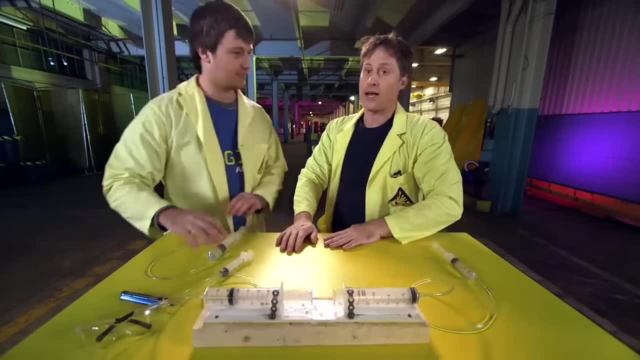 It's fine. I'm not really gonna eat that, I'm just kidding. Chris and I are maxing out our hydraulic crusher. Yes, yes, We're gonna have a little game I wanna play. Okay, great, Great, You can pick either the small one. 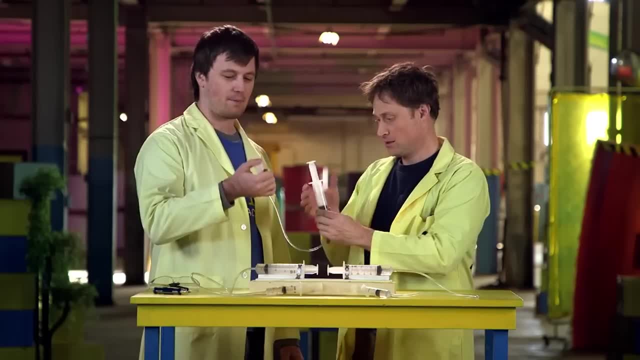 The big one, Okay. So what's the game? Simple thumb war. I'm gonna press down on this side, You press down on that side, We'll see who wins. Okay, are you ready? Yeah, One, two, three go. 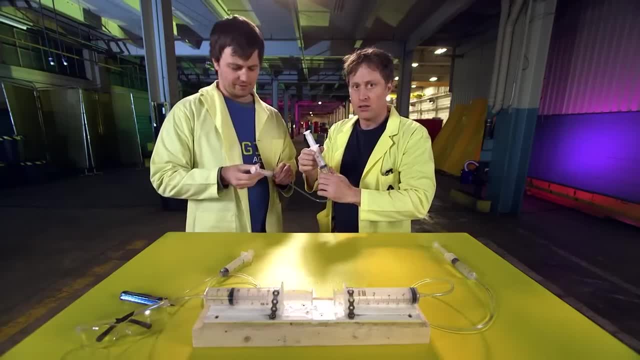 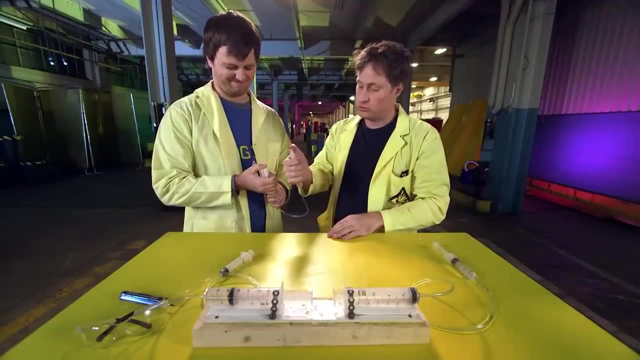 Oh wow, that was really tough. Why was that so hard? Well, Phil, I'm just really strong. Wait a minute, my turn. Okay, one, two, three go. Yeah, see, pushing down on this one is way easier. 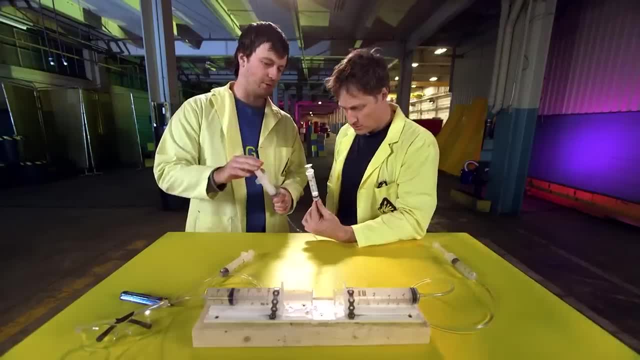 It is, You wouldn't think It is. You wouldn't think that one inch would be easier. Why is that? The reason for it is is that you have to push this one down a lot farther than you have to push this one down. 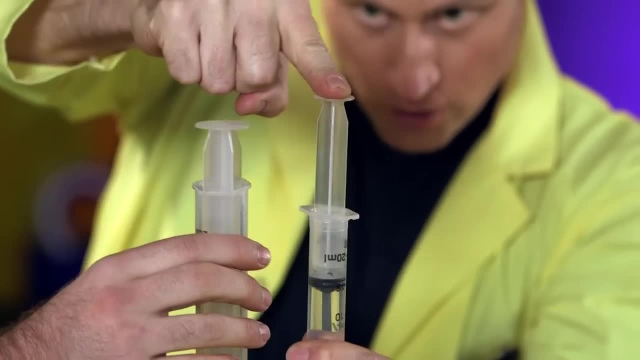 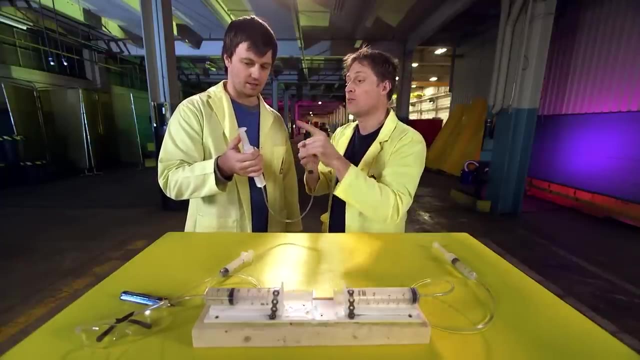 Let me see, See how far this one goes. and this one's barely moving. This one travels much more. This is how we can exchange a little bit of force over a long distance. That's right To a little bit of distance at a lot of force. 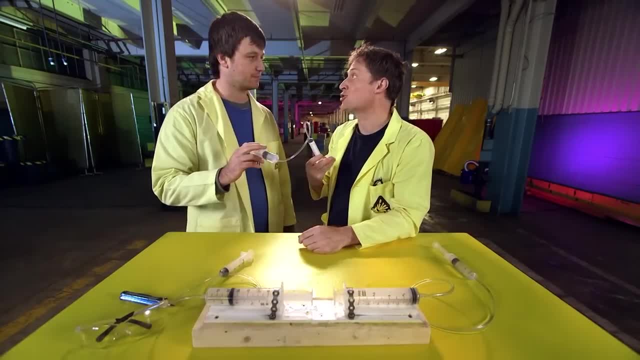 That's exactly right. Just like the lever, It's a mechanical advantage, But in this case it's hydraulic advantage. That's right, Chris, and I pushed down on small syringes, which gives us more force on our larger syringes. 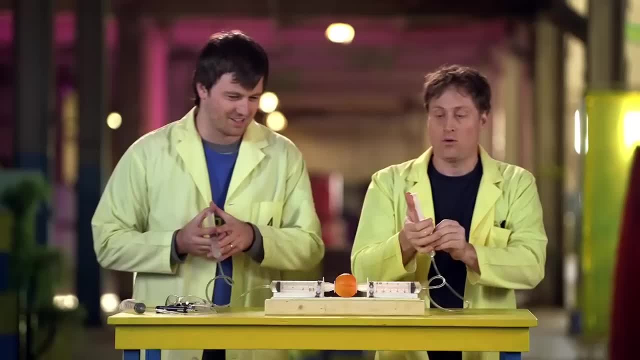 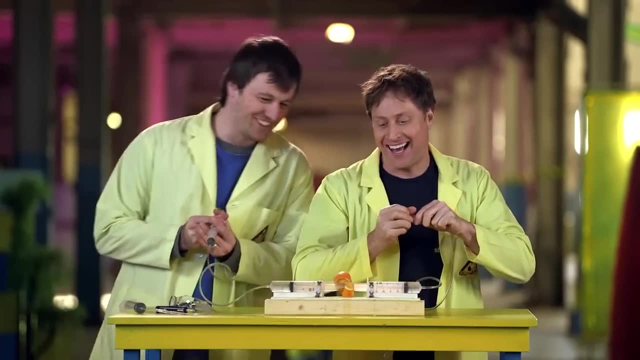 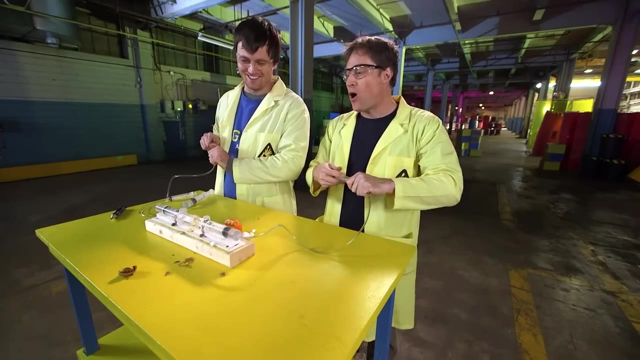 Our crusher was ready to go. Ooh, how about an orange? One, two, three. We squeezed down and Then we tried a walnut. Are you allergic to nuts? I am not. One, two, three When we tried a golf ball. 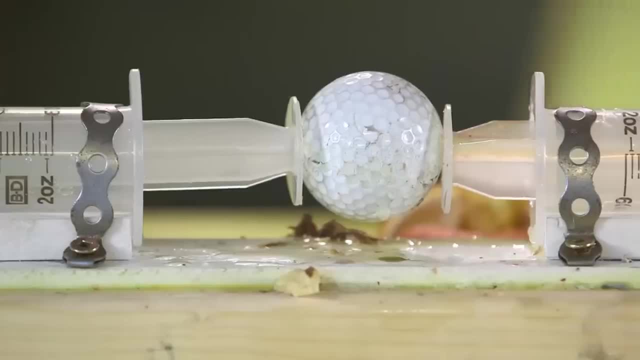 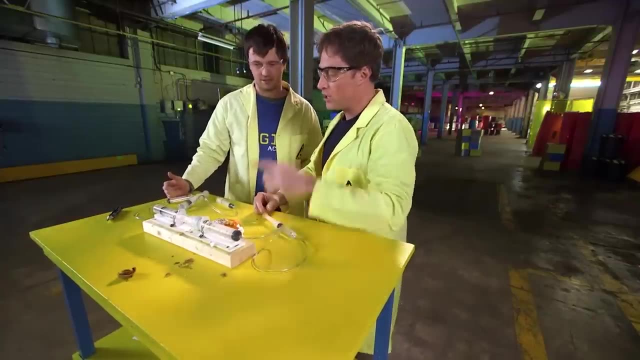 we reached the limit of what our plastic syringes and our hands could do. We need to come up with a stronger, more awesome crushing machine using hydraulics. That's right, I have some ideas. Okay, good, We can go to. 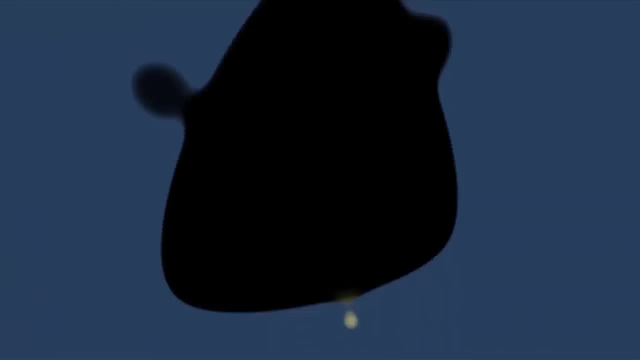 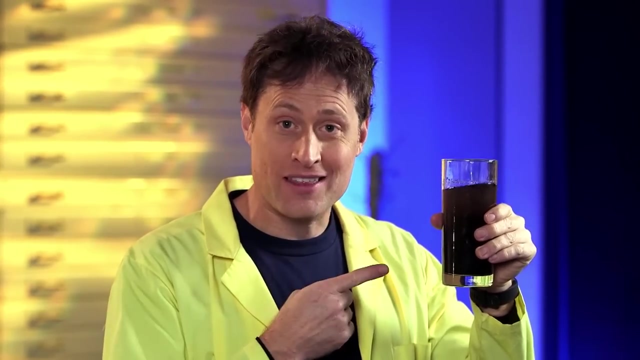 We can use metal. We can use metal And we can use- And we can go bigger as well. Ooh, this water is gross, But I'm gonna drink this water. Why? Well, because of science. No, but I'm not gonna drink the water like this. 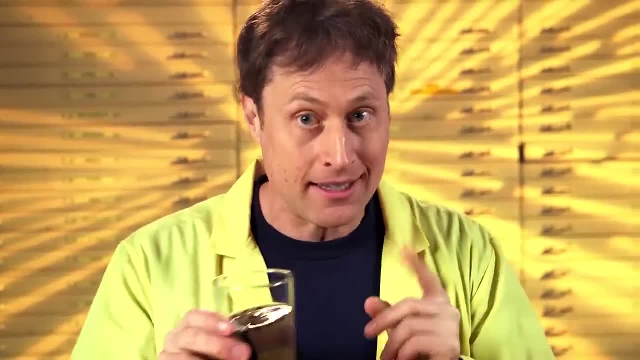 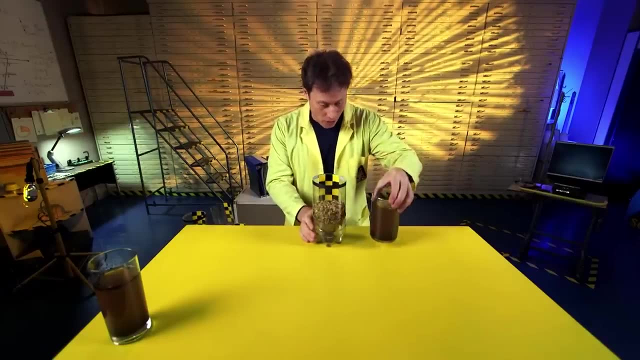 First, I'm gonna use the power of science to help me clean it. How? By using gravel. Gravel, yes, gravel. So say, I've got some dirty water And there are particles floating in that water, Large particles. 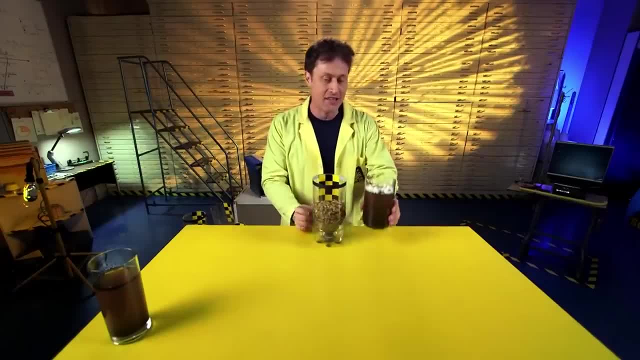 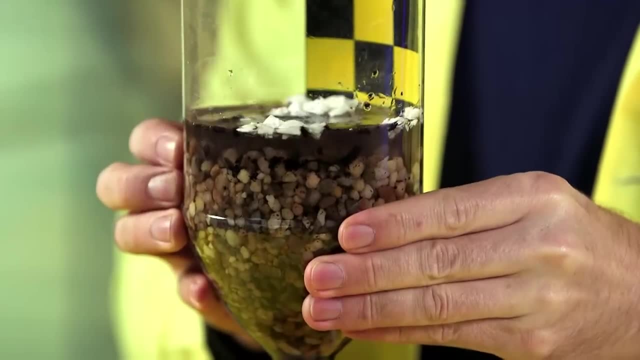 Your rocks, your wood. These Styrofoam bits will act as the large particles. You pour it into the gravel and the large particles get filtered out. See Nothing but clean, clean water. Yeah, I know what you're thinking. 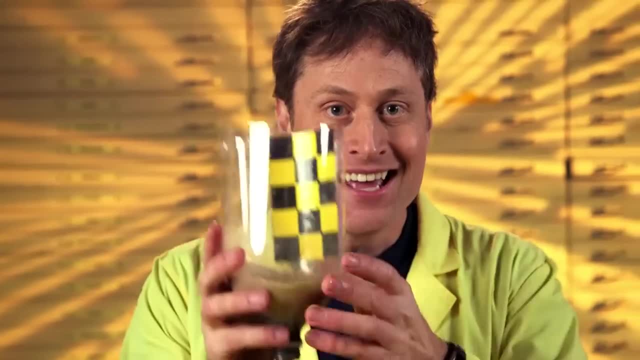 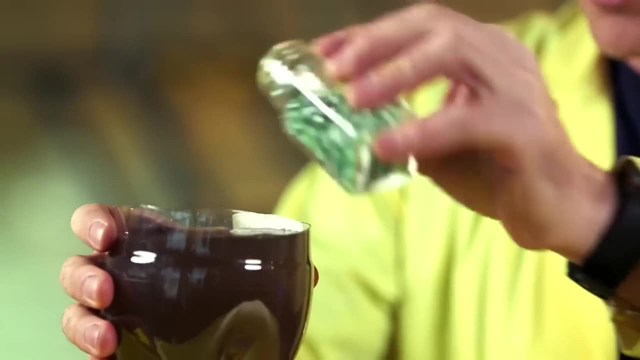 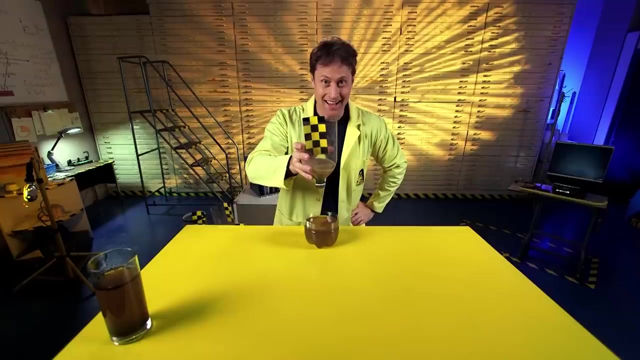 Phil, that's not really clean yet. That's because we haven't done step two: Sand, Sand, Yes, sand. Let's say that these plastic beads are small particles. That filters out the tinier stuff There, Huh. 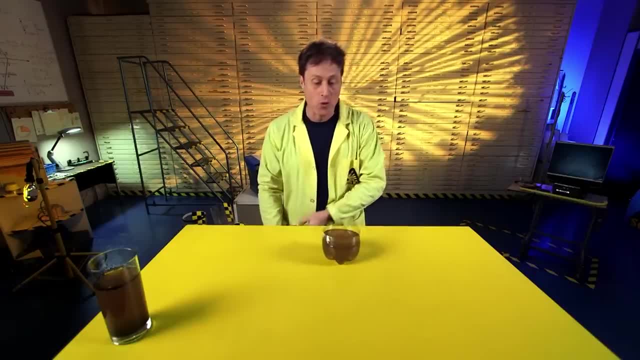 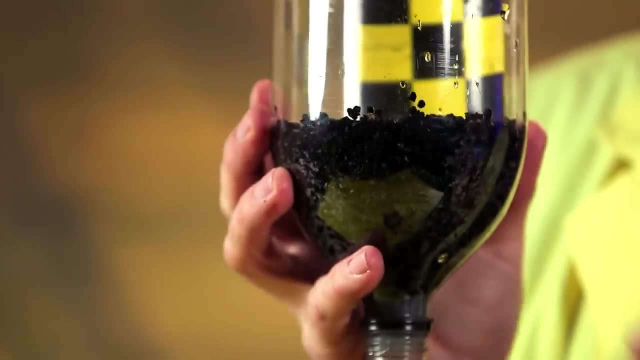 Clean right? No, it's not very clean. So we filter the water in the next step with charcoal. What Charcoal? Yes, charcoal. Charcoal works just like gravel and sand, except on a microscopic scale. Say: these bits are tiny particles you can't even see. 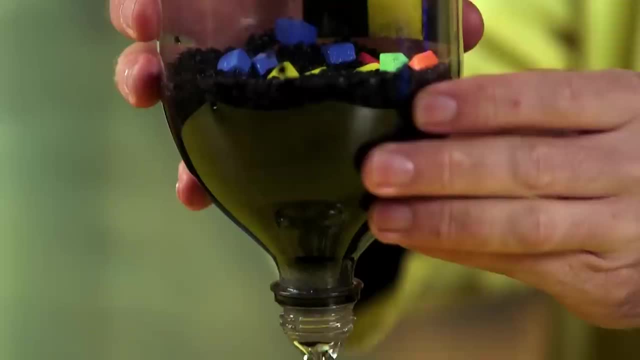 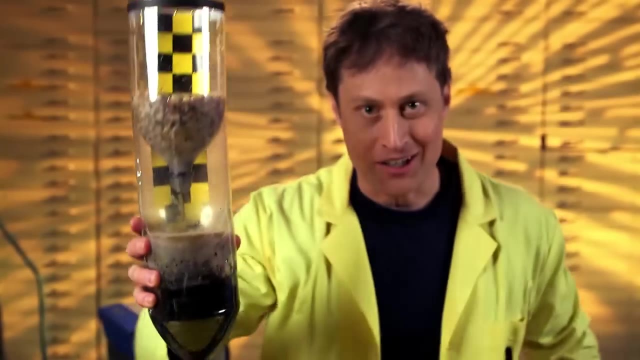 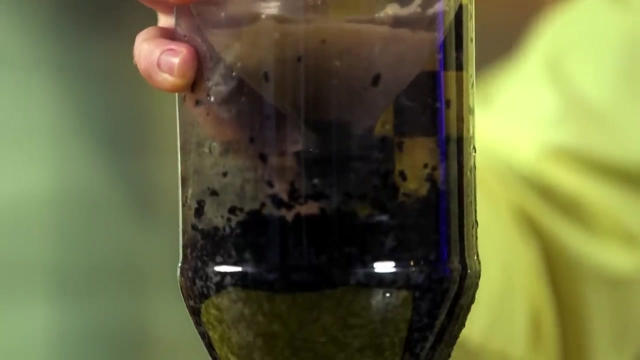 The charcoal catches these, like the sand, and gravel caught the larger particles. This is called a gravel, sand and charcoal filter. There you go: The gravel catches the big particles, the sand the smaller ones, and the charcoal the microscopic ones. These kinds of filters are used all over the world. 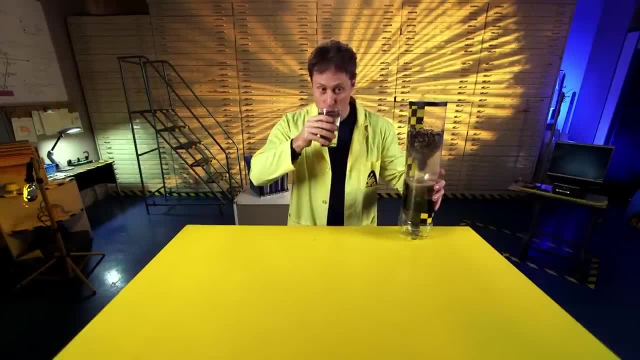 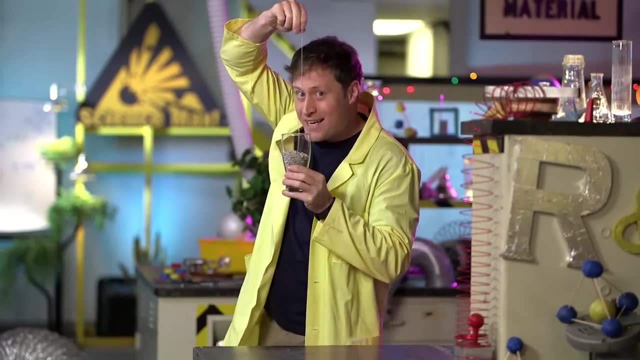 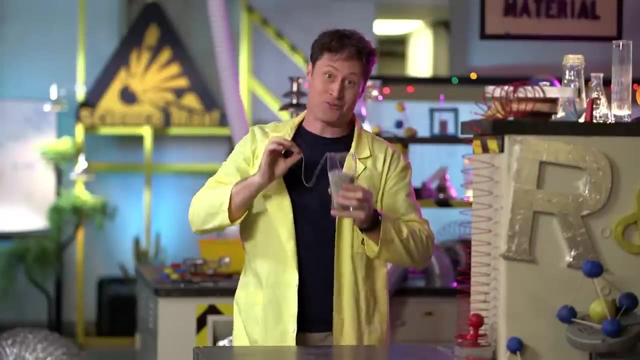 to clean drinking water. Ah, Delicious Science. This is a chain of beads and this is a glass. Now, if I was to drop the chain of beads, what'll happen? It will fall. Yes, that's right, It'll fall because of gravity. 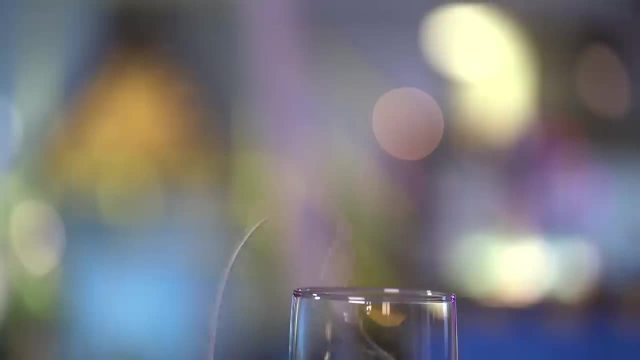 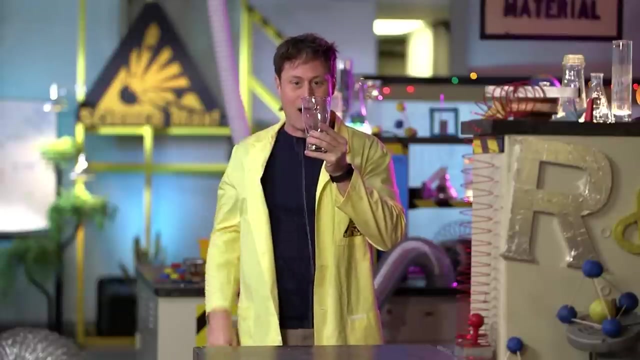 But watch this. This side goes up. Why? Because of gravity. Wait a minute, wait a minute. Why does one side go up? because of gravity? Well, it gets a little complicated, but I can explain. Um, but I think I should. 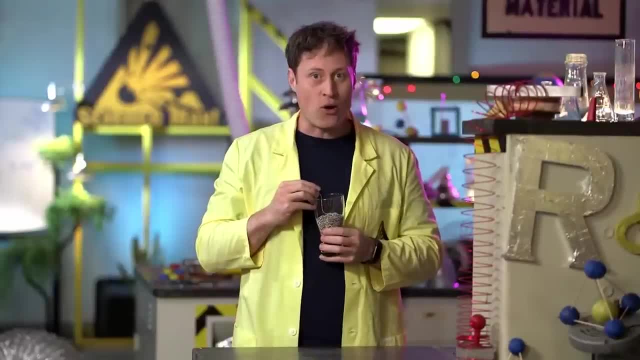 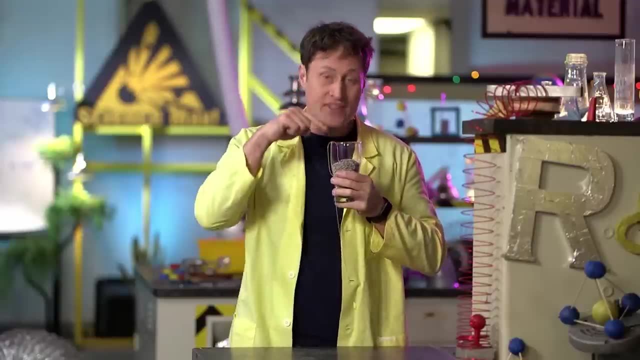 I have to put the beads back in the glass. Okay, so what's going on? Well, when this part of the chain starts falling out, it gets longer and longer and it has more mass than this side of the chain. And if it has more mass, then it has more inertia. 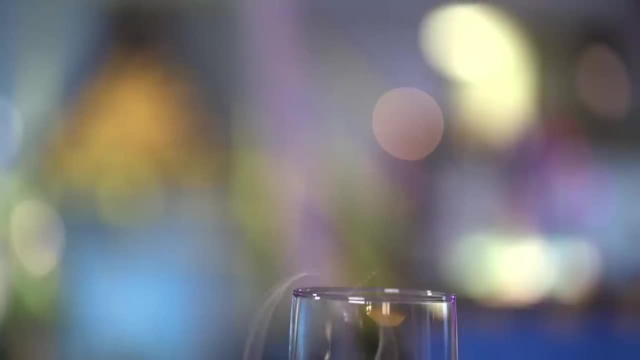 When it starts yanking out very hard, this side of the chain gets yanked up out of the glass very quickly. When it gets yanked up hard it flies into the air. But then of course the direction has to change. 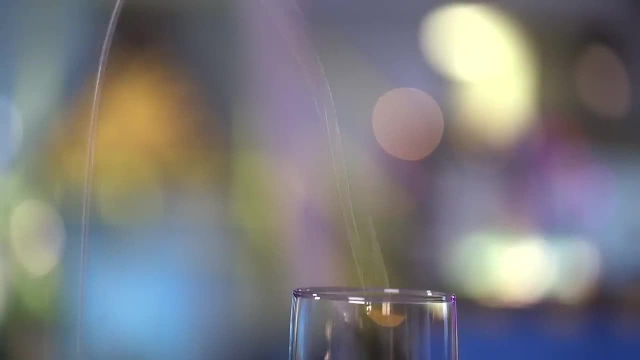 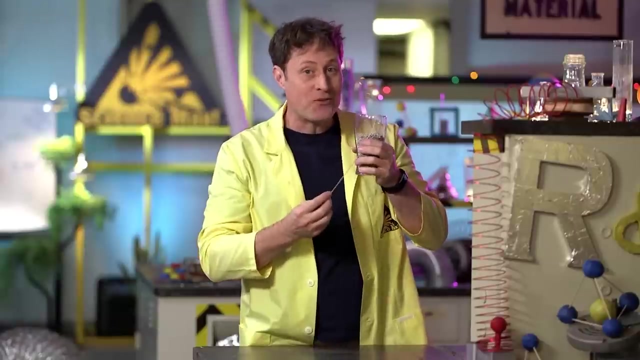 so it goes around a curve and then goes back down. Because of the speed that it's going, that curve starts lifting up over the top of the glass, And that's how it works. There's a big difference in energy, because this chain falls far. 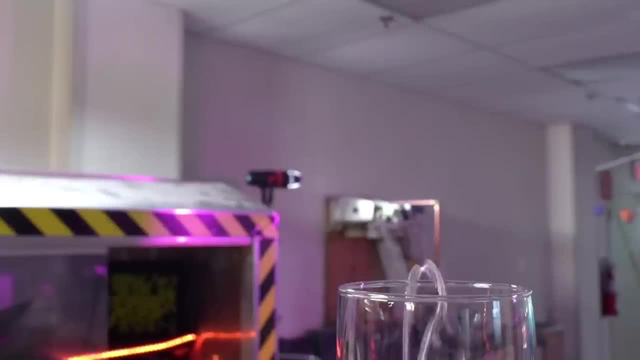 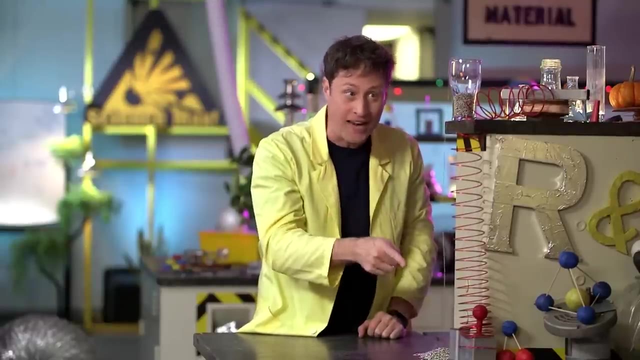 I try it from here and it doesn't work as well. Why? Because the drop from here to here isn't as big. You want lots of force acting on the falling chain, which means the higher you do it from, the better it works. 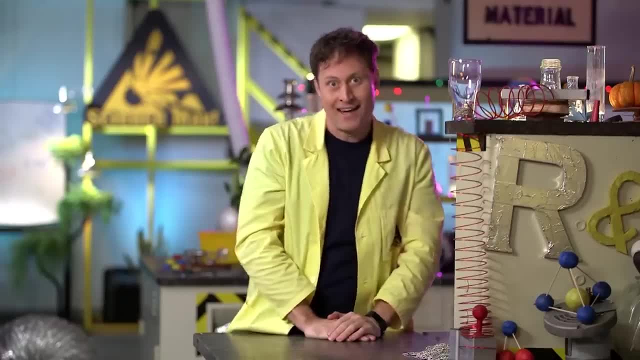 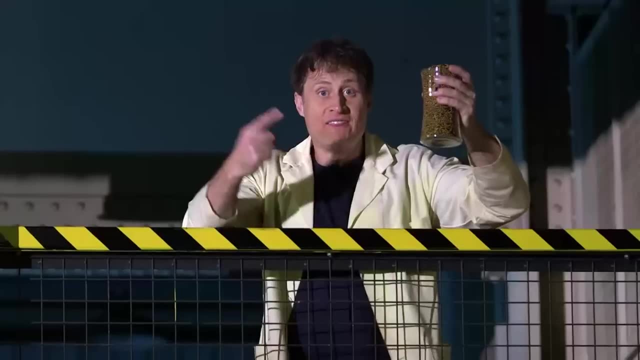 So maybe we should max it out. Yeah, Oh wait, we should wait for it to stop, And now let's max it out. This is a really long chain and this is a really long drop. Let's see what happens. 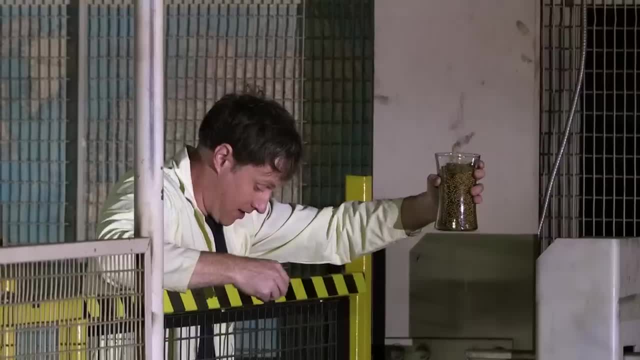 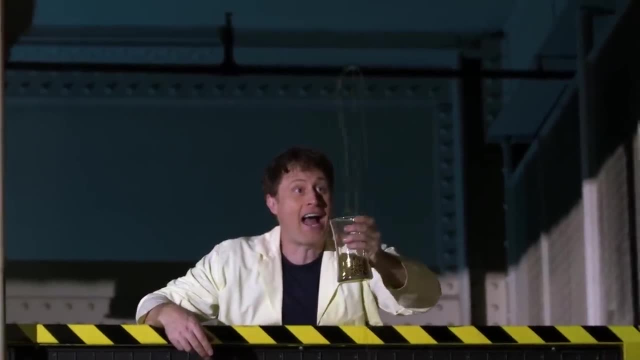 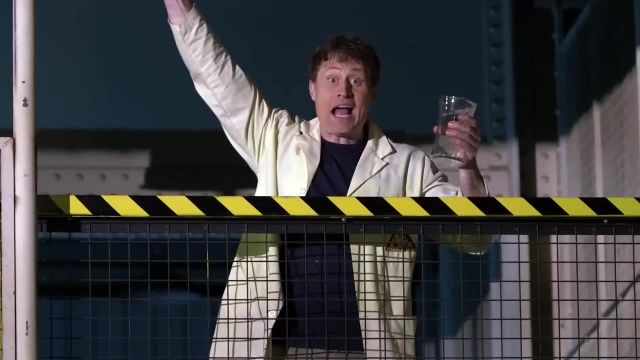 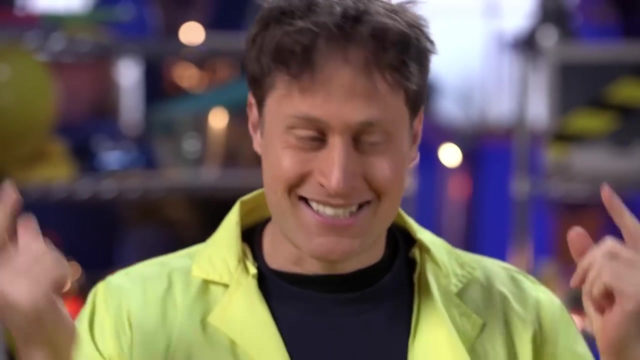 Let's see Whoa Ha ha ha. Look at that. Whoa Super maxed out Science. Now we're going to talk about tension. What's tension? One more than nine-shin. Get it, Because tension and nine-shin. 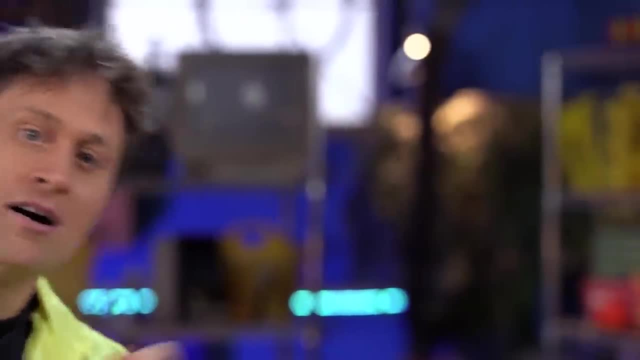 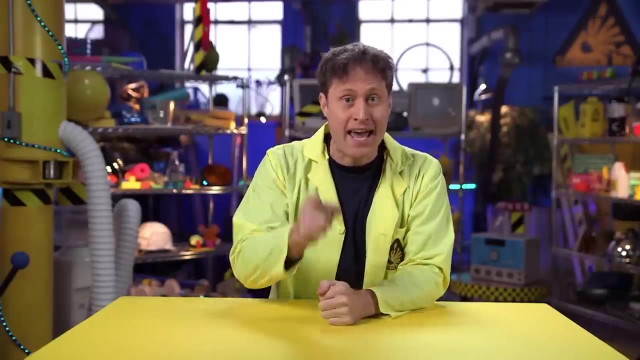 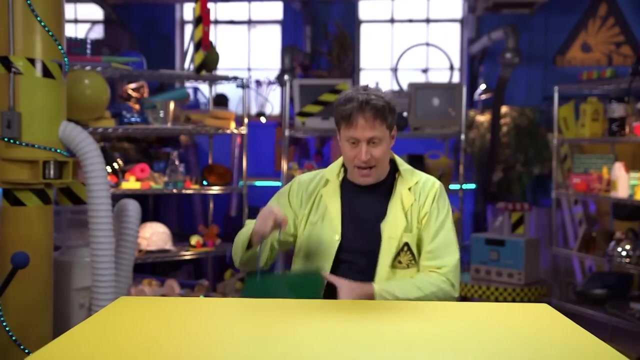 This. Okay, I'll You, Because that tension is the force that we usually talk about when we think about pulling a rope or a chain or something like that, Because you know the old expression, you can't push a rope. But today we are gonna push a rope. I have a rope right here and I'm going to push it using another force called. 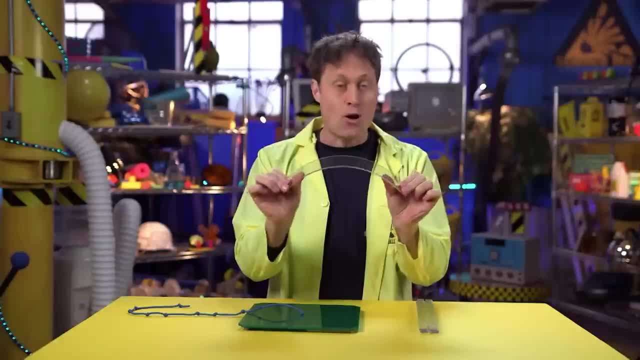 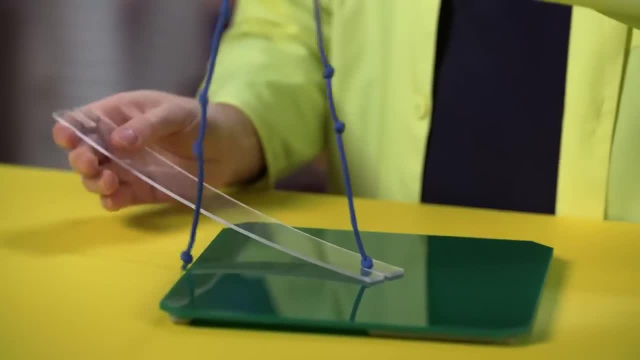 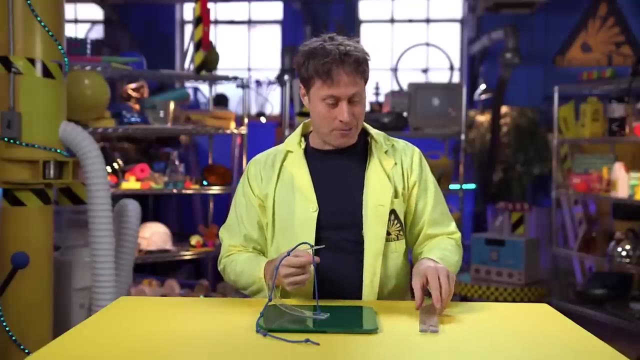 Flexion. I've got some pieces of plastic here and they bend or flex and when they do, they want to spring back. But I'm going to prevent them from springing back by putting them In between these knots. huh and look, the rope now stays up. and take another piece and I stick it on this knot and 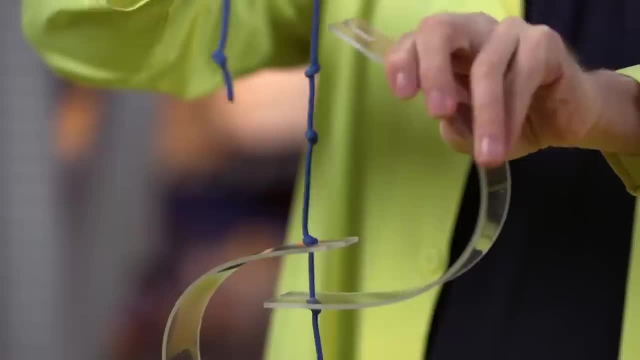 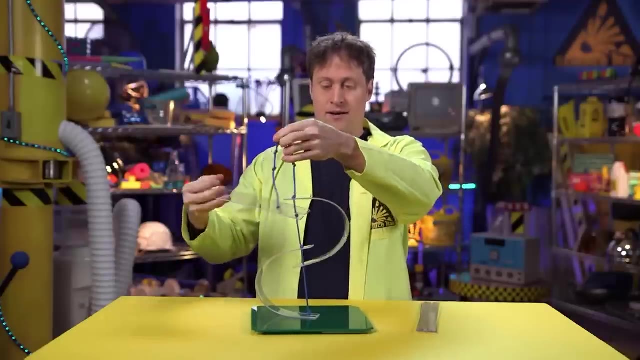 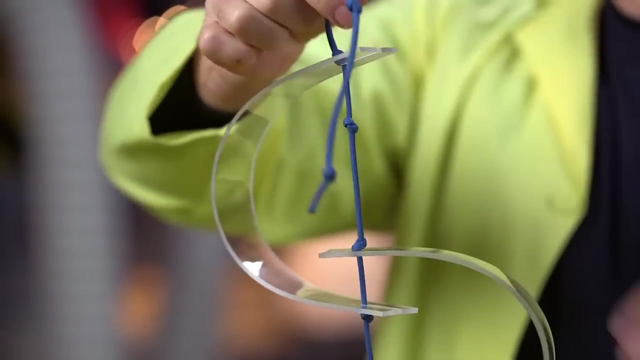 Then I bend it all the way. This is not terrifying, really, It's not terrifying at all. Okay, and then I take this piece and I put it here and I bend it around, and So now We have a rope that's being pushed and we're defying gravity and we're making a cool. 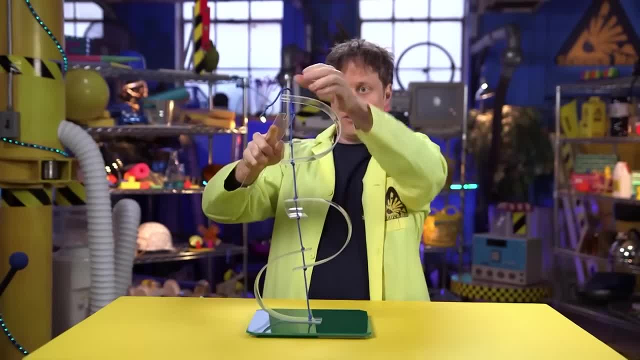 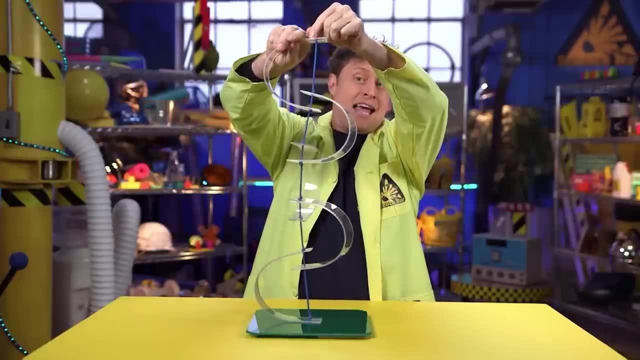 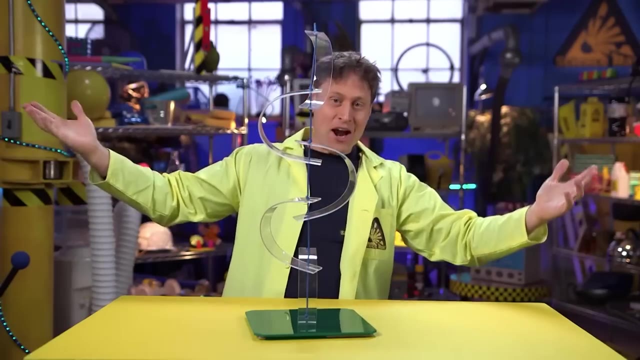 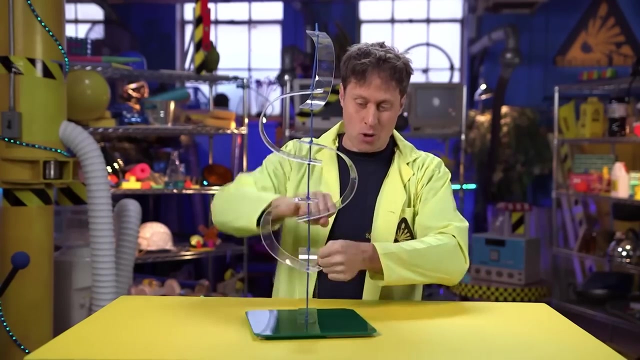 Art sculpture. all right, one more here. Whoa. okay, here We go and Flexing, There you go. I've pushed a rope, defied gravity and made a cool art sculpture. Okay, well, I guess technically I haven't really pushed the rope, because we're still pulling from each knot. 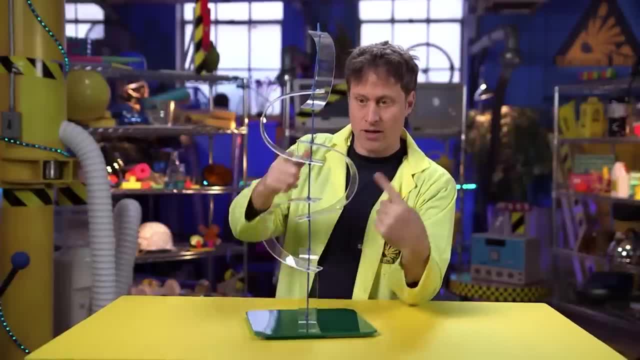 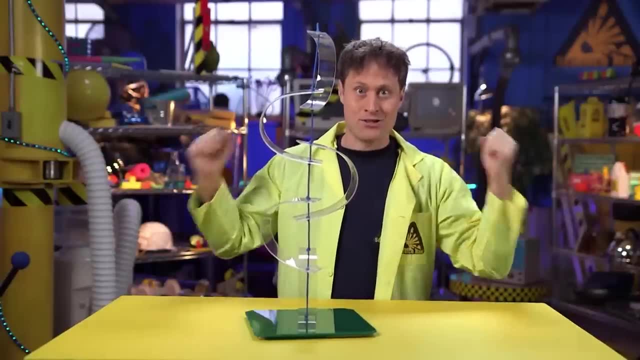 And I guess I haven't really defied gravity because that one's sitting on the table and all the others are sitting on top of that. But you can't argue that I made a cool art sculpture. Haha, art, I mean Science. here is an experiment you can do at home with friction. This is a toy boat. 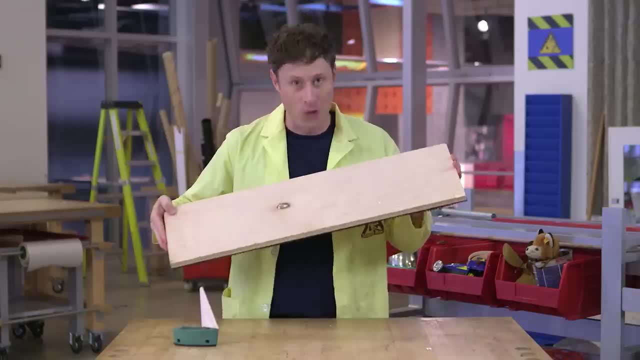 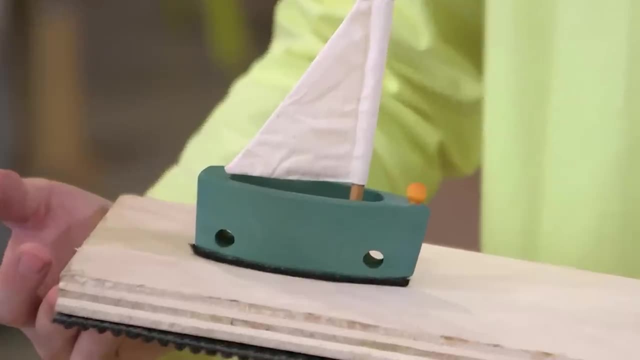 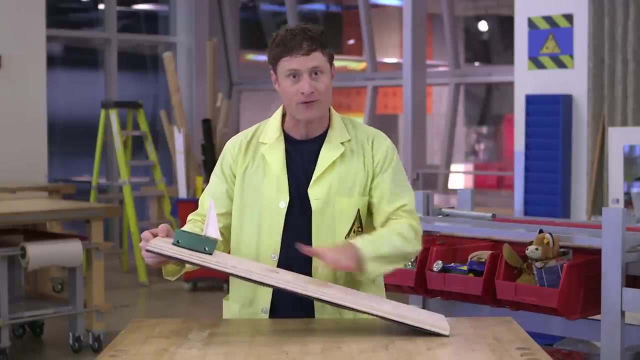 Yes, you guessed that right. and this is a wooden plant, correct? That's two for two. I put the boat on the ramp and watch what happens- Nothing. The reason why is because the friction between the boat and the ramp is enough to counteract the force of gravity. 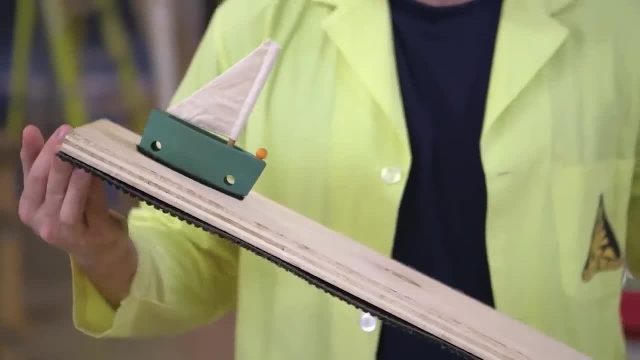 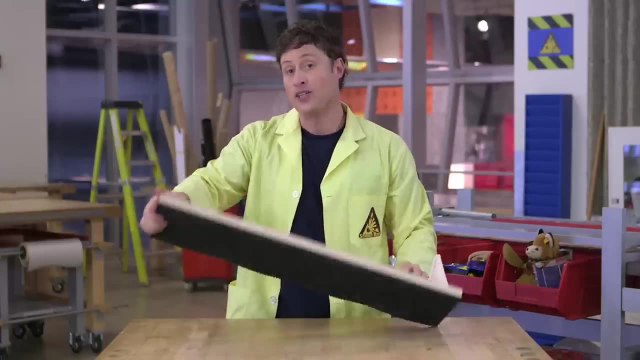 Trying to pull it down. but watch what happens. if I raise the ramp to the right height, the boat slides down Because the friction isn't enough and gravity pulls it down. but when we change surfaces to this carpet, Let's see what happens. same angle: I can raise it higher, higher, higher. 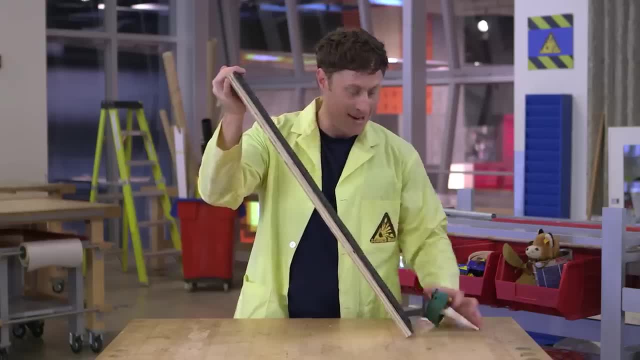 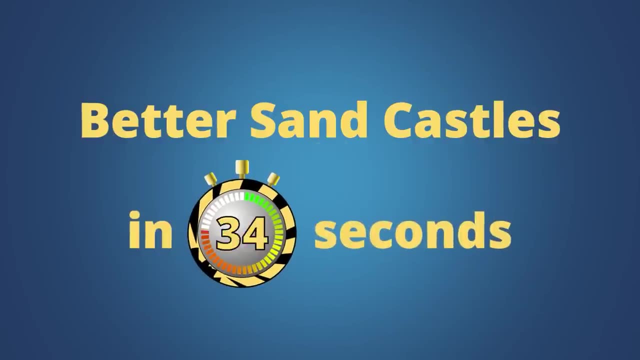 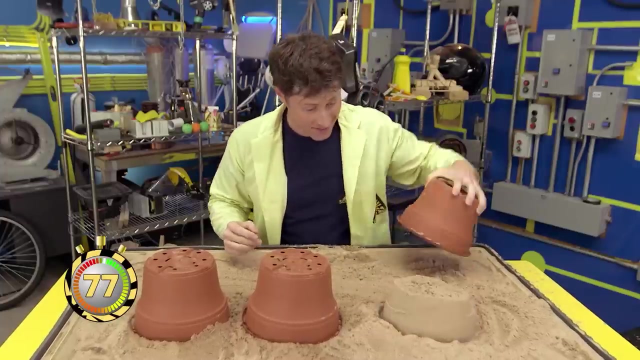 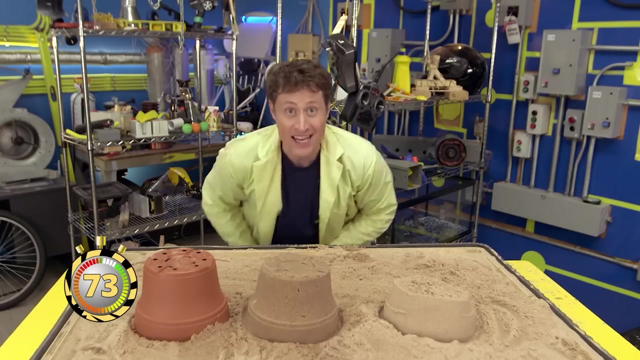 because There's more friction between the carpet and the boat than there was between the wood and the boat. better sand castles in 80 seconds. Building sand castles is fun, but you can't use dry sand because it doesn't stay up very well. You have to use wet sand. but even if you use wet sand, it doesn't hold a lot of weight. 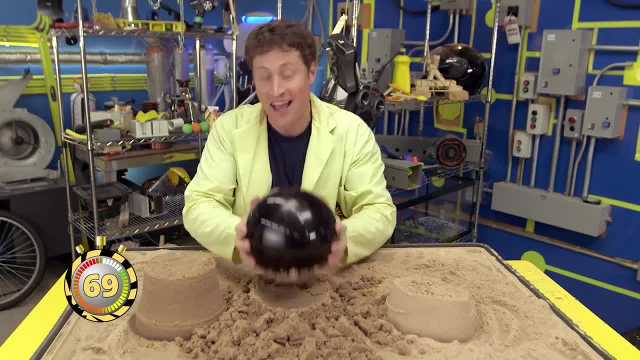 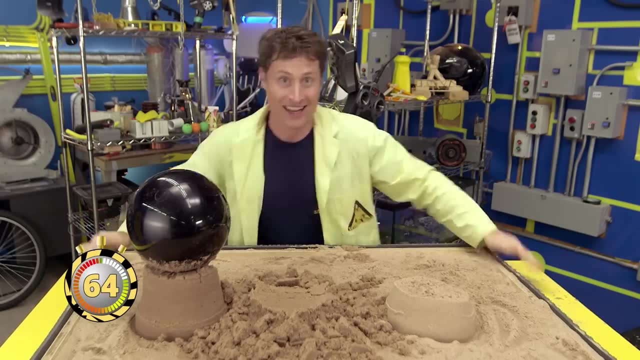 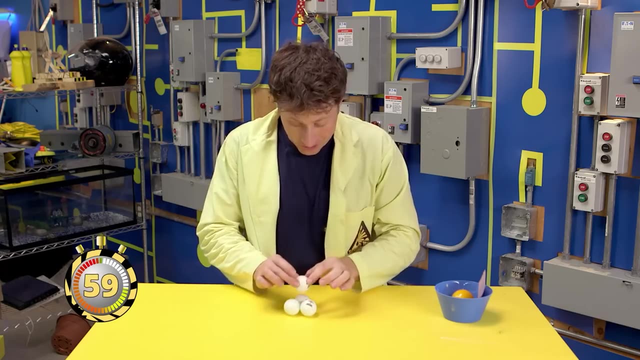 But if you use sand with the power of science, it does hold the weight. dry sand, wet sand, Science- and here's what's going on- Say: these ping-pong balls are grains of sand. when they're dry They don't hold together very well. That's why you can't build a sandcastle out of dry sand. 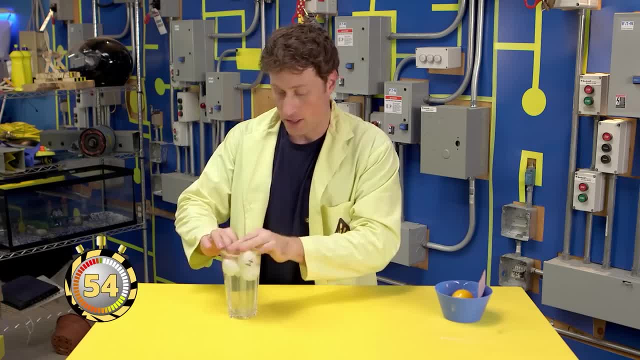 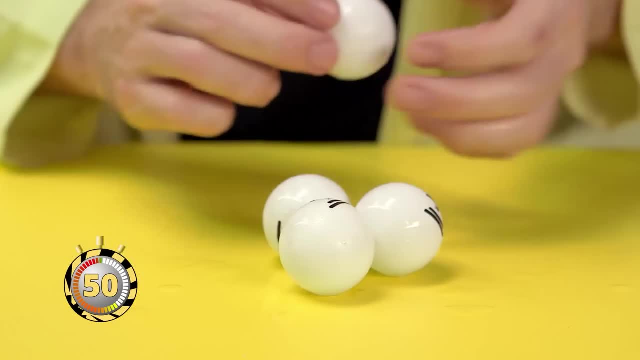 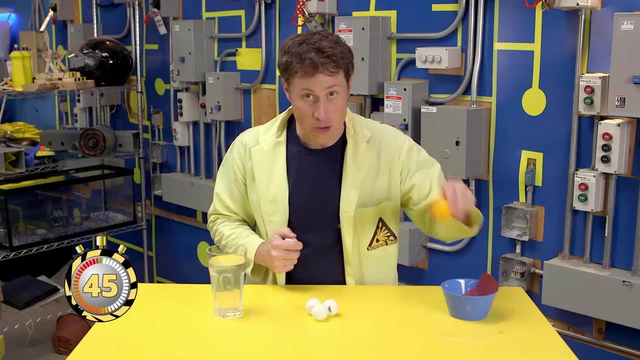 But if you get the sand wet a little bit, The grains of sand will hold together a little better because of the surface tension of the water. That's why it's easier to build a sandcastle With wet sand, but they still won't hold much weight. 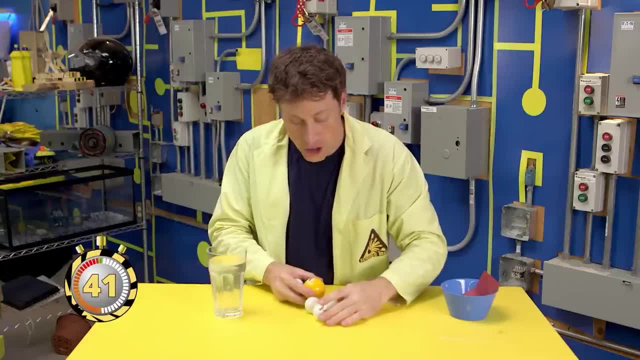 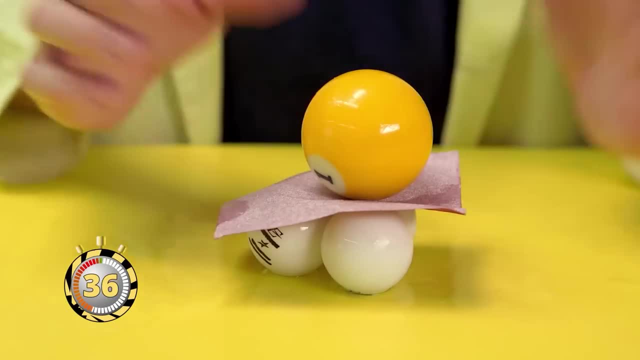 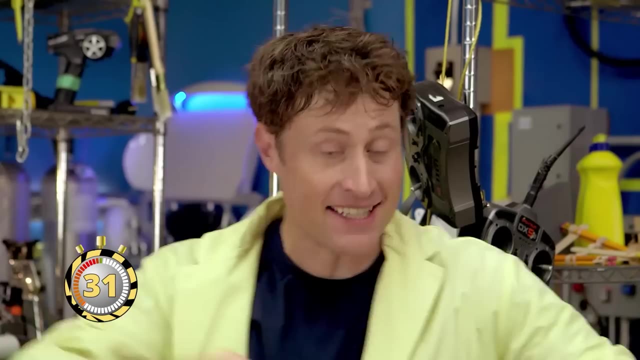 But if you add something that creates even more friction between the grains of sand, like, say, this sandpaper, It will hold the weight. So here's what you do: take Window screen and cut it into circles. Make sure you get an adult's permission first. Okay, deal, put in a layer of sand. 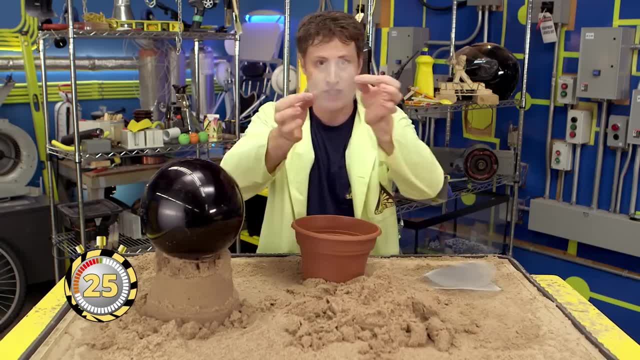 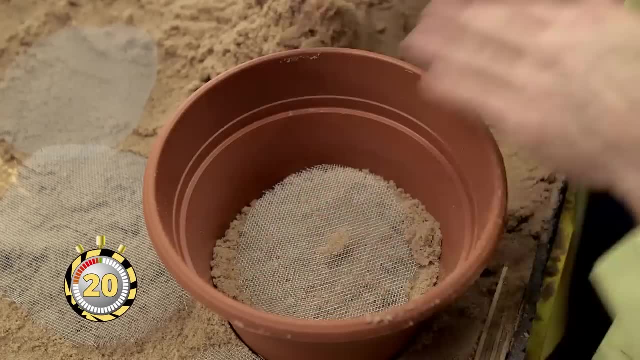 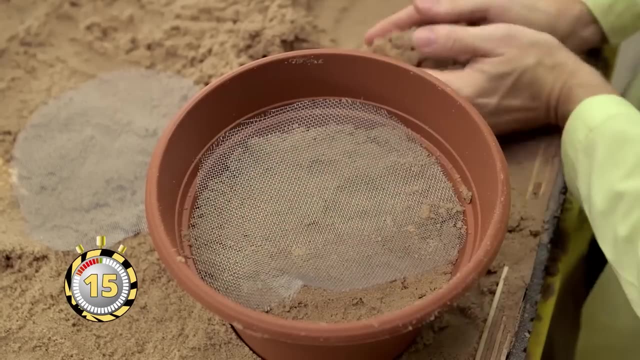 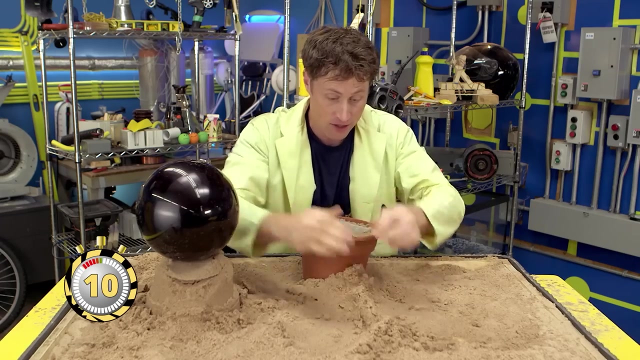 Pack it down and put in a circle of window screen and a layer of sand. pack it down circle of window screen. Then you guessed it layers and pack it down circle of window screen. The window screens are gonna add more friction between the grains of sand and will make your sandcastle. 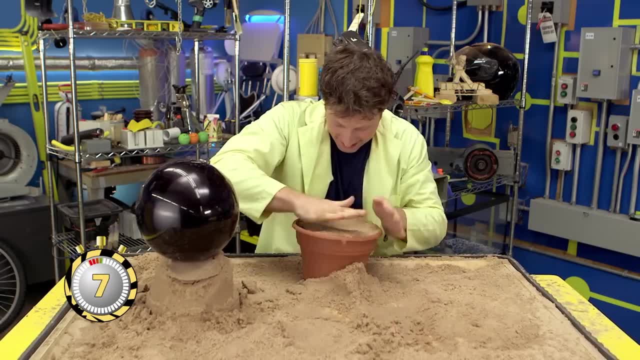 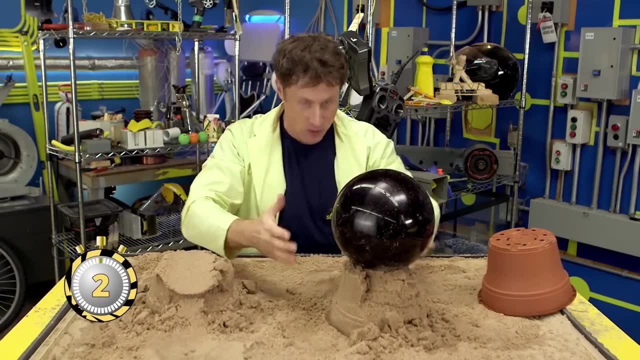 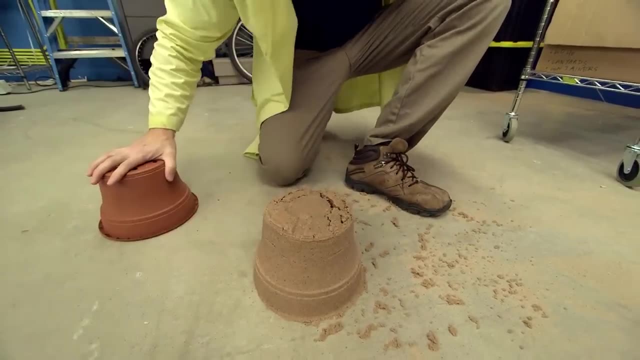 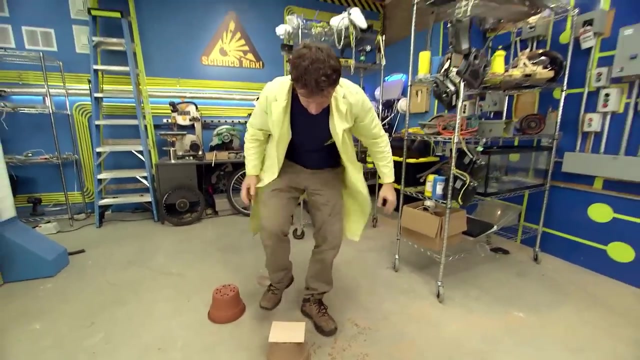 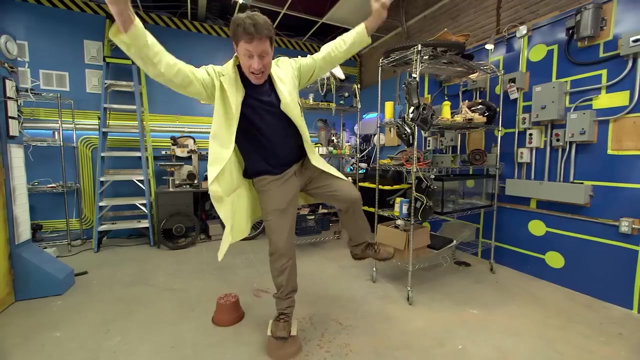 Strong, strong with the power of science, and then You can put lots of weight on it And there you go, sand with the power of science. Okay, I had to max it out. let's see how strong science and really is. Huh, Science mousetrap. 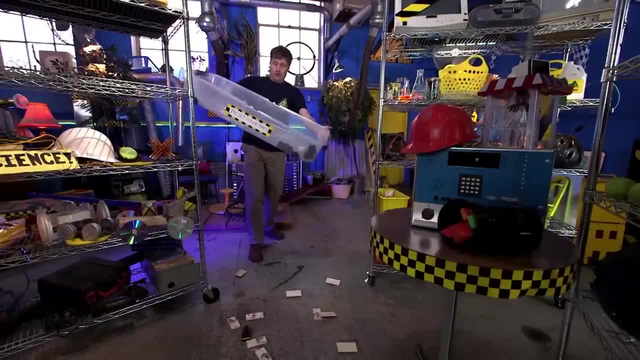 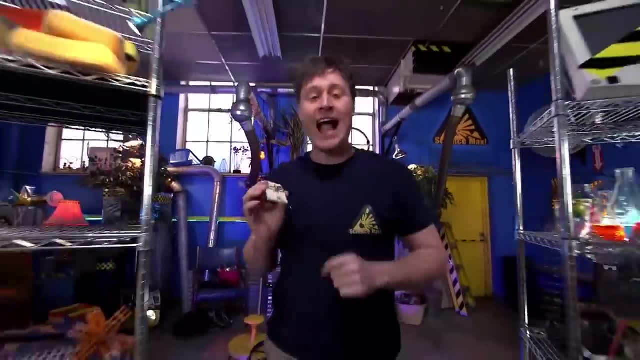 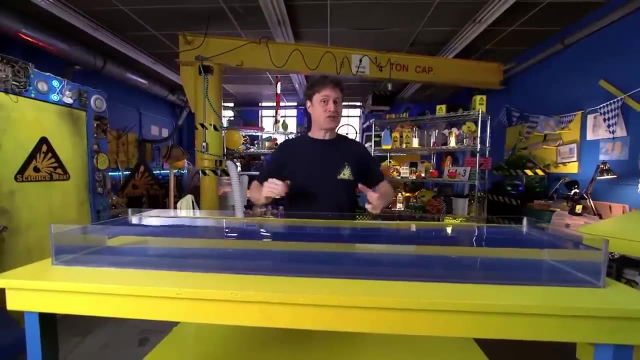 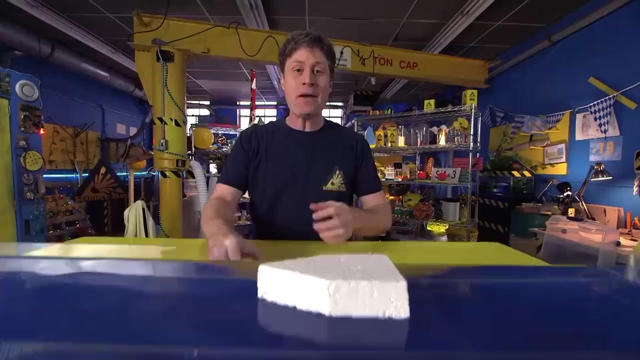 Oh, Like I said, we are going to be using, Huh, mousetraps, mousetraps as a form of Propulsion. that's the force that makes things go, and we are going to be making a boat go. And what is the thing that's going to make this boat go? a mouse, Oh, oh, it's not set, Sorry. 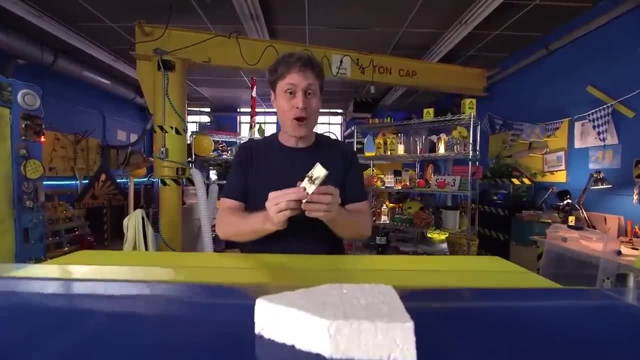 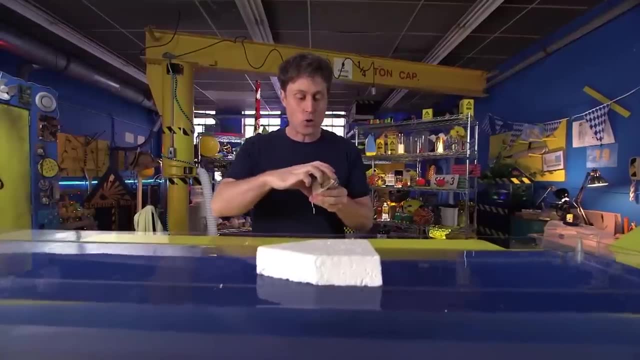 I'm really jumpy. Anyway, We're gonna be using a mousetrap and, don't worry, No mice are gonna be harmed in the making of this or any science max episode. But mousetraps are really great because they can store energy in the spring. if you see, there's a spring that makes this bar want to. 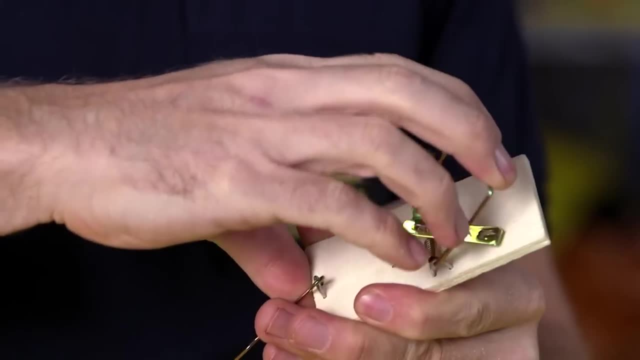 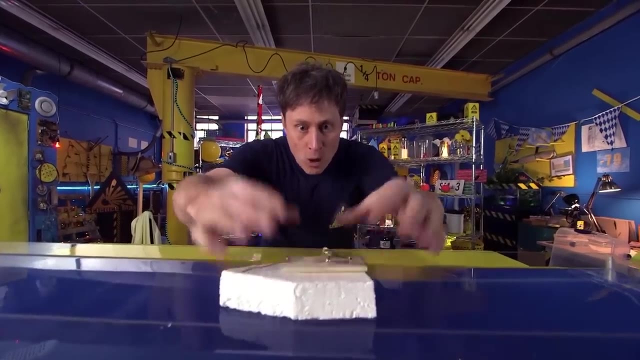 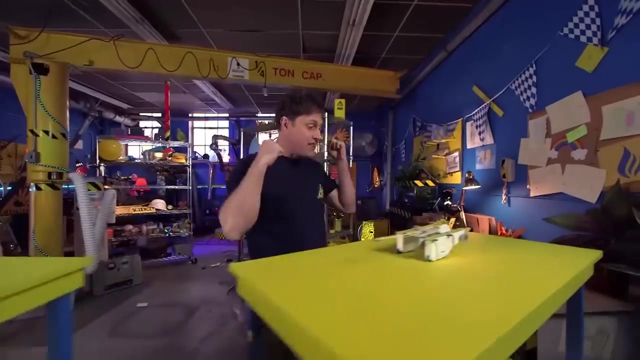 Snap back, but we can put energy into the spring and store it and then use that energy as it unwinds the spring To propel our boat. but it's a little more complicated than just this, So come on, I'll show you. What we're gonna do is build this. This is the mousetrap boat and it works like this. 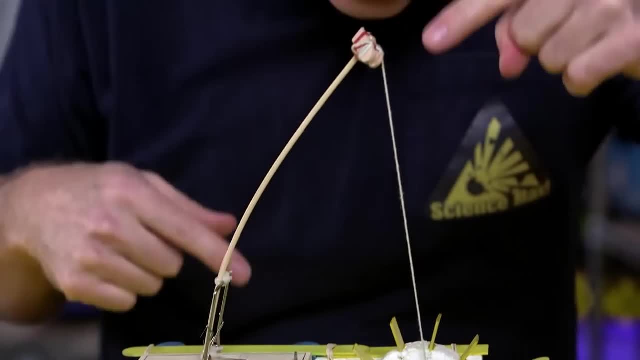 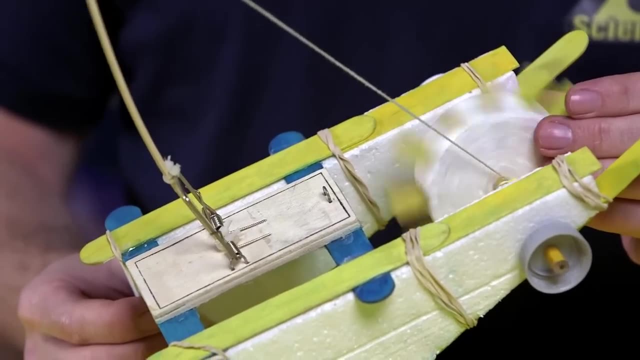 I've got the mousetrap and it's attached to a long arm. that arm has a string on it and it goes around the paddle wheel And as the mousetrap unwinds the paddle wheel spins Like that which pushes the boat forward. now looks kind of complicated. 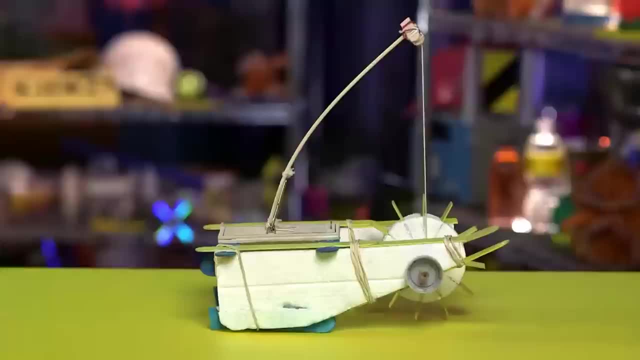 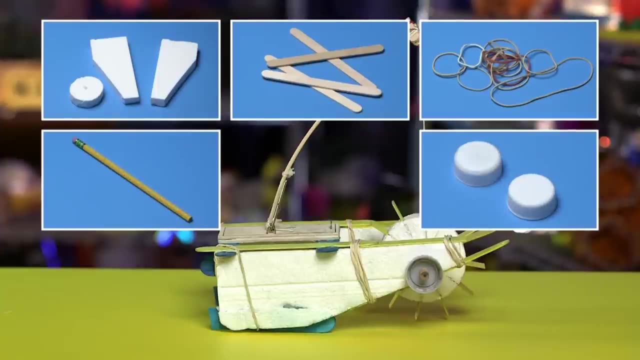 But it's actually quite simple to make, and here's what you need. My mousetrap boat is made with styrofoam, craft sticks and Plastics. you'll also want a pencil, plastic drink caps, a shish kabob skewer, small zip ties. 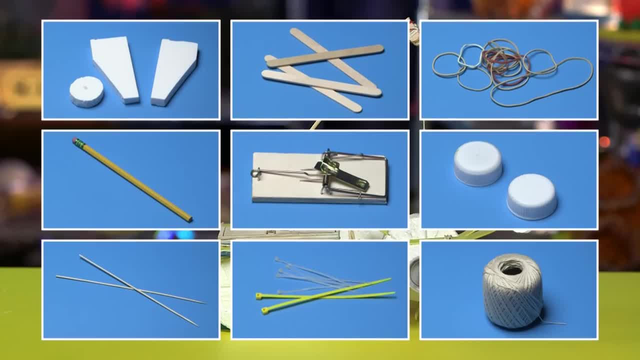 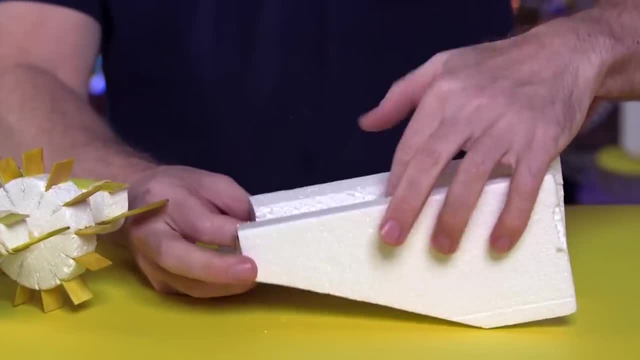 String and, of course, your mousetrap. now, mousetraps can hurt your fingers, So get an adult to help you when you use it. start with two pieces of styrofoam. I like to cut mine into this shape, But the only really important thing is that they're the same size. 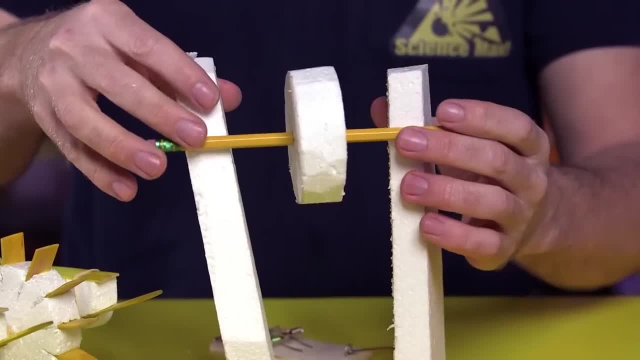 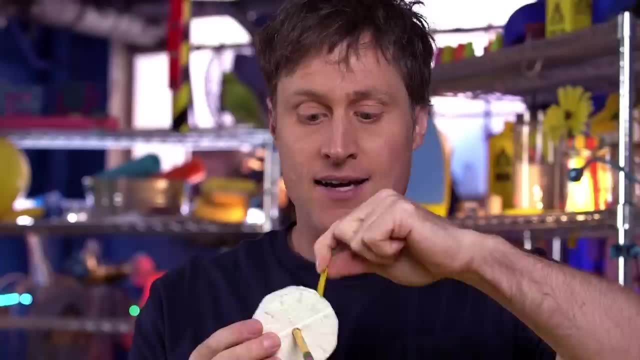 Your paddle wheel is made from a circle of styrofoam with it penciled through the middle and it will go across like this. To make the paddle wheel, I use cut pieces of craft stick- or they can be plastic- And make some cuts and then put them in like this: 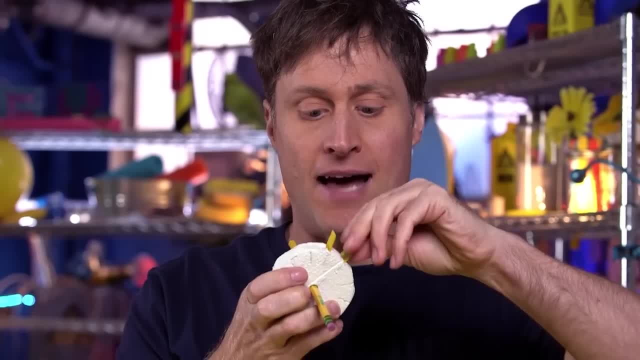 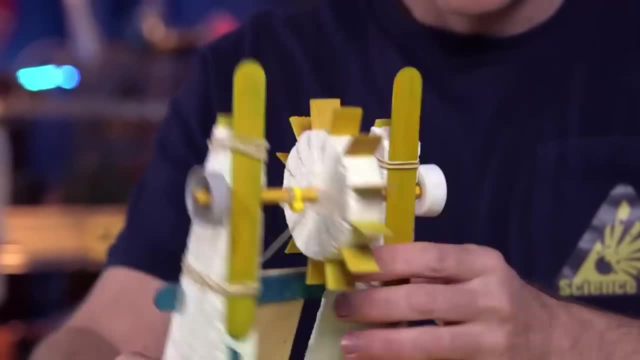 And that is what will make your paddles on the paddle wheel, because that's the wheel and that's the paddle paddle wheel. That's why they call it that stick drink caps to the ends of the pencil after sticking it through this styrofoam. I like to use a few craft sticks and elastics that help give this styrofoam strength. 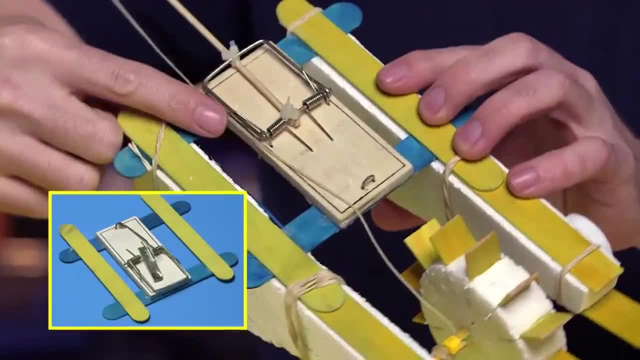 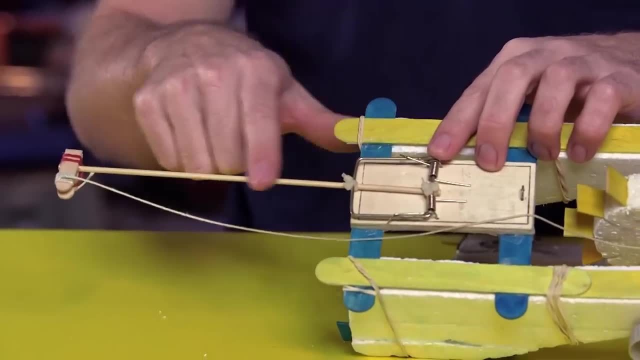 Next is the mousetrap which you want to glue down to a frame of four craft sticks. Attach the frame to the boat with the elastics, then attach the shish kabob skewer or a Pencil to the mousetrap with zip ties. I like to put some craft sticks on the end to make it easier to tie the string to it. 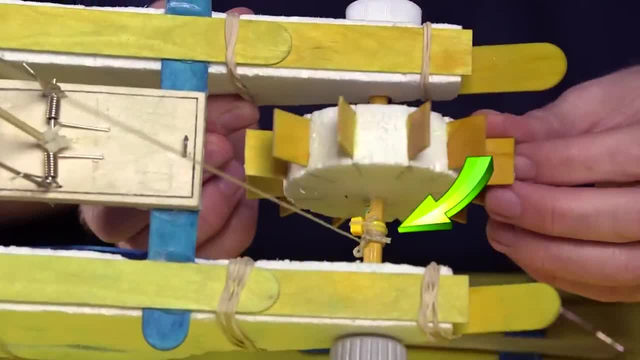 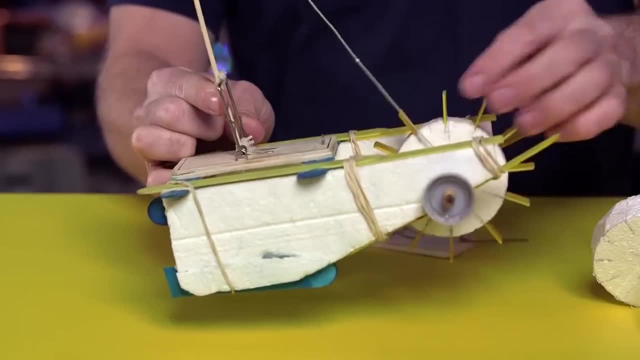 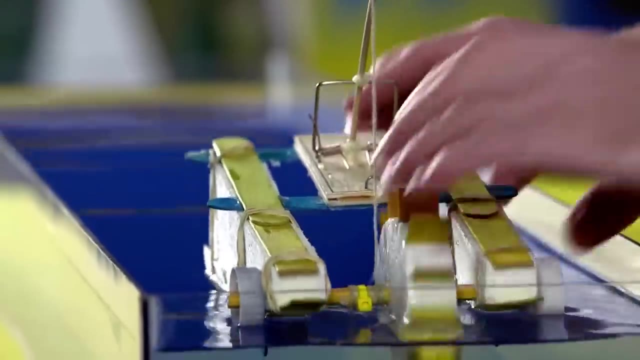 Wrap the other end around the paddle wheel pencil and remember you need enough string so that your stick can lie flat. Okay, let's try it out: wind up the paddle wheel. This will be a little hard as the spring will pull back, But that's where you're storing the energy, and when it's wound up, put it in the water and let it go. 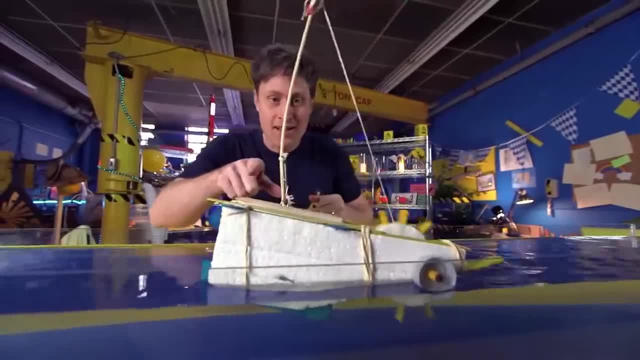 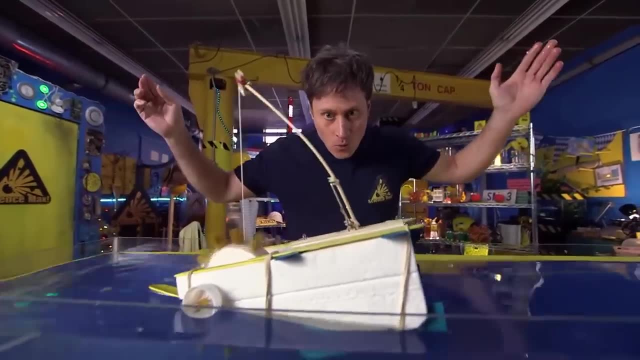 Paddle wheel turns because the mousetrap is transferring energy that we put in earlier And it goes all the way. We stored the energy in the tension of the spring. now that tension is pulling the mousetrap, the stick and the string Which turns the paddle wheel and makes the boat go. 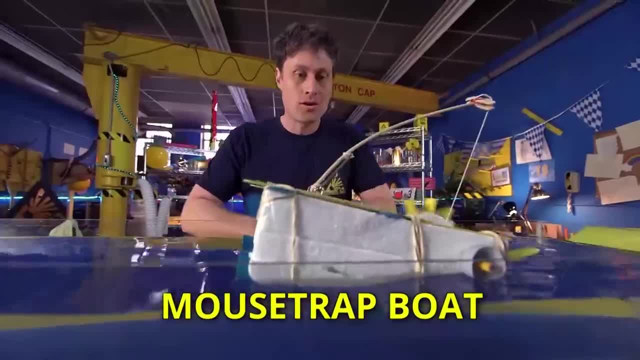 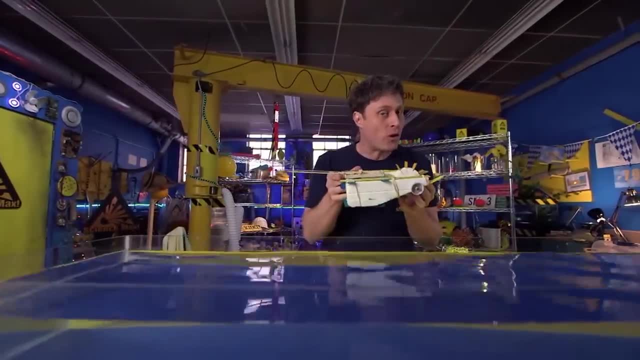 If you want more detailed instructions or other designs, look up mousetrap boat and there you have it, the mousetrap powered Paddlewheel boat, and this is what we're going to max out today. Come on, Greetings, science Maximites. My name is Phil and this is science max. 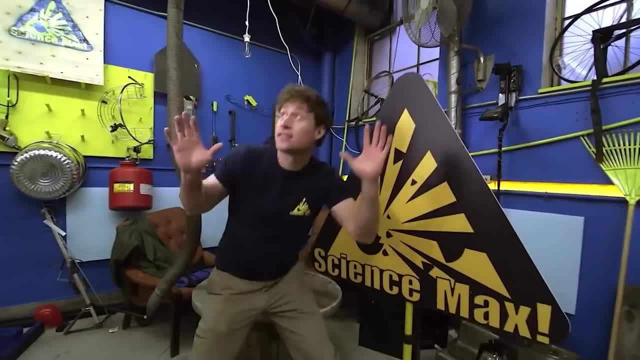 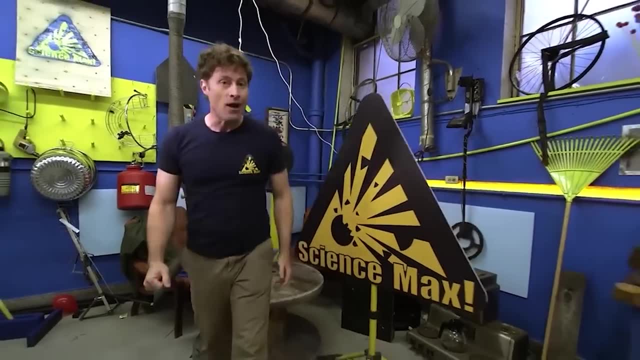 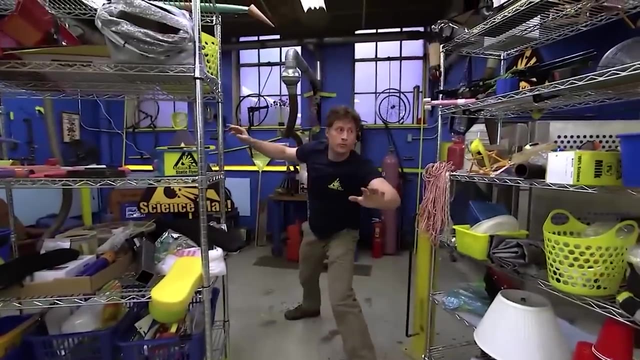 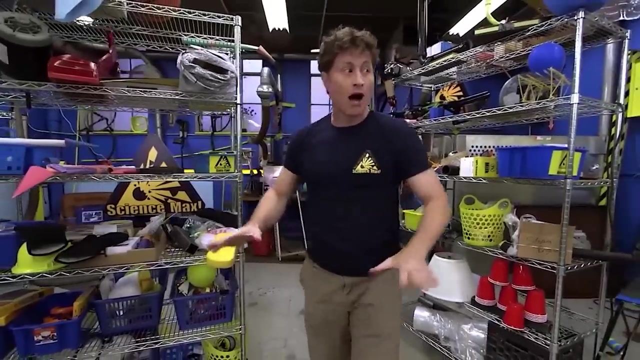 Experiments at large. today We're gonna be looking at earthquakes, Earthquakes, huh. today we're going to be looking at how to build something That was supposed to happen earlier. today we're gonna be looking at how to build something that stands up to the shaking of an earthquake. 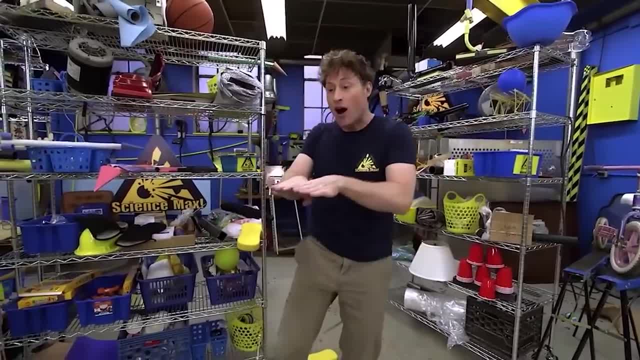 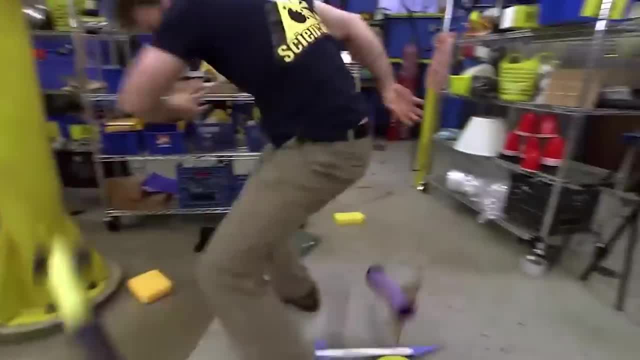 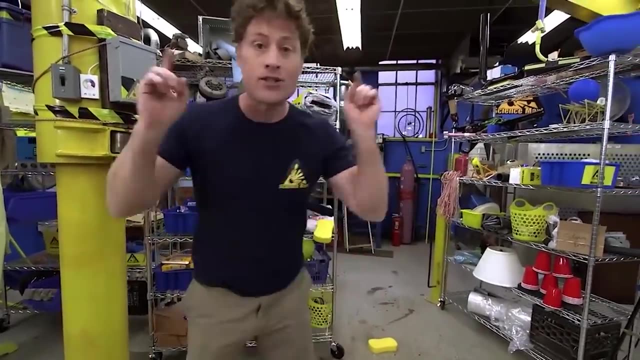 Hmm, earthquakes happen when two Plates on the Earth's surface rub together and it causes the ground to shake, Causes the ground to shake. sometimes it shakes a little, sometimes it shakes a lot. Chances are you do not live in a place that has earthquakes, But if you do ask an adult what to do during an earthquake so you can be safe. 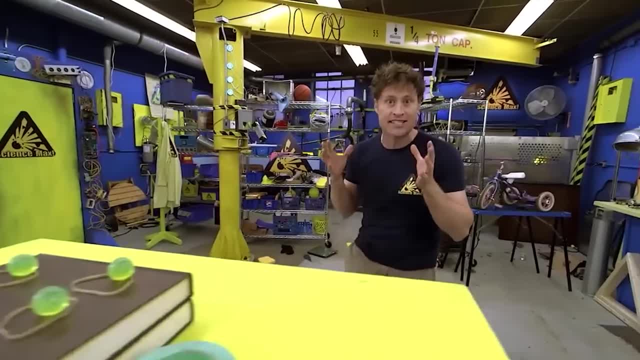 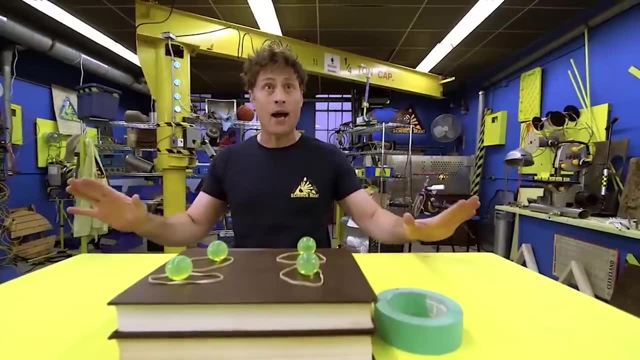 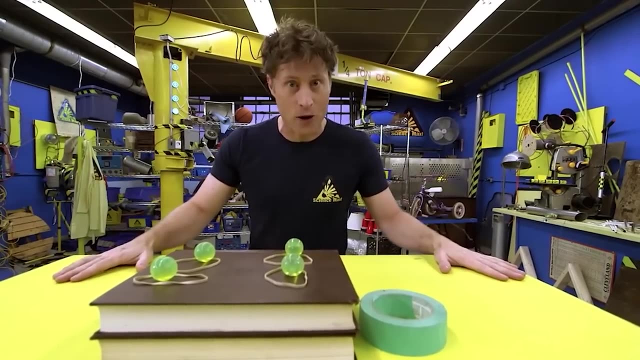 Modern buildings that are built in earthquake zones are designed to withstand the shaking, But how do scientists and engineers Build a building that stands up to the shaking of an earthquake? Well, that's what we're gonna be looking at today. first thing we have to do is simulate an earthquake. 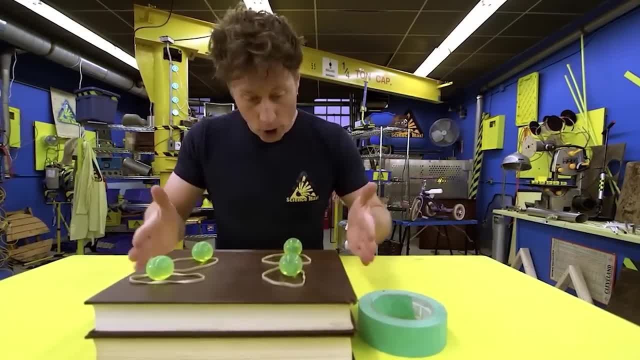 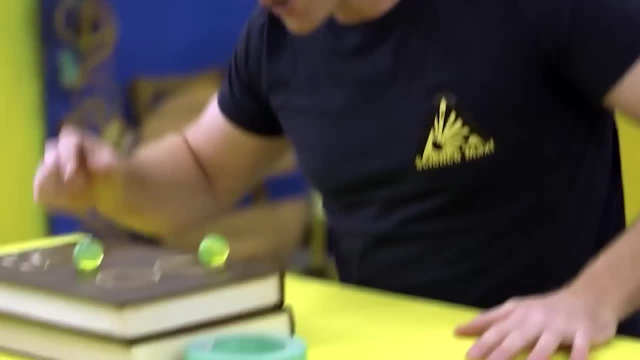 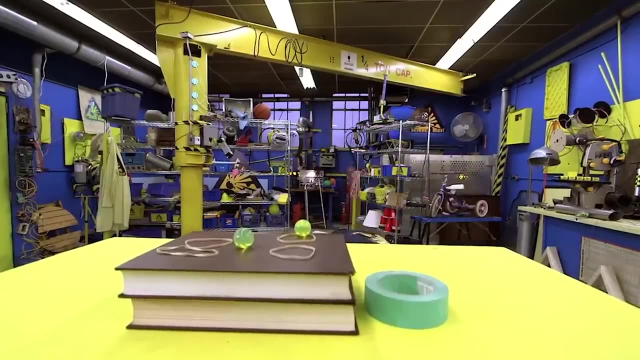 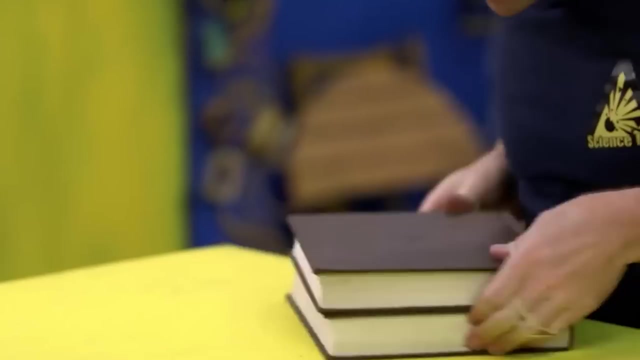 We're going to build a shaker table, and here's what you need: two books, Two books, four elastic bands and four, four rubber balls. Well, Okay, four rubber balls, all right. so the first thing you do is actually take your four elastic bands and 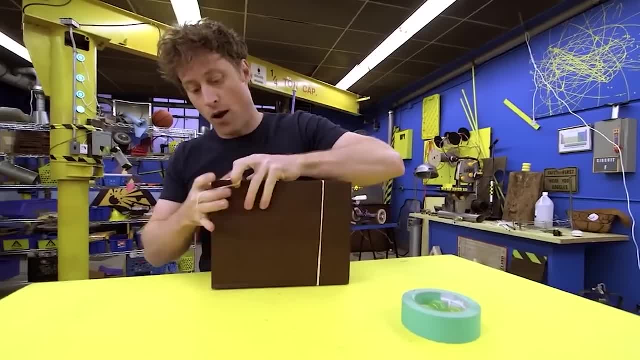 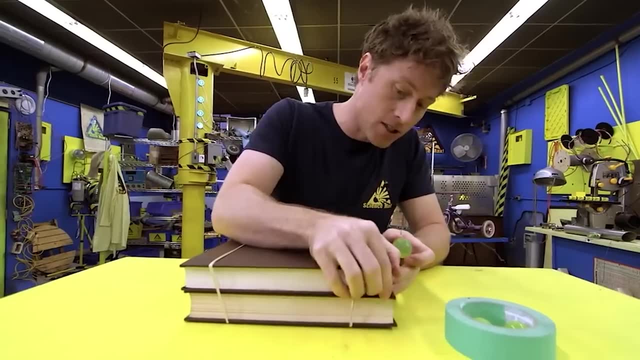 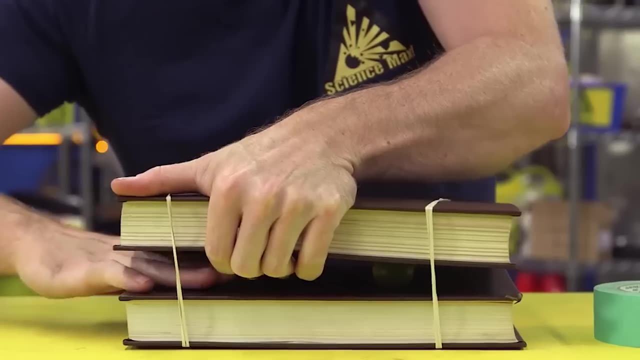 Wrap them around your books, put one set on one side, one set on the other side Till you have that, then you take your four balls and you stick them in between the books in the middle ish Area, but you don't want to have them too close to the edges. and now two at the back and tada. 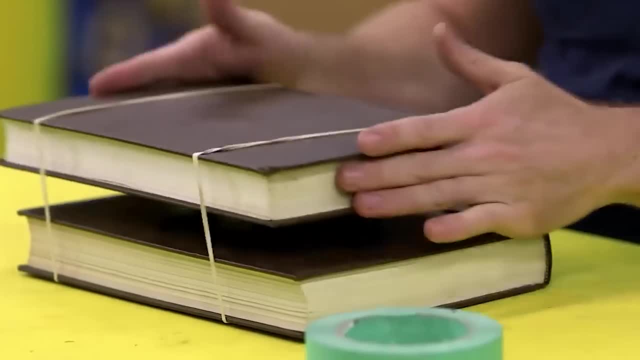 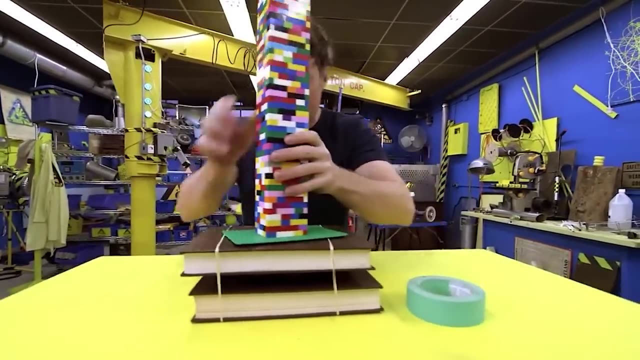 You've made your own shaker table. What are you shaking, you ask. I will show you. you build a tower- Well, like this one here- that I built out of building blocks. So here's what you do. You'll need your base to be securely attached to the shaker table. 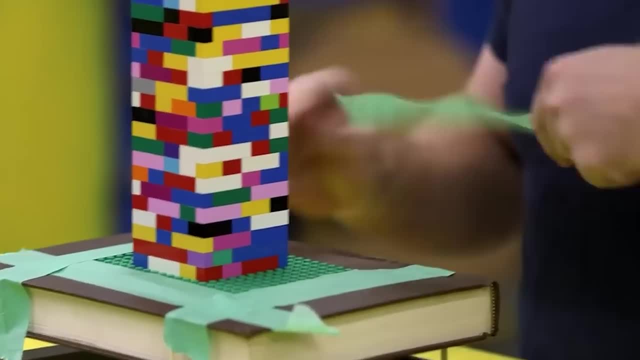 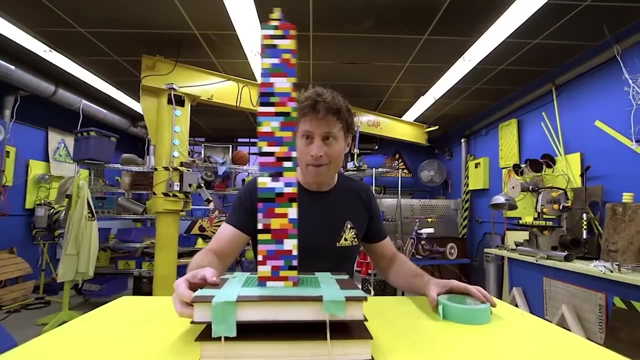 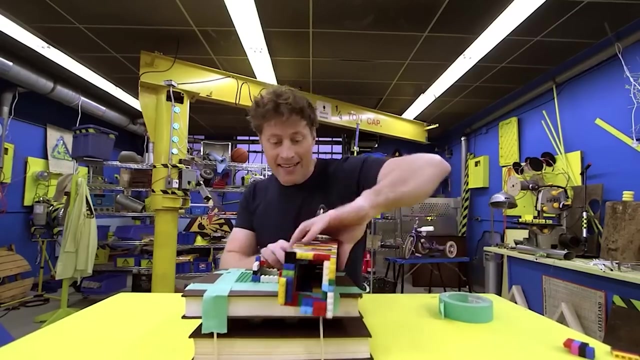 I use painters tape because it'll come off again without harming the books. And what I want to find out is just how much shaking this tower can take before it falls apart. ready, And there it goes. and when you've done that, What you do is you be a science maximite and you design another tower. 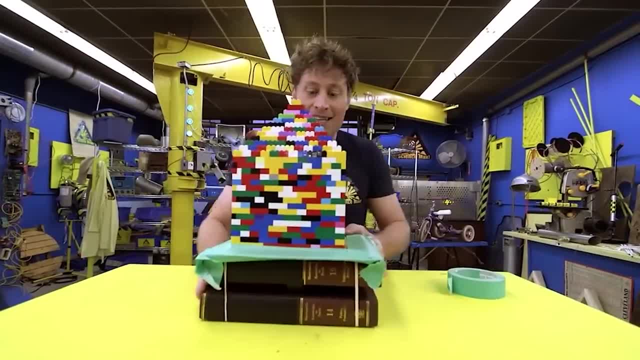 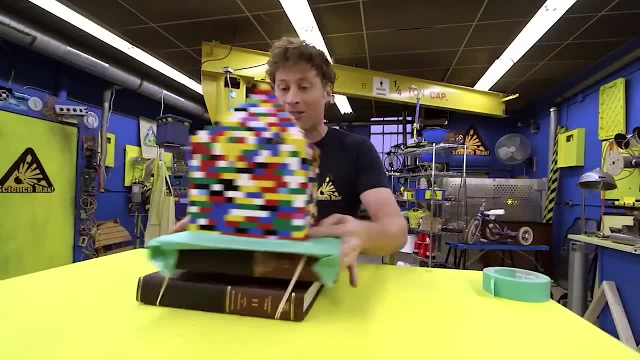 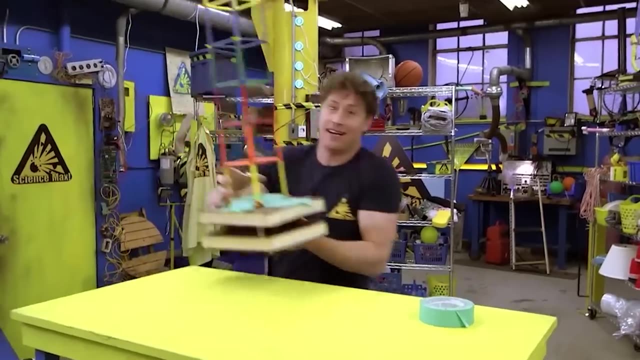 And you tape it down to your shaker table and see if you can make this tower Fall down in an earthquake and if you built it really well. But you don't have to just use building blocks. there's all kinds of other materials you can use. check out this building. 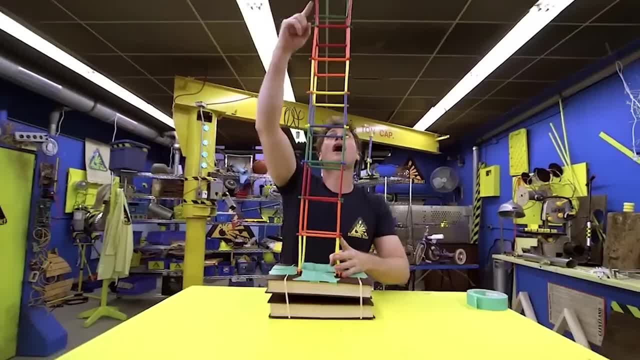 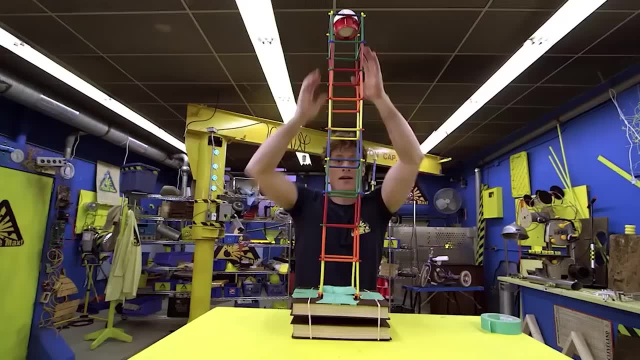 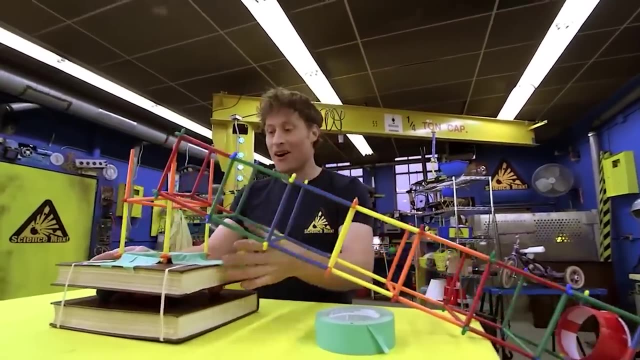 Which is really tall, and you'll see there's a cup at the top And that's for a baseball. Put it up at the top and that means there's a weight up there and then we shake it and we see what happens. There it goes. this is. 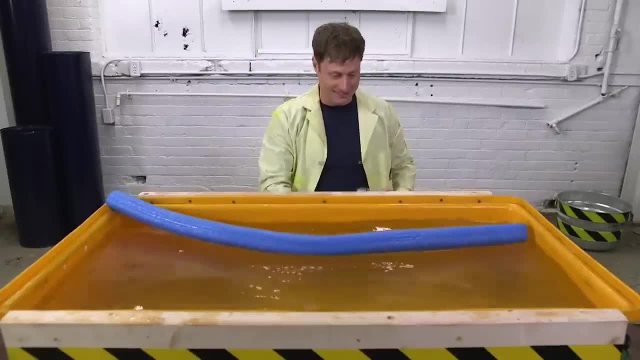 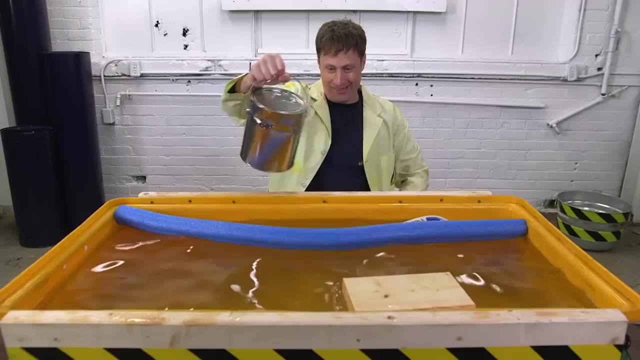 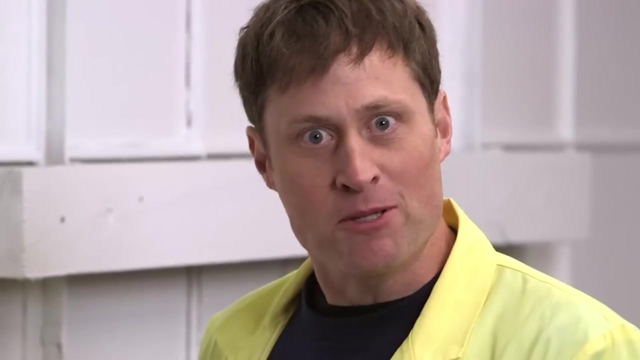 water. things float on water like pool noodles and wood and Toyboats. and now we're gonna do an experiment with how paint floats on water. How is it supposed to work? Oh, I'm supposed to take the paint out of the can first. This is a fun experiment you can do at home. 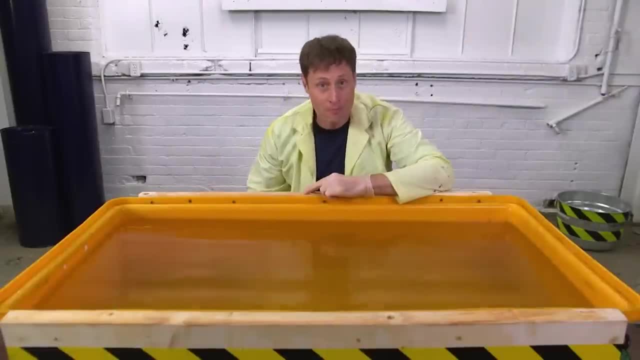 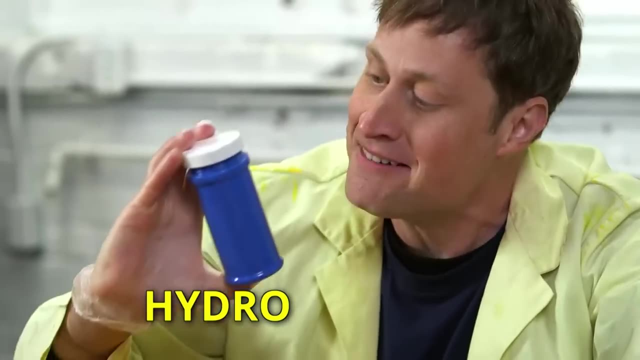 All you need is a container, some water and paint, But not just any paint. Special paint you use for hydro dipping. That's hydro meaning water and dipping meaning dipping. Carefully pour the paint on the water and add a few different colors. 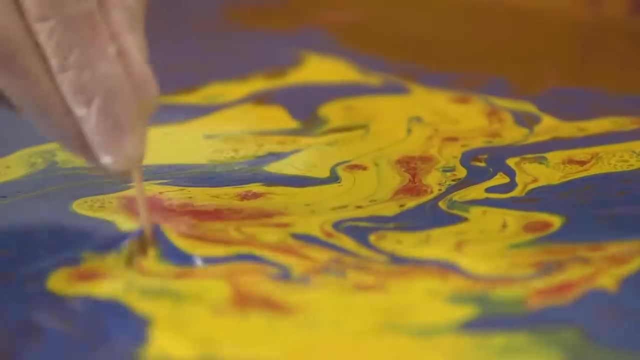 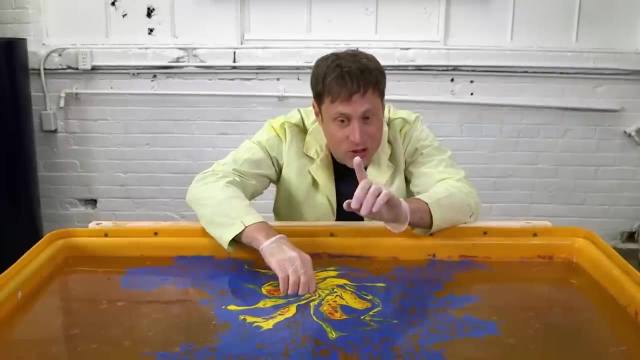 Then take a stick to swirl it up into a pattern. Then you get something you want to paint and you carefully put it in like so, But don't pull it out as soon as you get it in. You have to spread the paint away. 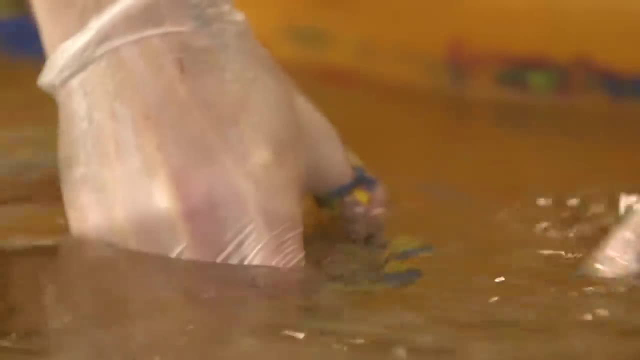 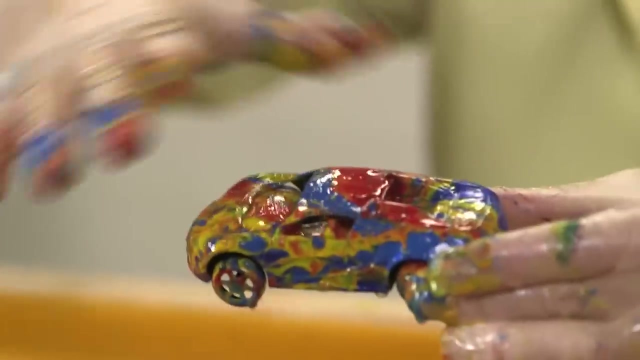 because it'll stick when you bring it back out. And then, when you pull it out, whoa, hydro dip. Let that dry and then you have a very cool painted toy. Let's do some other stuff. This is a bike helmet. 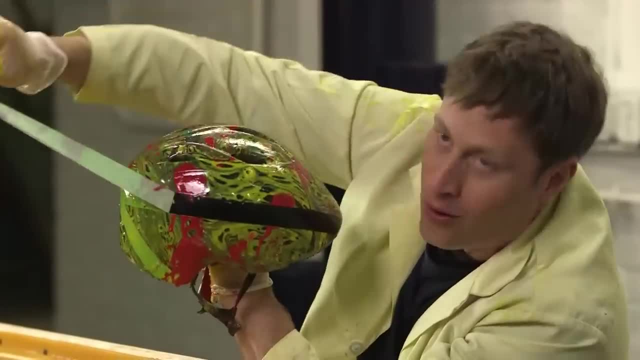 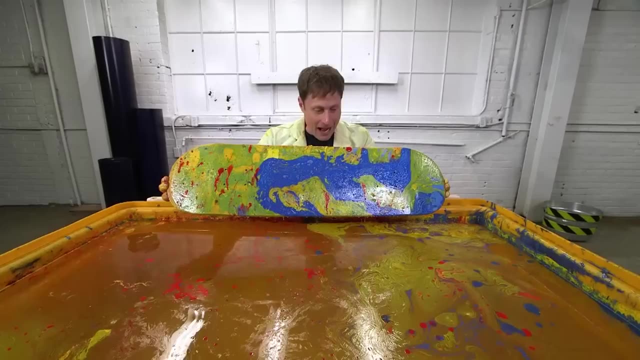 If you put tape on what you're painting, you can remove it later to make parts that aren't painted. Skateboard- Whoa. Oh, that's pretty cool. Now to max it out: Hydro dip pants. Wearing the pants when you do this is super messy. 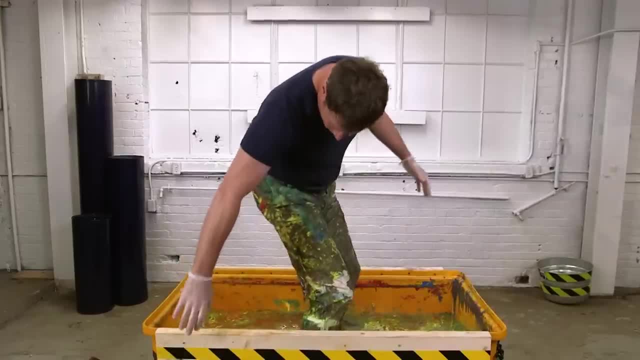 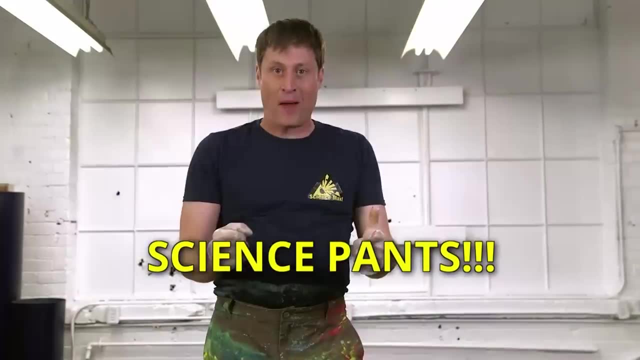 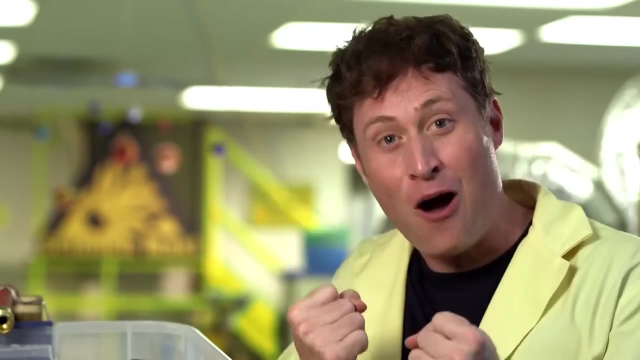 and not something you should try at home, But the results weren't bad. Science pants, Science pants, Science pants. One of the ways you can experience the power of water is watching it wash away dirt. You can do it, You can experiment with this yourself. 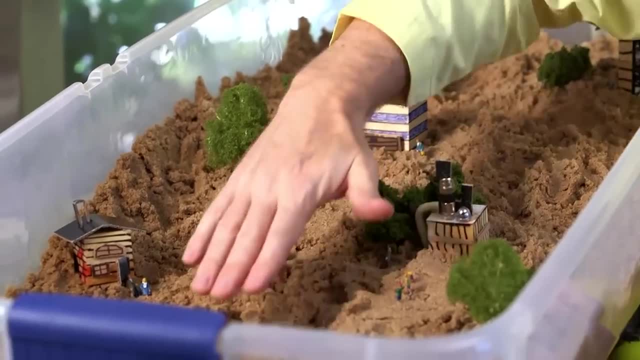 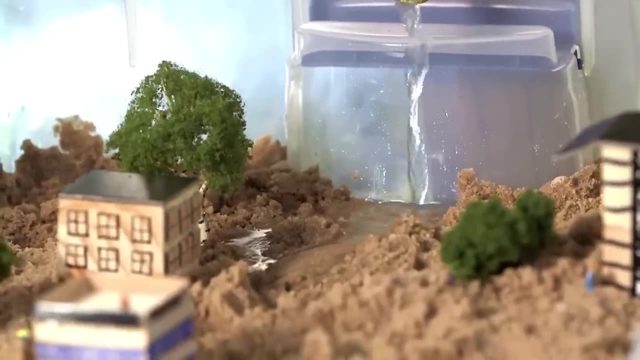 by making your own erosion table. To make your own, fill a plastic tub with sand and tilt it up. Cut a hole in the tub at the low end and put a hose with a trickle of water at the high end. Then, to complete your model, fill it with a little happy town. 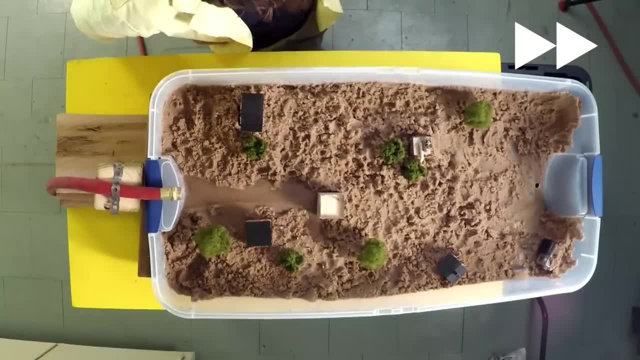 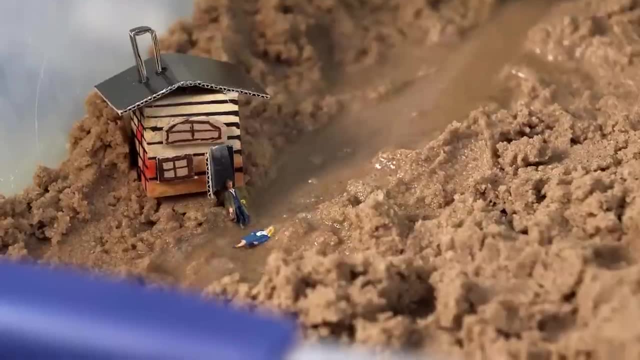 This small model shows how rivers cut their course to the ocean by following the lowest point. Try to design your town and the layout of the ground so the river goes around the buildings. I'll see you later. I'm going to take a look. 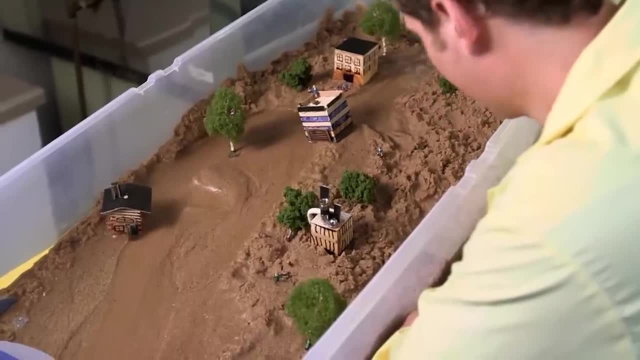 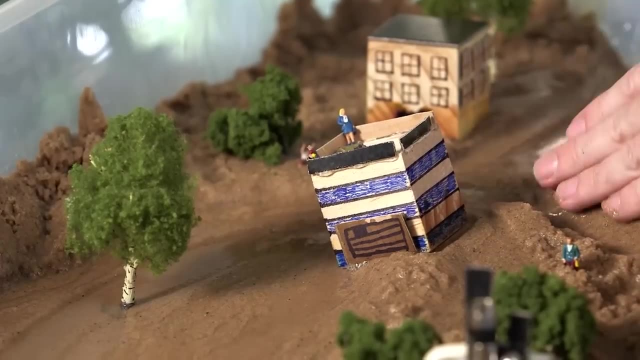 Swim in the river. now. There are lots of ways to experiment: Change the amount of water or the steepness of the angle. Look at the soil- it's all getting eroded over here. Or the way the town is laid out. Every time you do it, the river goes in a different direction. 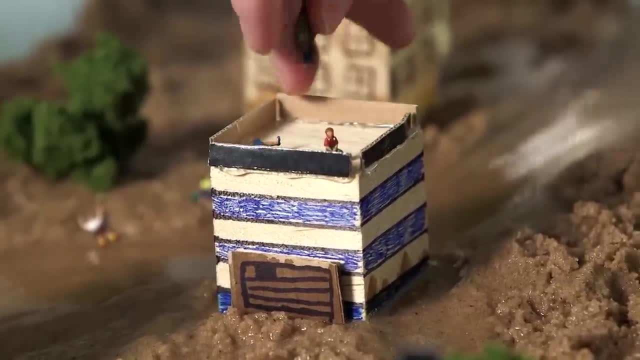 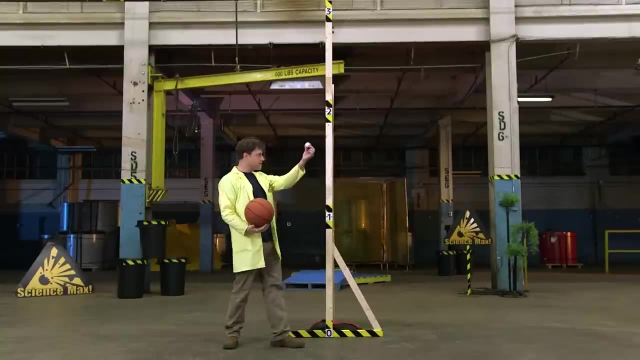 and have fun. Oh phew, I'm tired, I'm just going to lie down. And that is the power of water. This is a basketball: It bounces. This is a golf ball: It bounces, But it never bounces as high as where I dropped it. 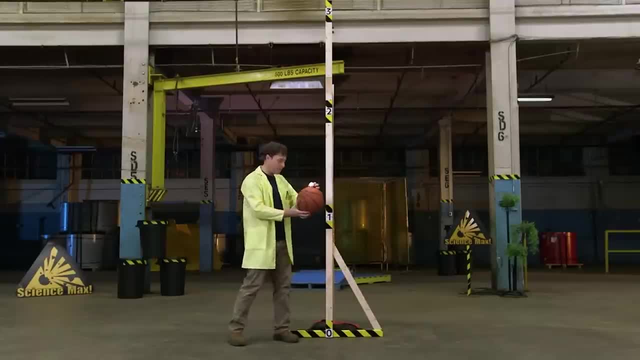 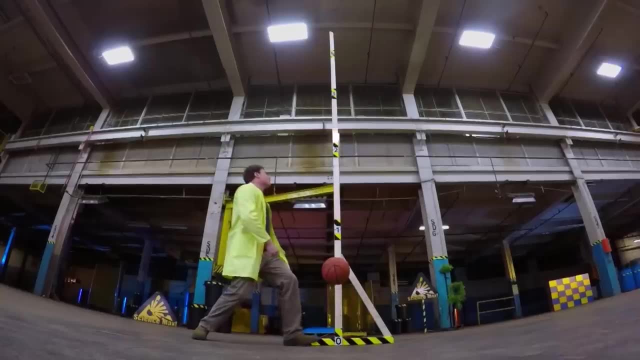 But watch as I put the golf ball on top of the basketball. Whoa, Why does the golf ball bounce higher than where I dropped it from? How is this possible? I only bounced the golf ball from one meter high. So what's going on? 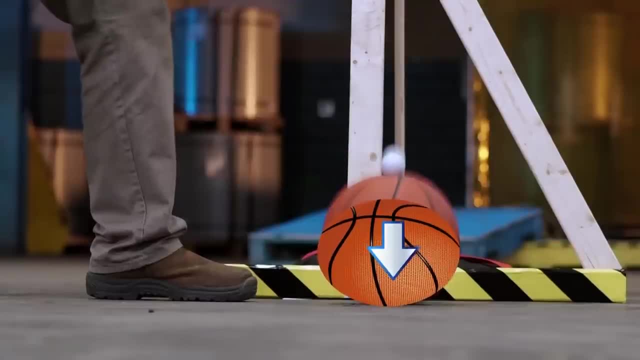 Well, as the basketball hits the ground, it compresses, storing the potential energy of its bounce, about to give that energy back as it bounces up again. But this energy works as a springboard for the golf ball. And since the golf ball has a lot less movement, 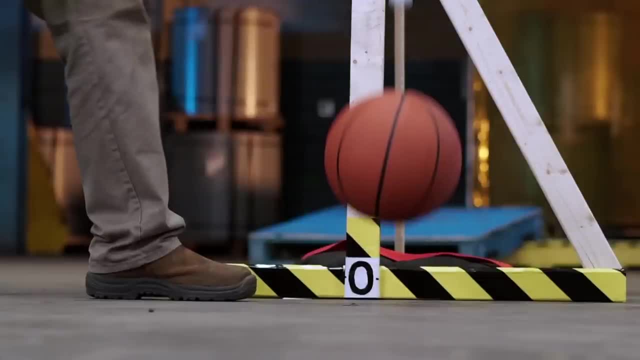 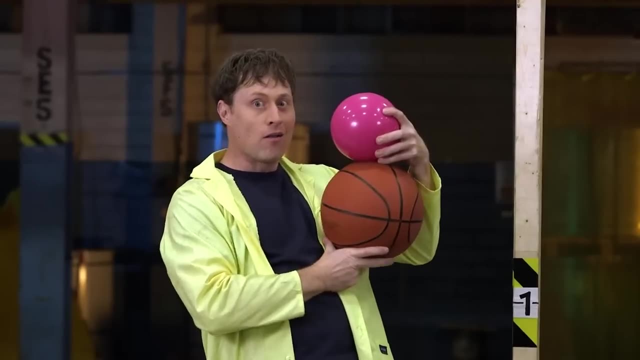 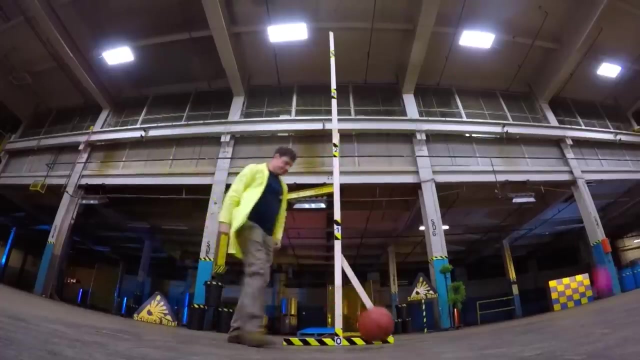 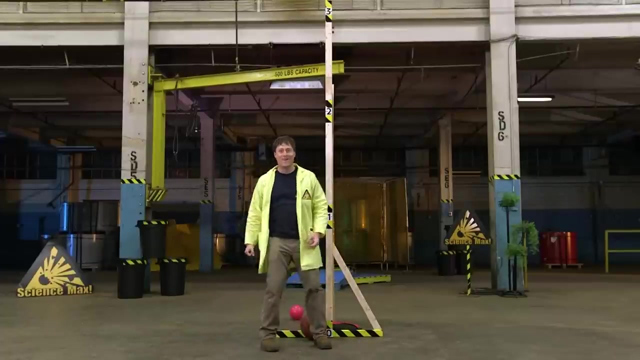 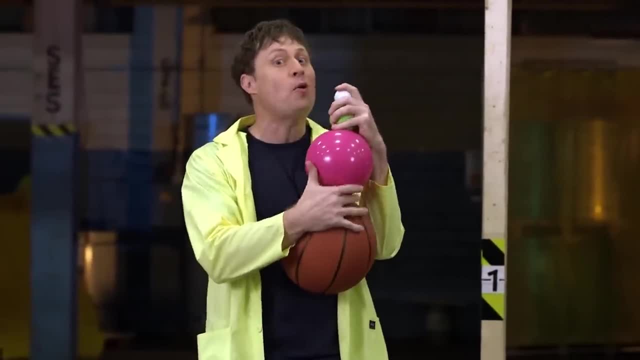 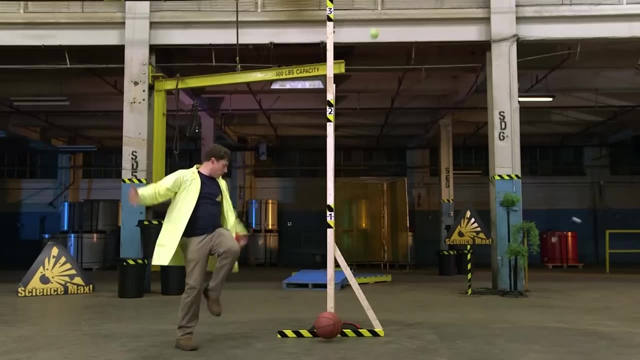 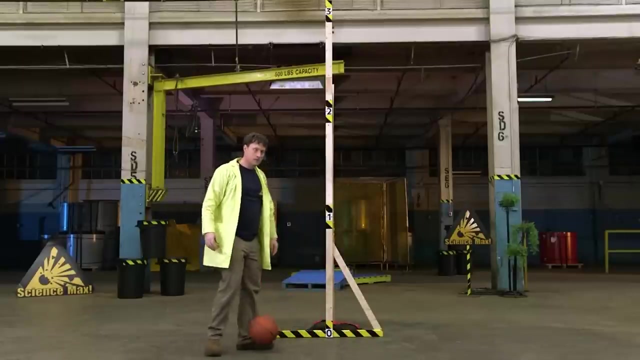 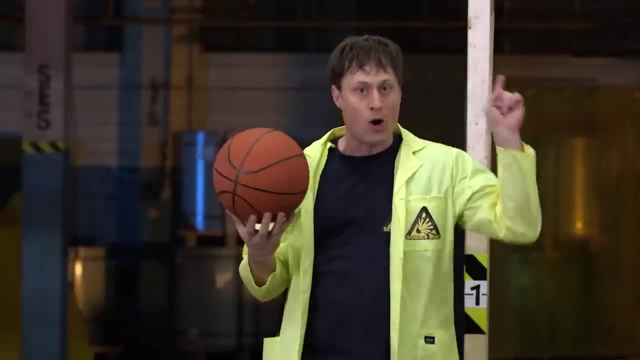 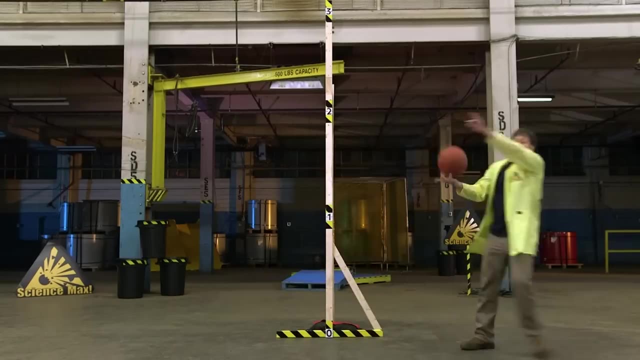 on top of each other is pretty difficult. So we know the mass of the ball is important. Why don't we max it out in a different way? This is a Swiss ball for exercising. It has a lot more mass than a golf ball. 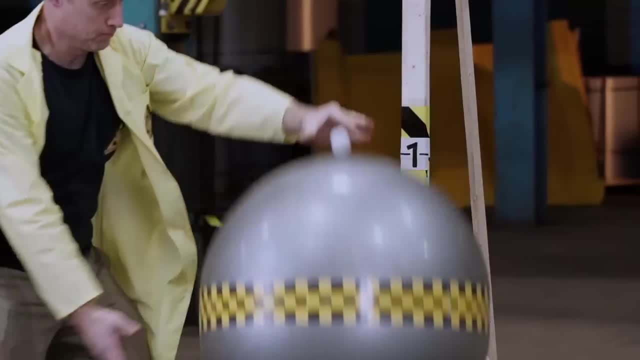 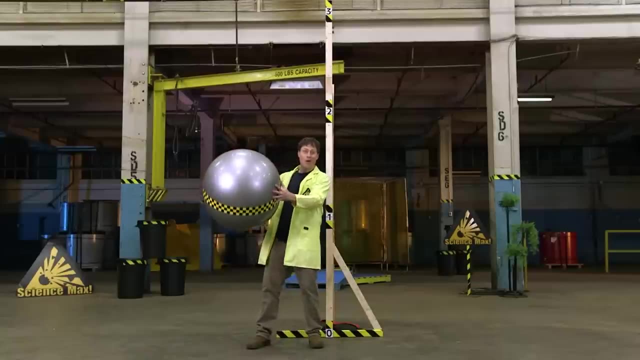 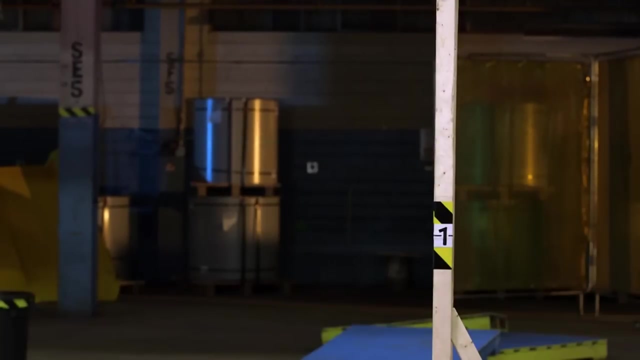 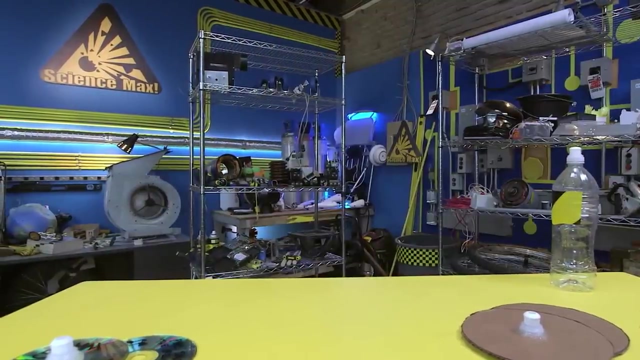 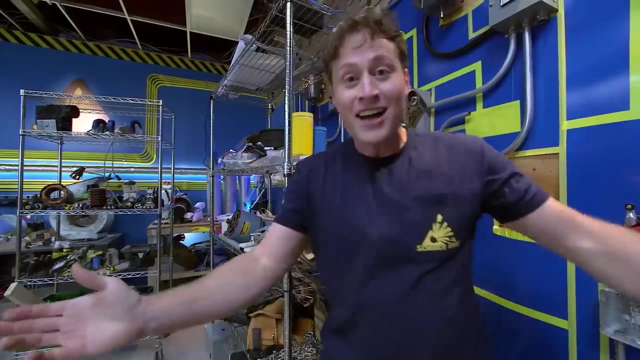 So let's try it out. There you go: The transfer of energy between balls. A great way to lose golf balls. Hey, Science Maximites I, I ah Ugh slippery, But that's okay, because today we're talking about friction. 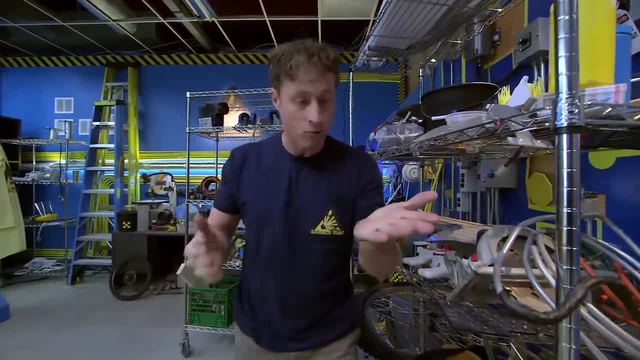 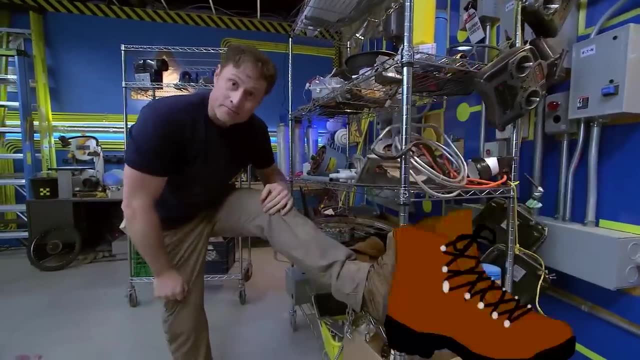 Friction is a force that is everywhere and happens when any one thing rubs against any other thing. We do lots of things to increase friction, like, uh, like, wear shoes with big treads on them, And we can do things to reduce friction. 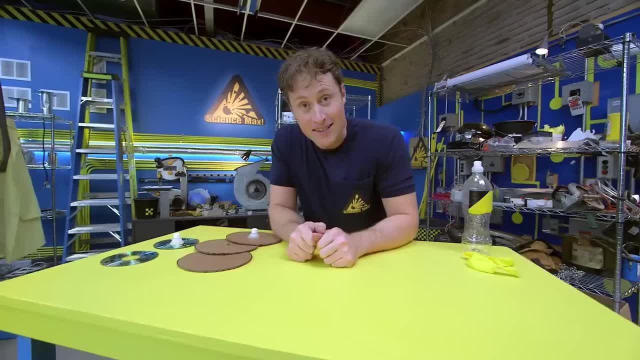 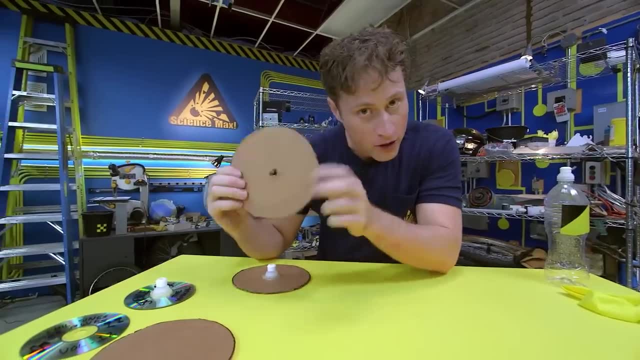 like the experiment we're doing today. We're going to build a hover disc and it's very easy. You take some cardboard and cut it into a circle, just like this, Then put a hole in the middle of the circle. You might want an adult to help you with that. 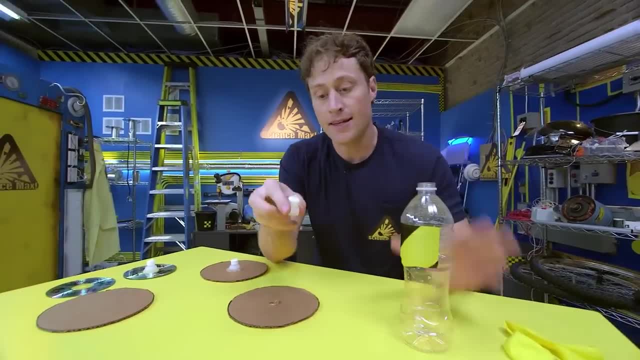 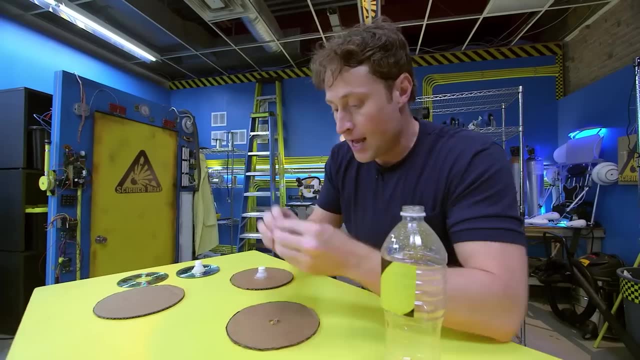 And then take a plastic drink bottle cap like this. I like to use the ones that you get on sport bottles, because they have a little nozzle that pops open or closed, And then you glue it around the circle and you get this. Then you need a balloon. 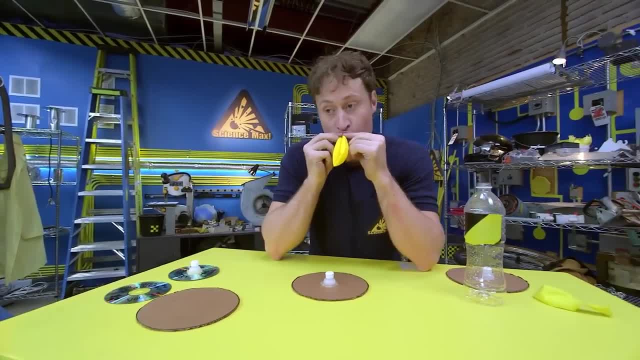 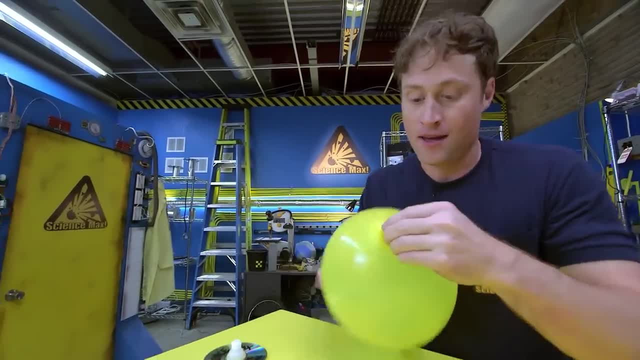 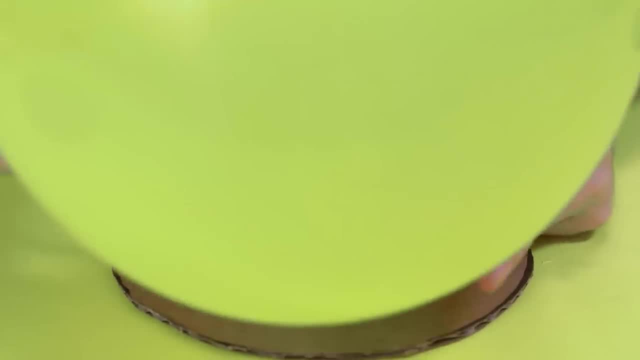 And then twist the balloon so it doesn't get away from you. When it's nice and twisted, you can stick it over the drink bottle cap like this and then untwist it, And this is why I like to use the plastic drink bottle caps. 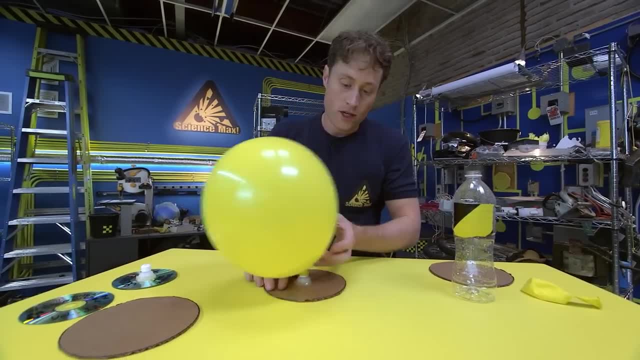 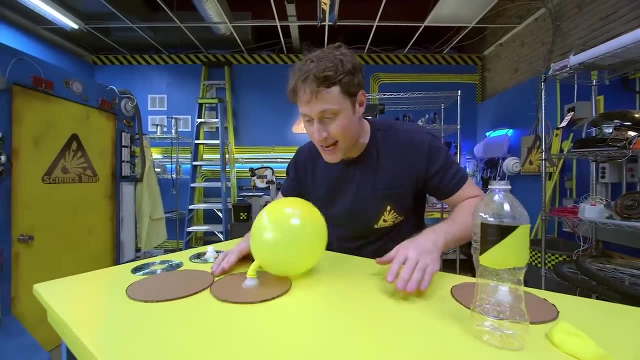 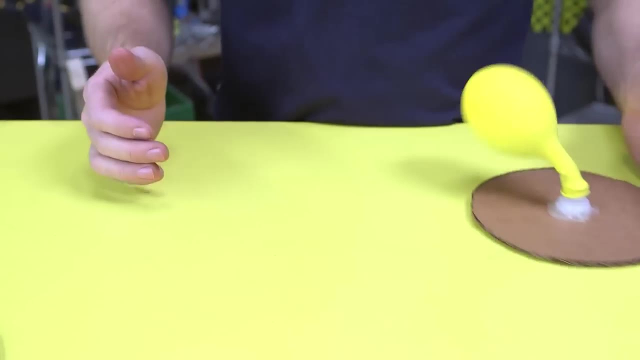 that come from sport bottles, because you can open it when you want And when you do your disc rides on a cushion of air, reducing the friction with which you lift the table and it's almost like it's sliding on ice. You can also use CDs if you want to do a different design. 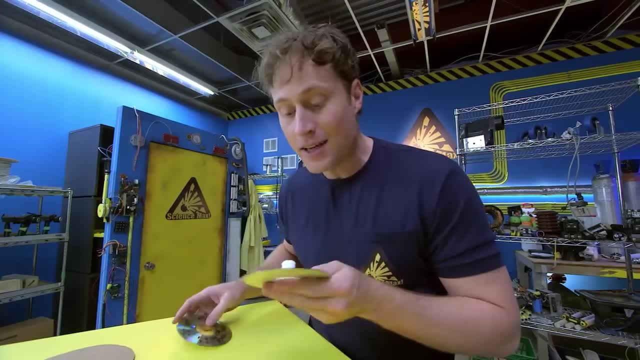 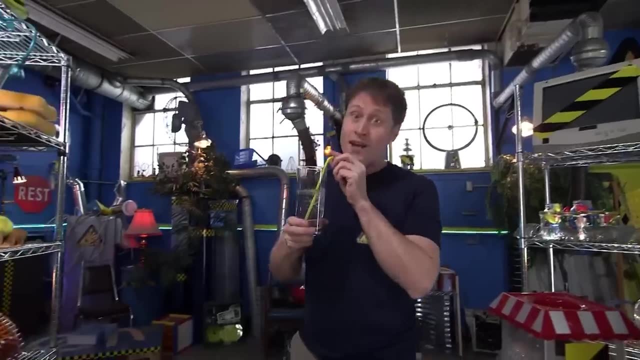 Just make sure you're using CDs you never want to listen to again. Now, if any of this is too fast, don't worry. You can always go to the Science Max website, where we have all of the instructions. Greetings, Science Maximites. 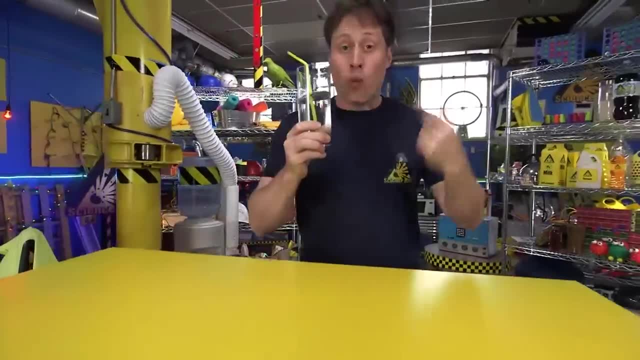 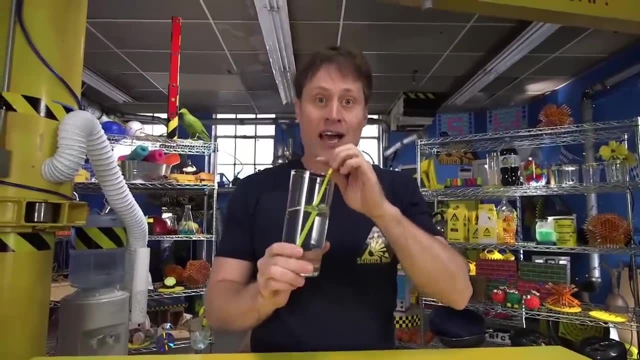 Today we're using fizzy drinks in our experiments, And a fizzy drink is just water with bubbles of carbon dioxide gas dissolved in it. So I thought, since we exhale carbon dioxide, I could make a fizzy drink by just blowing bubbles. 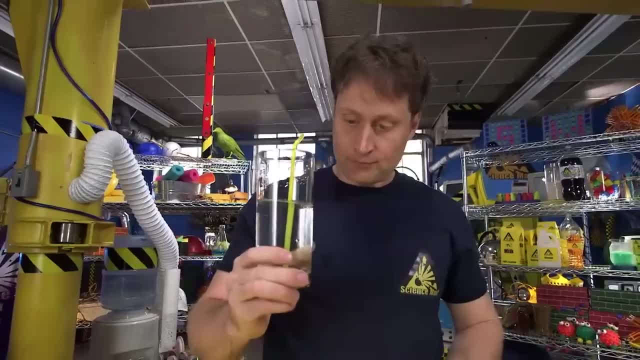 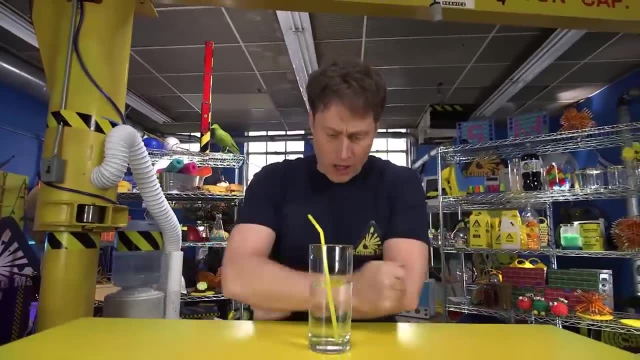 in this water Doesn't seem to be working, though, does it? I don't see any bubbles, Do you No? Hmm, Water does absorb carbon dioxide gas, but I don't have a fizzy drink. Weird Time to check the book of science. 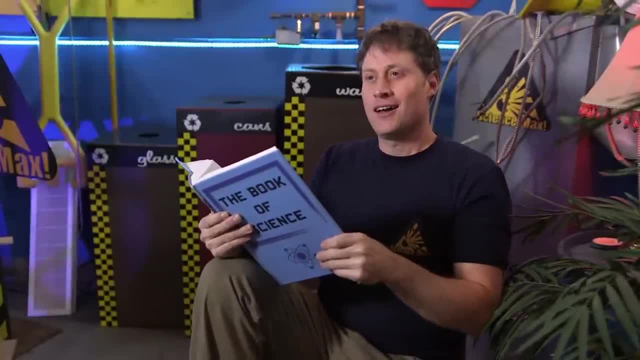 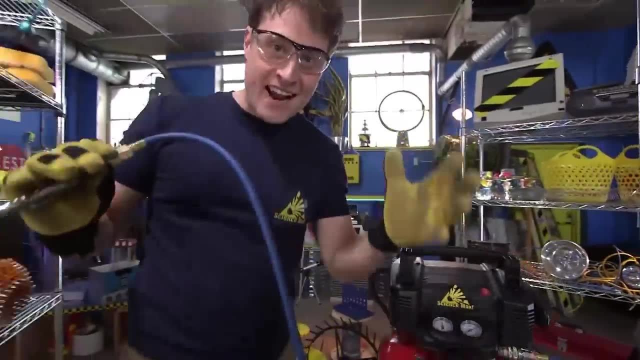 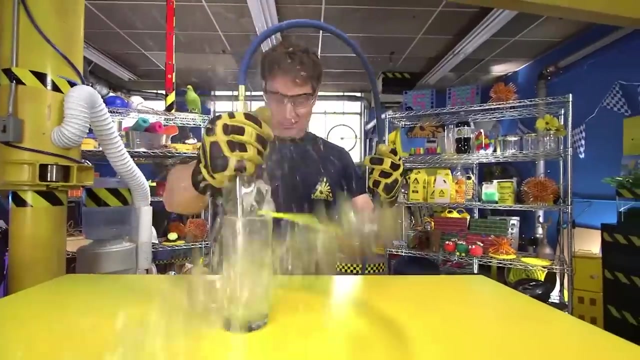 Oh, in order to make bubbles, you have to have pressure. So This is an air compressor. It takes air and compresses, it puts it under pressure. So, Hmm, The container needs to be pressurized. OK, When you get a container of a fizzy drink. 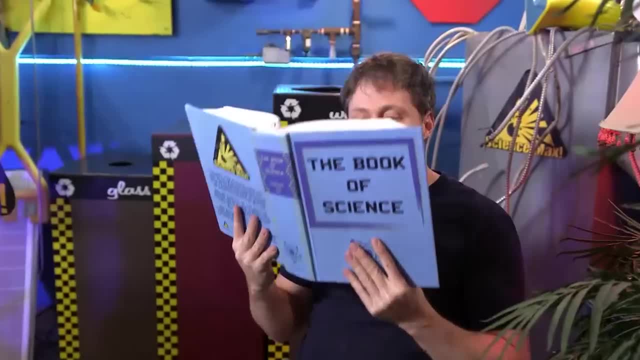 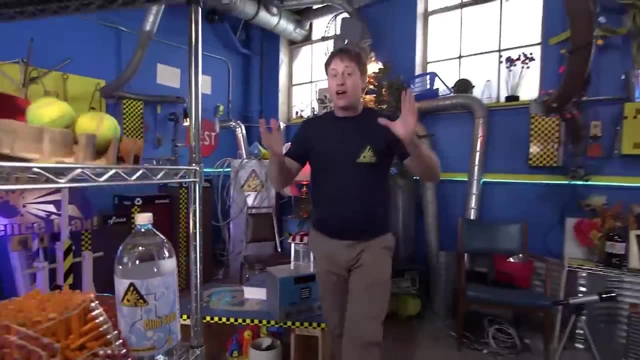 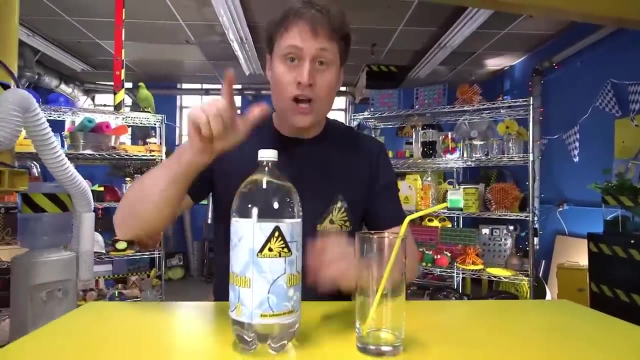 the carbon dioxide gas is put in there under pressure And it's so easy to get a fizzy drink out of it. It's a very simple process. It's a very simple process, but it's very easy to do, OK, And it stays in there under pressure until you release it. 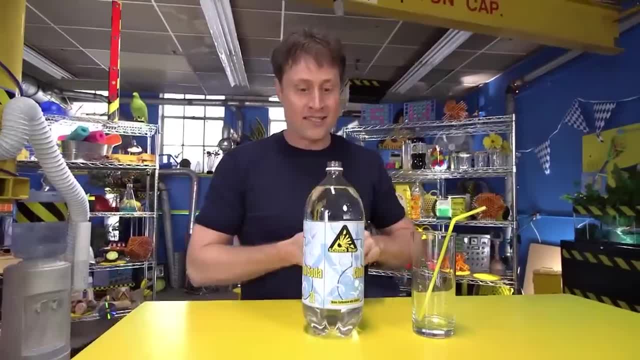 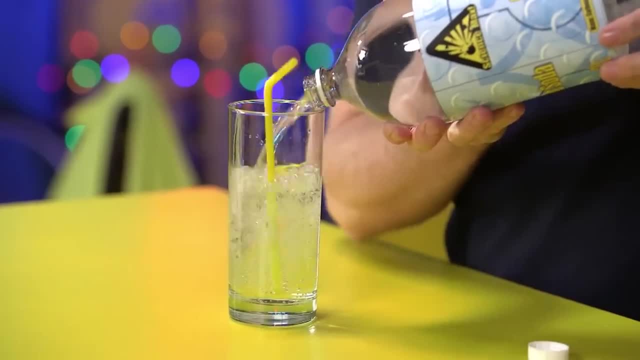 That's the sound of the pressure being released, And when it is released, the carbon dioxide gas starts to expand, And when it expands, it creates bubbles, And that's what makes your fizzy drink. This process takes a while to run out. 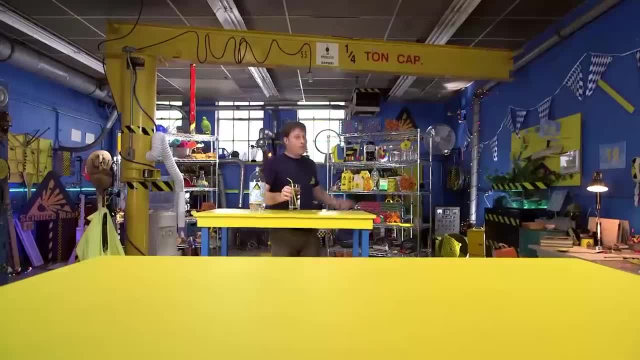 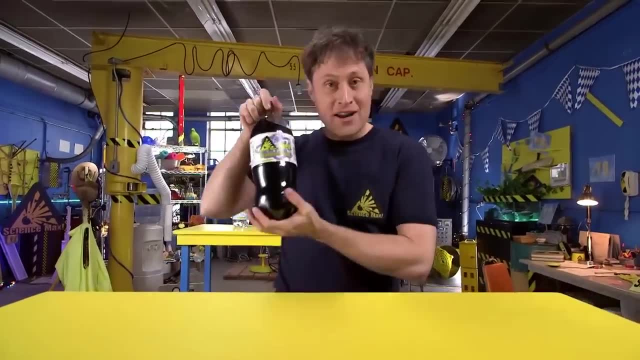 but eventually it will become flat. No more bubbles. But what if there was a way to release all of that carbonation all in one go? Well, there is, And for this experiment, all you need is your favorite brand of fizzy drink. 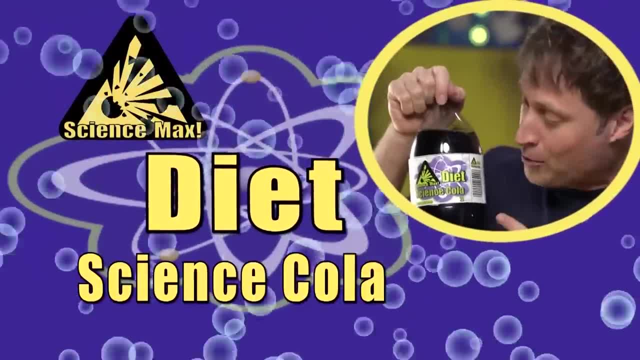 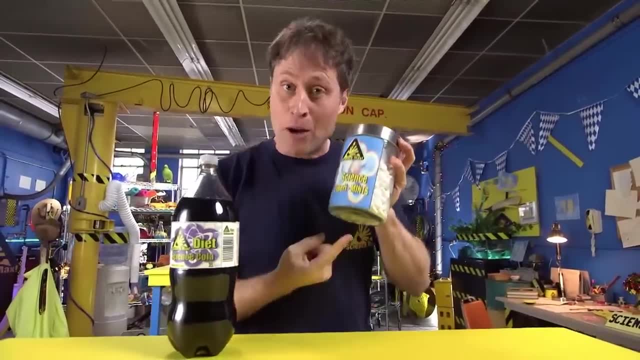 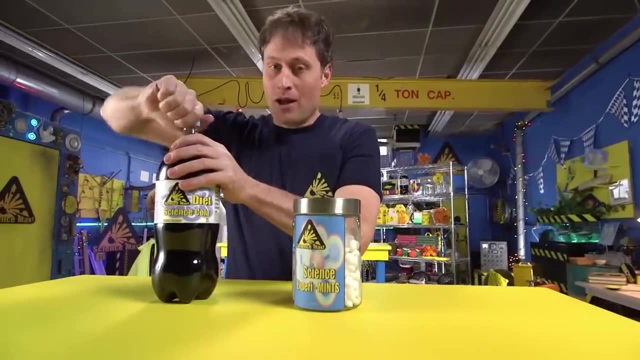 Science Max brand Diet Science Cola, 100% science, zero calories. And your favorite candy, like these science experiment mints- All the minty flavor that comes from pure science. So all you need to do is open this up. open this up. 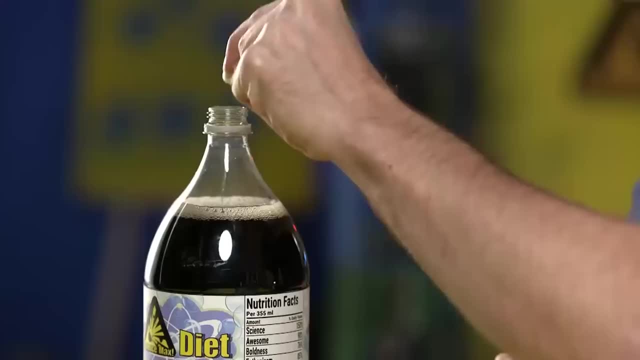 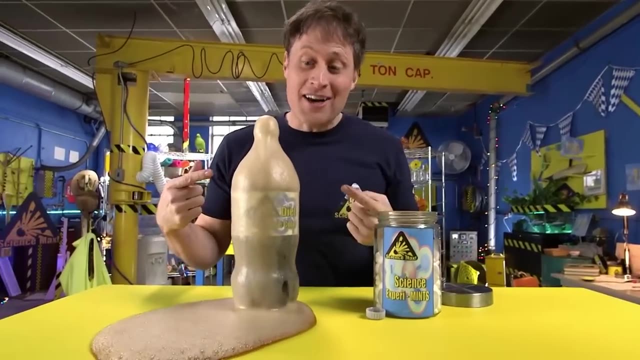 take one of these and put it in here with an adult's permission, because it can get kind of messy. What's going on here is all of the carbonation that was in the bottle is now being released much more rapidly than it would have been before. 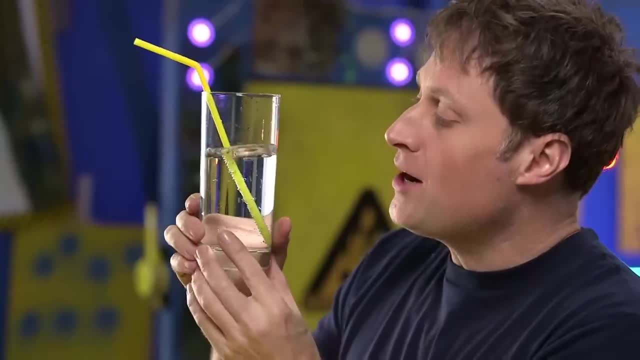 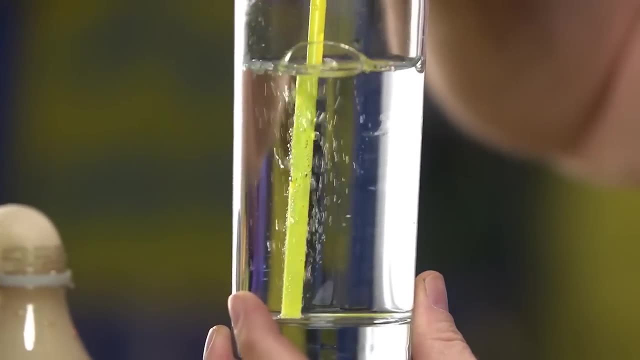 Now, why does this happen? Well, if you look at a carbonated beverage, you'll see that the bubbles don't come from everywhere. They come from the inside of the glass or, in this case, a lot are coming from the straw. 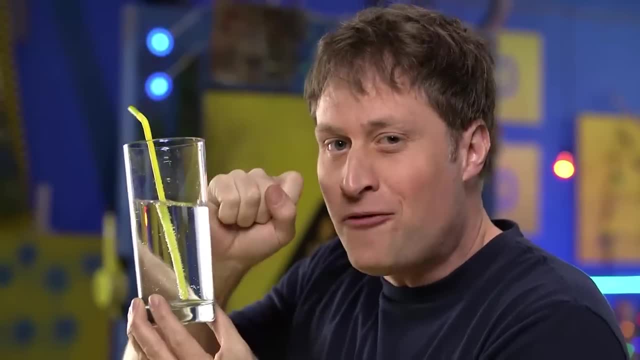 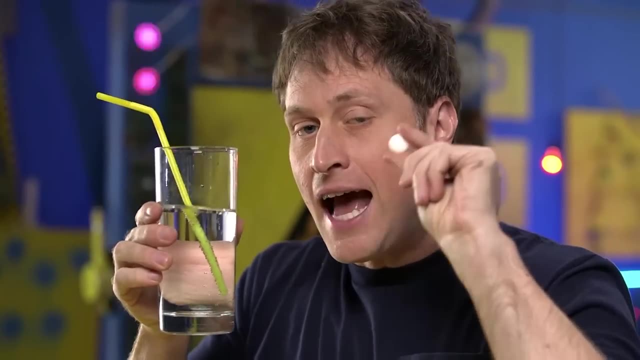 And that's because the carbon dioxide bubbles like to find a little imperfection, something to hold onto in order to expand and bubble out, And a candy such as this has a ton of little, tiny, microscopic imperfections, So when you drop it in, there's a lot more places. 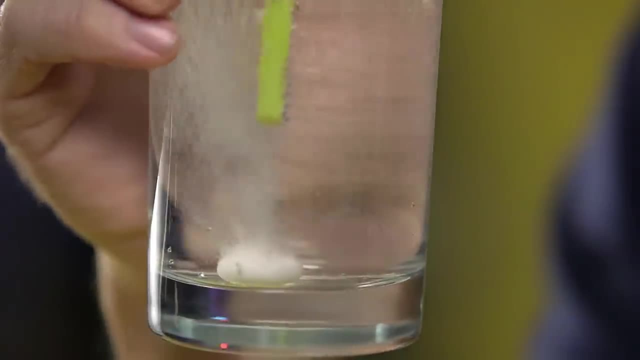 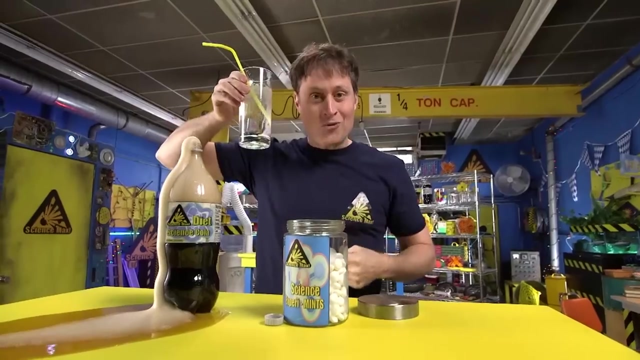 for the bubbles to attach and that makes the carbonation happen a lot quicker. But remember, this is not a chemical reaction. It all has to do with carbonation. So that's what we're going to be looking at today: Air pressure, more pressure, less pressure. 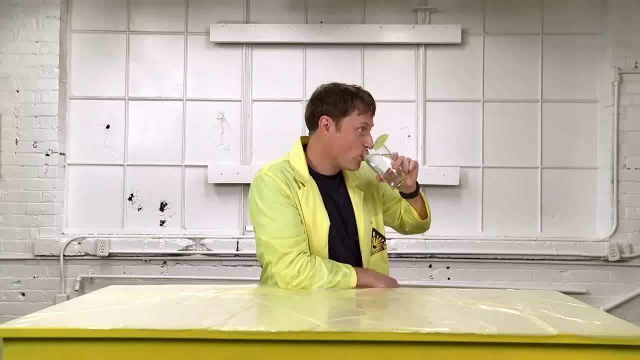 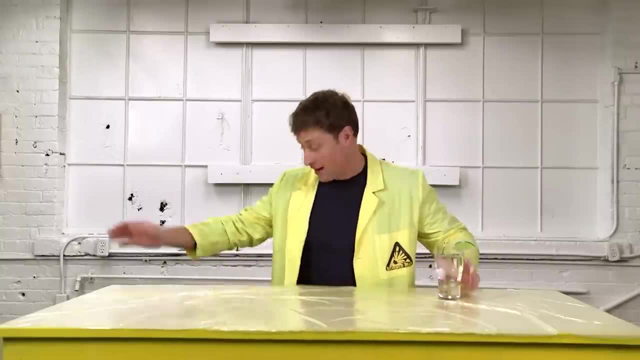 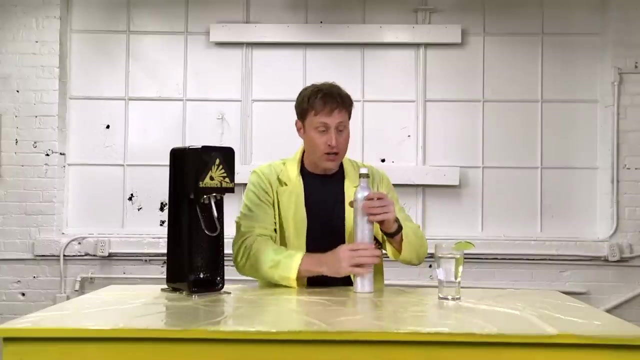 and of course, we're going to be maxing out this experiment. Nothing like a fizzy glass. And now there are ways for you to carbonate water at home. with something like this, the ScienceMax carbonation station, You have a bottle of compressed carbon dioxide gas. 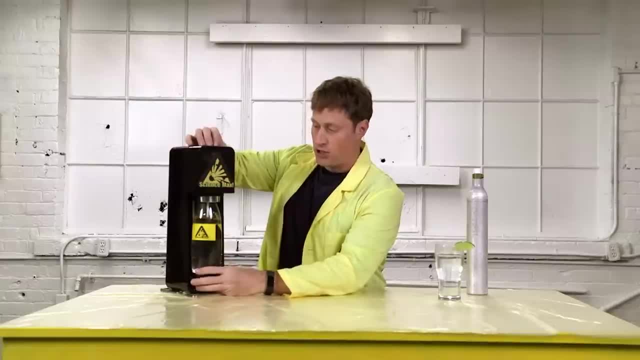 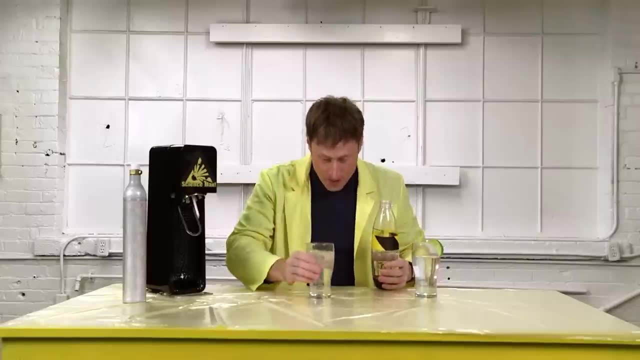 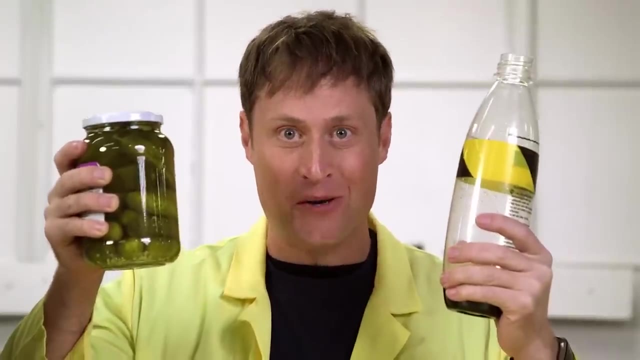 that's hooked up. You take a bottle of tap water, attach it and carbonate it. Voila, Carbonated water. But this is ScienceMax. Why just carbonate water? Let's carbonate everything. Let's carbonate pickle juice, Let's dampen it up. 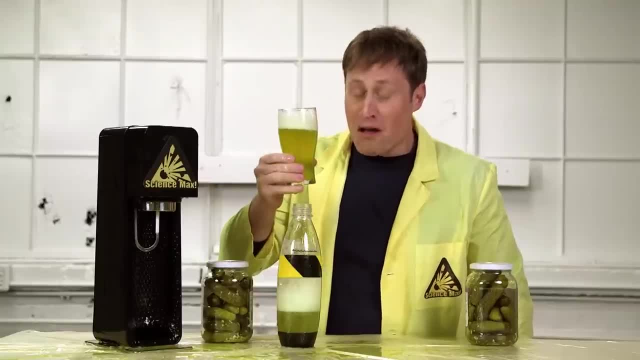 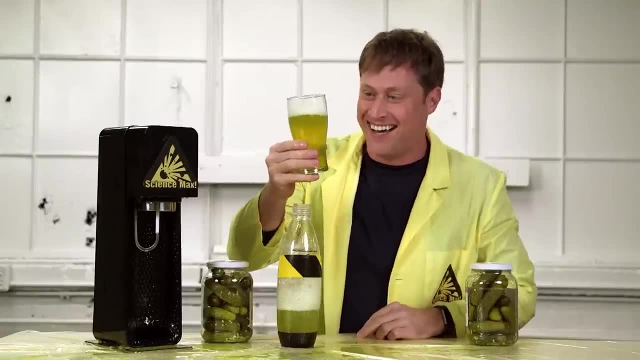 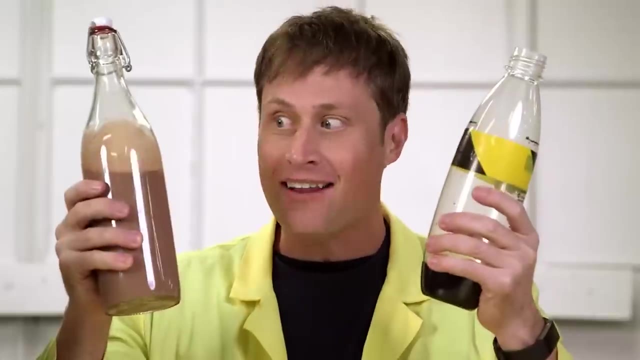 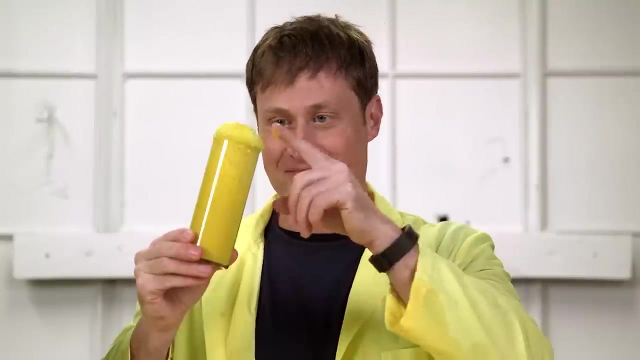 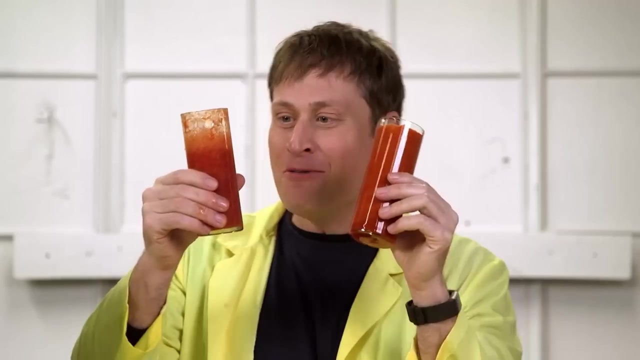 Ah, It's actually amazing Milk- It's like milk meets water, kind of very odd Chocolate milk. Oh no, that's way better. Carbonated mustard: Oh Mmm, Mmm, Mmm. Carbonated tomato juice, carbonated hot sauce. 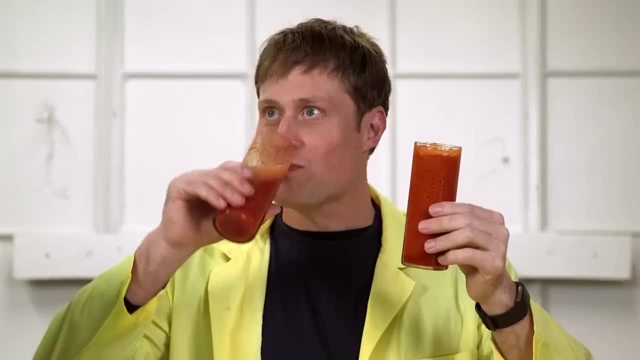 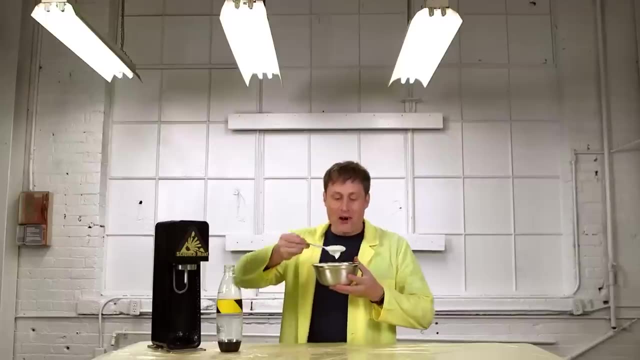 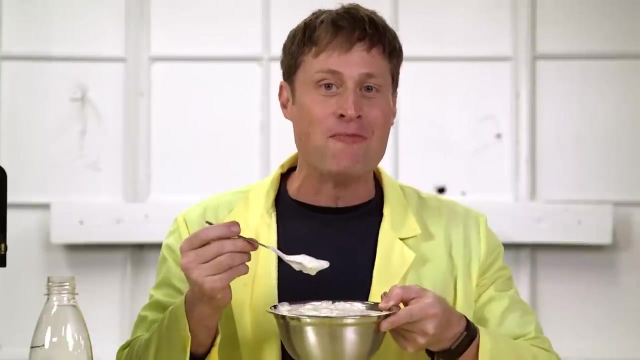 No wait, carbonated, that was the hot sauce. No, Carbonated clam chowder. Oh, there you go. carbonation not just for water anymore, And it's definitely not for clam chowder. No, that's just a big bowl of no. 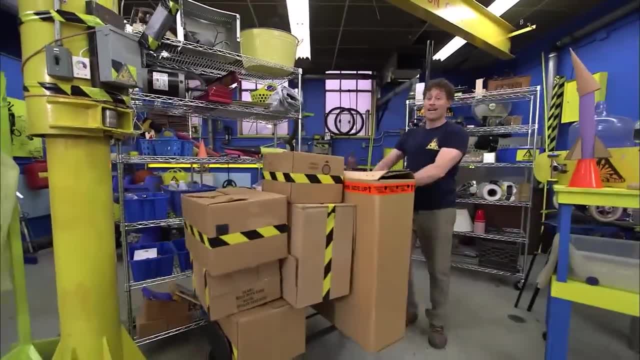 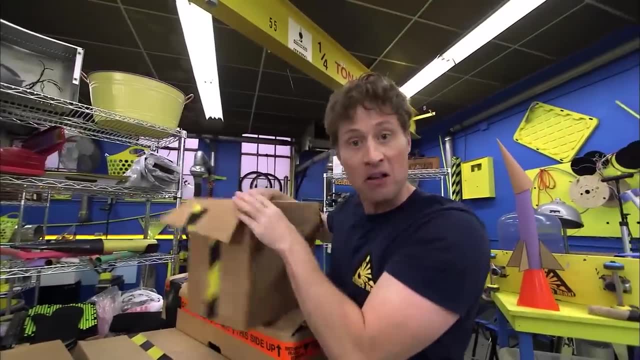 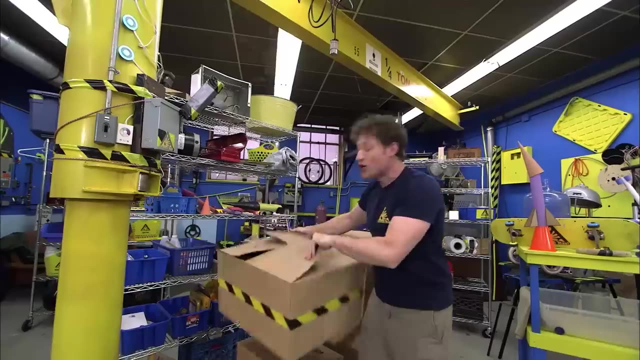 Never again. Greetings, Science Maximites. My name is Phil and it's moving day today on Science Max: Experiments At Large. Let's see where do I put this? This is probably a good spot. Today we are moving air. 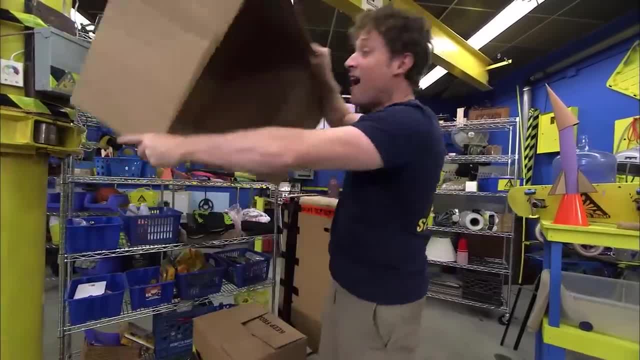 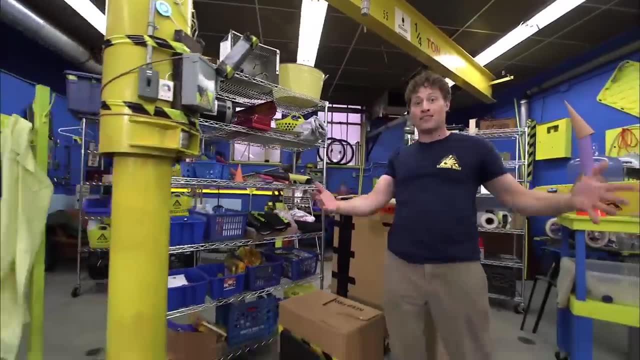 You probably don't think that moving air will have a huge effect, but you'd be surprised what you can do by just moving air. But don't worry, we're not just gonna move the air around in boxes, We are going to be moving air. 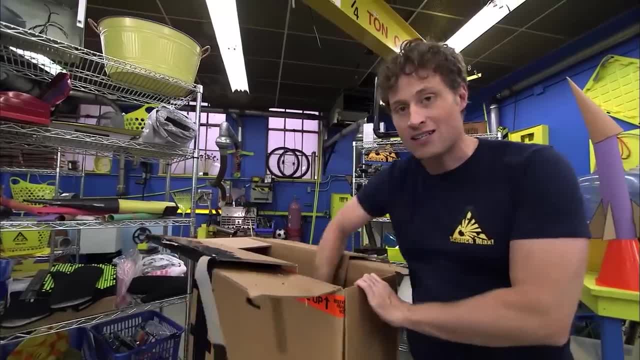 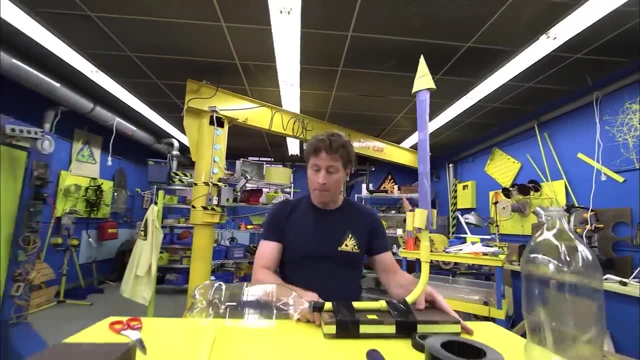 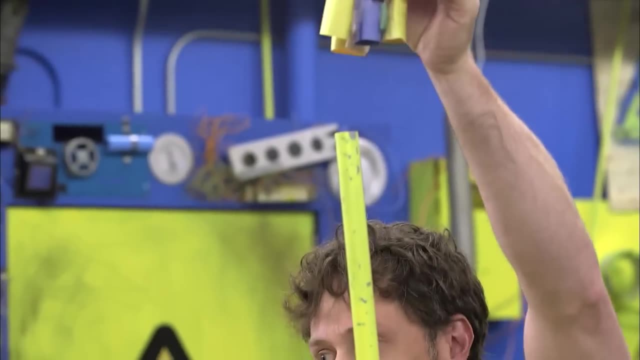 and build a rocket, And this rocket uses the science of stomping on something with your foot. This is a stomp rocket and it works by stomping on this plastic bottle and air shoots through this tube and pushes the rocket up into the sky. 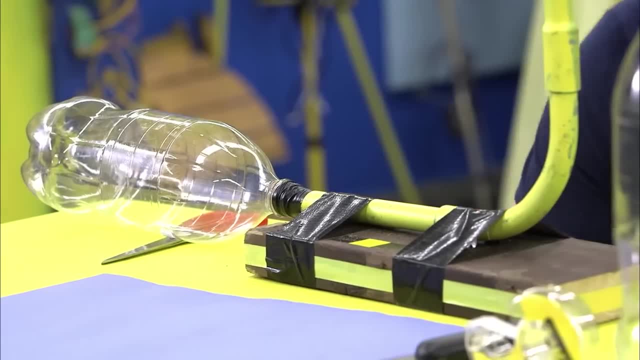 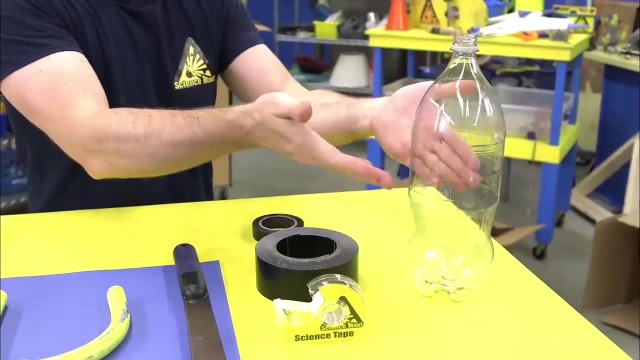 And here is how you can build one of your very own. And remember, if I go too fast, don't worry. All of the steps are on the website, so you can follow along at your own speed. All you need is a tube and you're good to go. 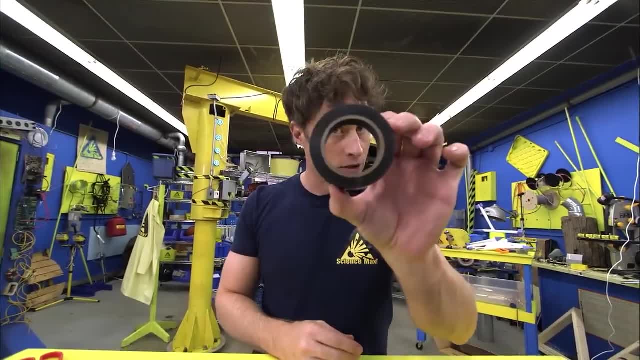 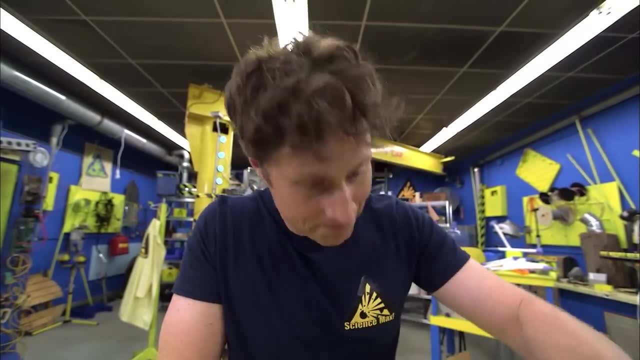 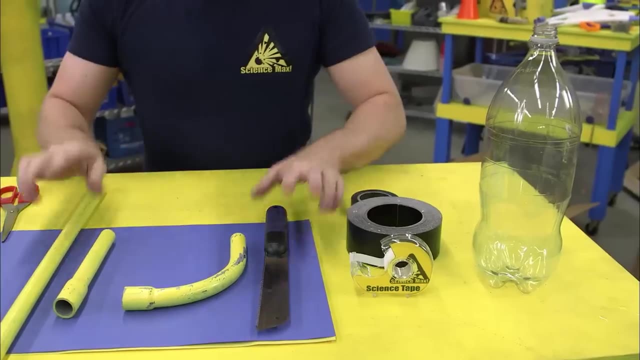 Two-liter plastic bottle. three kinds of tape: electrical tape, duct tape and science tape. Science tape is just the same as invisible tape, but I use this kind of tape for science. Then you want some plumber's tubing and some construction paper to make your actual rocket. 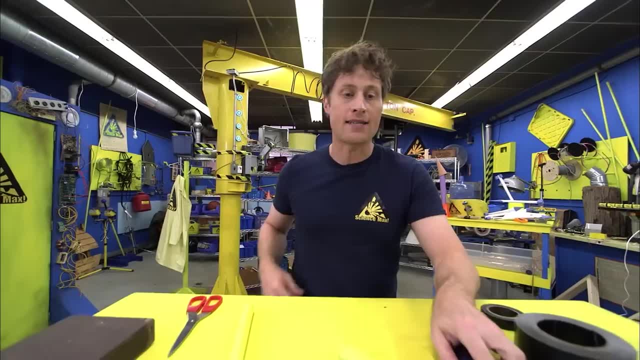 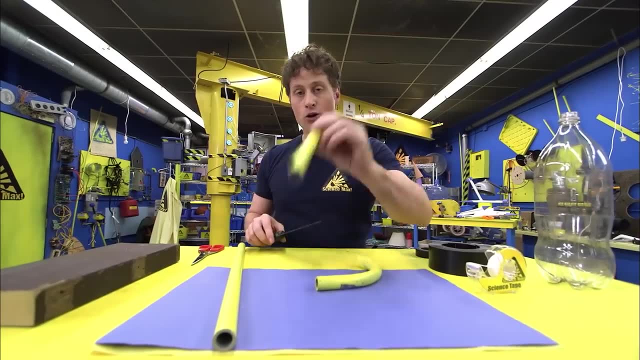 First, you want to take your plumber's tubing and cut it into three lengths- And when I say you, I mean an adult, because you need to use a saw. So you saw it up into a long piece and a short piece and an elbow piece. 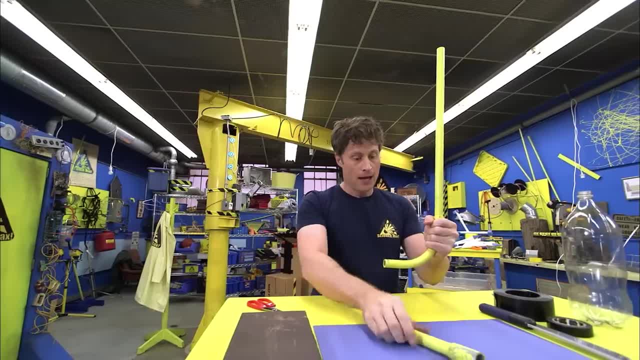 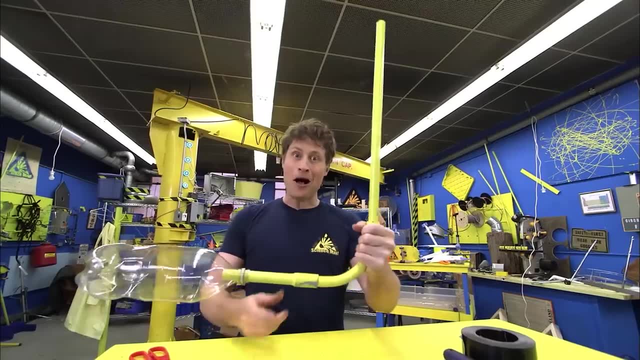 We want to make a long tube at the top, and then we also want to make a tube at the bottom so we can attach our two-liter bottle to. And there we go, Ta-da, Ready to go, But of course it doesn't stay up. 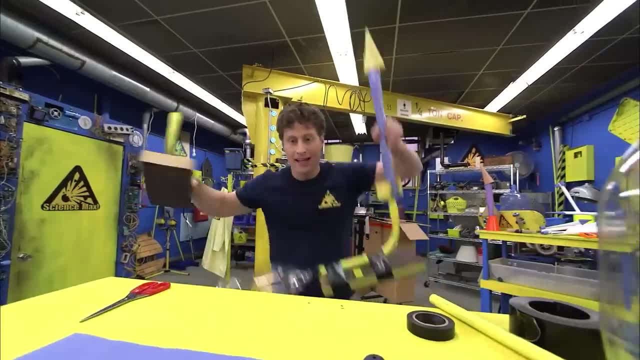 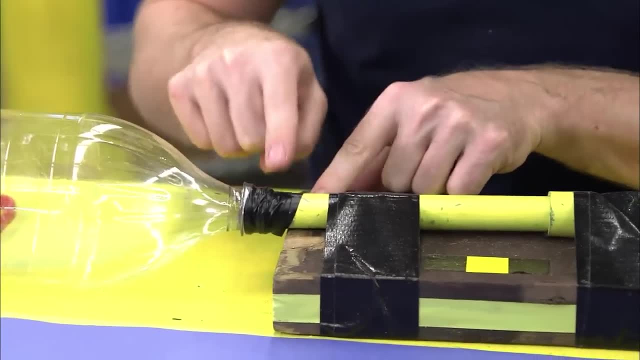 so we have to attach it to a base And it will look like this And you see, it's been attached with duct tape here and I've used electrical tape and I've wrapped that part around there. Now building the rocket. 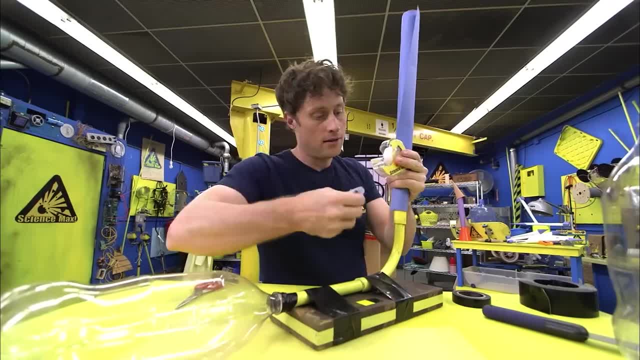 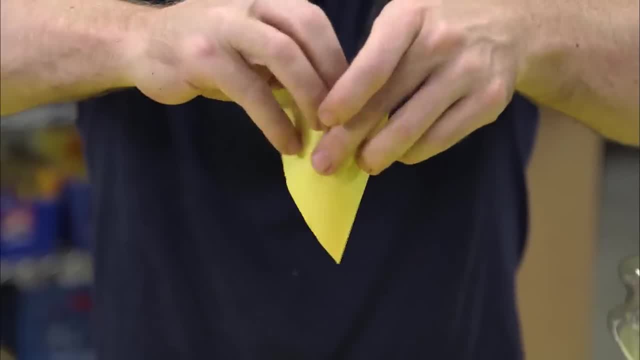 Wrap the tape around. Wrap the paper around the tube and tape it with your science tape. Tape the top closed so no air escapes. Then cut a semicircle to make the nose cone and three hoops for thrusters and tape them to the bottom. 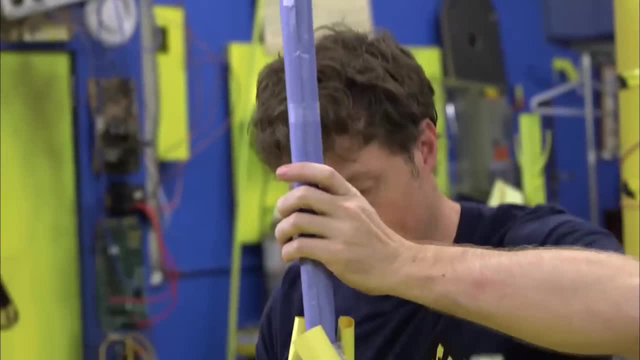 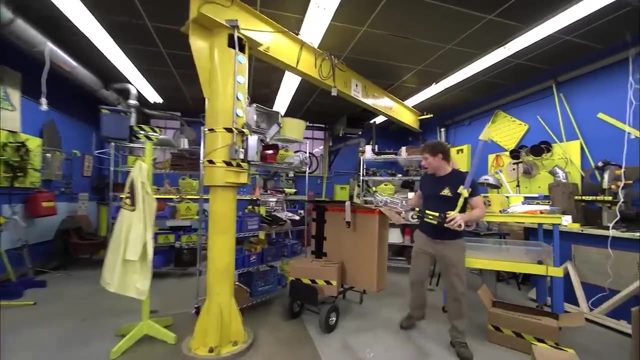 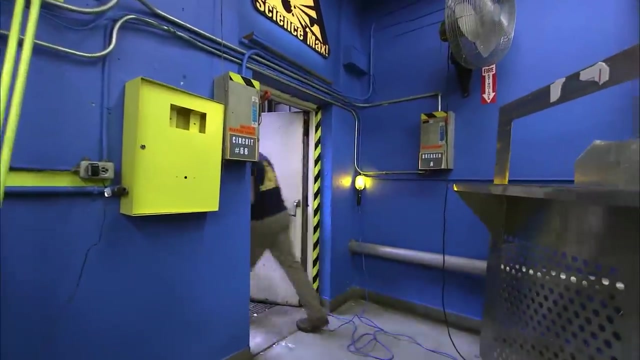 There you go. The rocket fits on the tube just like that And when you stomp on this bottle, it launches. But here's the most important part, The one most important rule of launching rockets: You shoot rockets Outside. Come on. 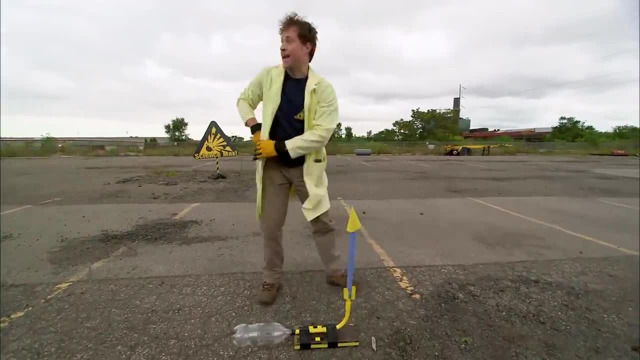 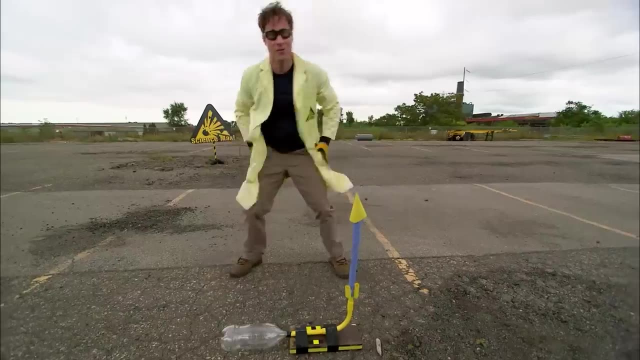 Once you get outside to a nice open area and you bring your safety glasses with you, all you need to do to make the stomp rocket work is, of course, stomp on it. You ready, Here we go. Three, two, one. 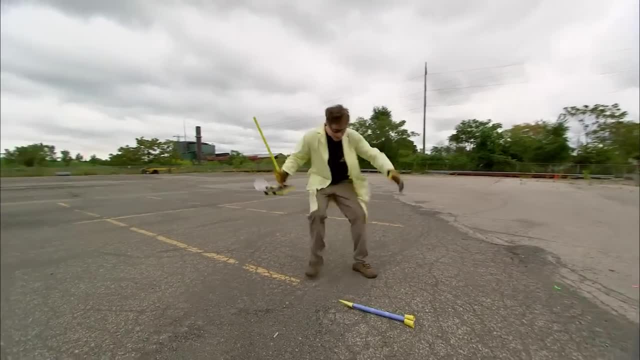 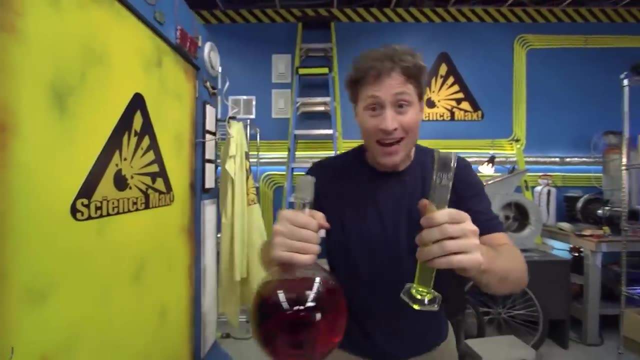 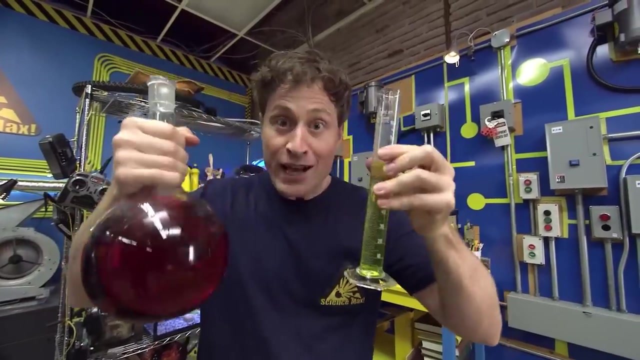 Whoa, You see that That was amazing. Today we're taking a closer look at chemistry. Ooh, Chemistry is the science of atoms and molecules, the things that make up all matter, and how they interact with each other. Take, for example, this glow stick. 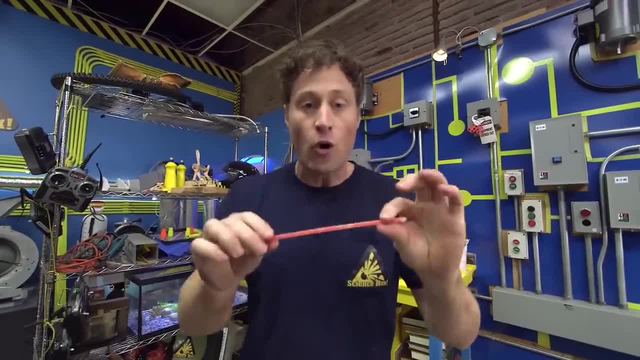 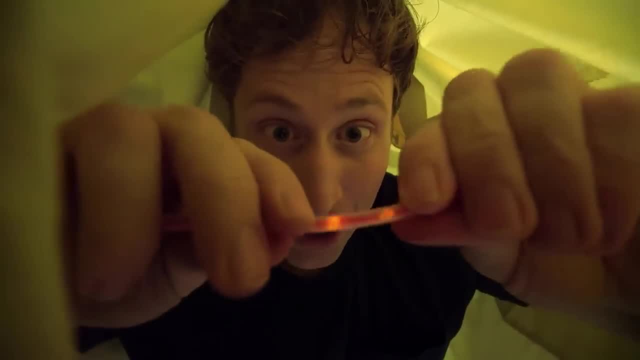 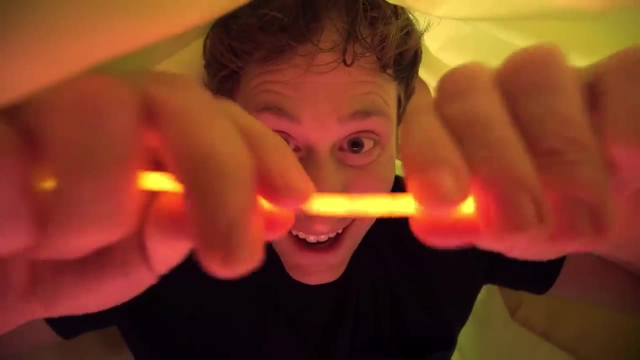 Actually don't take it, because I kind of need it. The glow stick doesn't glow until you- um, the glow stick doesn't glow until you break the barrier and mix the two chemicals and they start to glow. Huh. 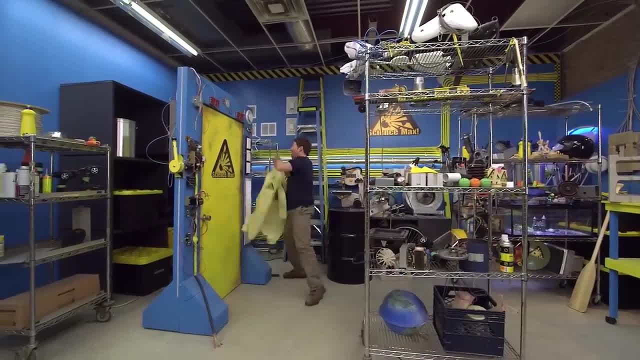 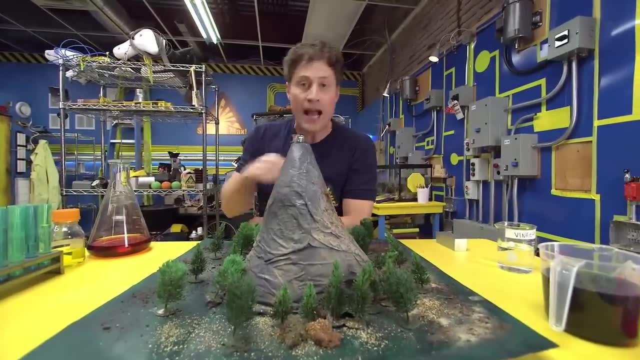 Pretty cool, huh? Chemistry, Chemistry. Now, the chemical reaction we're looking at today is the old vinegar and baking soda volcano, But this reaction doesn't have anything to do with volcanoes, It's chemistry. Now, this experiment is totally safe. 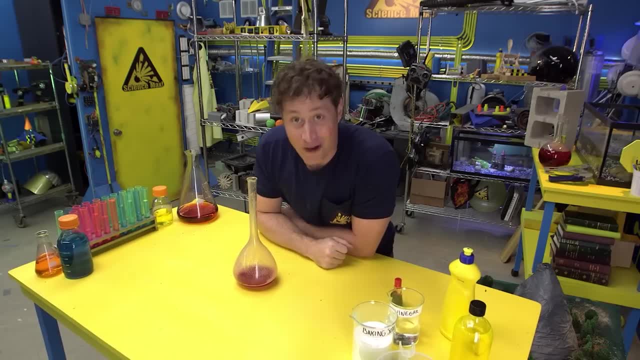 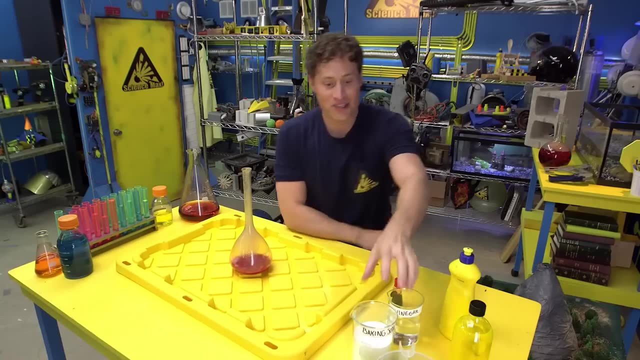 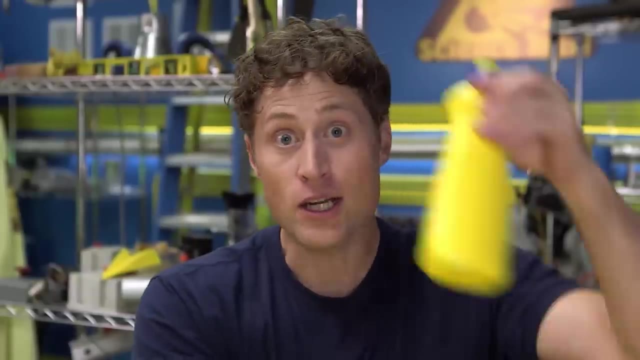 but I do recommend you get an adult's permission before you do it, because it's very messy. Uh, uh, yeah, Ha ha. First you're going to want baking soda and vinegar. These are your two main ingredients, But you'll also want dish soap and red food coloring. 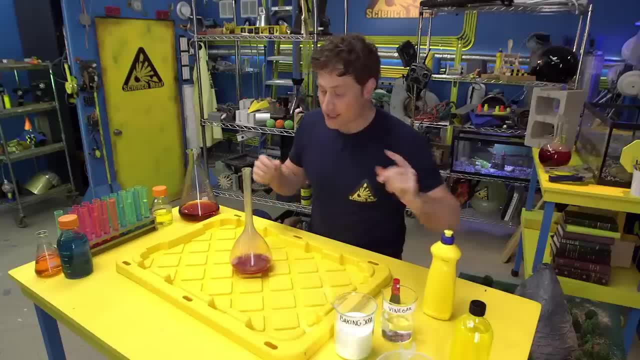 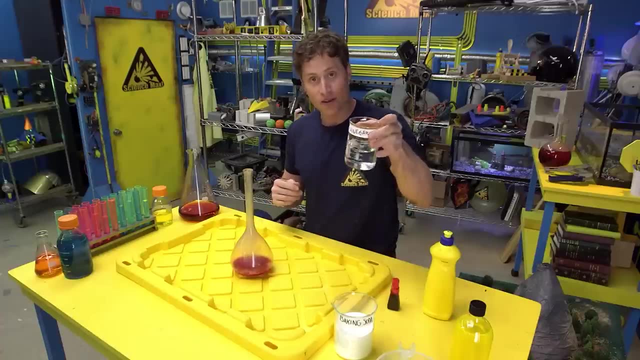 if you want it to look a little bit more like lava. Now I like to mix the baking soda, red food coloring and dish soap together with a little warm water. So all you have to do is add the vinegar, And when you do this is what happens. 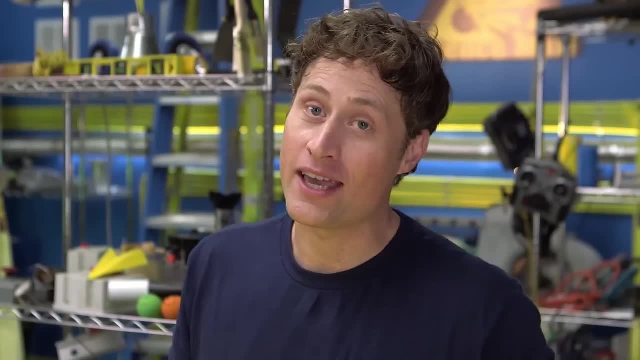 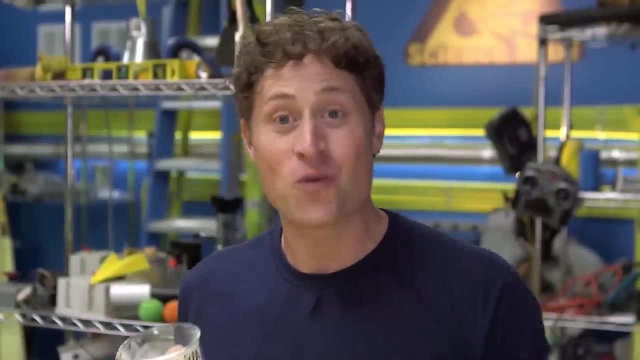 And there you go, Chemical reaction. Now I know what you're thinking. You're thinking, Phil, how much vinegar, or, uh, vinegar, more baking soda do I use? Well, I'm not gonna tell you. This is where you can be science maximites. 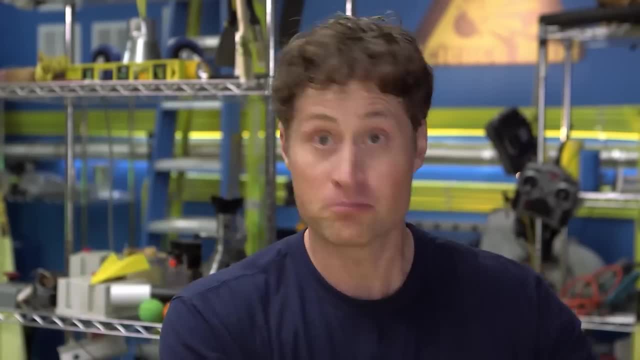 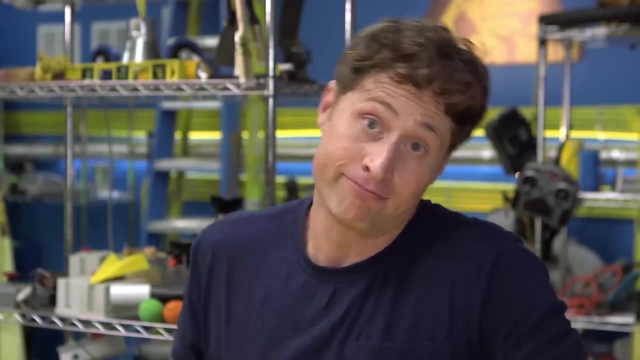 Try different amounts: More vinegar, more baking soda, more dish soap- who knows? Write down the amounts each time you use it and find out what amounts work best. That's called science. Here's another fun way you can play with elastic force. 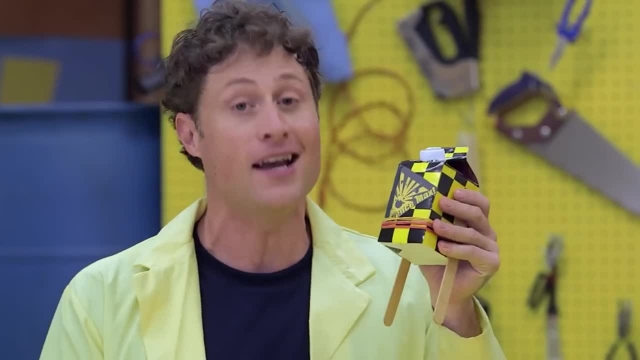 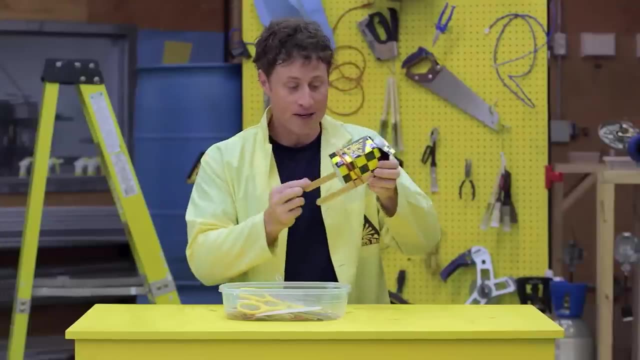 Take a milk carton. I prefer science max milk because it's the creamiest: 2% cream, 100% science. Wrap some elastic bands around it with some popsicle sticks on the bottom, sort of like feet. Then take some clamshell packaging. 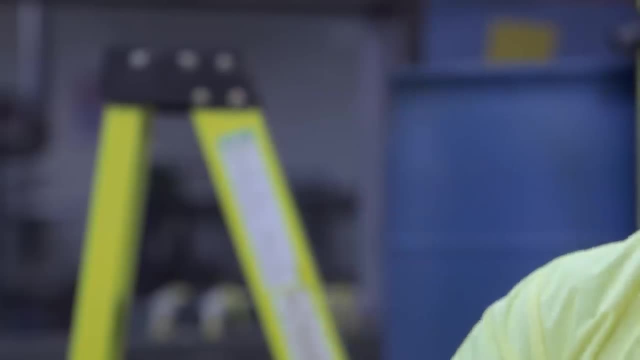 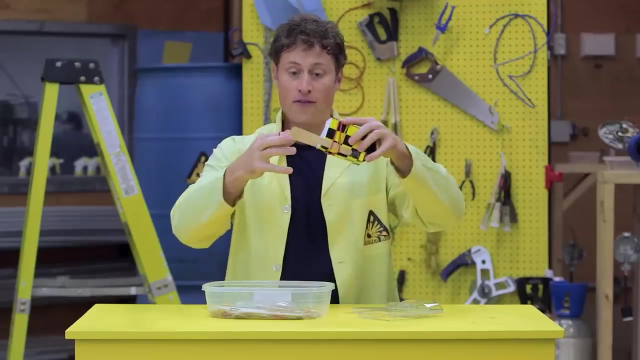 which wraps just about anything you buy nowadays, and cut out a square or a rectangle, Then wrap some tape around that square with an elastic in it and put the elastic on the feet of your milk carton, Then wind it around and make sure you go backwards. 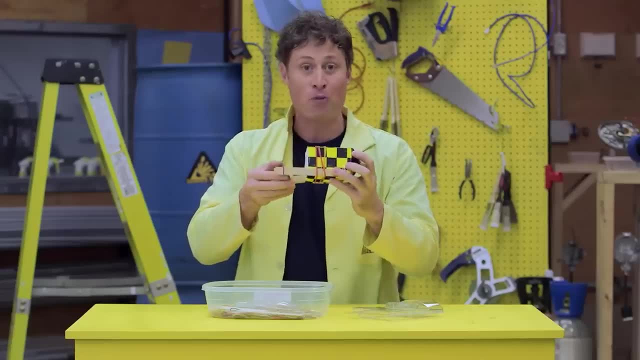 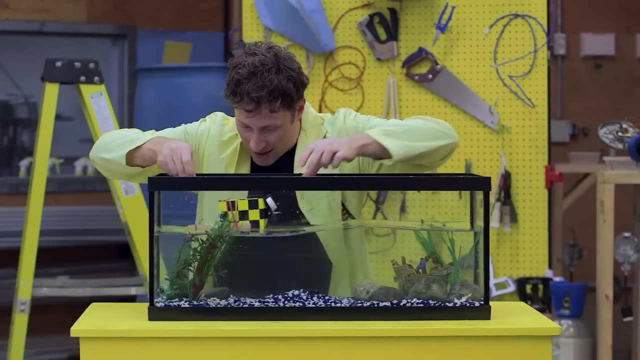 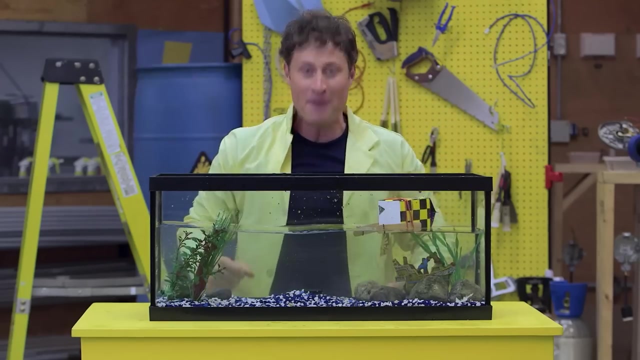 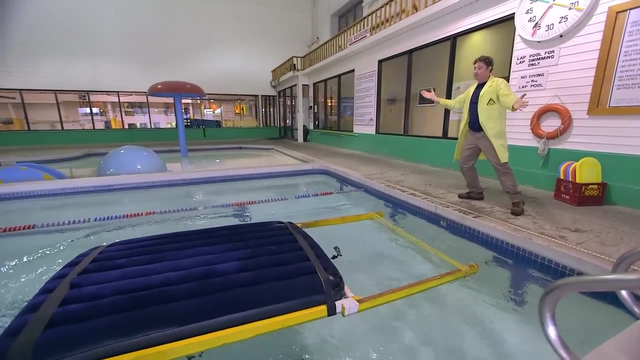 so your paddle wheel boat will go forwards when you put it in The water. And there you go, a paddle wheel boat. Now it is time to max it out. Ahoy, the SS Maxed Out. Elastic Force Paddle Wheel Boat Mattress. 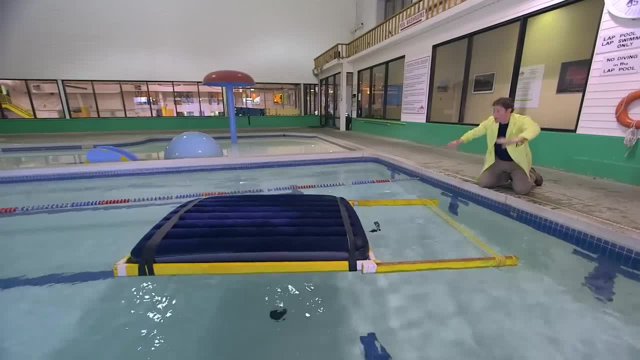 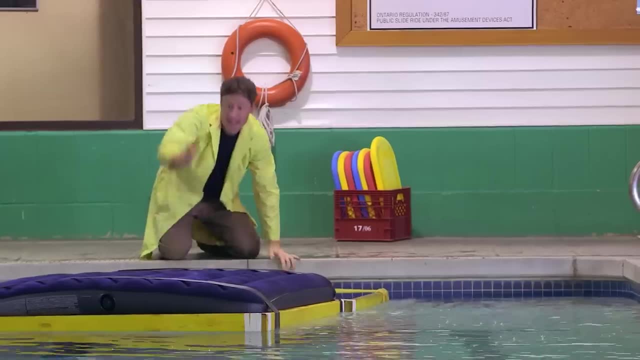 I need a better name, But I've made a giant paddle wheel boat that works on elastic force, because I've got surgical tubing as my elastics And that's an air mattress And then I use some lumber to hold it all together And of course, I need a paddle wheel. 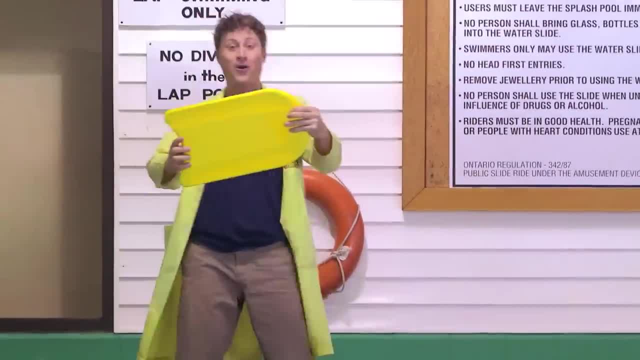 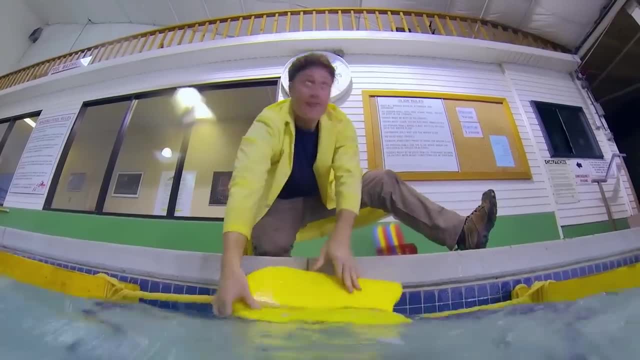 And what better thing to use in a pool than a flutter board? OK, here we go. So normally, you're not allowed to wear your clothes and your shoes in the pool, But I got special permission because of science. Besides, I'm not worried at all. 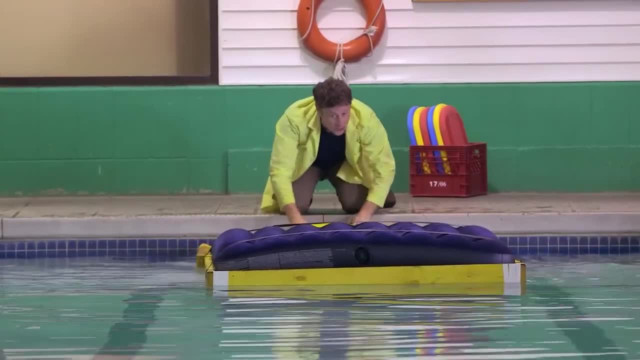 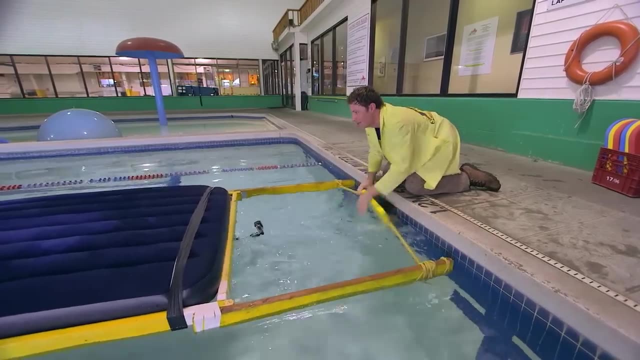 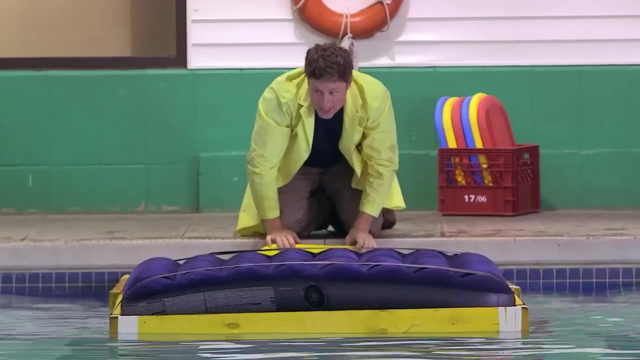 So I didn't wear my swimming outfit because I figure I can totally do this entire experiment without even getting wet. That is how confident I am. All right, now the tricky part: we'll be getting on to the mattress. OK, here we go. 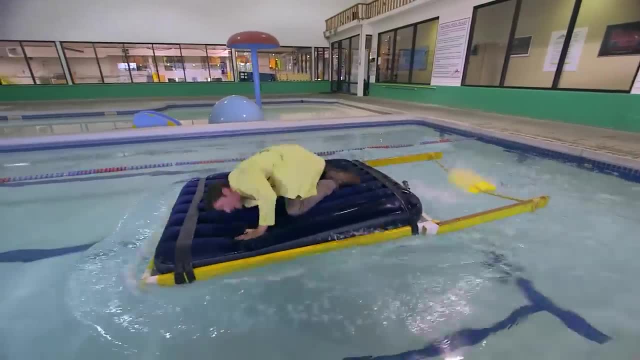 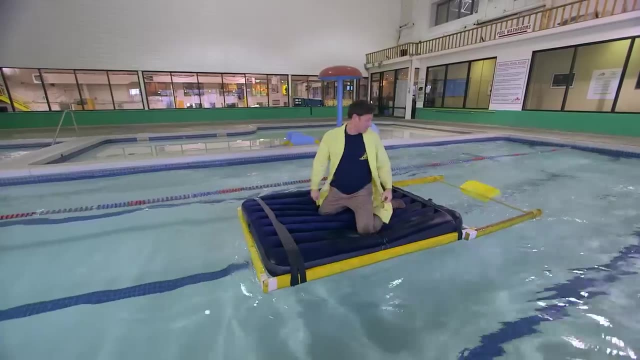 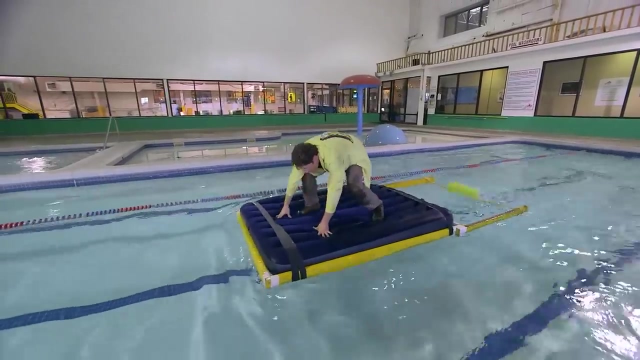 Ha-ha, Uh-oh, Ah, Ha-ha. The SS Science, The SS Science. Hey, SS Science, That's a great name for this. Look, it works great And I managed to stay totally dry, Huh. 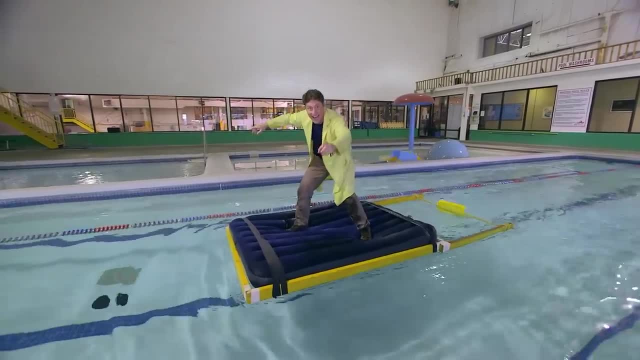 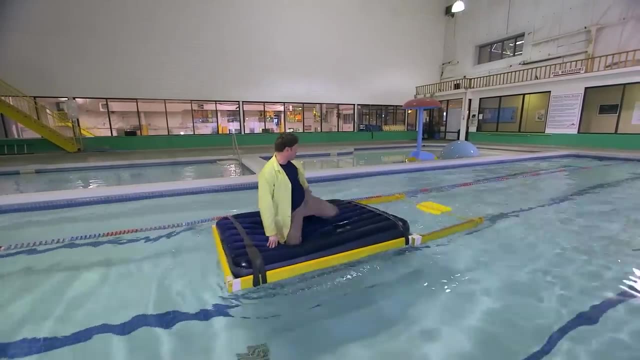 Well, almost, Whoa, Oh, Oh, Ha-ha. You thought I was going to fall in the pool, but I didn't. Uh-oh, My flutter board has stopped moving and I'm in the middle of the pool. 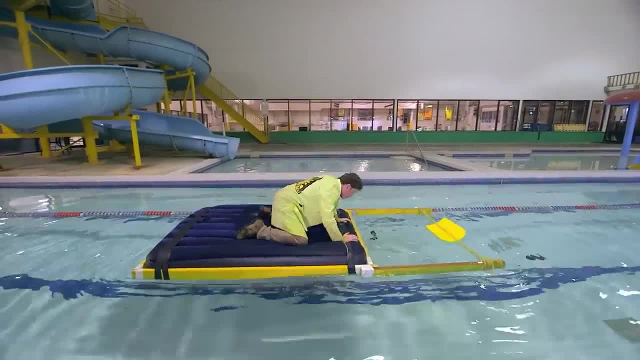 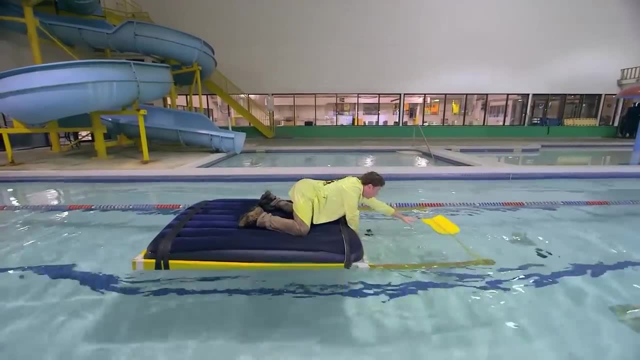 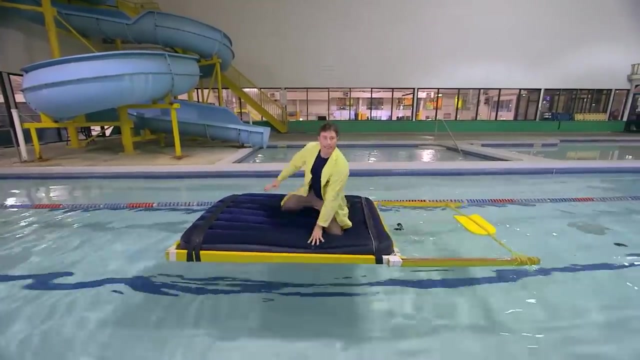 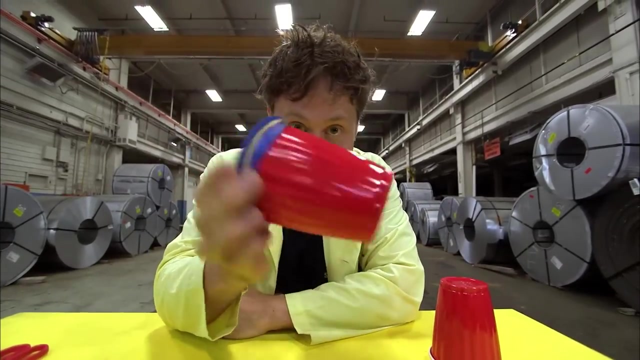 Almost, Almost. Yeah, Didn't think this through. No, No, No, No, that's not going to work. Maybe I'll wait. Moving air is a lot of fun, especially if you use one of these, a Vortex Canon. 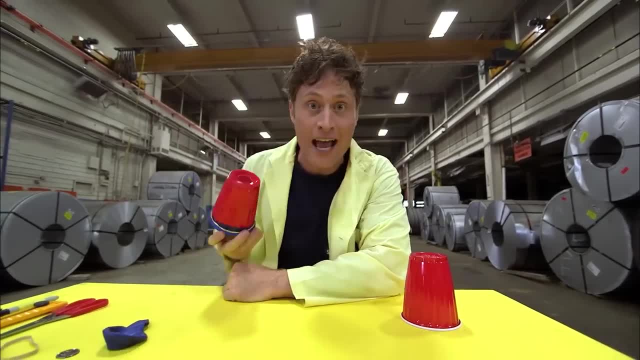 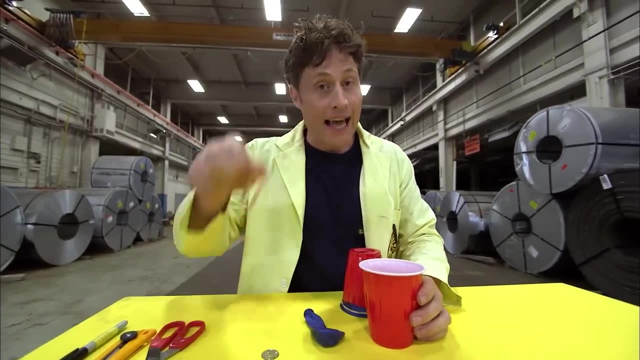 They're pretty impressive and they use some pretty amazing science. I'll show you how to build one. It's pretty simple. All you need is a plastic cup. You want a balloon, something round an elastic scissors or a craft knife, and a pen. 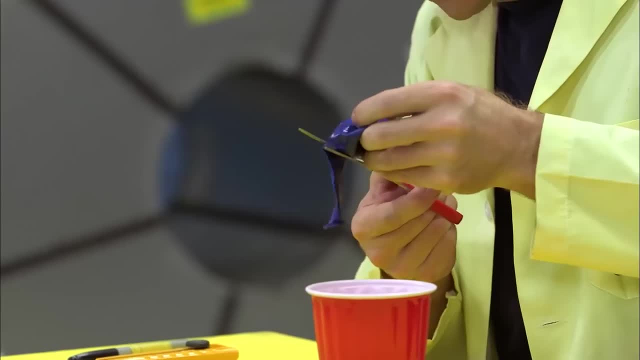 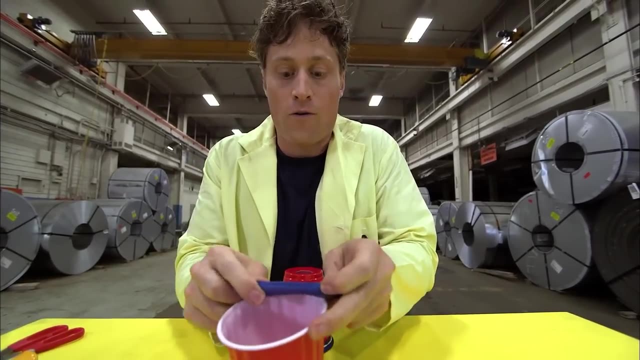 Here's what you do: Take your balloon and cut it just where it gets wide. You take the mouth of the cup right there and you have to stretch the balloon over the top, And then you want to put an elastic around it. keep it in place. 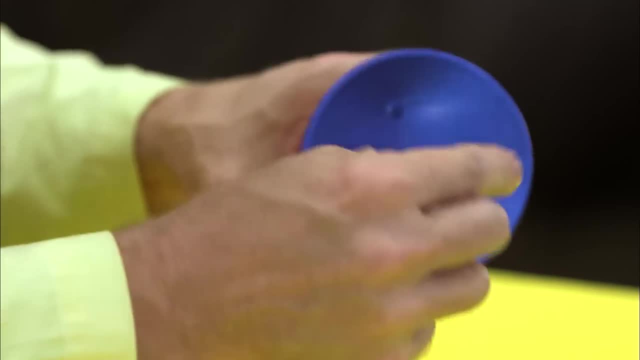 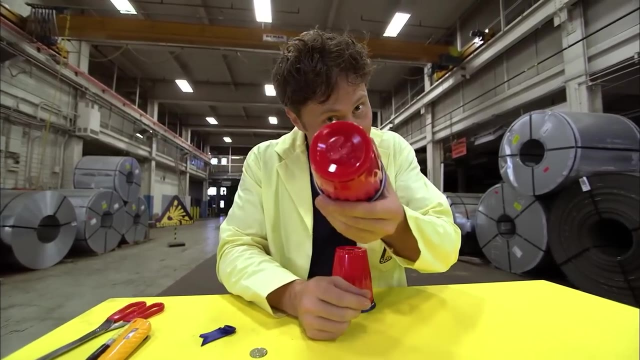 And this now is a surface on the top And that's what you're going to use to pull back and create your burst of air. But of course, the air is not going to go anywhere until you make a hole in the bottom. So here's what you do. 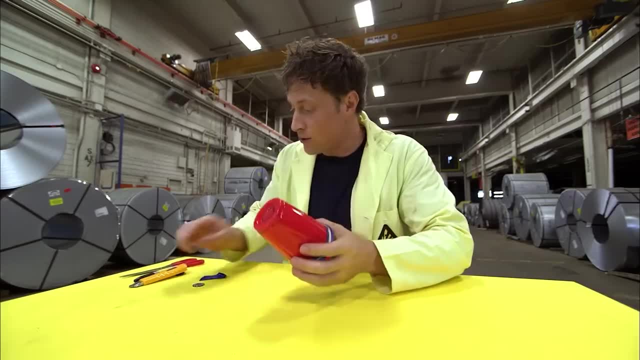 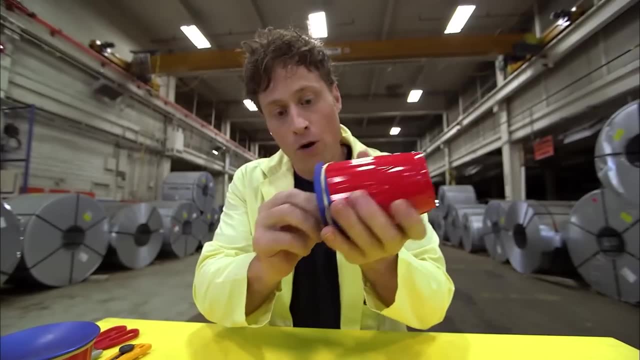 You take your round thing and draw a circle And take your craft knife or scissors and an adult and get them to help you cut out a hole. And when you pull back on the balloon a burst of air comes through the hole. But the air has an interesting shape. 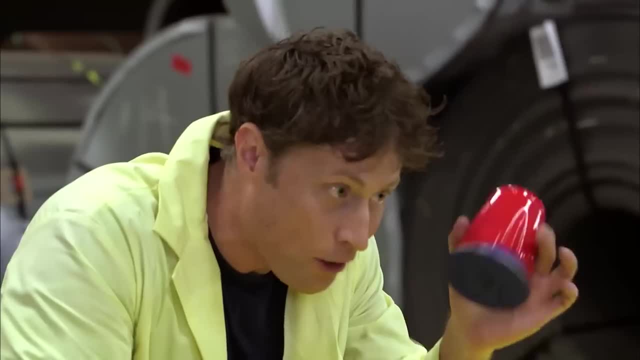 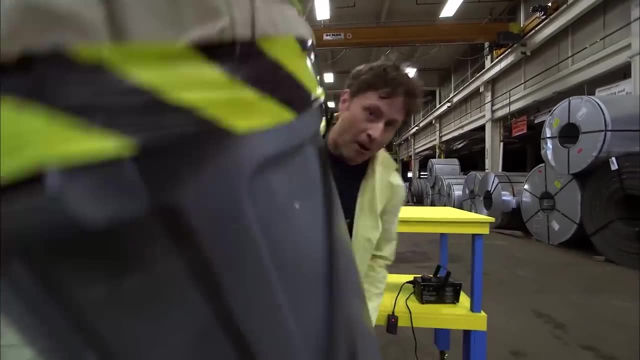 Now I know what you're thinking. You're thinking, Phil, air is invisible. You can't tell what shape it is. Well, I can show you. Come on, This is my maxed out vortex cannon. It's made out of a garbage can. 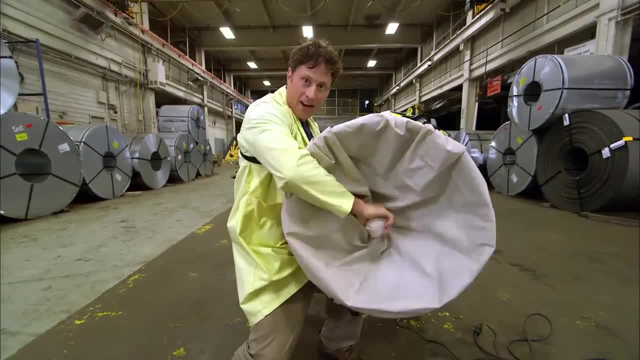 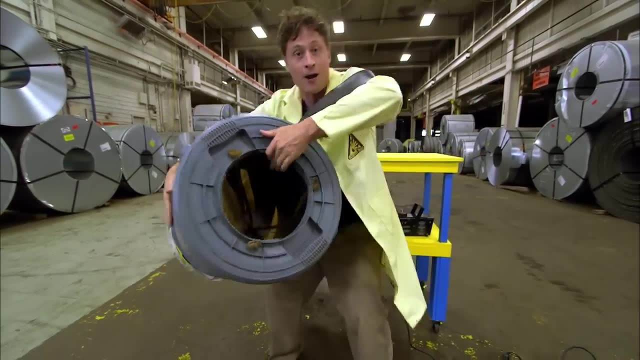 I've got a hole in here And this is a shower curtain with a ball that I can get a grip on and pull, And then it shoots forward like this. Now it makes a big puff of air, But again the air is invisible. 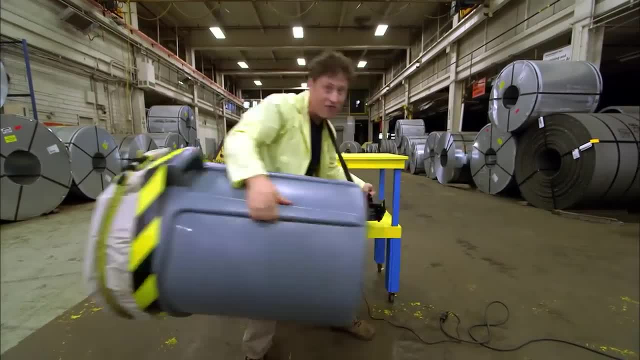 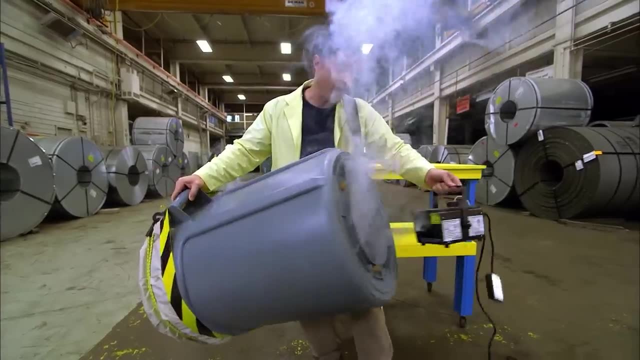 So we don't know what shape it is. But I can help with that Because I've got this, a fog machine. I fill the inside of the garbage can so we can see what the air is doing when I fire the vortex cannon. 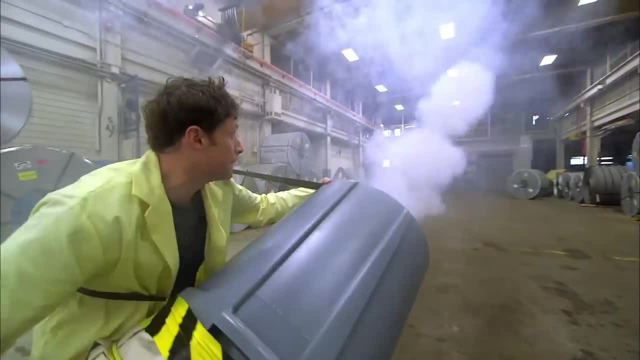 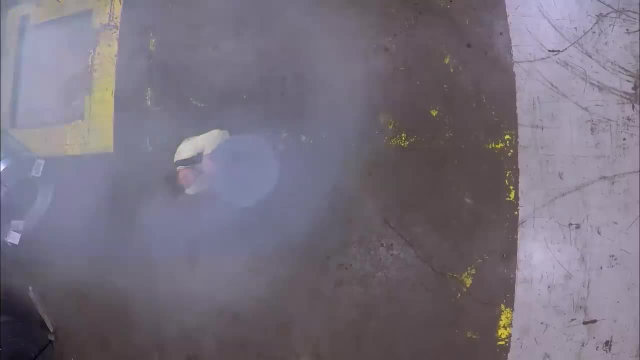 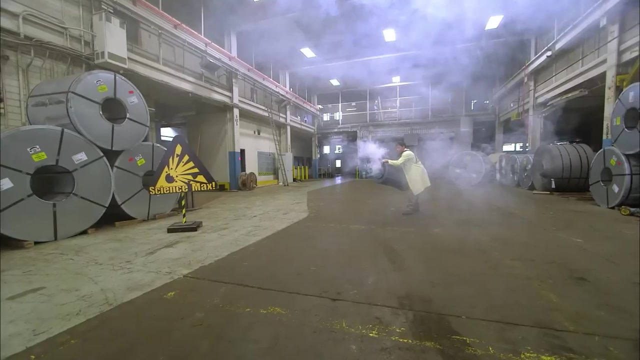 OK, come on over here. Ready Whoa, OK, ready, Check it out. The vortex cannon shapes the air into a ring called a vortex. It makes a ring Well, actually sort of a donut Because of its shape: the air in a vortex. 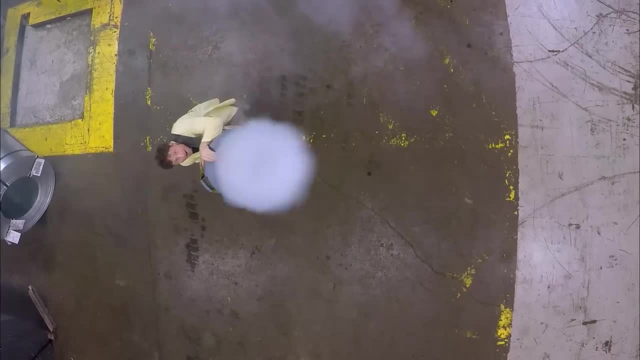 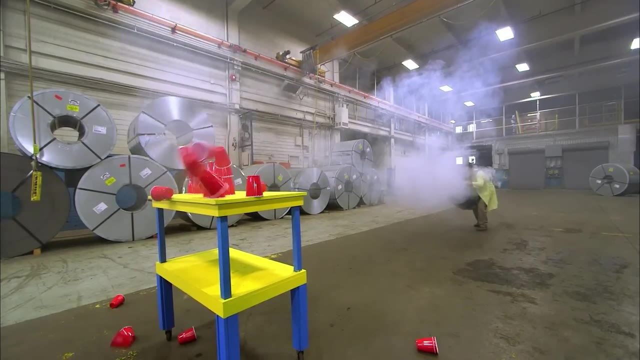 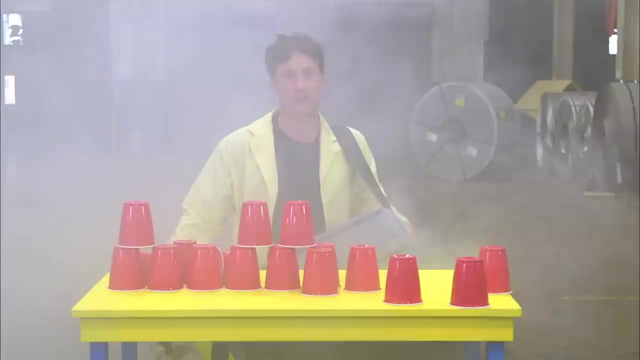 can move much farther than the air, And it goes a lot further than air that doesn't have a shape. Vortex cannon Air that has a shape goes a lot further than air that doesn't have a shape, And it's also way more fun. 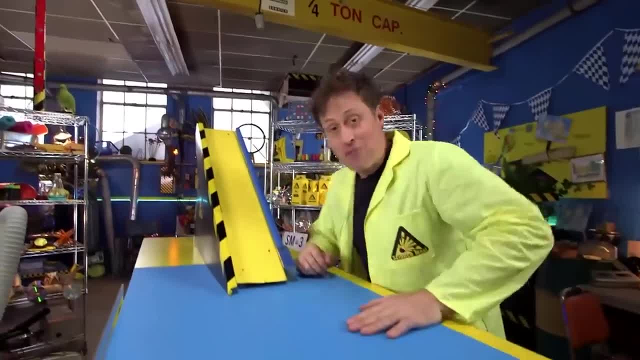 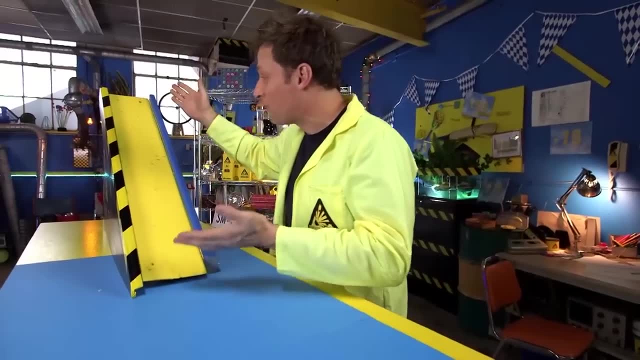 Woo-hoo. As you may have already guessed, today is about friction, And here's a really easy friction experiment you can do at home. All you need is a piece of wood. You don't need the frame And you don't have to do anything fancy to it. 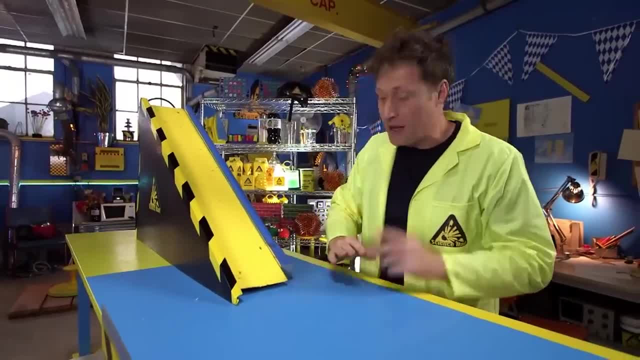 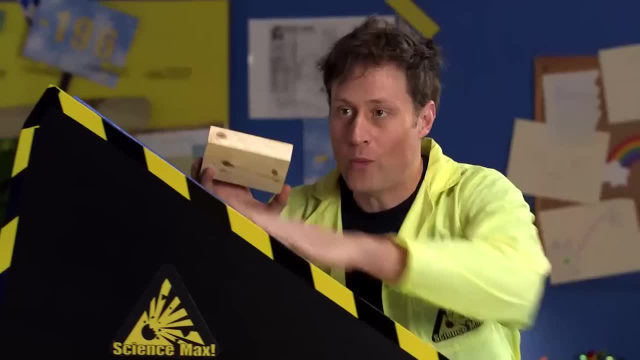 Just put one end up on a couch or a coffee table and make a nice ramp. Then you want something to slide down that ramp And I like to use a piece of wood. Now check it out: Wood ramp, wood block. The friction is so much that the wood slides to there. 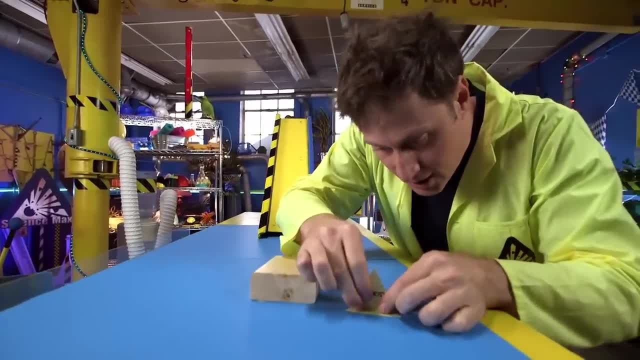 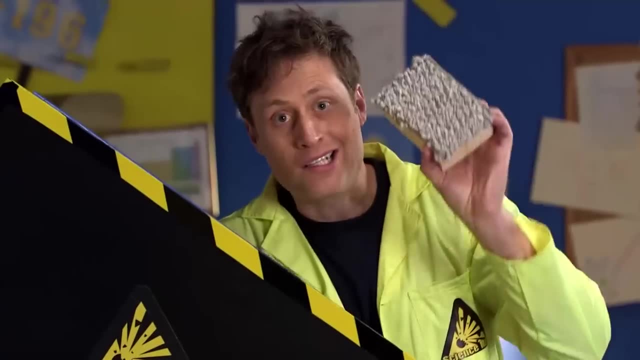 Now what I like to do is take a little flag and mark the results. Recording the results is good science. Now here's where it gets fun. Get another surface and attach it to the wood like carpet And wood. Let's see how far this goes. 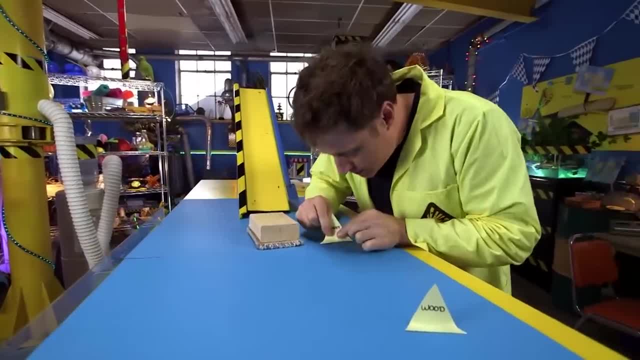 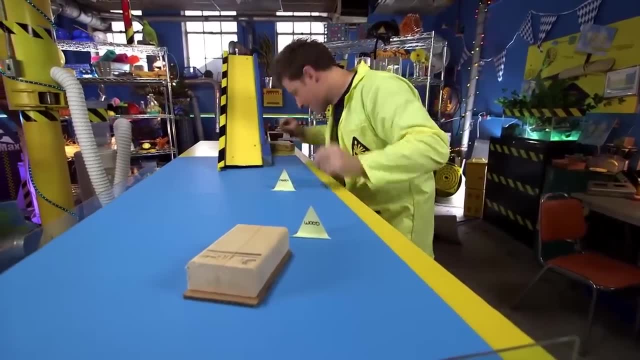 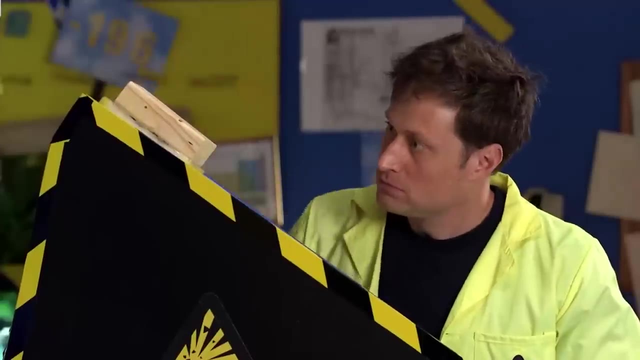 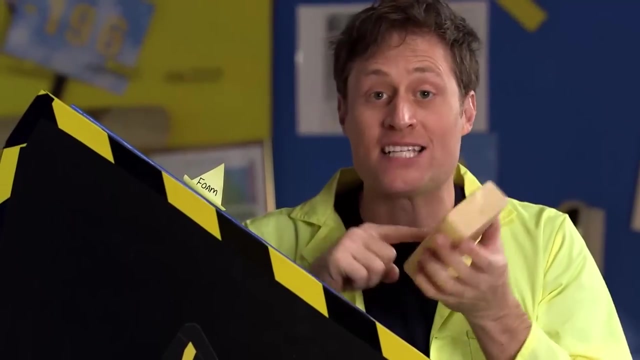 Hmm, not as good. All right, Record the results. Cardboard- Ooh, nicely done. cardboard Foam And this wood has been waxed like on a floor, and it's been waxed, which makes it nice and slippery. 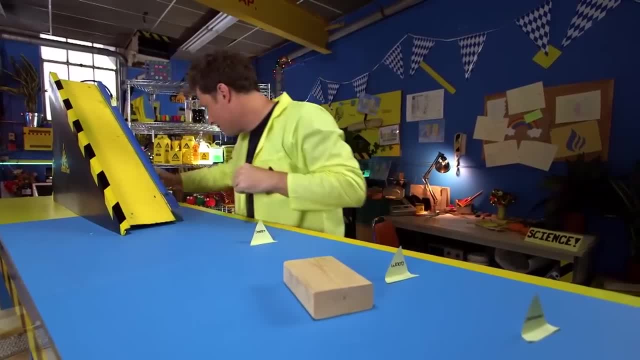 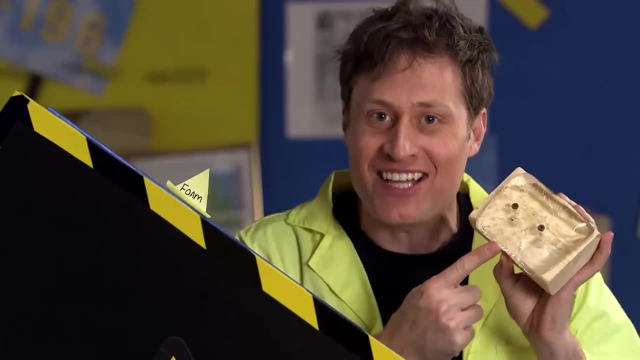 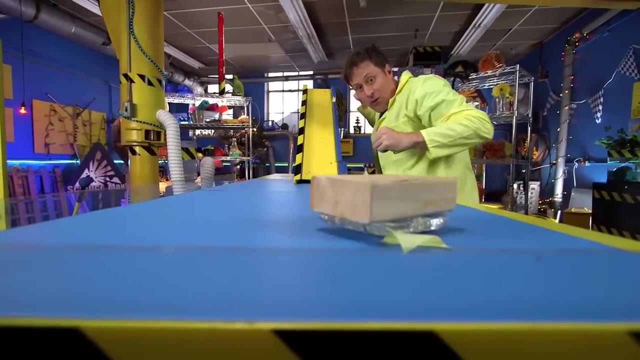 Let's see how that does. Ooh, Ooh, And now the ultimate ice attached to wood. This is actually harder to do than I thought. All right, let's try it out. Ooh ice, The clear winner. 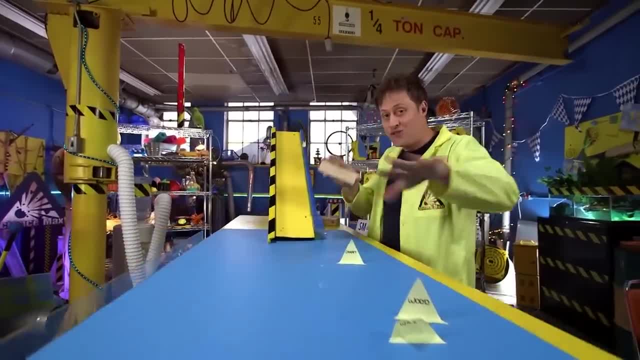 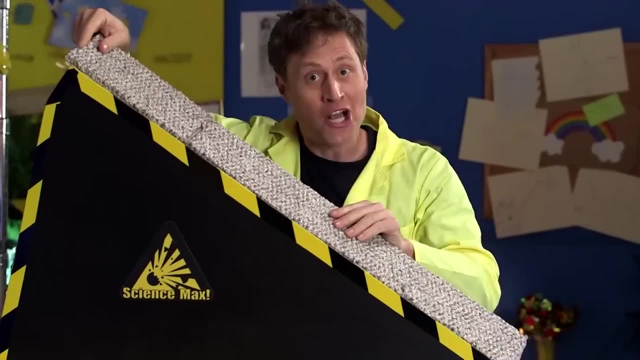 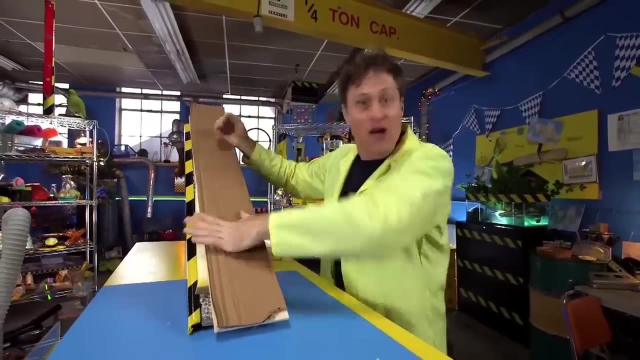 Not a big surprise. right there And get this. Once you've done all of that, you can change the surface of the ramp. Go to waxed wood, carpet, foam, cardboard, Well and well, yeah, you get the idea. 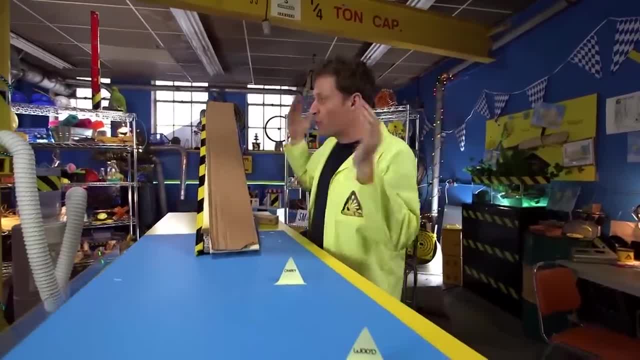 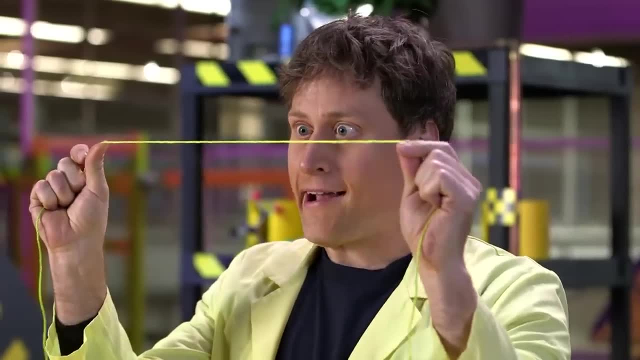 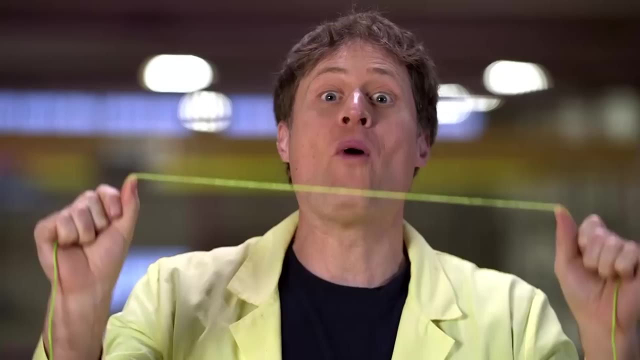 Record all the results, compare them and there you go: Friction ramp experiment. And that's what we're going to be maxing out today. So come on, let's go. This is a string. You can pull a string, but you can't push a string. 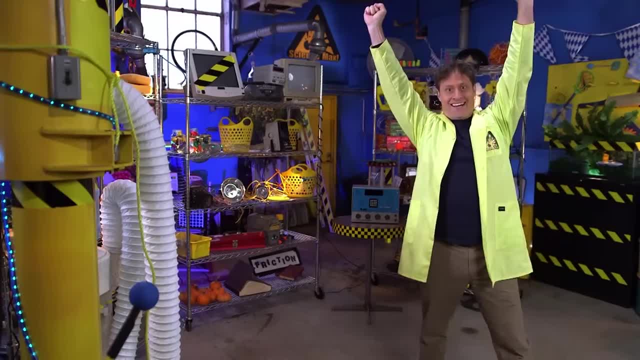 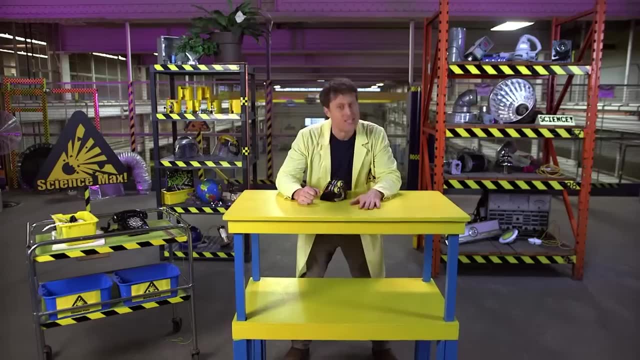 Well, you can, You can push a string, You really can. OK, quit it, Quit it. This little contraption works sort of like a baseball pitching machine, but in miniature. See, there are two motors here and the wheels. 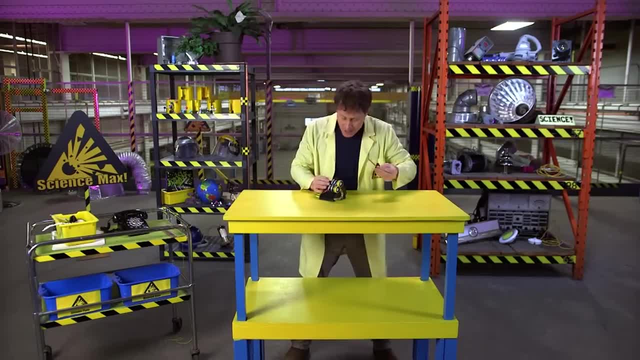 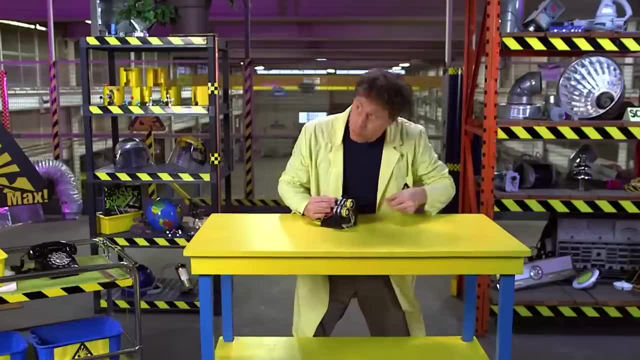 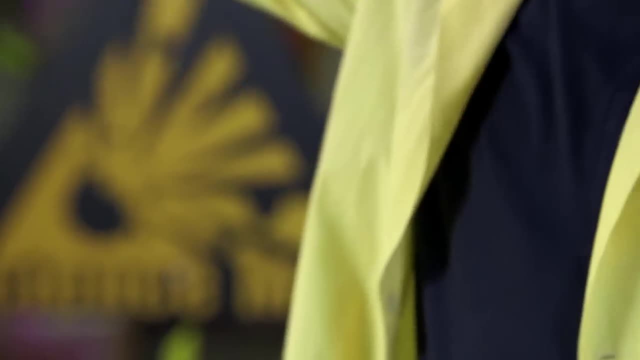 spin together to shoot things out this way, things like this craft stick. Watch this, Whoa. Let's watch that again, Whoa. But now watch as I put a large loop of string through. What Pushing string? How does this happen? 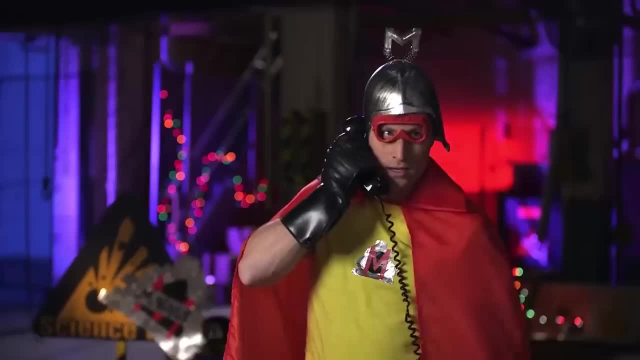 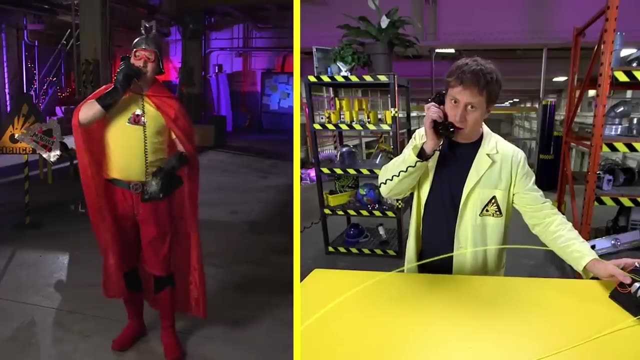 Hello, I don't suppose it's the Magnus effect. No, it's not the Magnus effect. No, that's all right, I'll be in my lair if you need me. OK, right, Bye, Right, where was I? 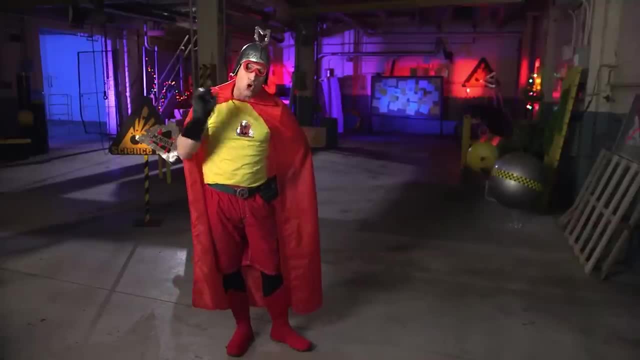 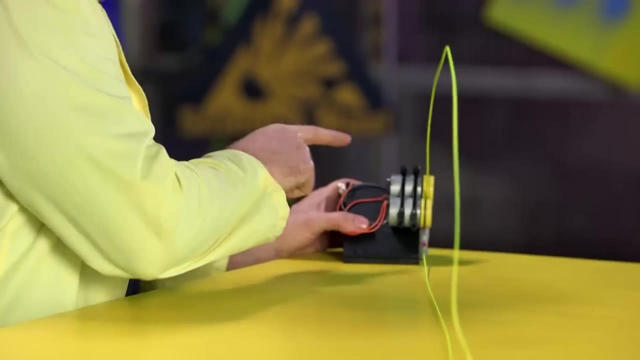 I believe you were at. the reason why this works is Right pushing string. How does this happen? It's all because of inertia. Check it out. The wheels are pushing the string through fast. It's got some weight and it's got some speed. 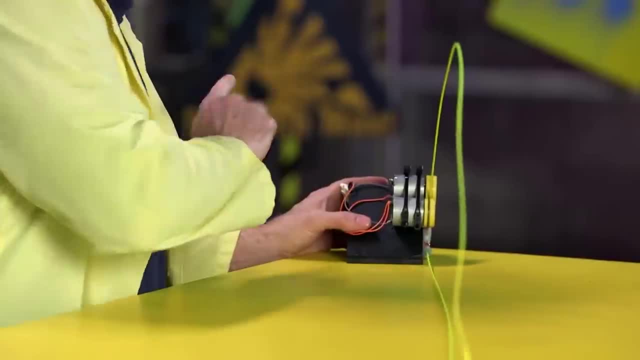 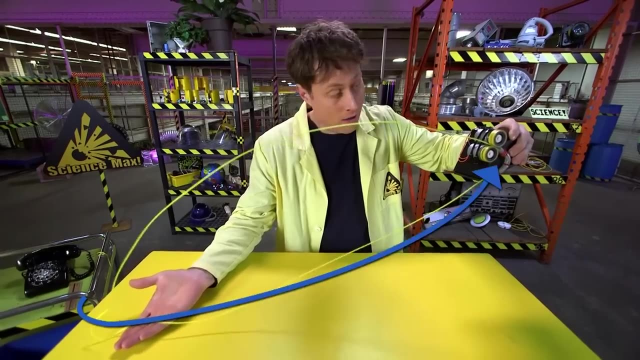 which means it has some inertia. So when it goes this way, it wants to keep going this way, But it goes all the way to the end and then, because it's a loop, gets sucked back in this way, which means all of this inertia. you. 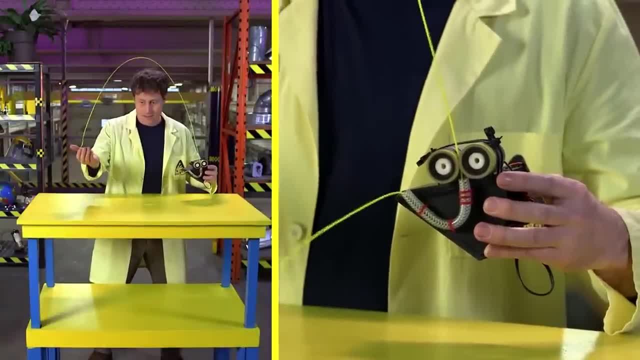 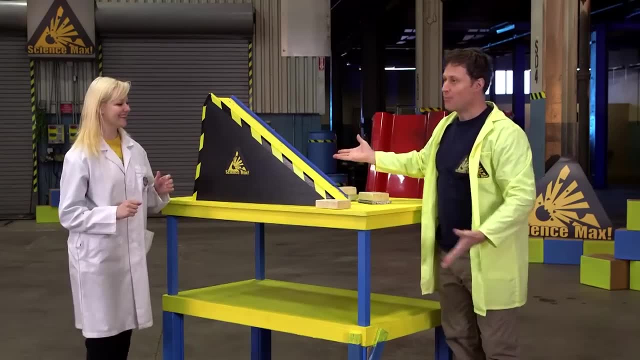 can sort of overcome gravity Pushing string science. So here we go: Amazing, The friction, The friction ramp. It's pretty simple. You just take I've got blocks of wood with different surfaces- Amazing- And then you just slide them down the ramp. 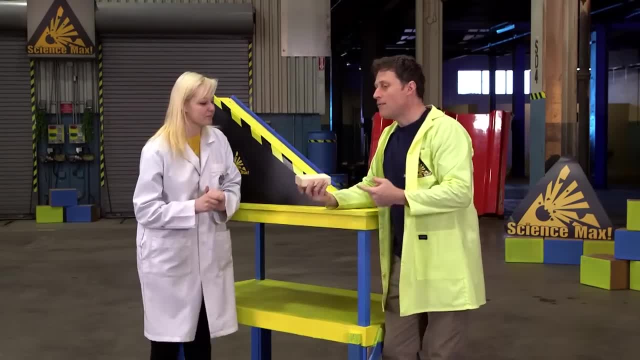 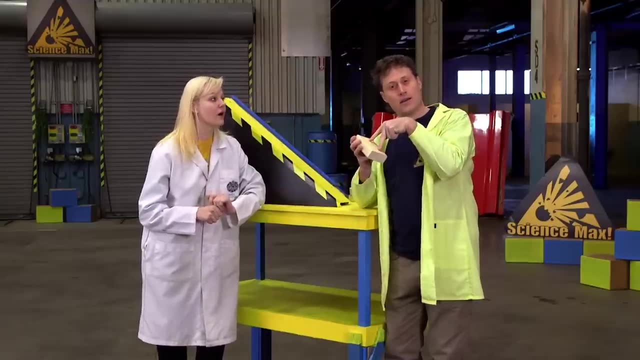 All right, So cool, Yeah. So what if? to max it out, what if this is us? We're a block of wood. No, I mean like we are on the block of wood. Oh, And then we can try changing the bottom. 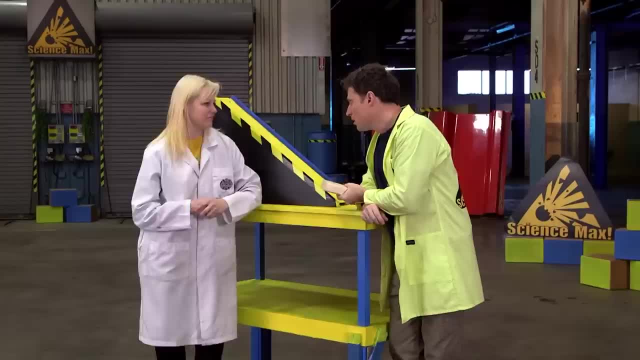 I guess a block of wood isn't the right thing to use, though. Right, yeah, Maybe we could use like a sled. Yeah, OK, like a right, like a snow sled. That's a great idea. OK, so we'll tell you what. 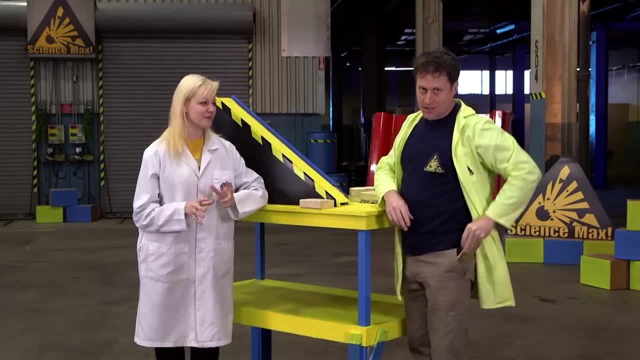 I will portal in a sled for us. Are you sure you want to portal in it? I'm sure Just stand. just stand back, though, OK, OK, Ha. Ah, there we go, Maxed out friction slide You ready, Sarah? 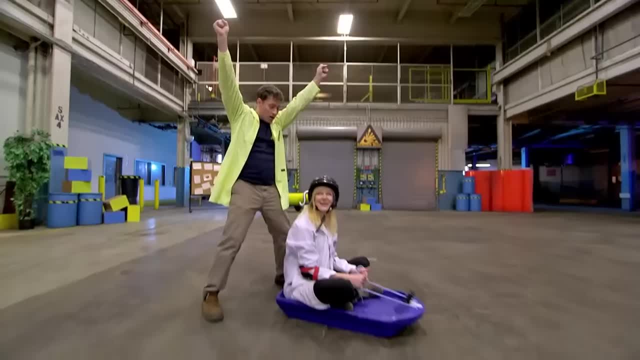 Yeah, I'm ready. OK, here we go. All right, Sarah and I pushed each other around on the sled, which was fun, But it was also tiring. It's uh, it's pretty hard. This is uh. 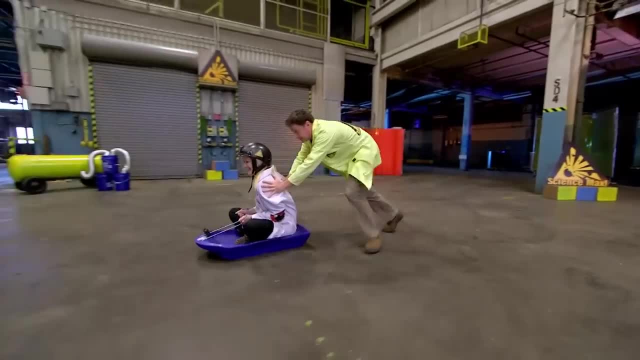 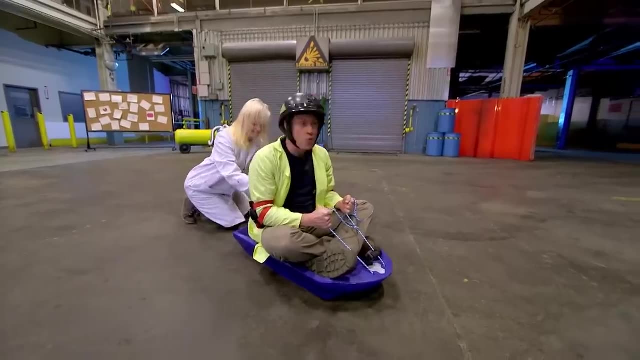 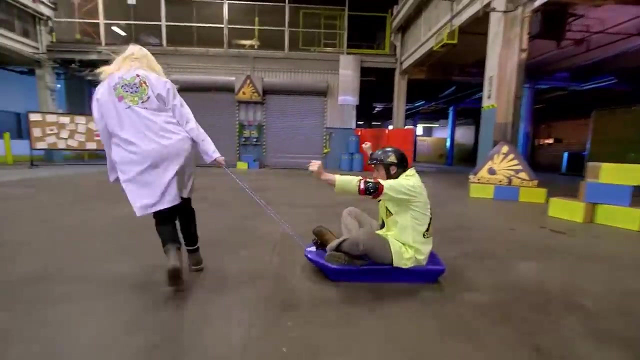 My turn, My turn. All right, Yeah, Whoa, Whoa, Whoa, Whoa, Whoa, Whoa, Whoa. Friction, Yeah, friction, Yeah, Yeah, friction. But we soon realized it'd be pretty hard to measure how much friction there was. 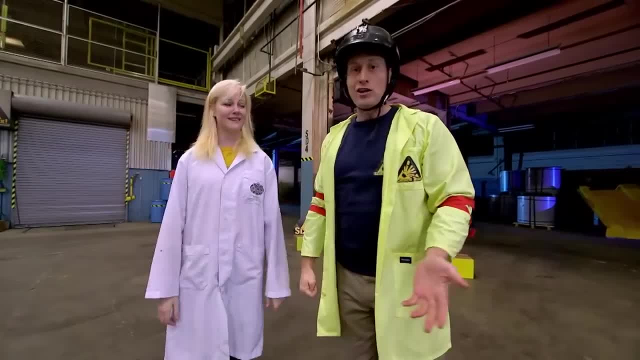 You know how hard you were pushing. I had no idea how hard I was pushing- A lot, but that doesn't really help in science terms. so, Exactly, What do we do? Well, with your first experiment, you used a ramp. 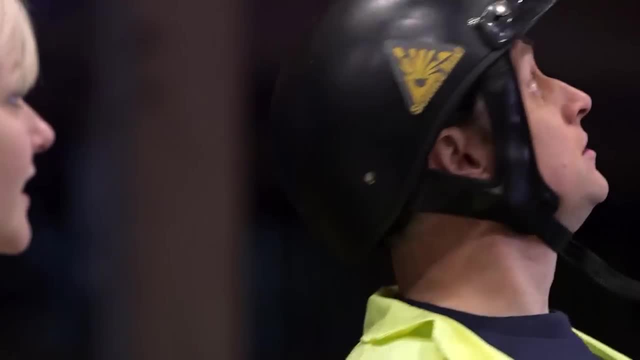 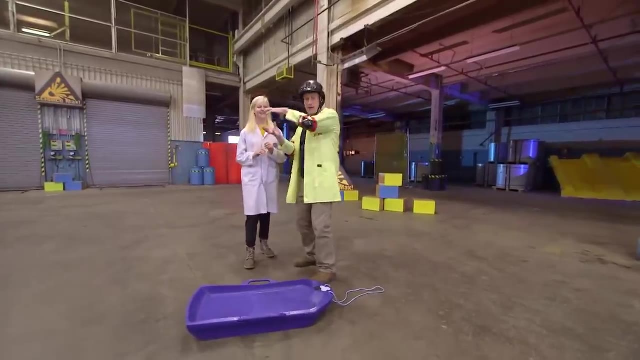 Could we maybe put a ramp up in here, In here, In here, yeah, I guess, uh, Then we can measure also how far we go, so we know how much friction is being used, Right, So we get some control. and then we have all the just like the blocks. 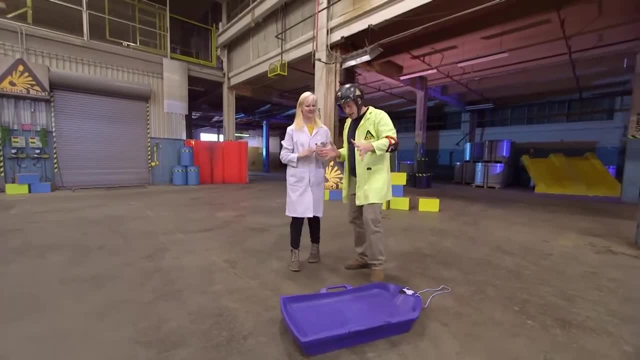 Exactly, just like the blocks. Okay, great, So we get the ramp. we get a bunch of wood. Yes, We'll get some tools. Yep, Whoa, Whoa. This is a Prince Rupert's drop. It's a piece of glass that has a long snaky tail and a bulb at one end. 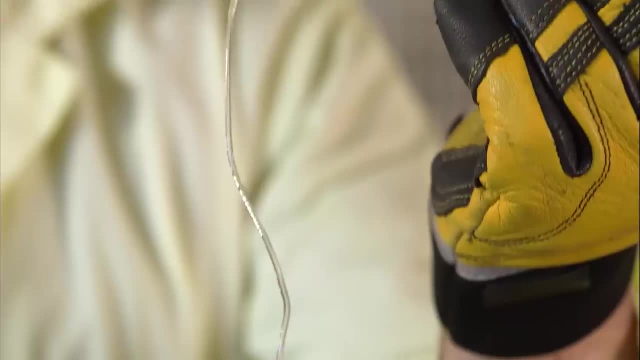 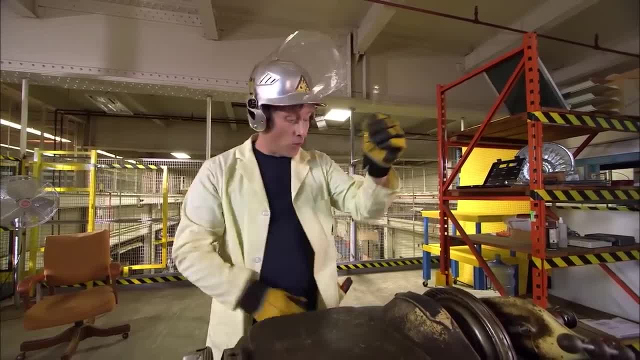 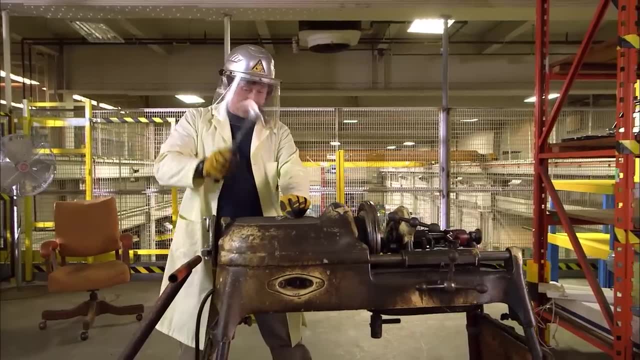 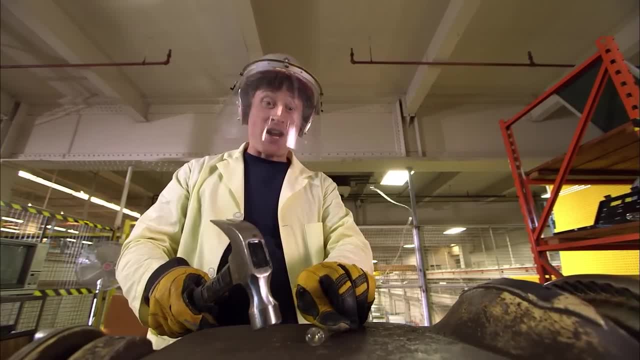 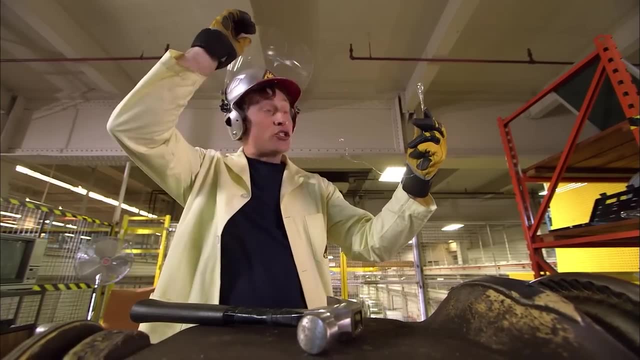 Molten glass is dropped into cold water. What happens is the outer part of the drop cools off first, leaving the inner part still hot. When the inner part eventually cools, it contracts, pulls out and then it cools off again. 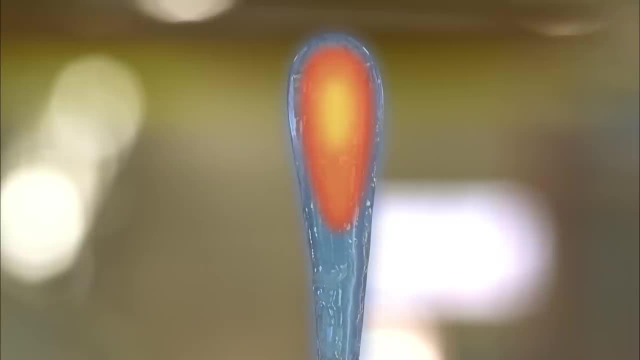 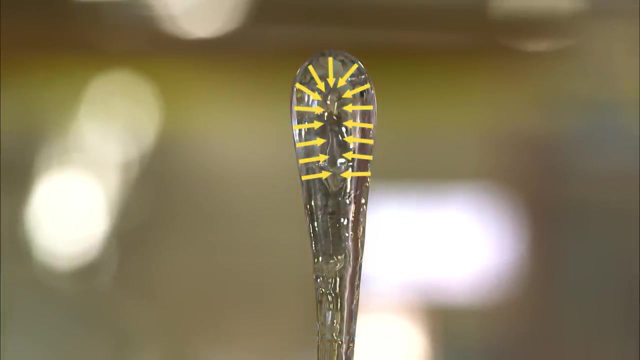 That's what happens when the inner part of the drop cools off first, leaving the inner part still hot. When it actually cools, it contracts, pulling everything in tighter and tighter, keeping it under a lot of tension. And because it's round, 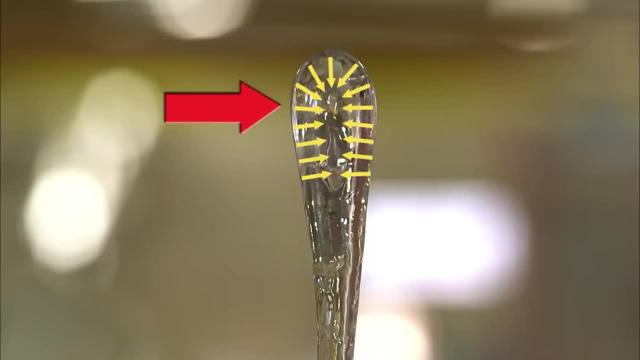 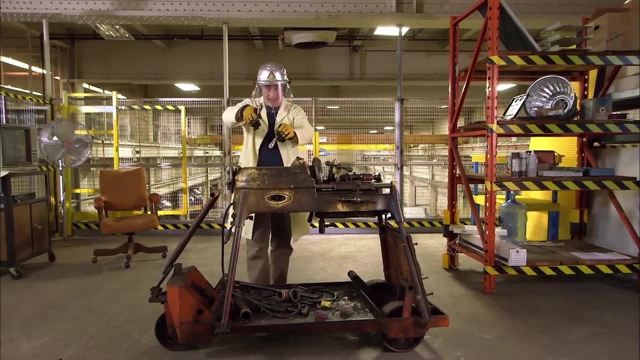 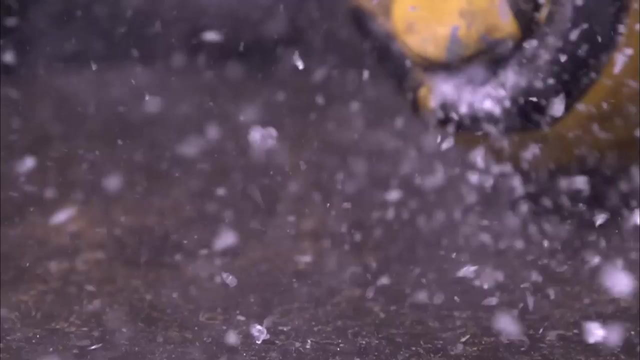 the force you put on, it is distributed all the way around, just like the force is distributed on an arched bridge Until you get to the tail. Just the tiniest break in the tail and It explodes. All that energy is released in a chain reaction. 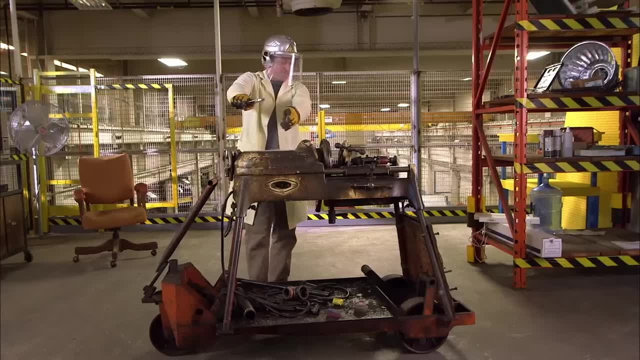 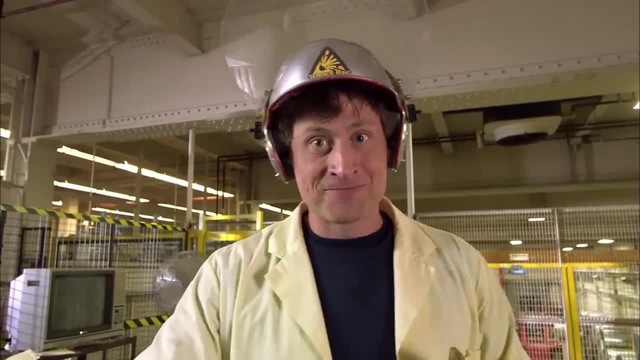 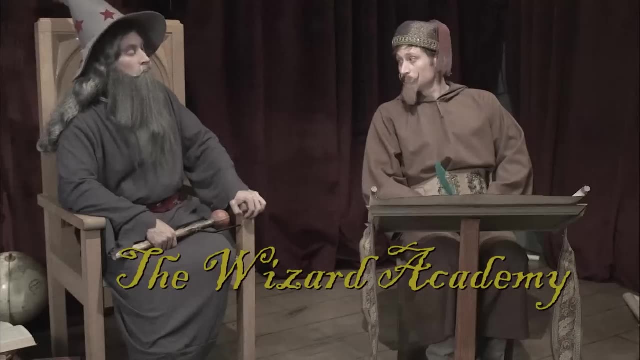 Why it's so strong. you can hammer on it on one end, but it explodes when you break the other. puzzled scientists for centuries, But now we know it's all in how it's made The Wizard Academy. All you have to do is demonstrate true magic. 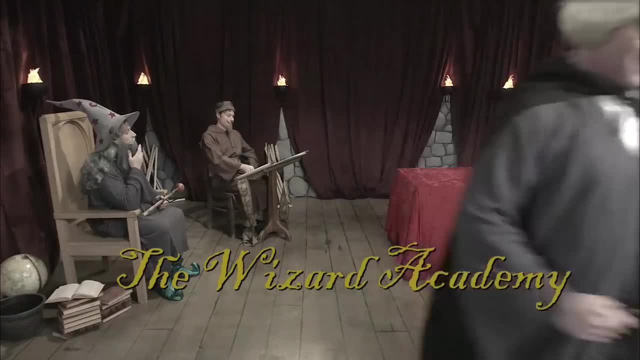 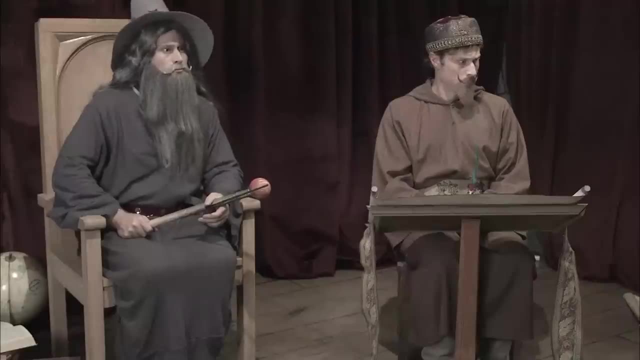 and you will be granted entry. Send in the next applicant. Okay, gonna, let them see you. Gonna, let them see you. Okay, Magic smoke, And here we go, Speak entrance. Behold, it is I Overwhelmo. 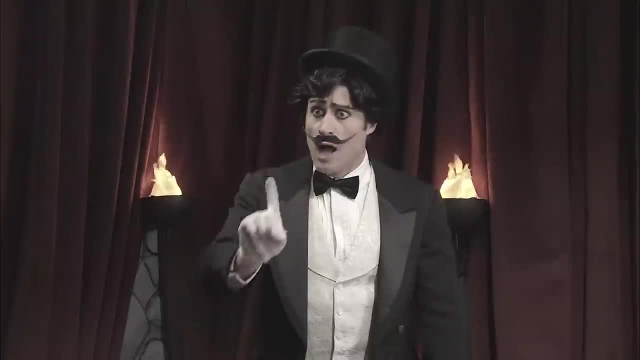 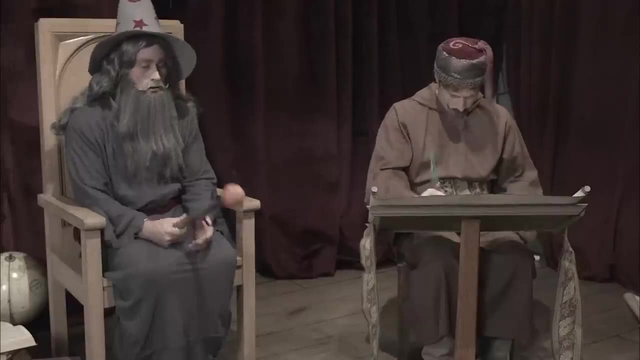 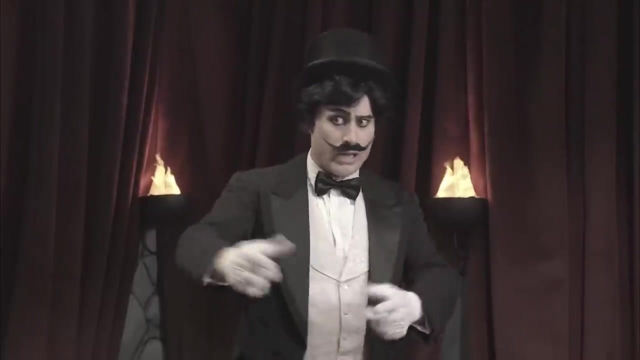 You again. I only have to demonstrate magic one time and you have to let me into the Wizard Academy. And last, last time does not count. So prepare for your mind to be boggled and your eyes to also be boggled, because I shall do a trick. 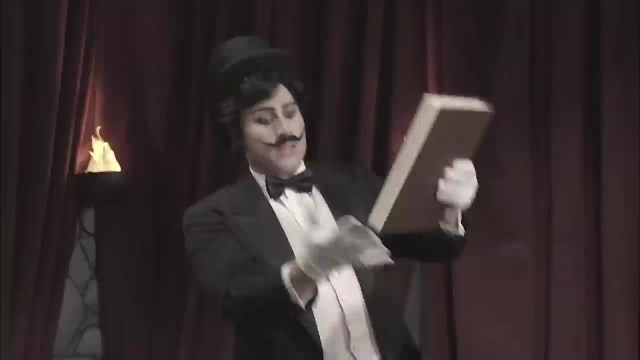 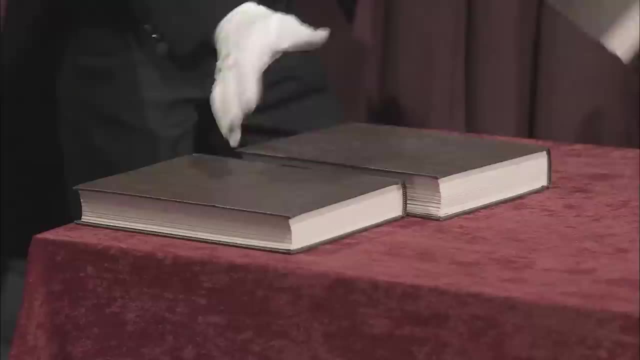 I will just get to it. Here is a book: Behold, And now feast your stupefaction as I produce another book. Ha-ha, And then two or three more times, behold. as I put as I, 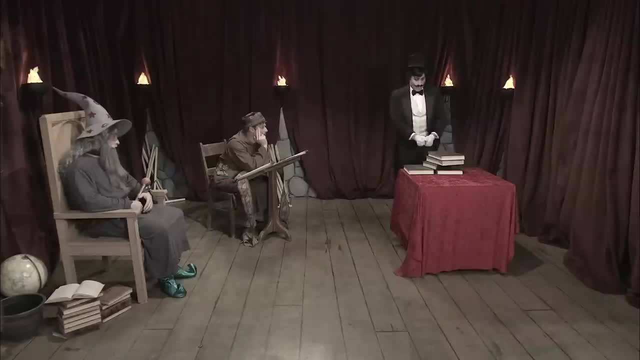 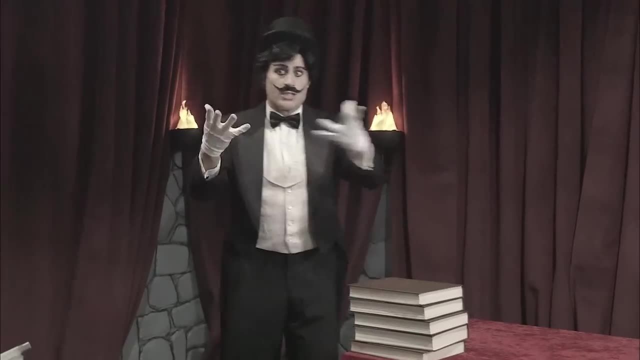 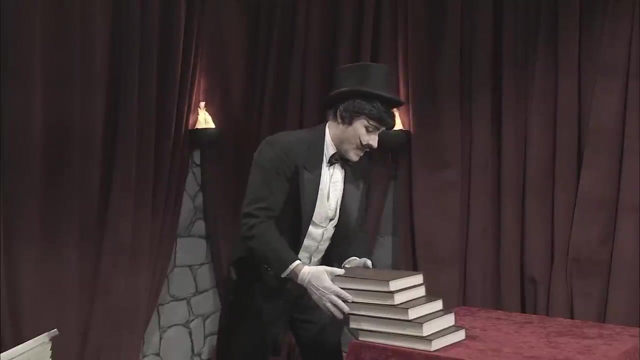 That's good Behold. And now look upon the wonderment as I stack these books on top of each other like this, And now feast more stupefaction as I I cleverly move the books off the table, And now, now comes the magic. 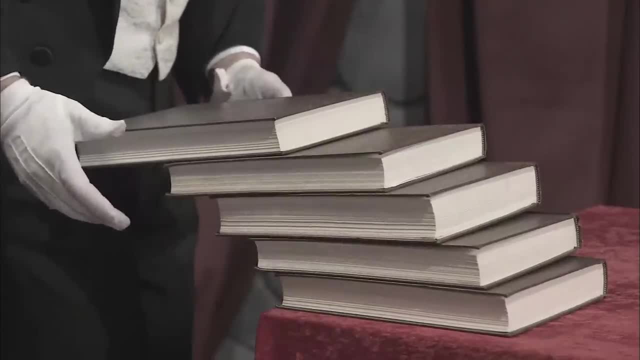 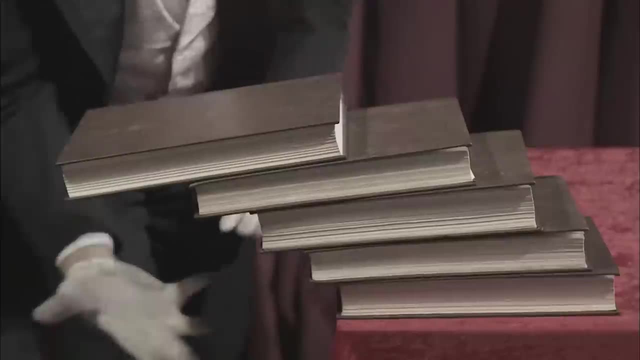 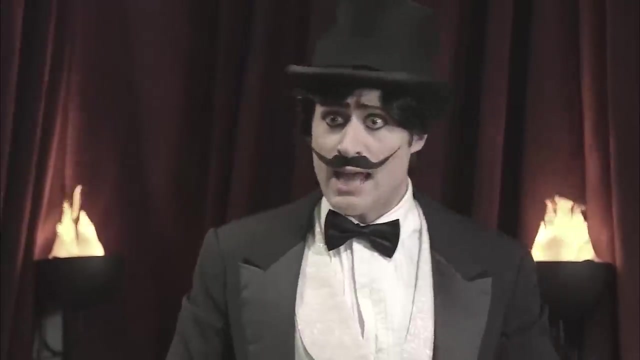 The magic word. Now I say the magic word, The magic word, And behold, the book is levitating. It is completely off the table. I have done it. Magic, No, No, Not magic, That's science. But the book is levitating. 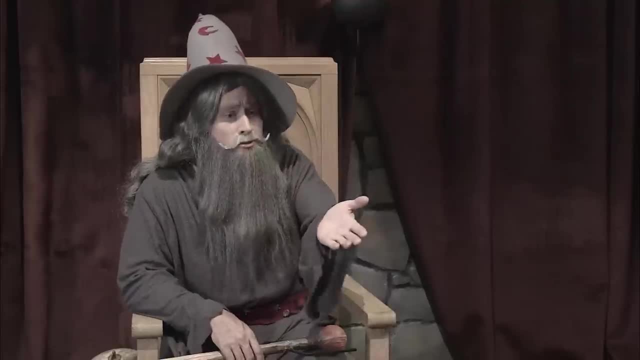 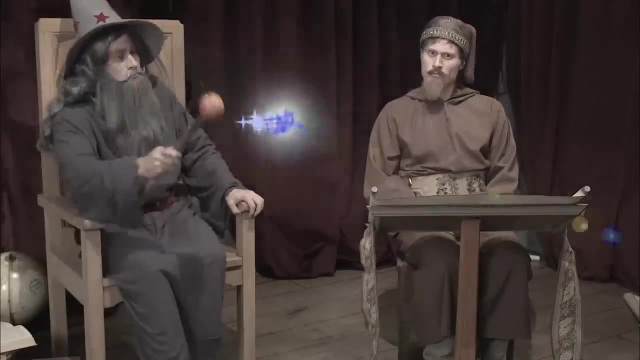 No, Look at it, It's not even touching the table. No, it's being supported by the books below. because of the center of mass Preposterous, I'm afraid it's very posterous. Each book is balanced on the one below. 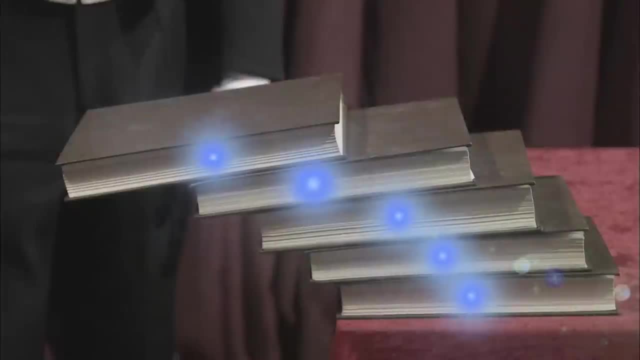 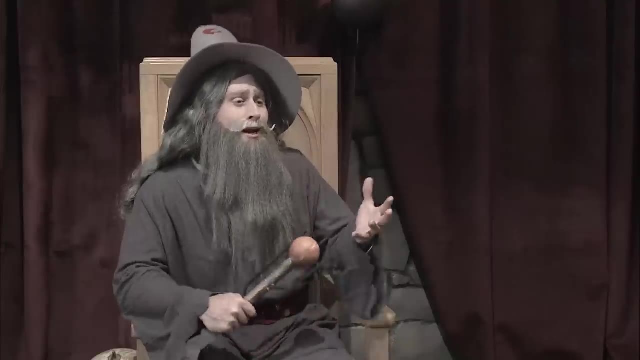 in a way that the center of mass is behind the edge of the book below And the entire stacked center of mass is behind the edge of the table. So it may look like magic but it's science, So I can't get into the Wizard Academy. 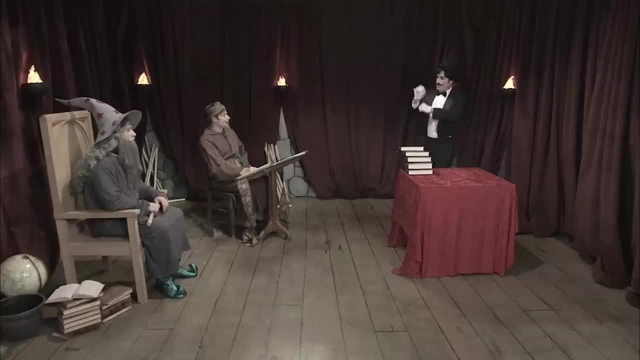 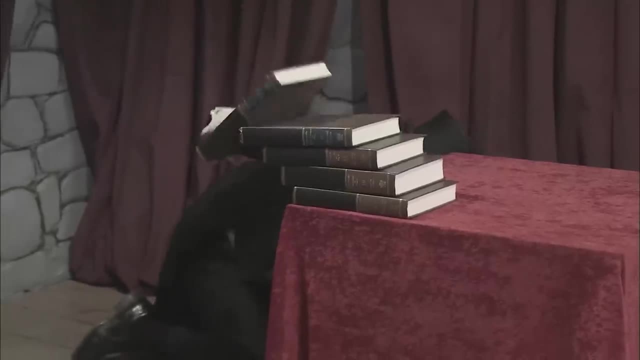 No, I'm afraid not. I, good Alakazam, you will rue the day that Overwhelmo did not. I will return and then you will see: Oh ow, This is a bike tire. It's pretty light. 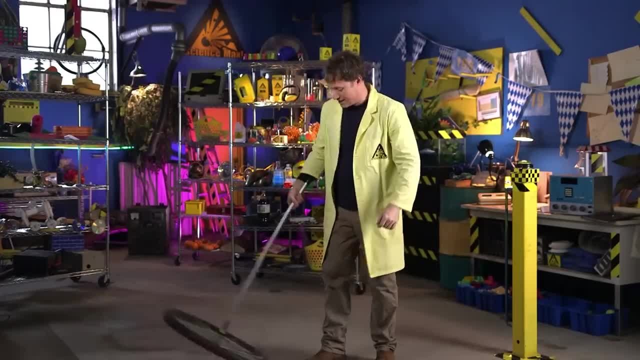 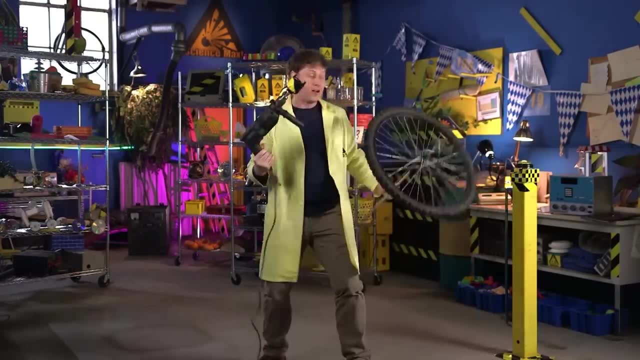 but I still can't hold it from the end of the pole like this with one hand. Nope, nope, But I can, if I get it spinning fast enough. I just use this drill and then I get. Okay, so this is gonna be awfully hard to do. 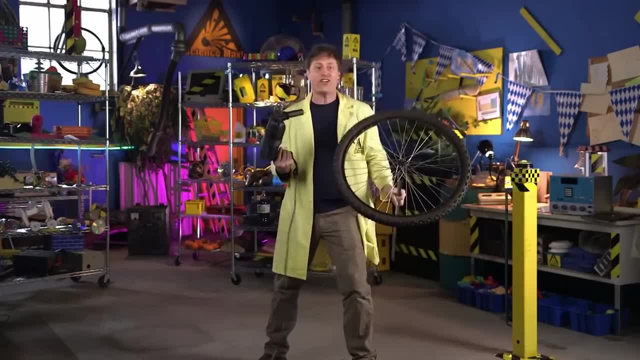 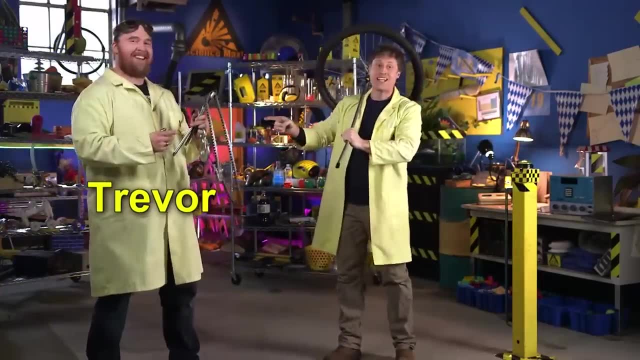 with one person. Uh Oh, This is the perfect opportunity to use the Trevor Button. Ha-ha, Trevor Button. Hey, Trevor from the Science Max Build Team. Uh, what are you doing, Maxing this out? Oh, right on. 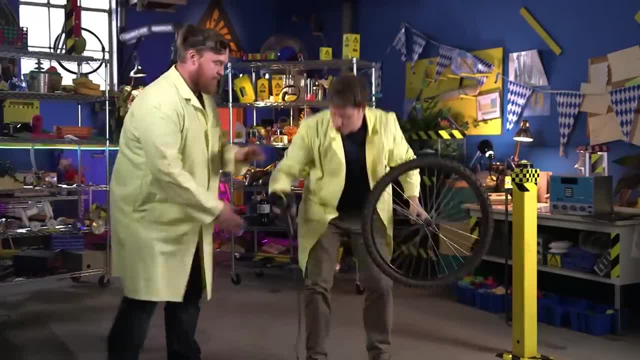 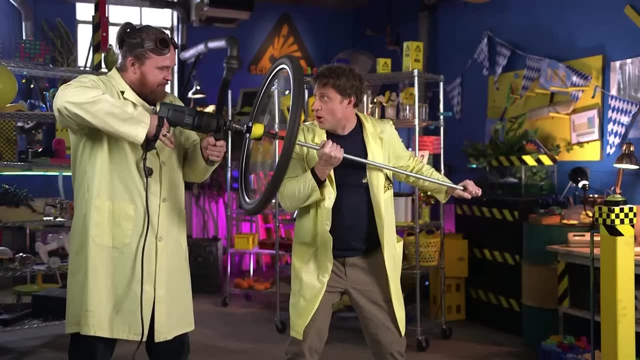 Can you give me a hand for a second? Sure, Awesome, Okay, so you take this, this drill, and we're gonna get this wheel spinning really fast. Okay, I don't know if it's um, No, No, I don't wanna know. 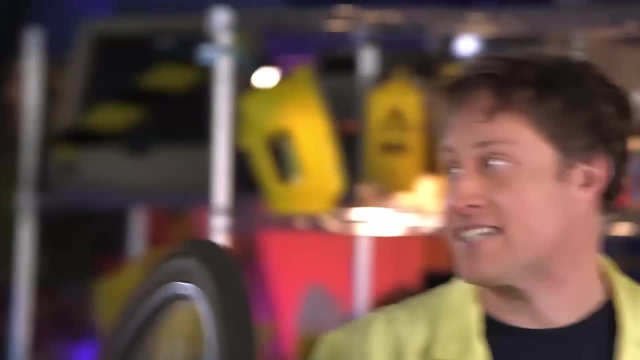 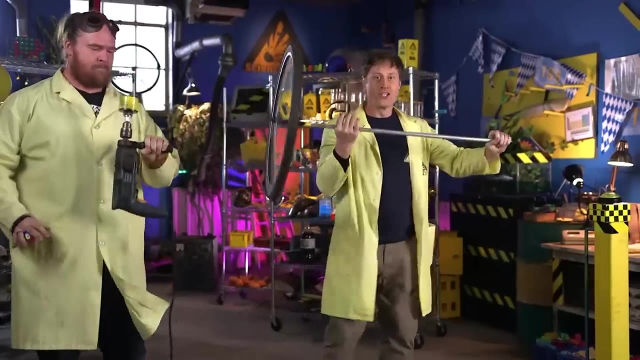 I don't know if I remembered to. No, it's fine, Max it out. We gotta max it out, Oh, Ah-ha-ha-ha-ha-ha. So Because it's spinning, I can hold this heavy weight in the air. 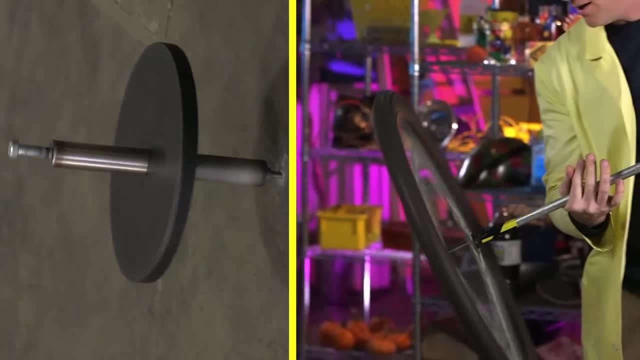 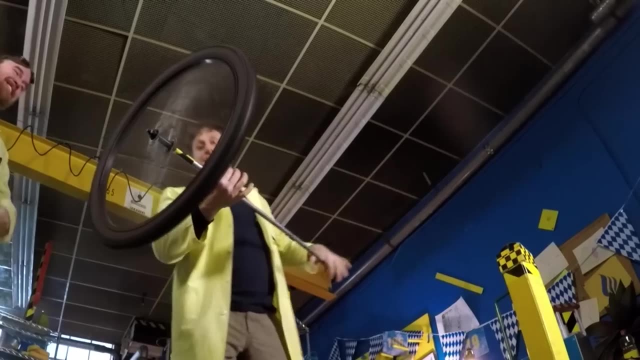 How is this possible? Because the wheel is basically a top. The forces that prevent a top tipping- angular momentum- are still working here. This angular momentum resists a change in direction this way, which is how gravity would want it to tip. 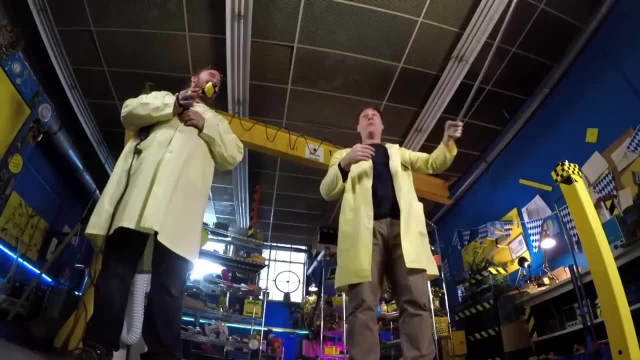 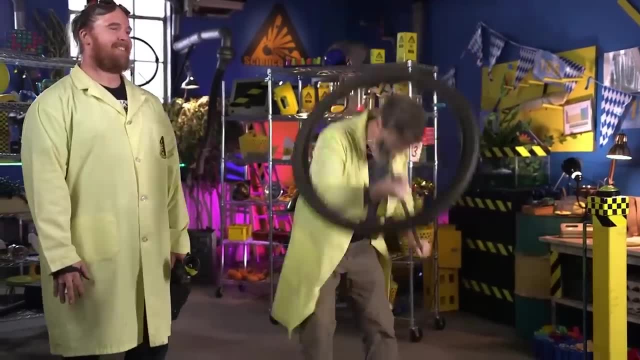 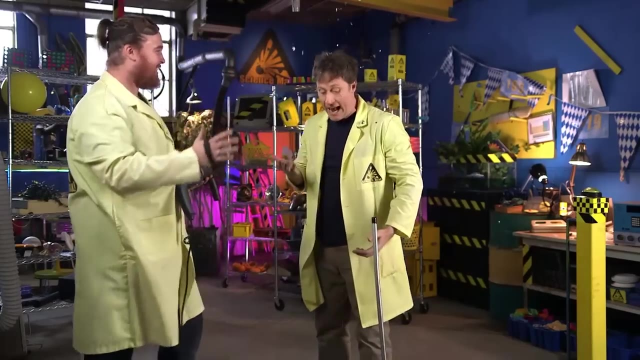 Interestingly, these same forces also keep it spinning around me in a circle, So I can lift a heavy weight in the air just by spinning it. Awesome max-out experiment, Trevor. Yeah, What was that? It's my science confetti high-five I just made. 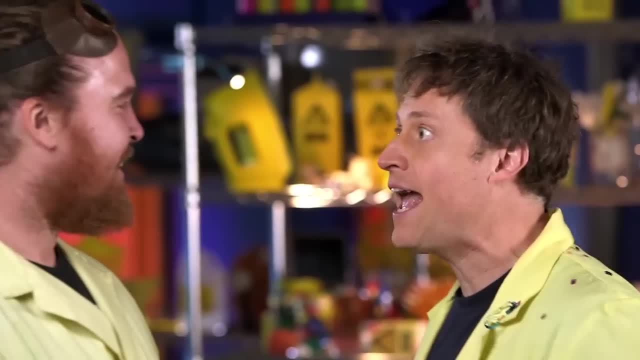 Well, you know what we should do, What We should max it out. Yeah, we can make a giant one and then a whole bunch of confetti in it, and then people like jump up and do more confetti. that would come out right. 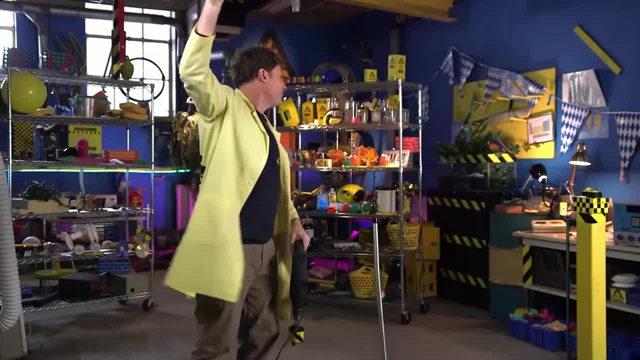 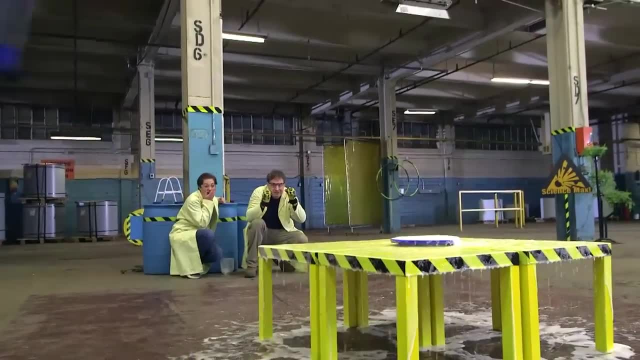 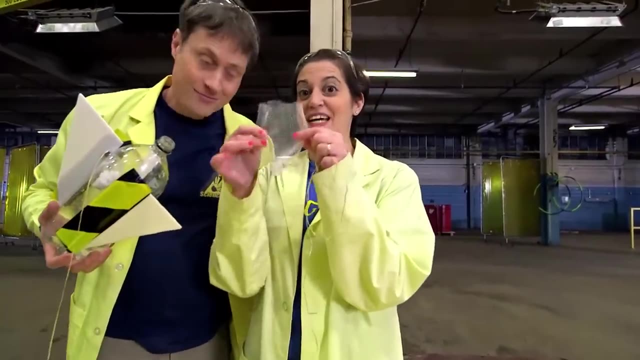 And then? so what would happen is there would be all this Trevor. Our maxed-out rocket worked great. Whoo Now to make it look more like a rocket. So we have a mesh bag here to put the antacid in, Right. 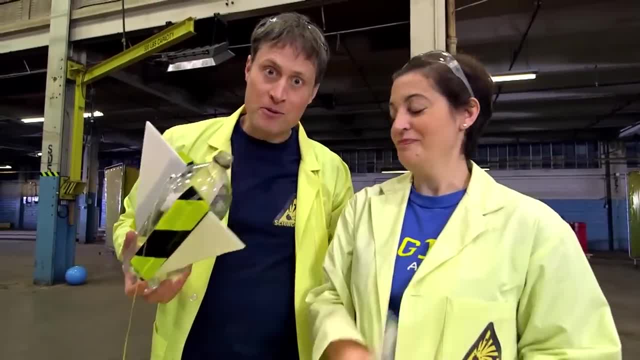 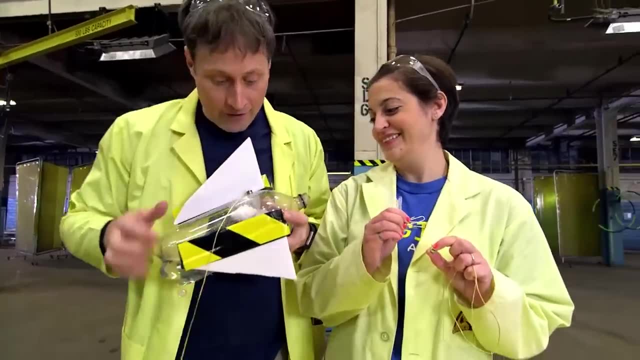 And we have some paper clips attached to it. And what are the paper clips for? Well, Phil, we have a magnet, Ah, And so the magnet sticks to the paper clip, And so that's what we have here. You see, the bag is full of the antacid tablets. 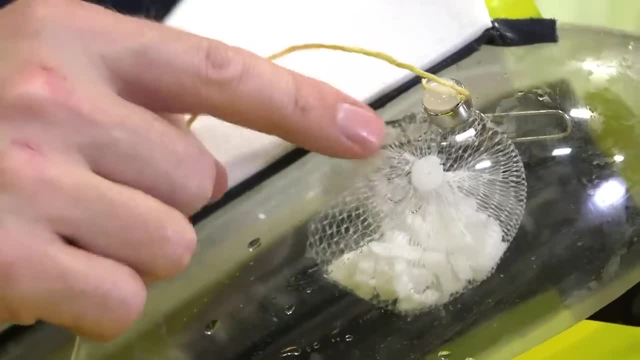 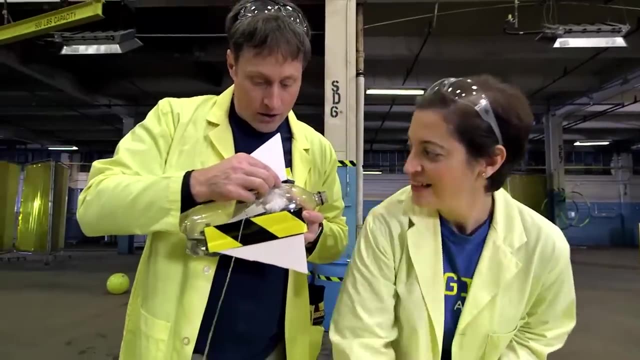 which we put through the mouth of the bottle, and the magnet is holding the paper clips on the other side of the plastic So we can sort of move it along, So we can start with the bag over here where the water's down there. 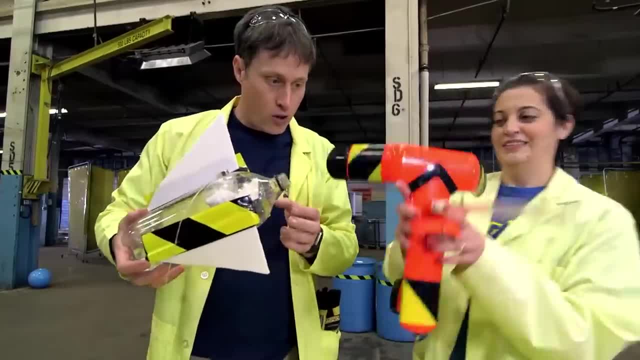 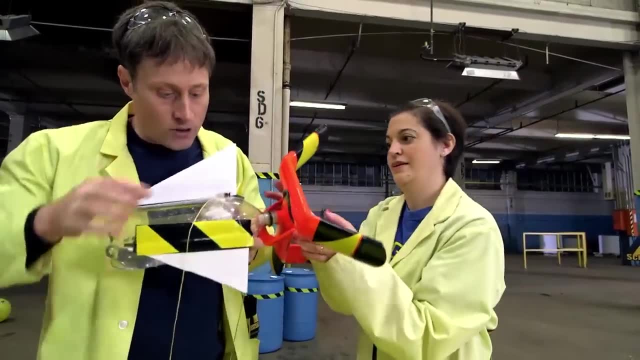 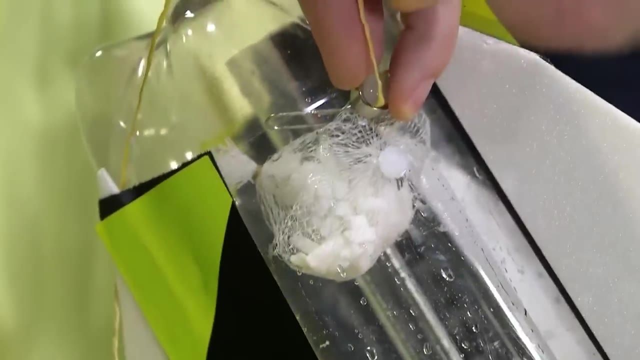 but now we attach the launcher, like. so. All this effort is to keep the reaction from happening until the bottle's on the launcher and we're ready to go. And then, as we pull the bottle over, we bring the bag up this side, and there the water and the antacid have never touched. 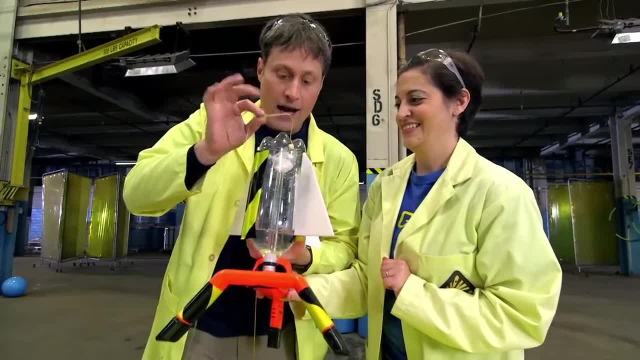 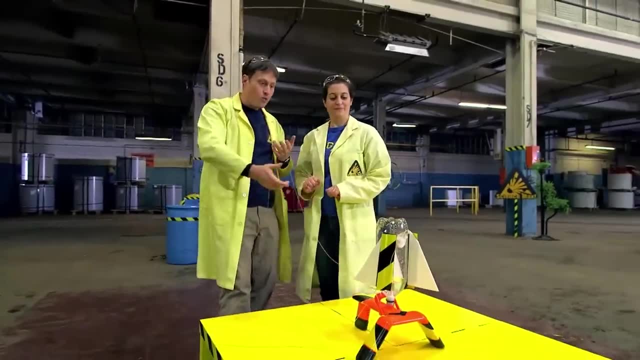 No reaction. All you need to do now is just we pull this magnet away and the bag will fall into the water, And then we will have the launcher down here and we pull the release and the rocket will go. We add some weight to the launcher to help keep it in place. 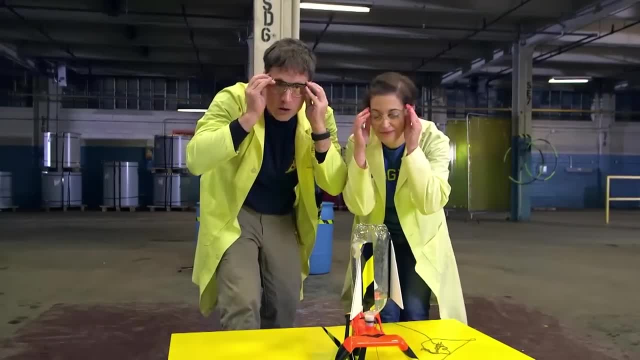 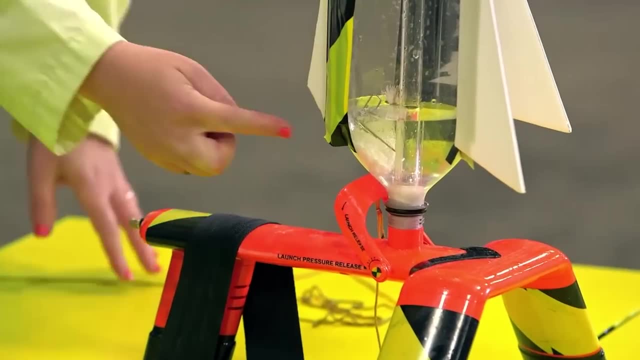 Okay, right, wait, glasses Safety first, Okay, ready. And then we pull the string with the magnet That drops the bag of antacid tablets in the water and starts the chemical reaction, Because we have a latch holding the bottle down. 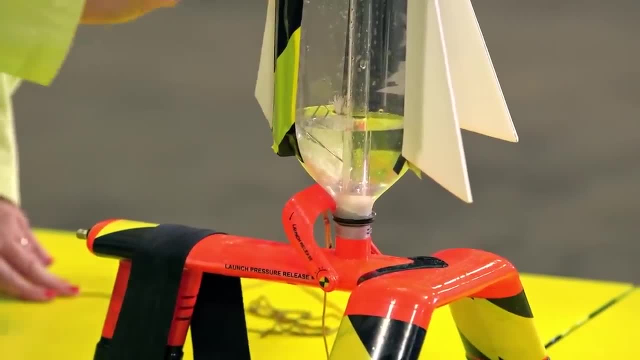 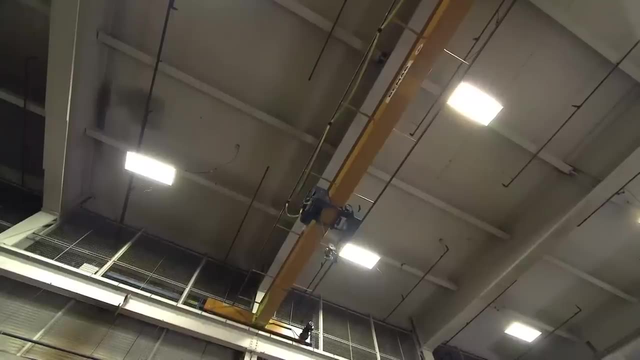 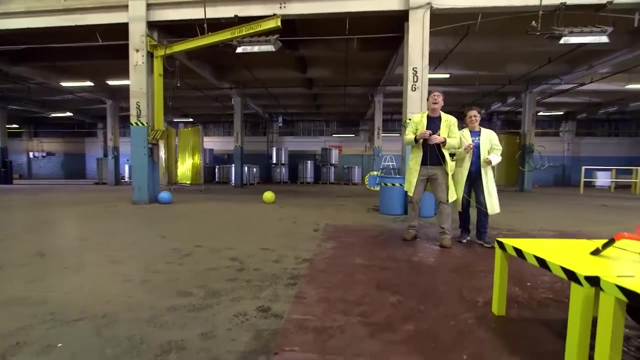 we can wait until the chemical reaction happens fully and there's a lot of gas pressure in the rocket before Three two one, Three two one Run Whoo. Oh, That worked. Yeah, it hit the ceiling. 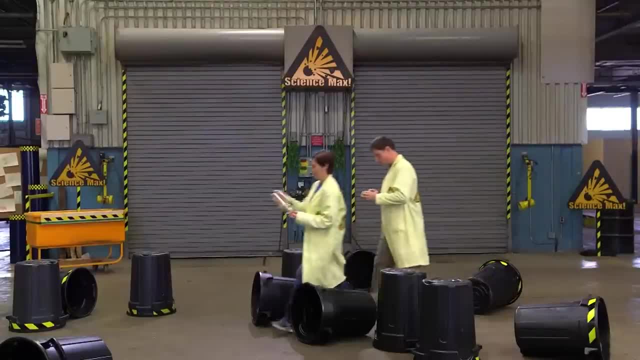 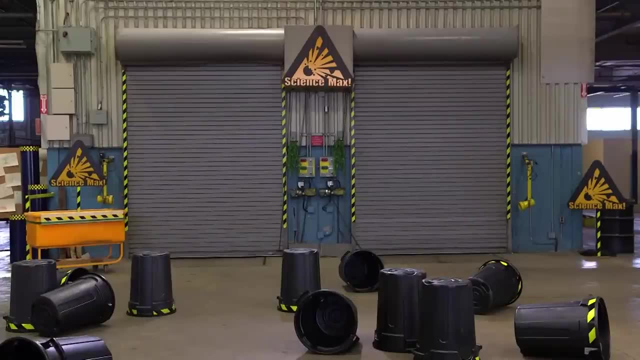 Uh, I think we need to do this outside. Yeah, I think we definitely have to do it outside. All right, totally great, Weird. Anyway, I was saying we should put three or four of Three, two, one go. 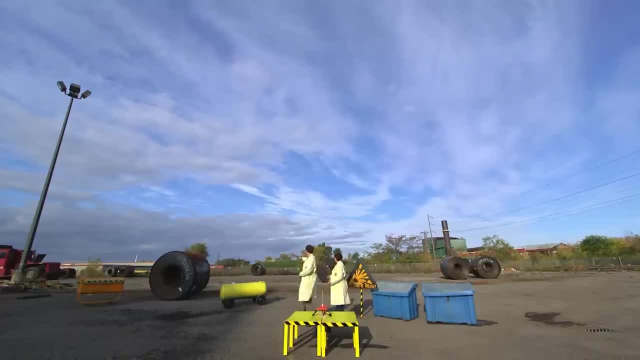 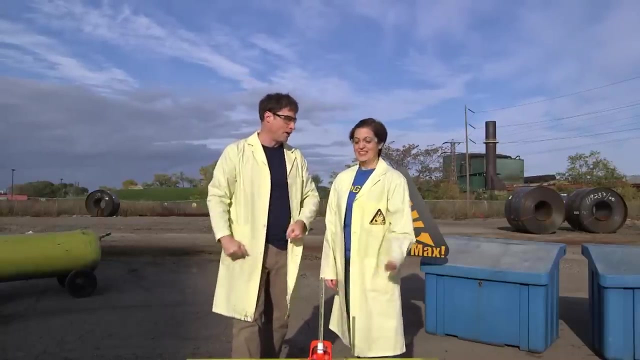 Whoo, There it is. Oh my gosh. Yeah, We tried it outside and it worked great. The only thing left was to max it out even more. So larger chamber, Yep, more antacid, More antacid, more air, more water. 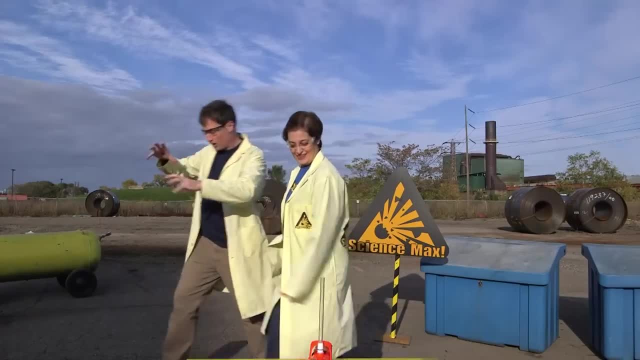 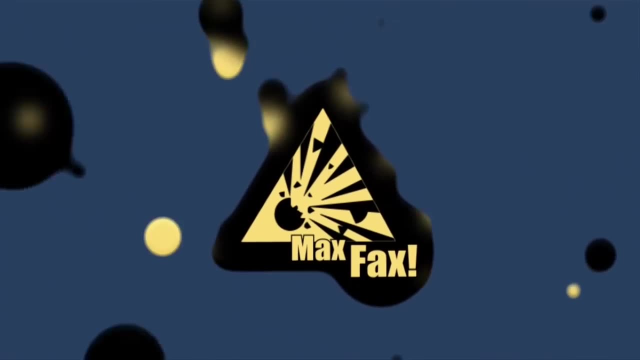 Absolutely Bigger rocket. Okay, so you know what. I know how to splice two bottles together and we can increase the size of the chamber. All right, Let's go. This is sodium acetate. How do you get sodium acetate? 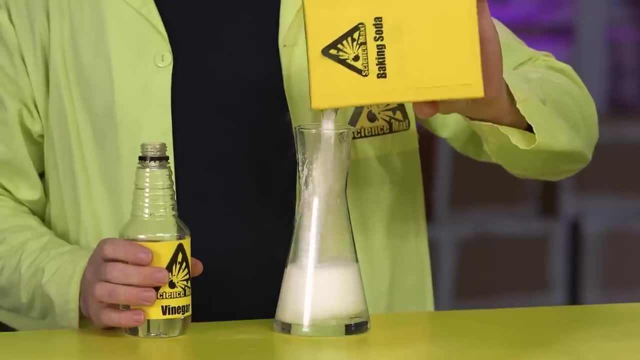 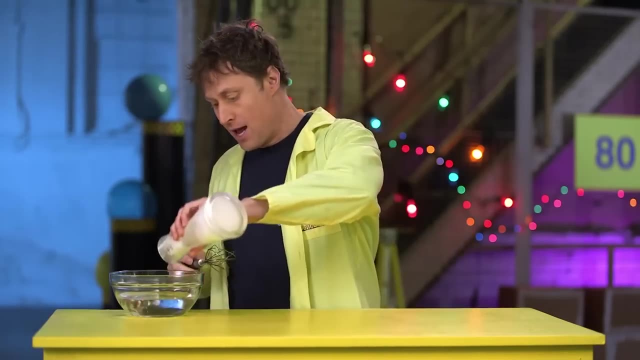 Well, when you do a vinegar and baking soda reaction, what you have left once the reaction is finished is sodium acetate. It's a crystal and you can do something fun with it. that may seem familiar. You make a supersaturated solution of sodium acetate. 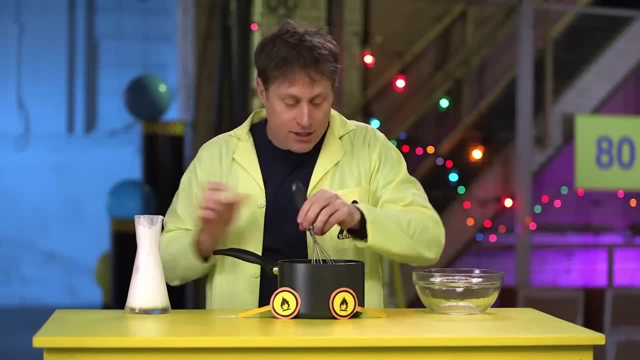 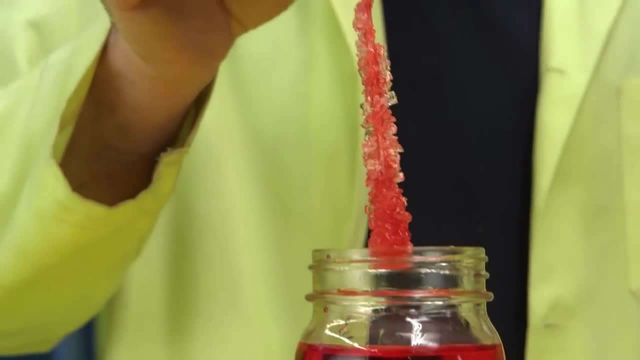 by heating water and dissolving as much as you can, and then, when it cools, you can get the crystals to reform. Now, if you did this with show-off, you could make a sugar pop, which we've done before. If you do it with salt, you could make a salt pop. 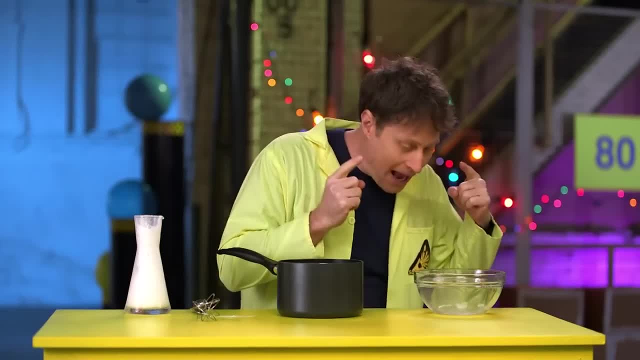 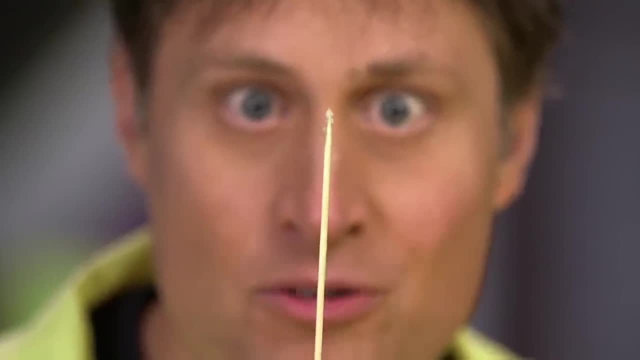 which is less appealing. And if you do it with sodium acetate, you can do this Just like with the sugar pop. all it needs is a seed crystal to get the crystals to reform, But unlike sugar, which takes a few days. 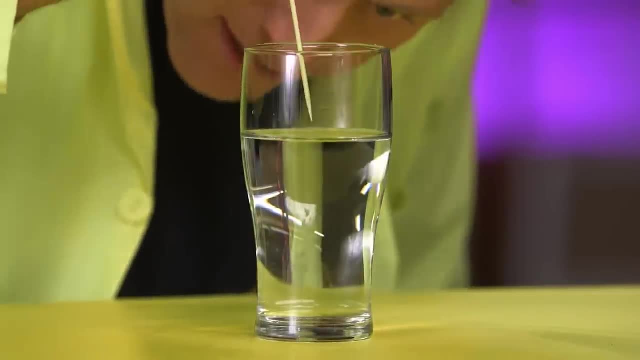 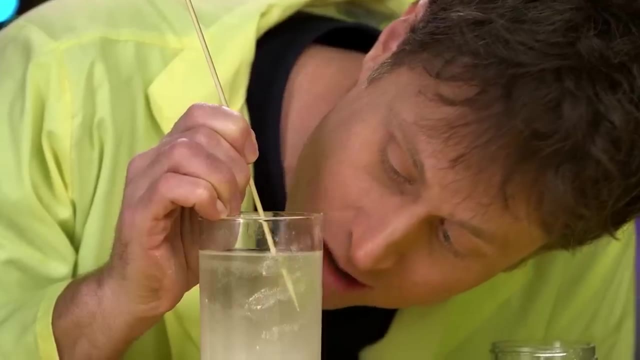 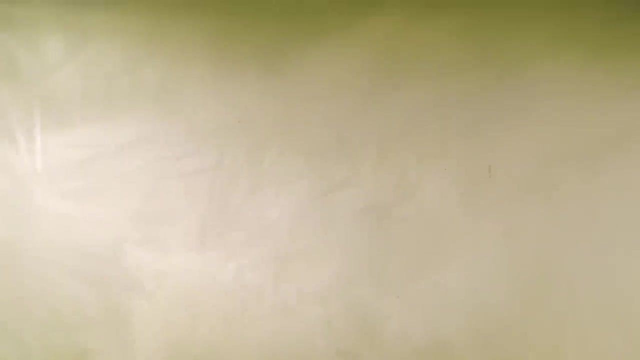 sodium acetate recrystallizes right before your eyes. Because we heated the water, it allowed more crystals to dissolve in it, Ooh- But then it cooled down afterward. There's more crystals sitting around in this water than there should be at this temperature. 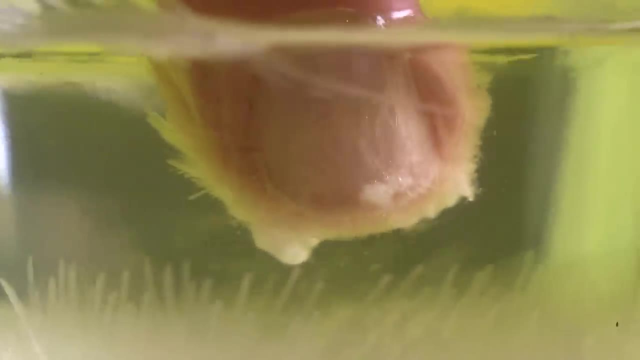 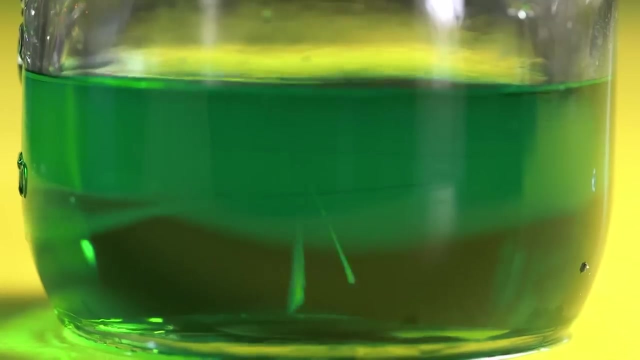 They want to turn back into crystals, and all they need is something to start them going. I've colored this one green because I don't know science. Maybe it'll look cool. A tiny crystal on the end of the stick is all we need to start the reaction happening. 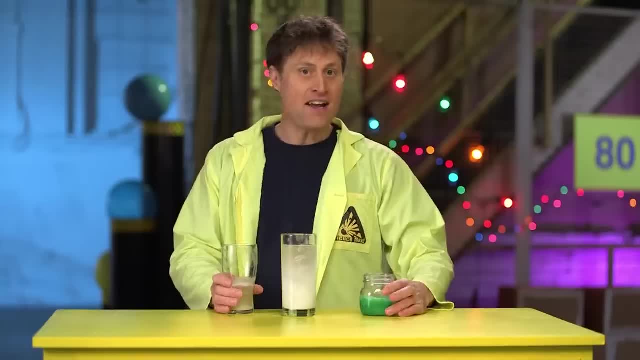 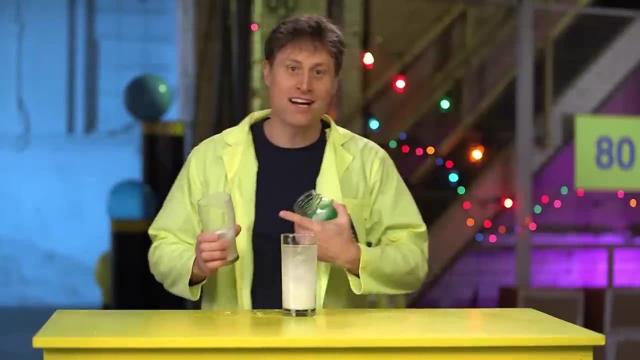 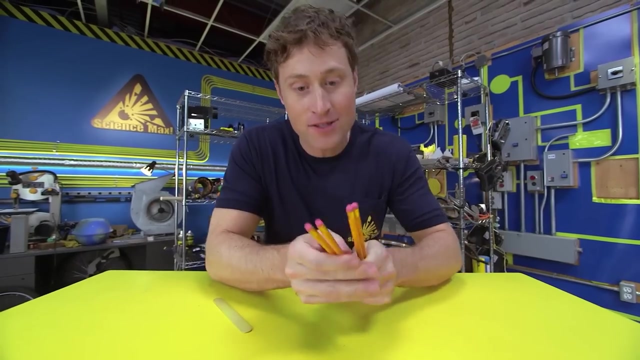 Whoa, Wow, And there you go. sodium acetate. Ooh, That one wasn't done yet. All right, let's build our catapult. The first step: take four pencils and stick your Popsicle stick in between, so you have two on the top and two on the bottom. 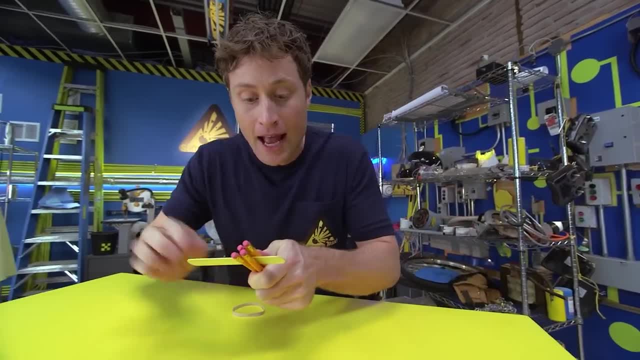 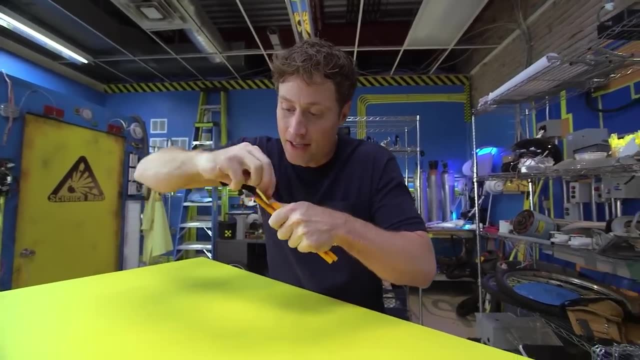 And then use your elastic to go around and around and around. That's why I like building things with elastics: because it makes it very fast to tie things together, Because once you go around and you have it nice and tight, you just pop it over the end and voodoo. 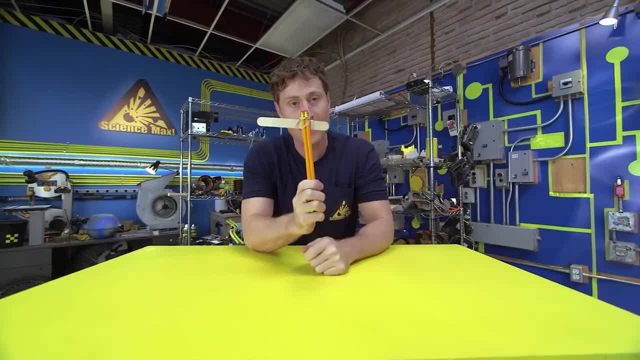 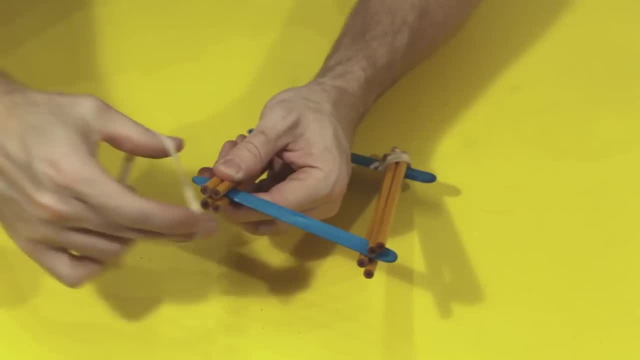 And that's it. All. right, let's go, Let's go. Voila, it stays together. And that is how you start making your frame. Put more pencils on that side and another Popsicle stick on the other end, held on at the corners with more elastics. 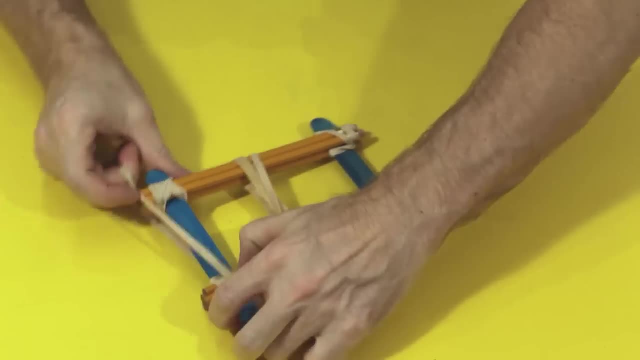 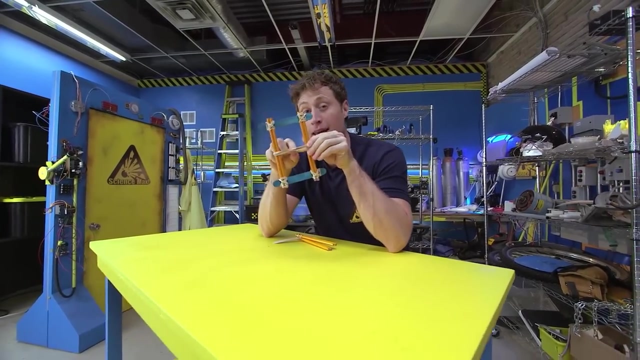 Then take even more elastics and put them right around the middle until you get this. I've added a few more elastics around the middle here, and that is where we're going to get all of our elastic force. I think I have six. 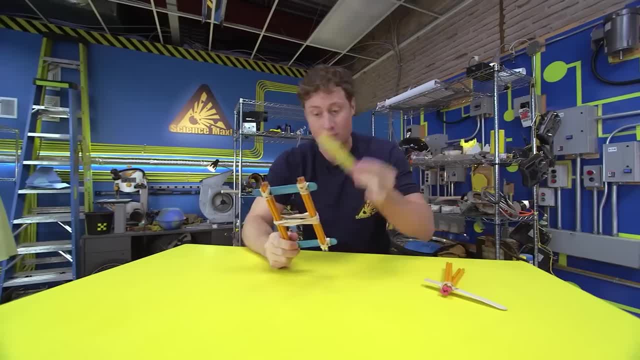 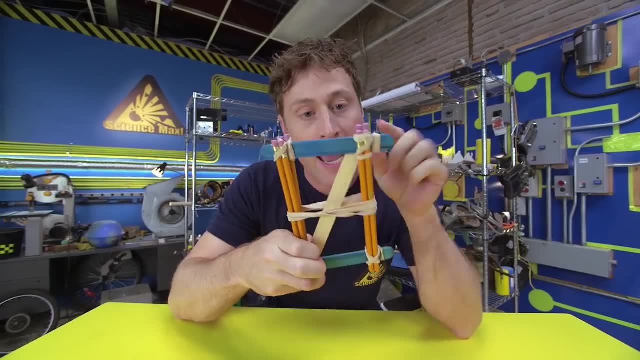 The more you use, the better it's going to work. Take your Popsicle stick, stick in between the elastics and then start spinning it around. Here's the reason I use pencils and Popsicle sticks is because the pencils are a little bit longer, which. 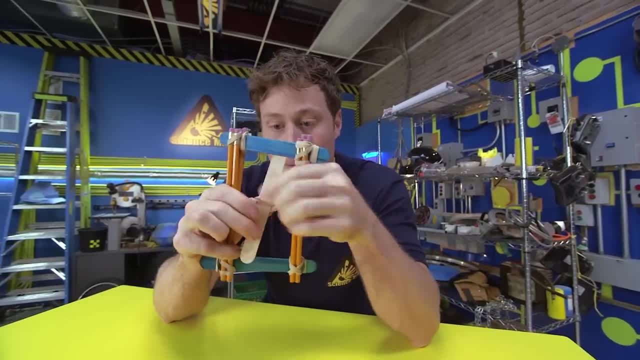 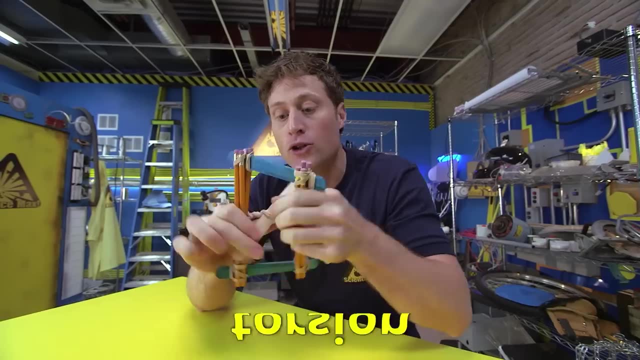 allows you to twist the Popsicle, stick around in the middle and build up the elastic force. Now, because I'm twisting, the elastic force we're using here is called torsion or twisting force, When you feel you have enough torsion. 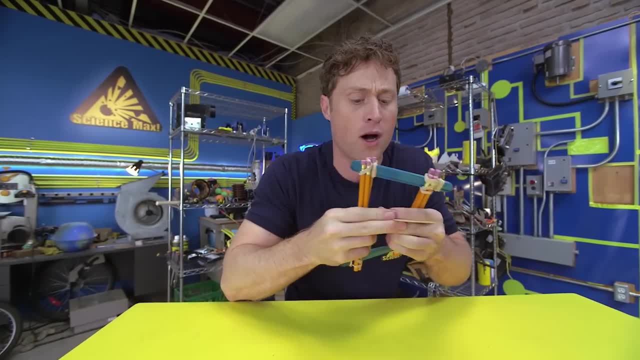 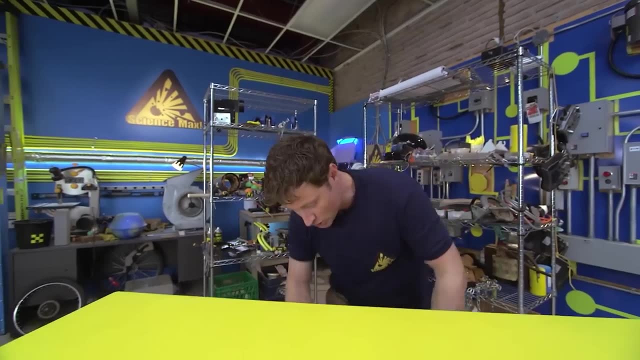 pull your Popsicle stick down a little bit so it won't unwind on you, And you'll see that you have all kinds of elastics and all kinds of elastic energy. Then take your spoon and stick it on the Popsicle stick. 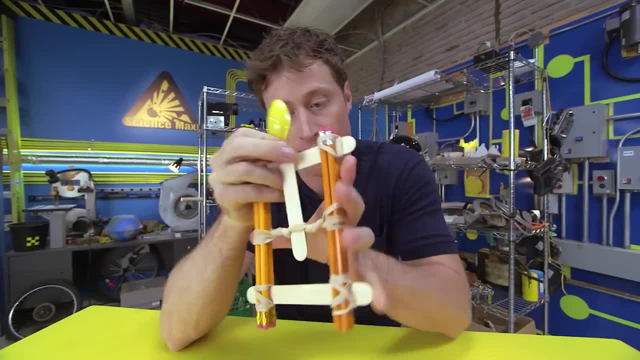 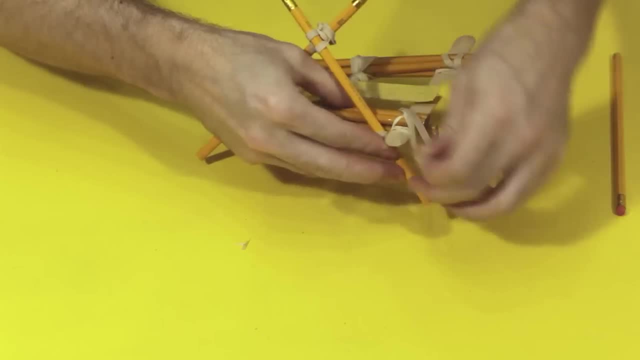 And you can also break off the Popsicle stick if you want to make sure it's the right length And it works like that. To make the frame, you just need more pencils and elastics. The trick is to make a triangle with two pencils. 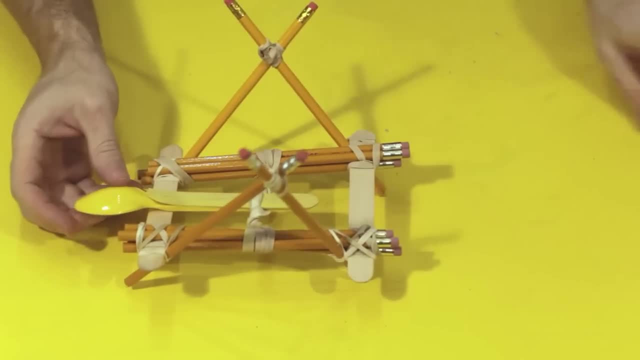 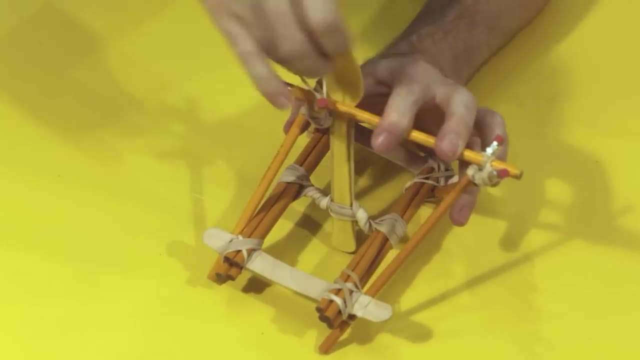 attached to your frame. They should stick up right where your catapult arm would be fully upright. Then take a final pencil and put it across the top. Don't forget to pull the arm back before you put the pencil across, otherwise it'll end up on the wrong side. 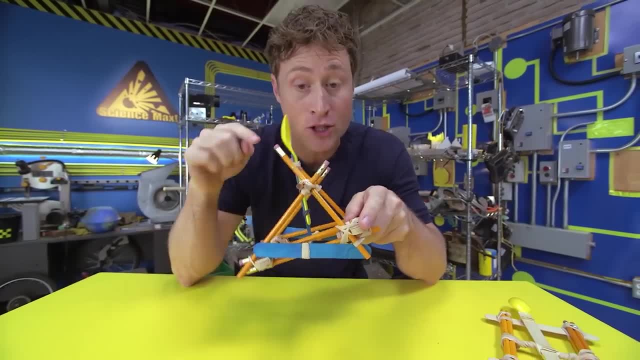 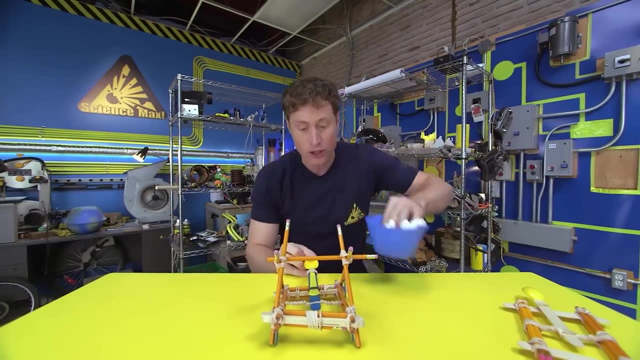 Now, this is very complicated and I went pretty fast. So if you want the step-by-step instructions on exactly how to build this, go to our website And there you go, a catapult of your very own that you can use to knock down very small castle walls. 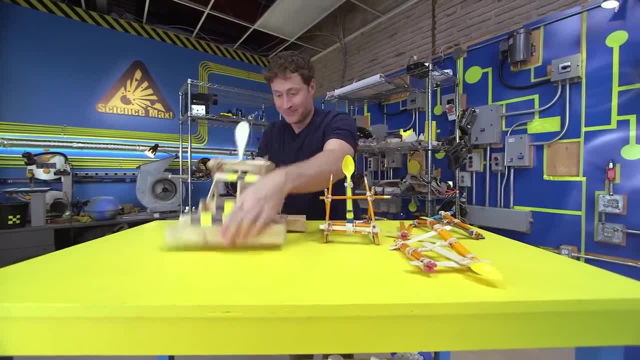 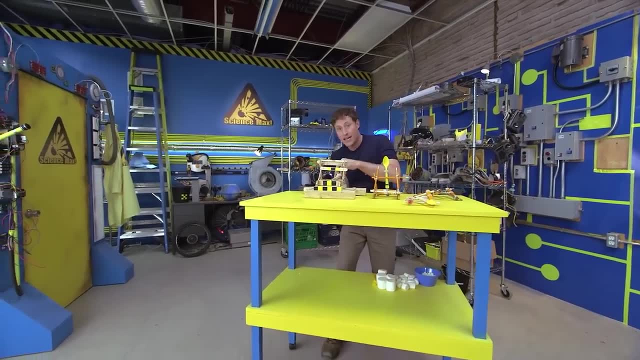 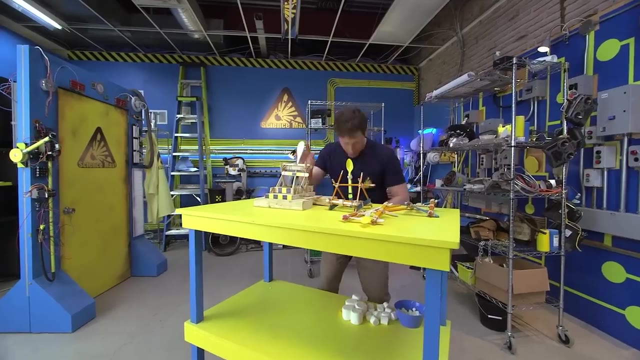 I've also built a larger catapult using all of the same principles. Pretty good, huh. I've got a longer arm, which means I can throw marshmallows even further. Whoa, Or I can throw larger marshmallows, Or I can throw very large marshmallows. 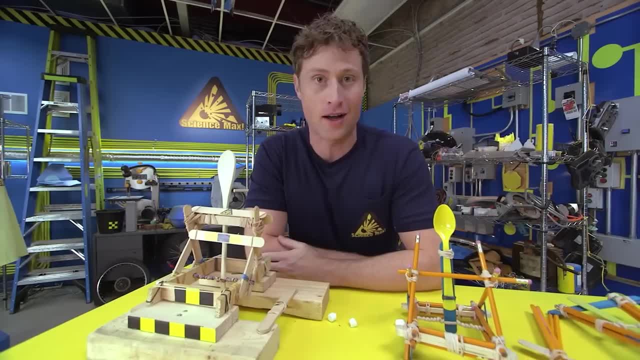 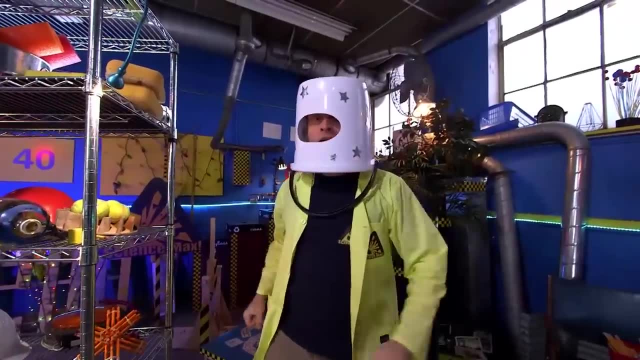 Now I know what you're thinking. You're thinking, Phil: is that the largest catapult you're going to make? Well, of course not. This is Science Max, experiments at large. OK, Science Maximites: prepare to hurtle. 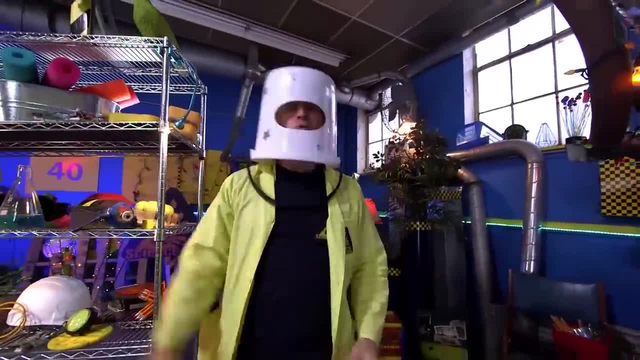 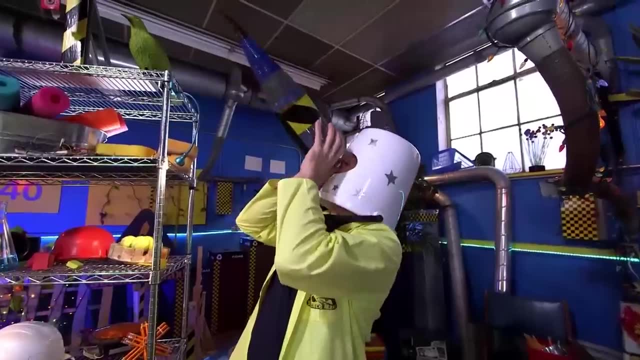 through the cosmos. I am Captain Phil, and today we're going to be building rockets on Science Max. Now, we've built rockets before like this one powered by air pressure And this one stomp rockets, which were also technically 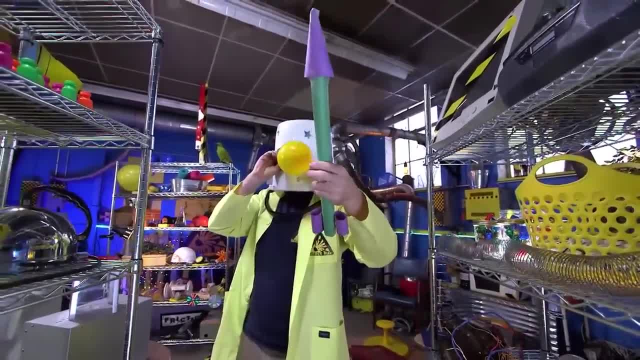 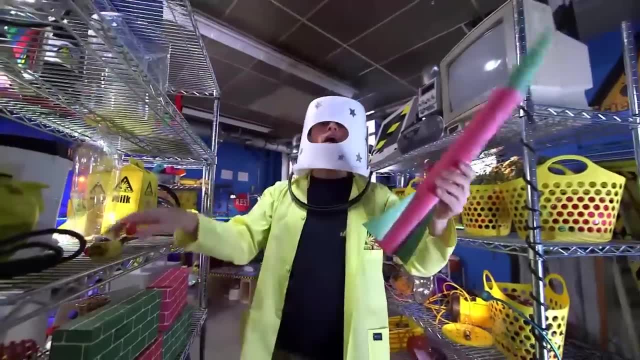 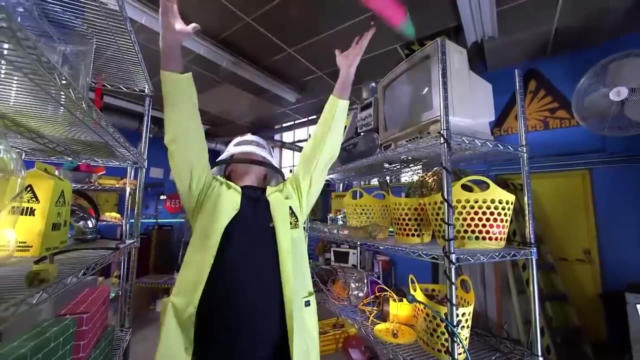 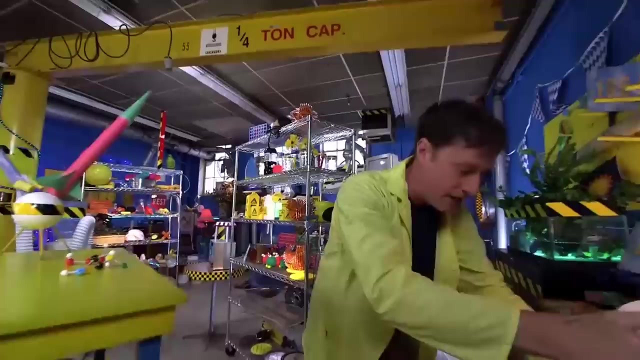 powered by air pressure: Air pressure rocket. But today, Science Maximites, we are going to be building rockets powered by chemistry, chemical powered rockets away. OK, I promise it'll be more exciting than that, Because today, Science Maximites, we. 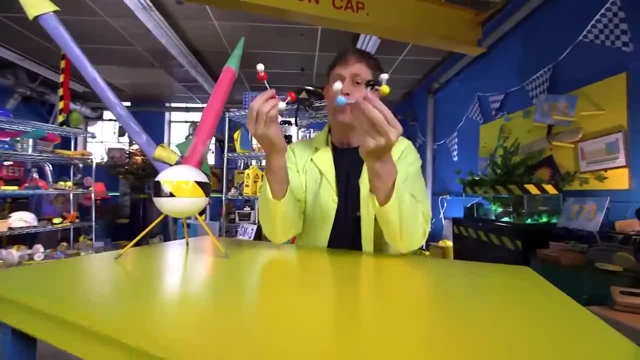 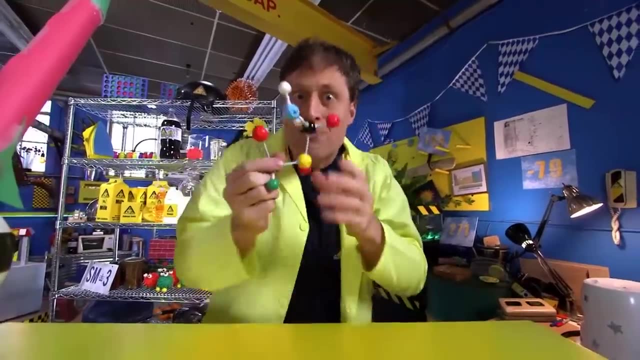 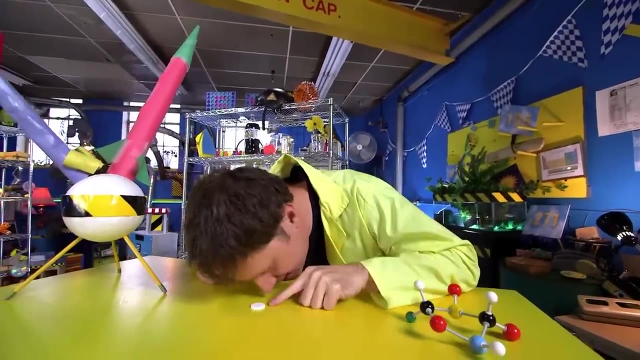 are going to be looking at chemistry. Chemistry is when two molecules combine to make another molecule, like magic Ooh. So let's take a look at what will be powering our chemical rocket. This- It's an antacid tablet. When you put an antacid tablet in water, 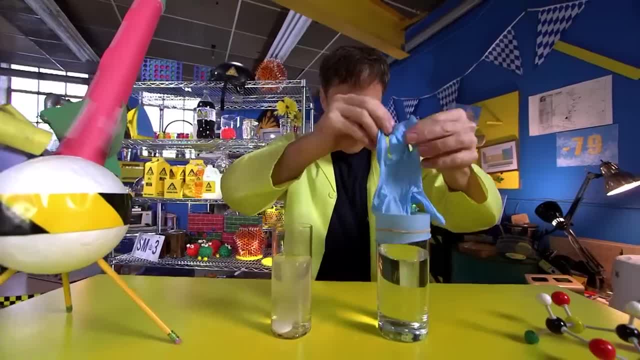 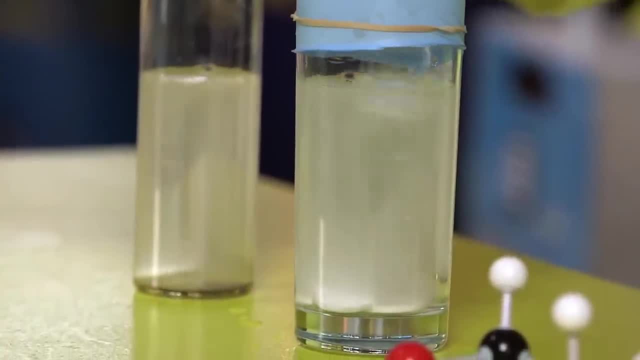 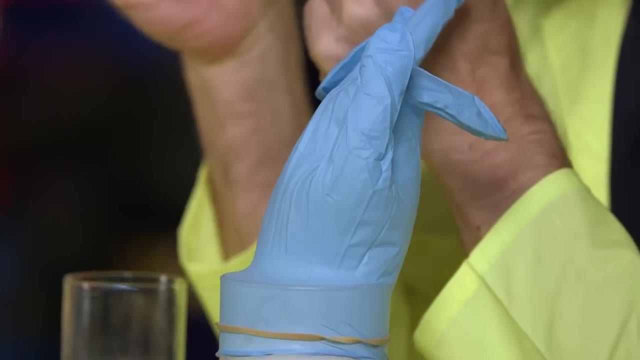 it makes little bubbles of carbon dioxide gas. This happens because of a reaction between two kinds of molecules called acids and bases, like vinegar and baking soda, but all contained in a small package that won't start working until you put it in water. If we contain the reaction, the carbon dioxide gas builds up. 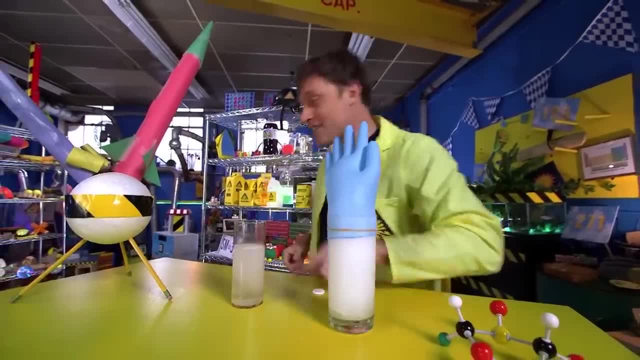 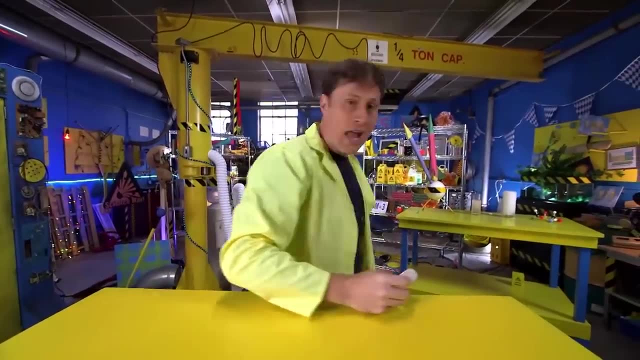 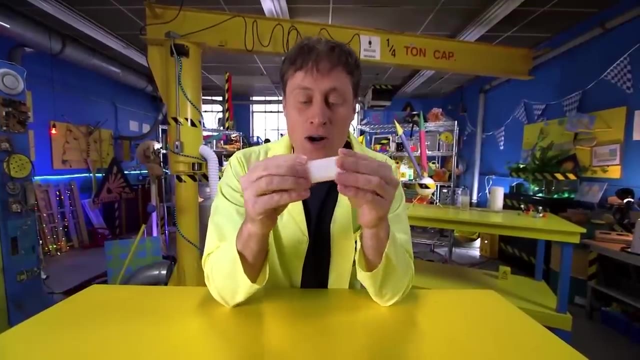 and creates pressure. High five for science. All right, so let's look at our chemical powered rocket. What you need is one of these. This is a film canister, And ask your parents what that actually means, because they're not used for holding film anymore. 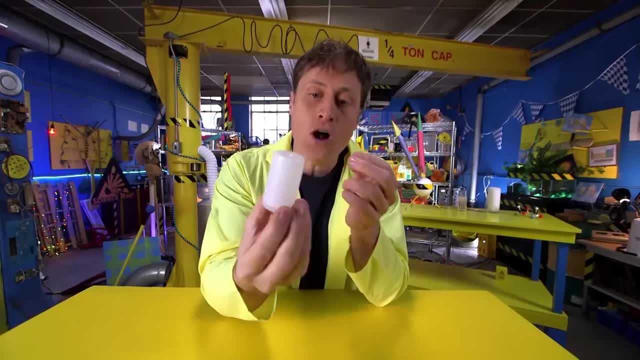 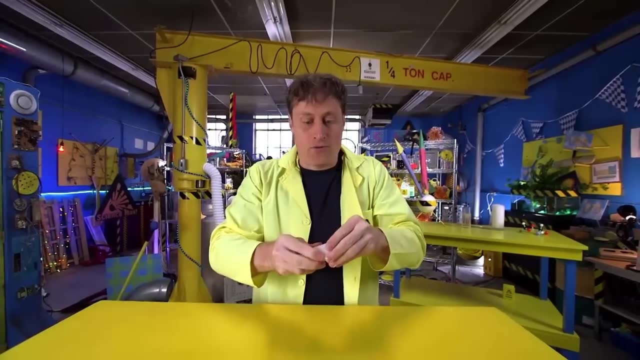 You can get these at craft stores, though, to hold paint or little things, But really all you need is a plastic container with a good lid that snaps on, nice and tight and keeps the air in. And then, of course, what you need. 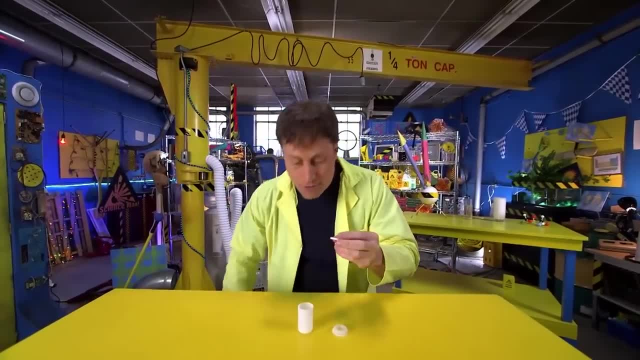 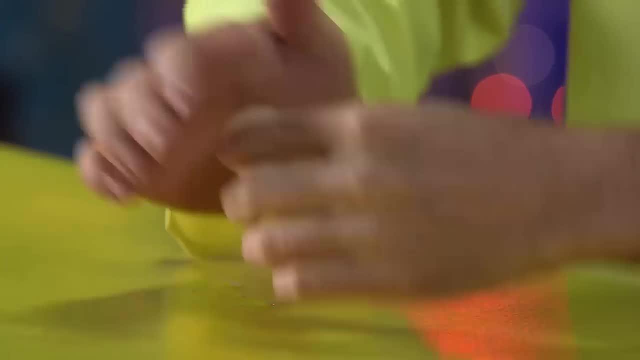 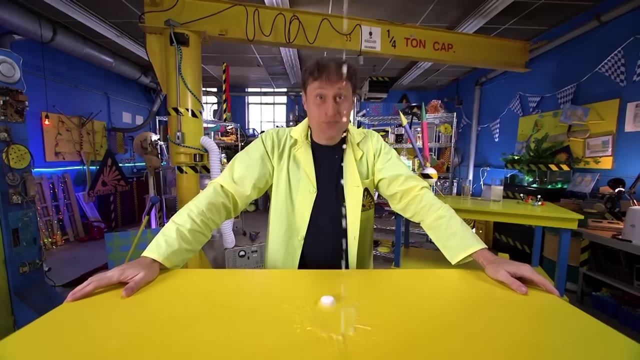 are your antacid tablets and a little bit of water. So pour in some water and then put in your antacid tablet and snap the lid on, flip it over and wait for the carbon dioxide gas to build up, which will build up pressure, which will 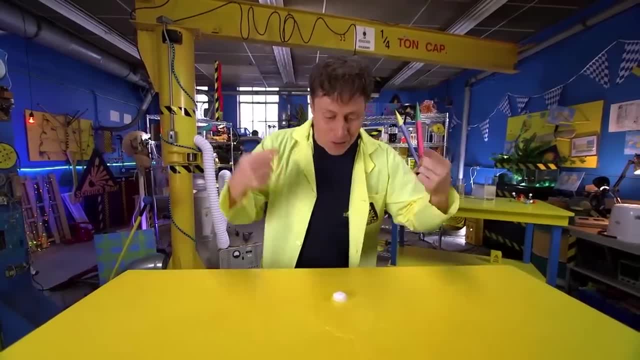 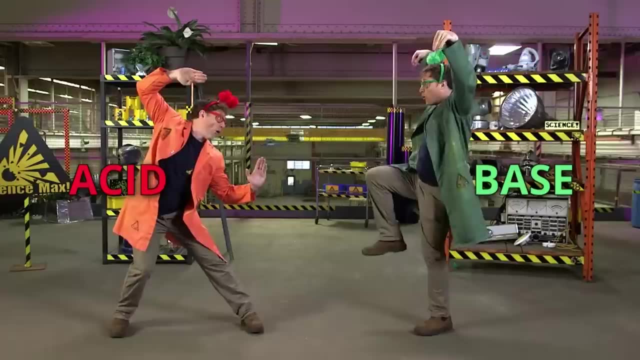 launch your rocket, Ha ha. So there you go: a chemical powered rocket. I'm an acid and I'm a base, and we are enemies. Whoa Well, we're not really enemies. Yeah, that's true. It's all about how we react chemically. 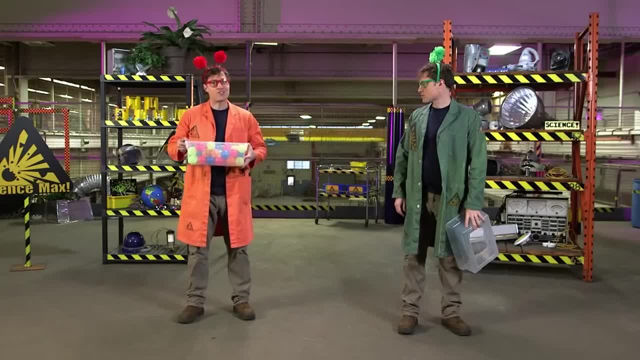 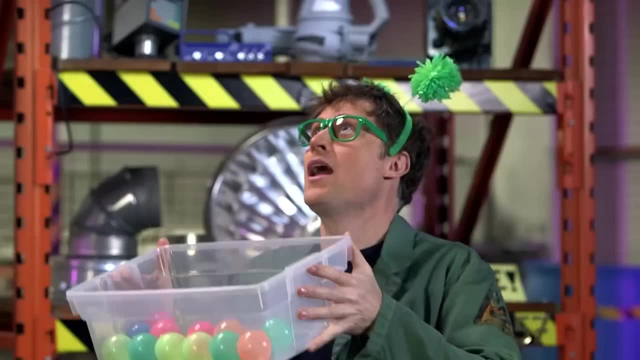 You see, as an acid I really want to give back. I want to take the protons away. Protons, Who needs your protons? Get your protons here? Protons, I got more than I want. I don't need them anymore. 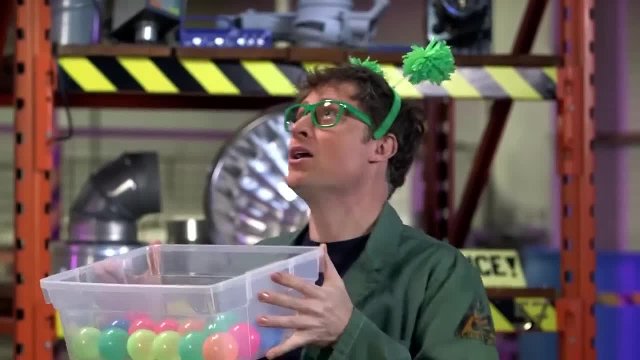 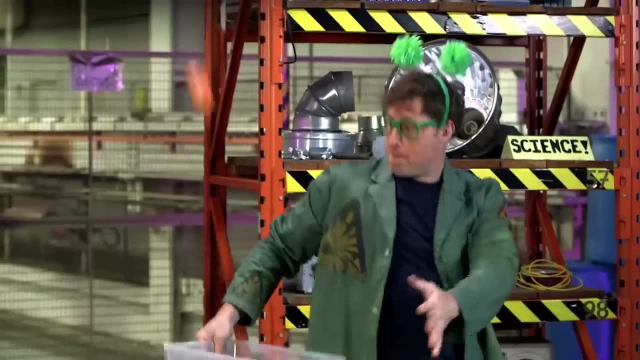 And bases. we need protons. We'll do anything to get them Protons. are you giving protons away? I'll take some. I'll take some protons. You think that when you get these two together you'd have some pretty great chemistry? 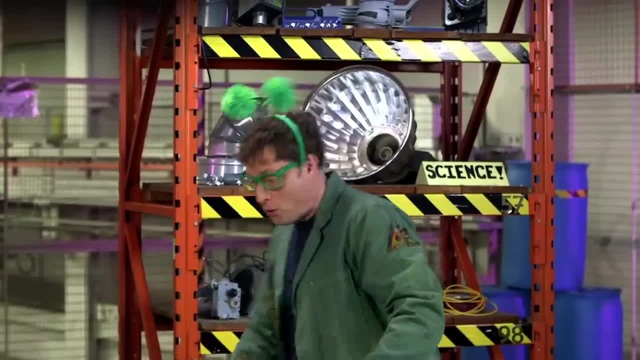 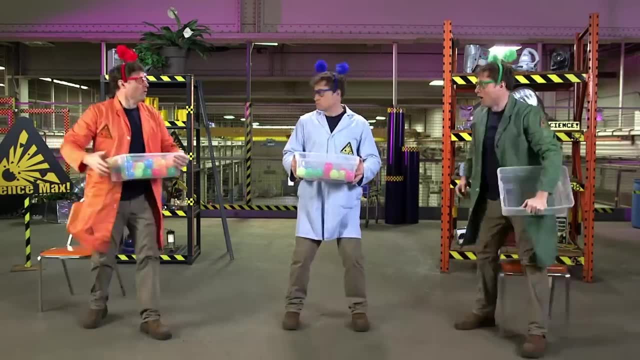 But the truth is, when they're together, they often don't react Whoa. That is until water gets involved. Once you have water, acids and bases react Whoa. Here, take some protons. All your bases belong to us. 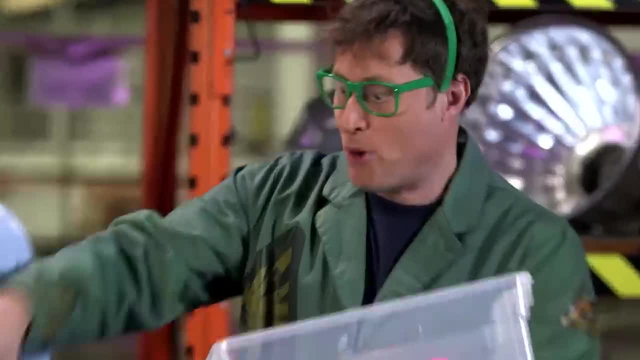 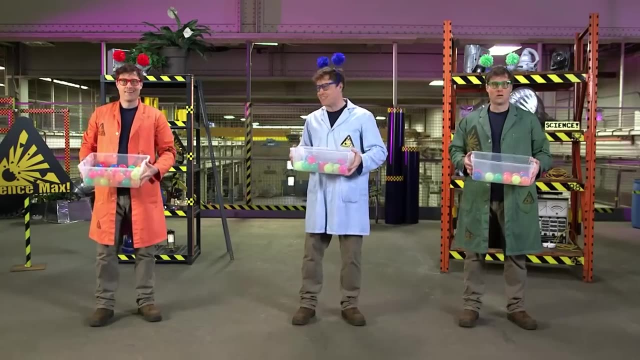 Here you go. Take some protons. I don't need any more, I want more. I want more protons. Water is a solvent allowing the chemical reactions to take place. Depending on the strength of the acids and bases, that reaction can be mild. 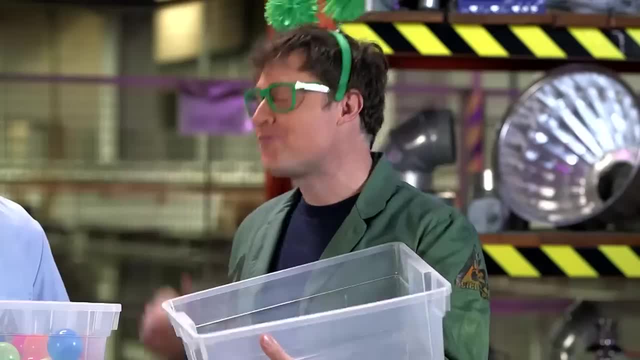 Would you like a proton? Oh no, really, I could Please, please take it. Oh well, thank you, That's very generous. Have another? Well, perhaps, maybe I will. Here's one, Maybe just one. 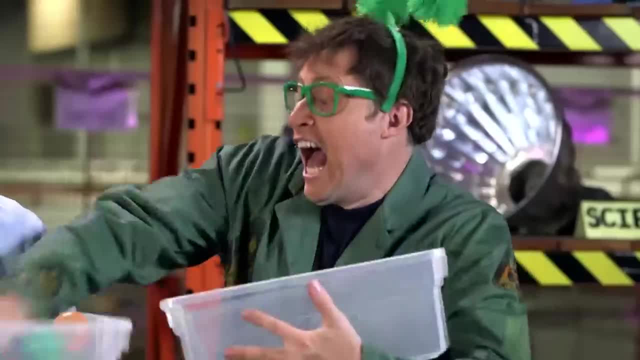 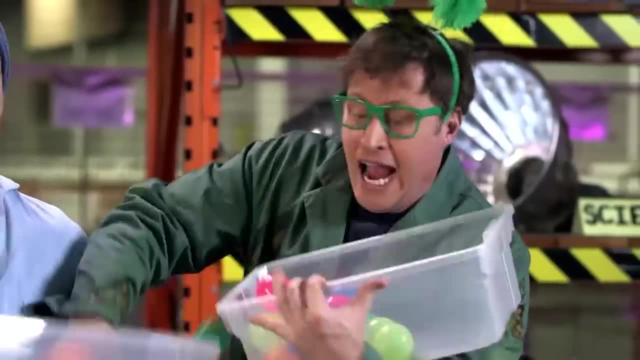 But if the acids and bases are strong, the chemical reaction can be really extreme. Aaaaah, Aaaah, Aaaaaah. This is what's going on in the antacid tablet And why, without water, nothing happens. Oh, Water. 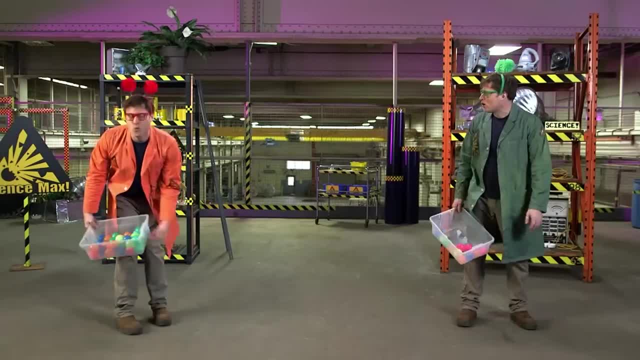 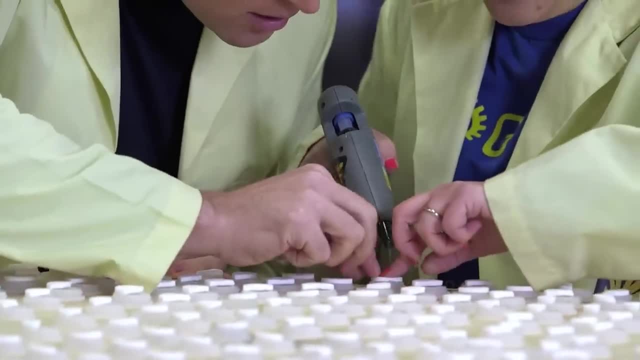 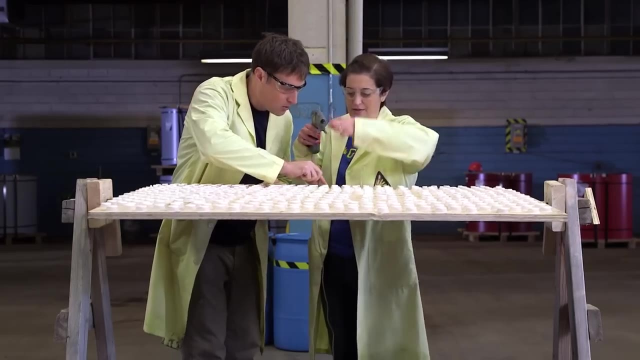 Water. Come on, What did you do? What? And that's the last one, Lisa and I are maxing out our chemical powered rocket, not by making it bigger, but by making more of them. How many more? 400 caps all glued down, 400 antacid tablets, or part of? 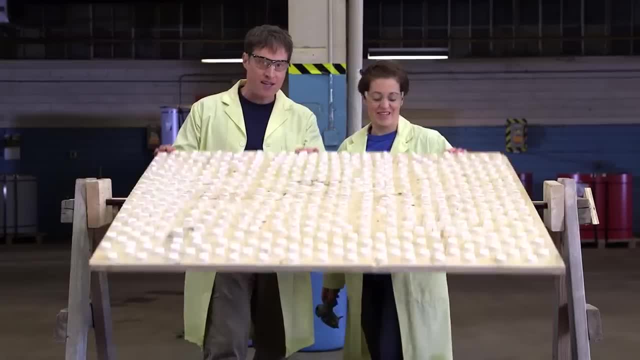 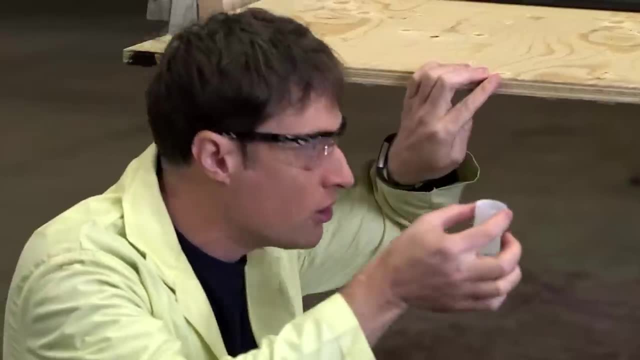 all glued down. and they're glued on this fancy-pantsy spinning surface. so we rotate this part upside down, We fill each container with a little water and snap it on underneath. This way, the antacid tablet and the water don't mix. 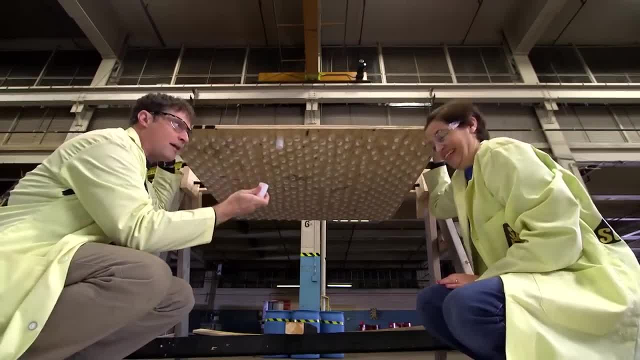 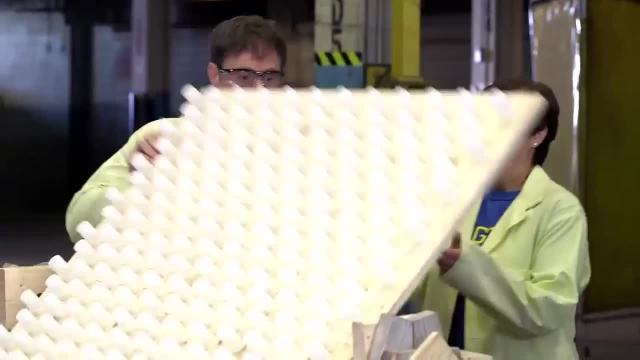 until we flip it back over. It also allows us time to snap them all on. Okay, ready, Ready, All right, 400 containers, Here we go, Let's do it. Once we flip the board back over, the reaction started taking place. 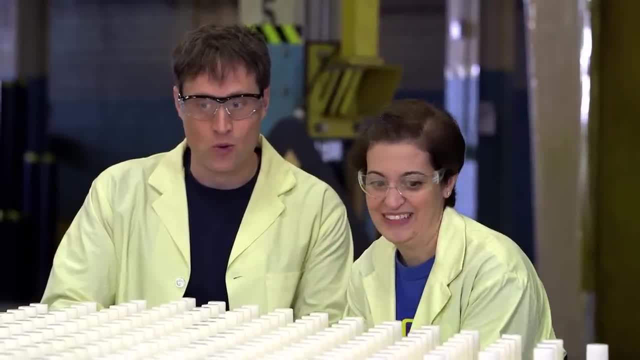 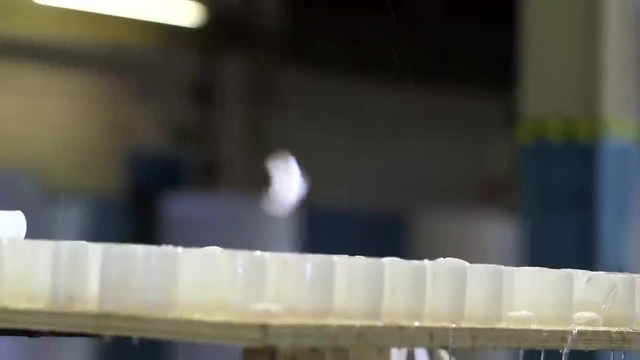 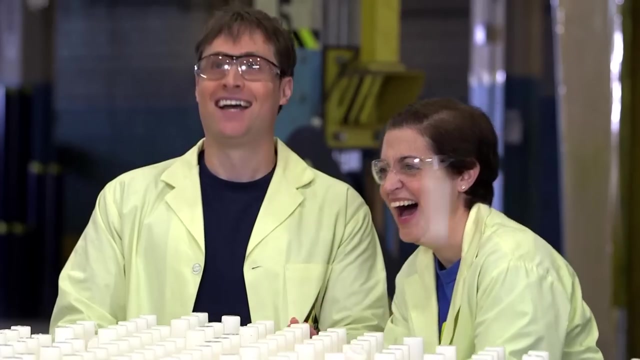 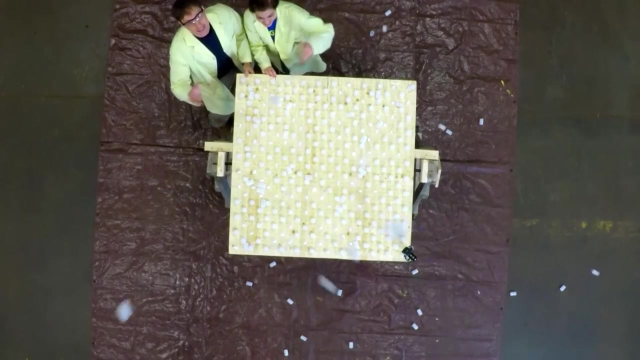 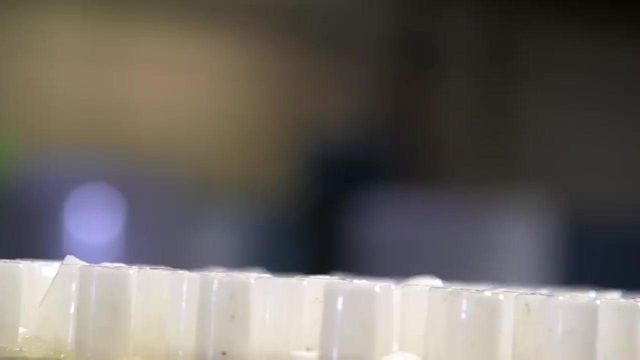 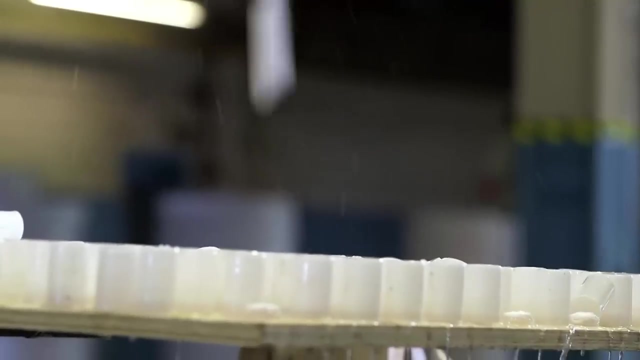 building up carbon dioxide gas and increasing the pressure until Oh yeah, Oh yeah, Good luck if you catch one. Wow, Wow, that one was really hot. Oh, Awesome, That totally was great. Wow, Okay, so high fives on that. 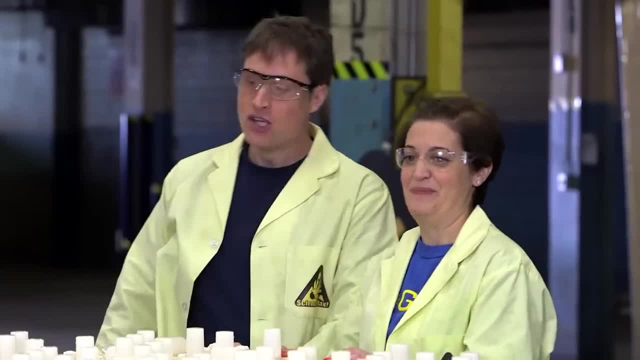 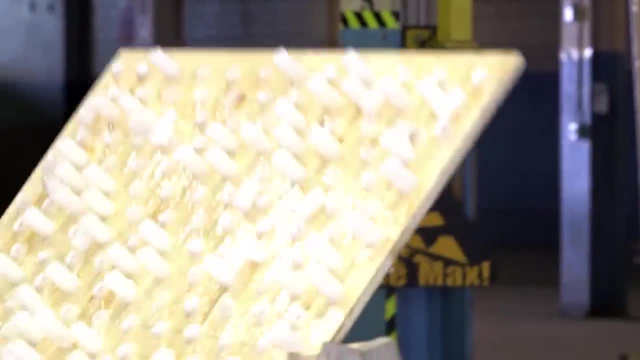 Yup, That worked spectacularly. That was awesome. So we've done this. Let's go bigger. Let's go bigger, Bigger, OK, so let's go, and we'll clean this up afterwards. Let's do it. OK, let it go. 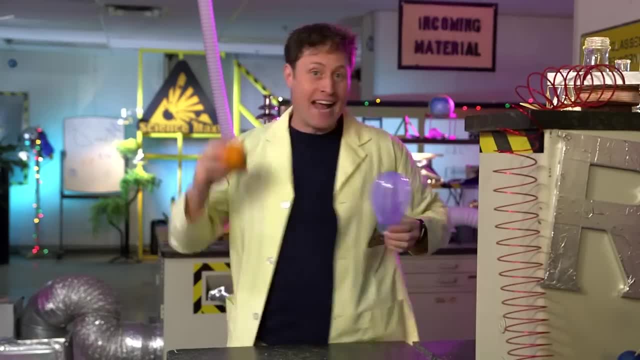 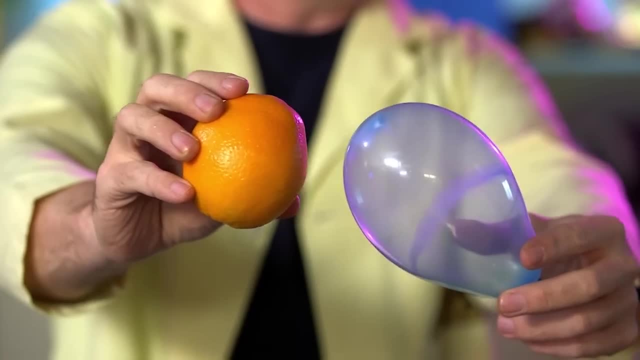 This is a balloon and this is an orange. When you put them together, a chemical reaction happens. How'd you go in there for a minute, didn't I? No, No, All right, Well, you can actually do a chemical reaction. 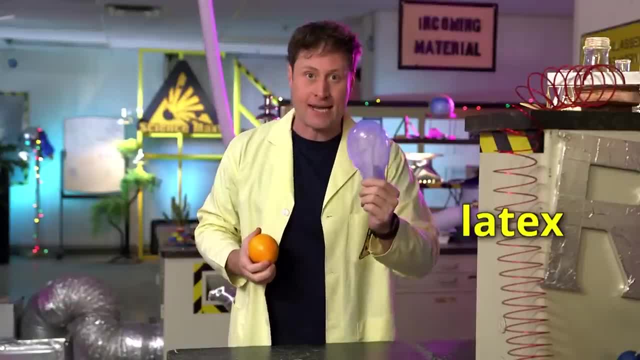 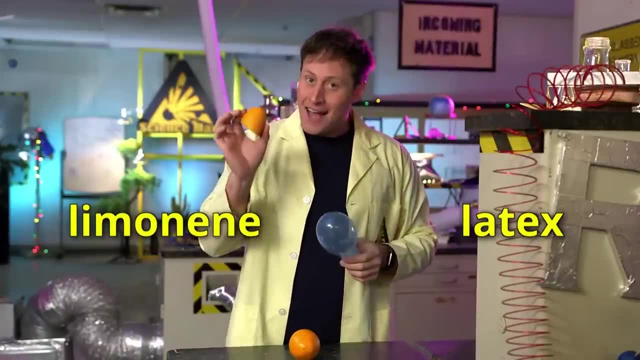 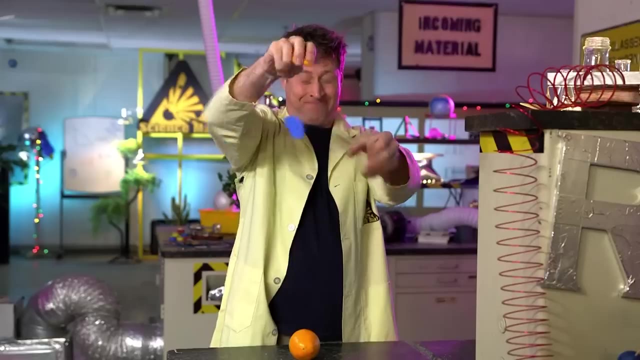 between a balloon and an orange. You see, balloons are made of latex, which is a kind of polymer that's very, very stretchy, And orange peels contain a chemical called limonene. Limonene breaks down latex. So we have three questions. 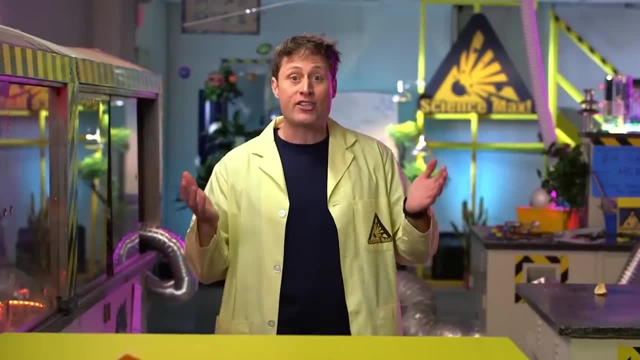 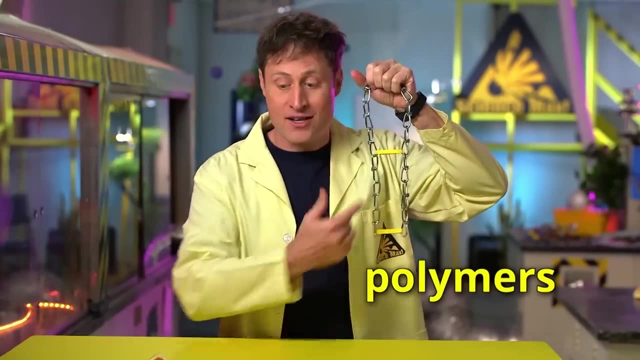 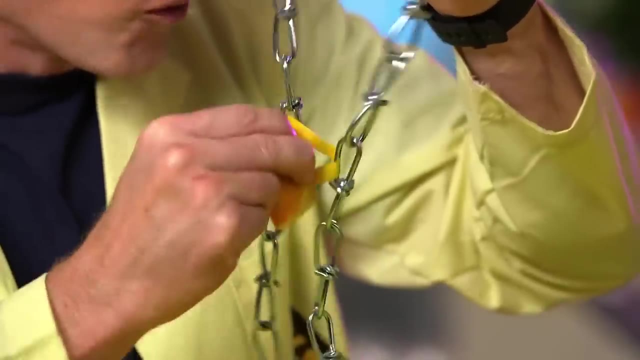 The first is: why does this happen? Well, like I said, it's all chemistry. You see, balloons are made of polymers, chains of molecules held together by chemical bonds. A limonene molecule attacks those bonds. Om-nom-nom-nom, Om-nom-nom, Om-nom-nom-nom. 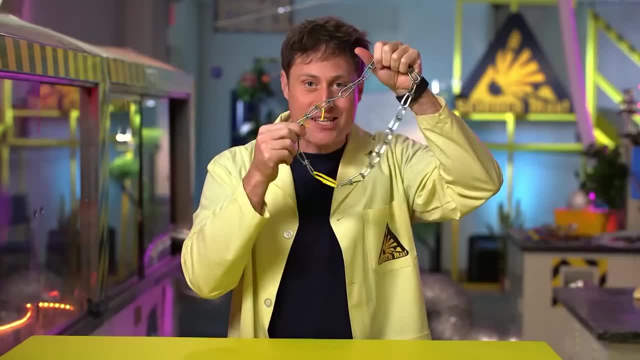 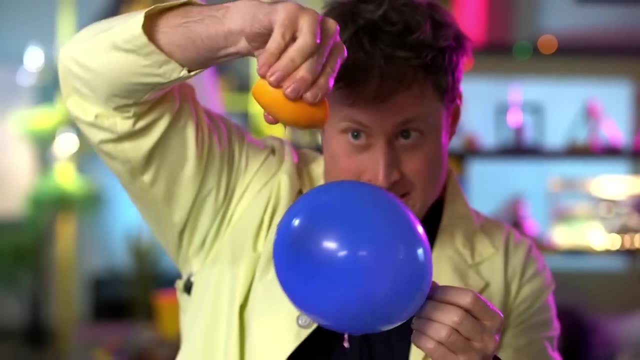 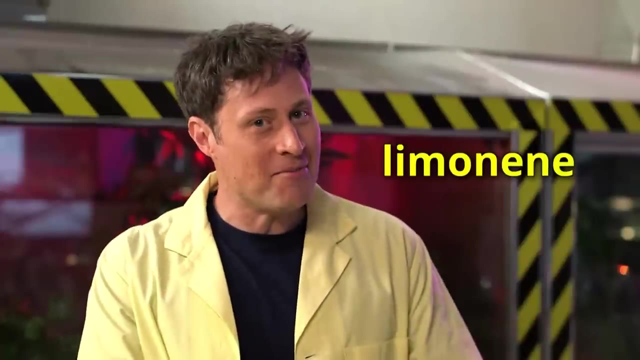 Om-nom-nom Delicious And breaks it. That separates the polymers and that pops the balloon. But remember it only works with natural latex, So make sure you're using natural latex balloons. Second question: why do they call it limonene? when it's in orange peels. I mean, yes, it's in lime peels and lemon peels, but the chemical itself smells like oranges. They should call it orangenine or citrus frutinide, or Anyway. 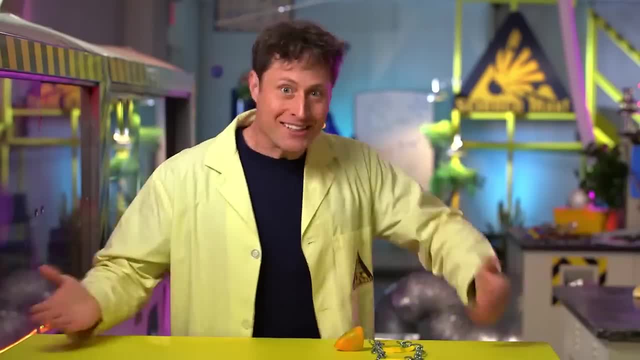 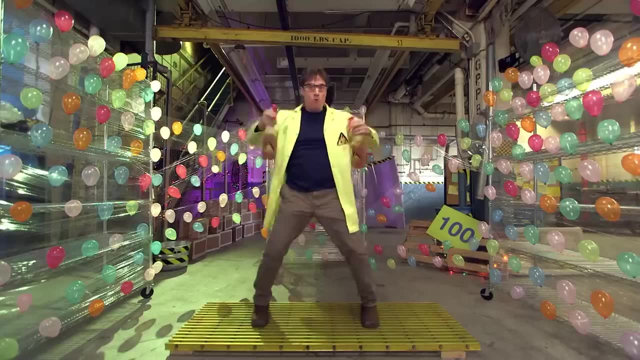 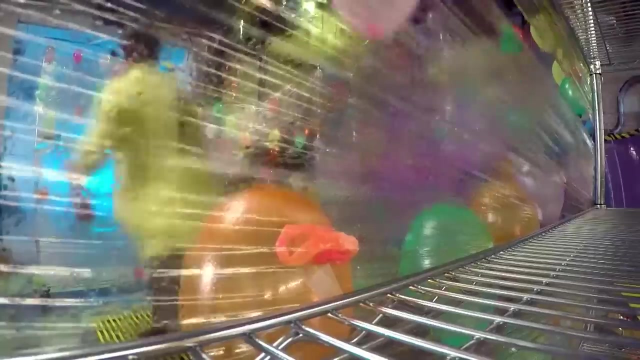 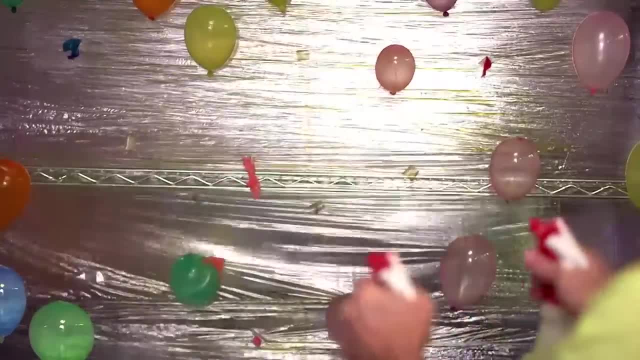 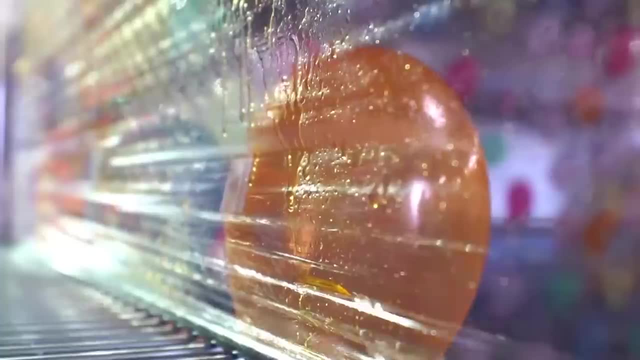 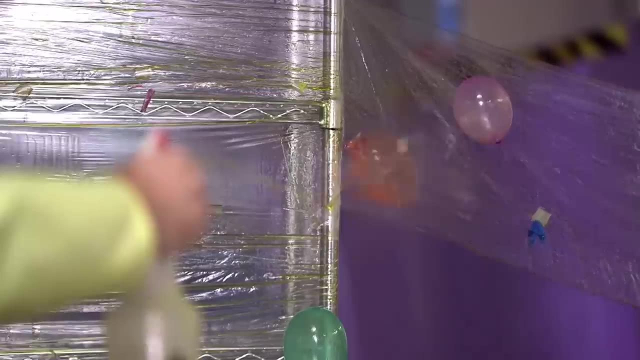 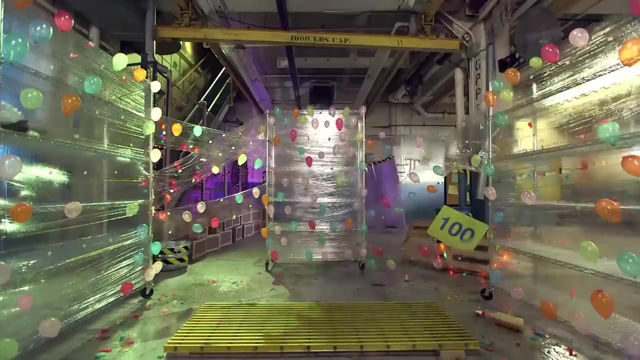 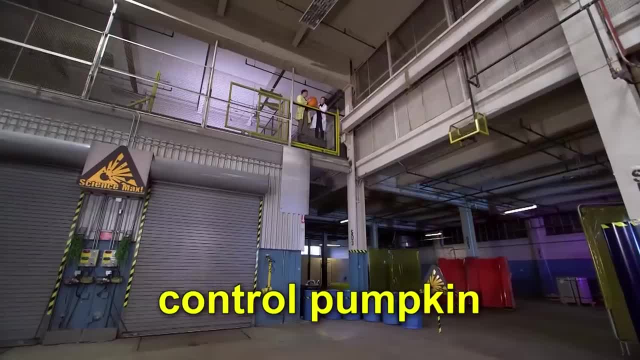 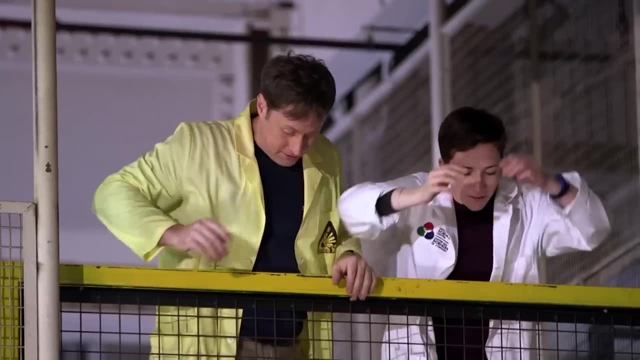 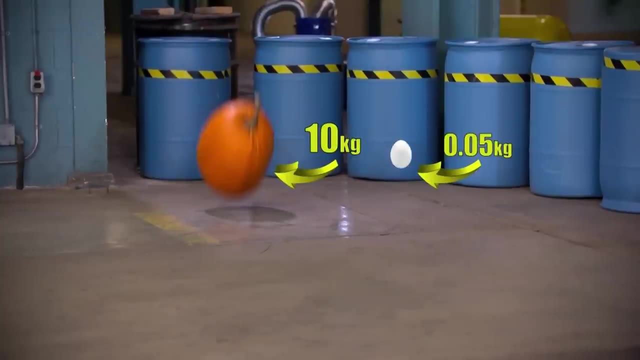 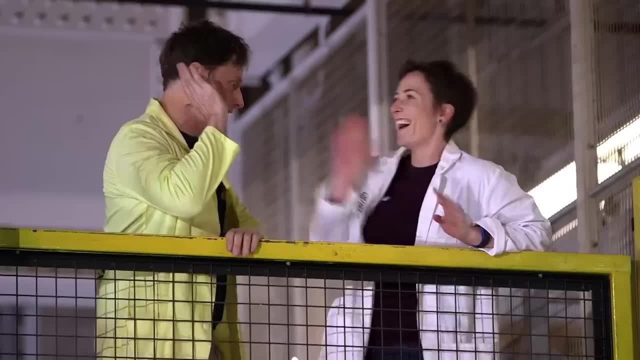 Well done. you both have worked. Sounds like the work you've done. How are the results of studying them stuck around here? Well, we have some, because a pumpkin has a lot mass than an egg, which means it's going to be more harder. 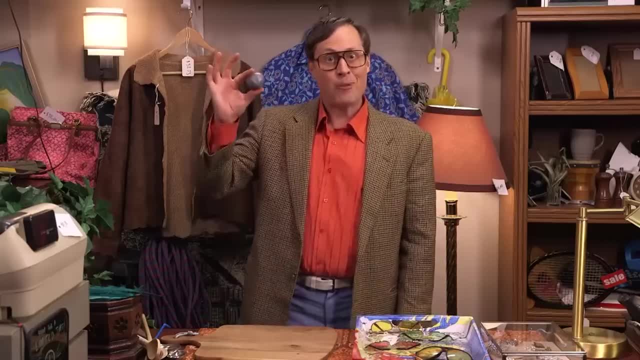 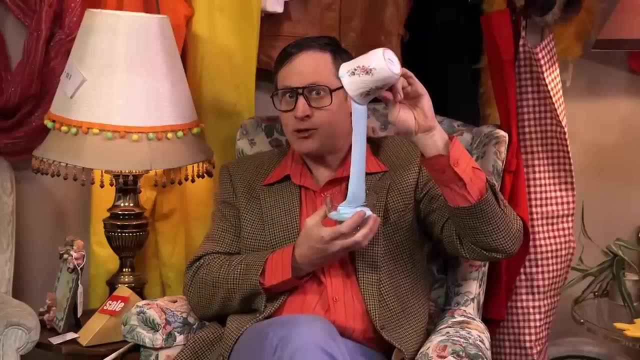 to stop once it's moving. So now all we have to do is come up with a couple ideas to stop that from happening. XOE Pastotherm Blupifoam. You need hydro-gelatinous substrate. I got it. 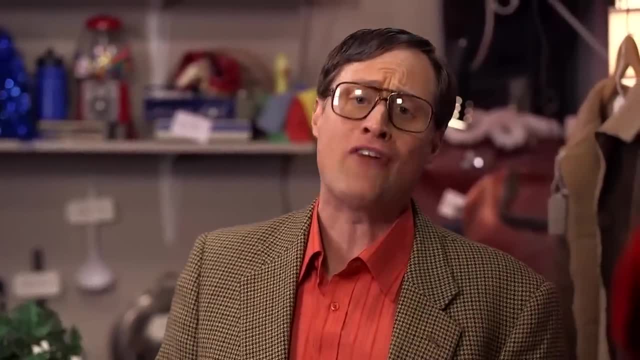 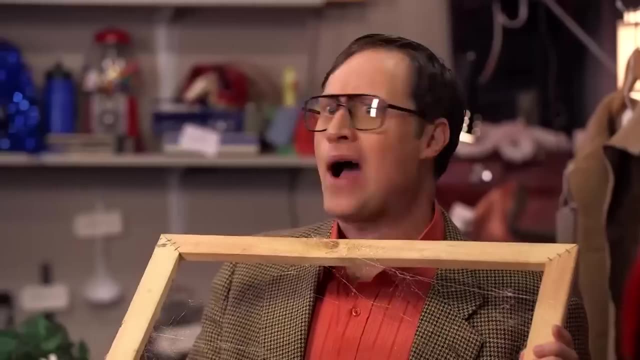 But you know, all those fancy materials are nothing compared to the good old-fashioned spiderweb. Huh Hey, where's Gary Ramona? Gary got away again. You know, people ask me: Sal, is it true, spiderwebs are stronger than steel. 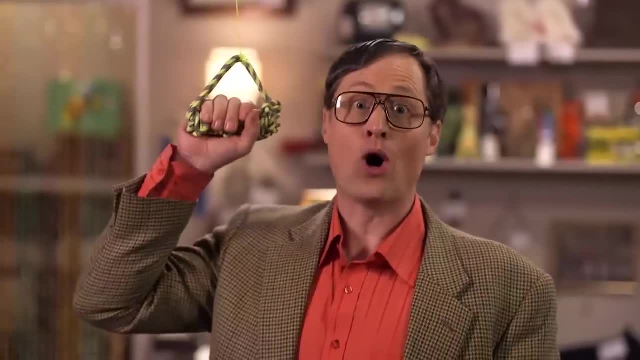 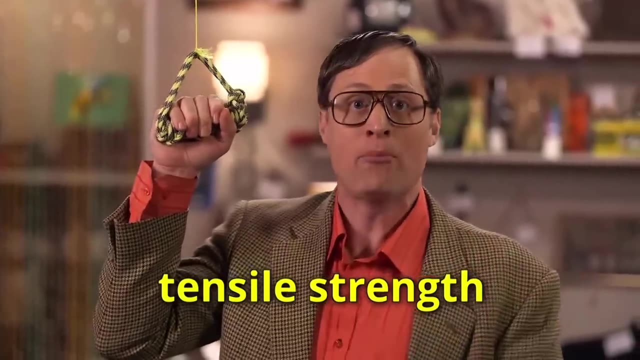 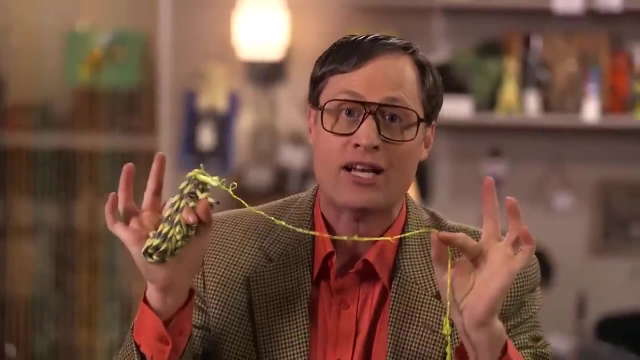 And I tell them it depends. When you look at a rope or a thread or a fiber, you talk about its tensile strength Or its ability to withstand force before breaking, But you're comparing different things, So you have to compare them by thickness. So if you're comparing a steel cable to a spiderweb of the same thickness, then yes, steel is stronger But spiderweb is six times lighter than steel. So if you are measuring strength to weight, spiderweb wins every time, Gary. 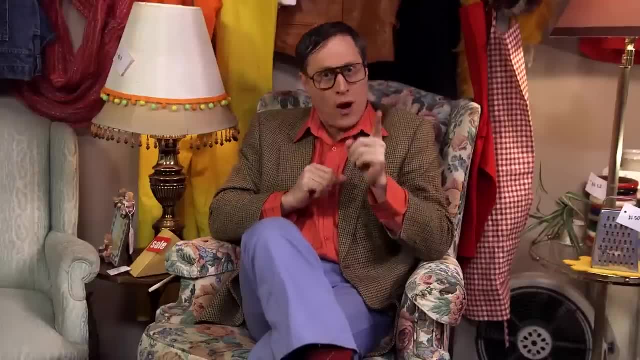 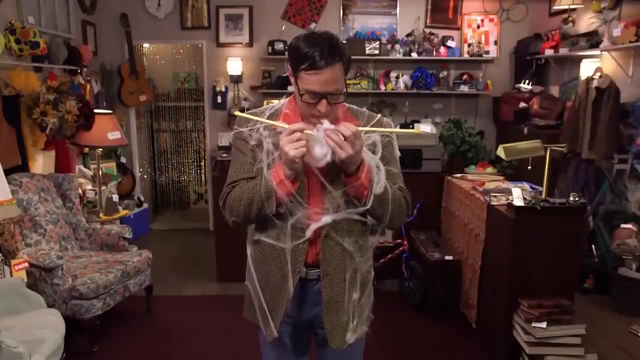 So why don't we build more things with spiderweb? Well, for one thing, it's sticky and difficult to work with Almost finished knitting this spiderweb sweater, It's only going to take me about 80 more hours, And it's not easy to train spiders. 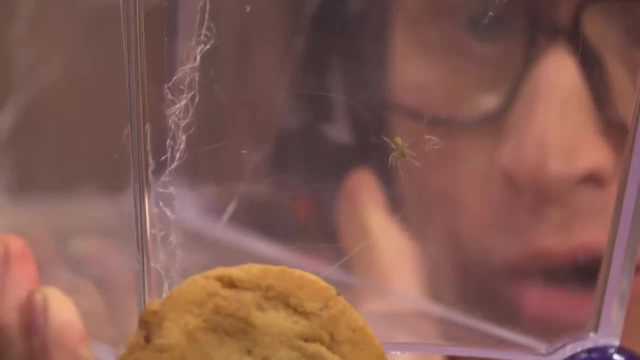 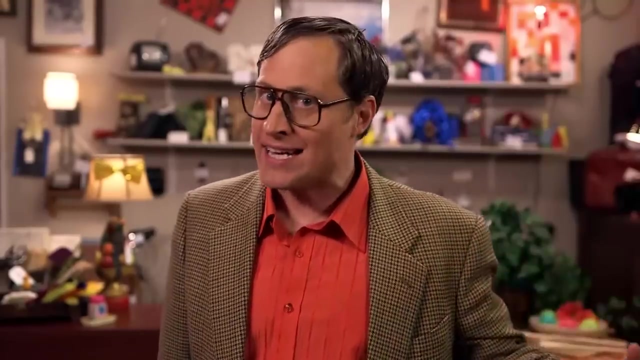 Okay, Steven, one long, non-sticky thread and you get a cookie. okay, And hey, where's Marco And Petunia? Huh, But no need to train spiders now, because modern science has surpassed the spiderweb. 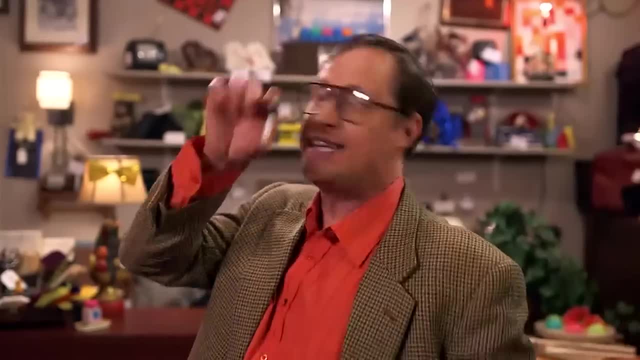 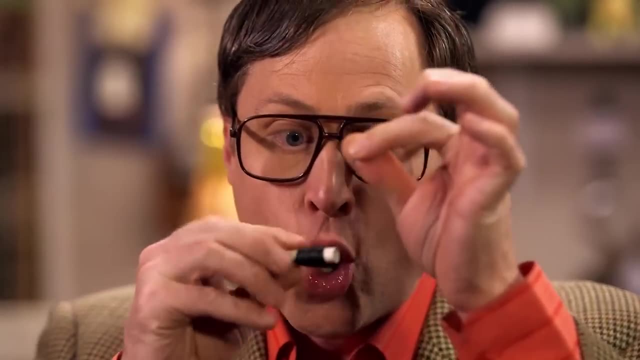 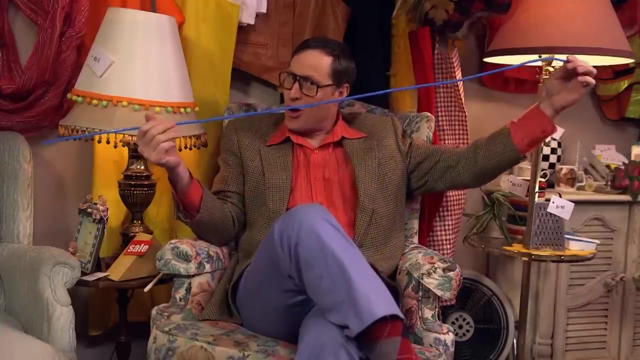 Enter carbon nanotubes. Huh, This thread doesn't look like much, but it is made of tiny little tubes made of carbon atoms, Thicker than like a straw, But a really long straw. Carbon nanotubes are incredibly light and strong. 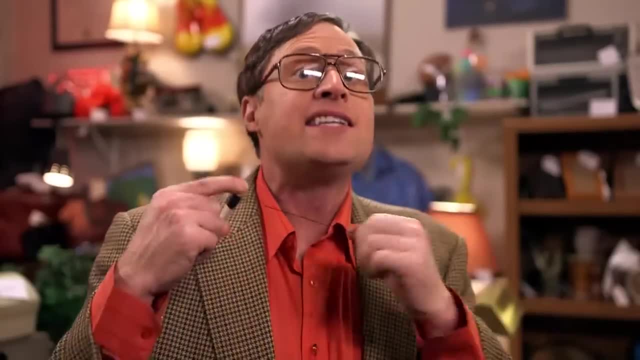 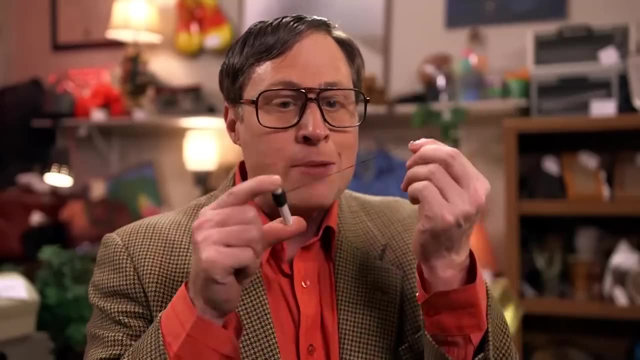 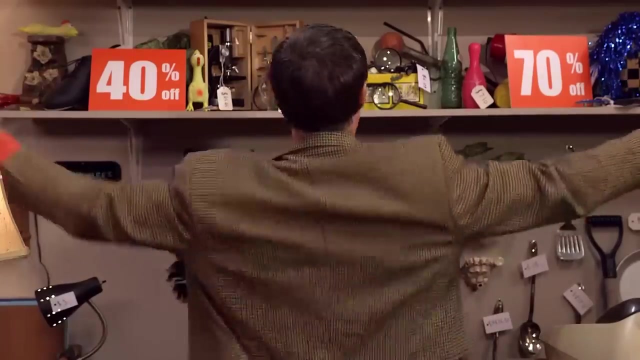 Remember when we compared strength to weight? Well, steel is heavy, Spiderweb is about six times stronger by weight And carbon nanotube is about 50 times stronger than that. That's so great. So why aren't we making everything? 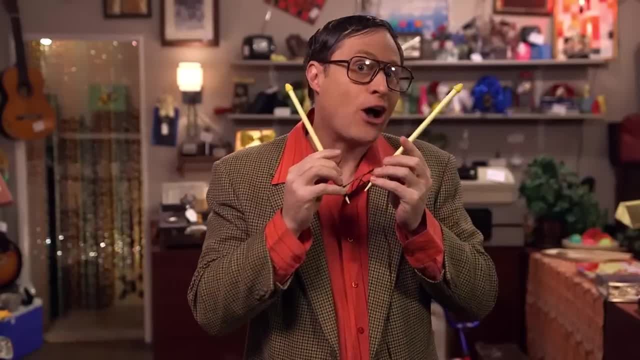 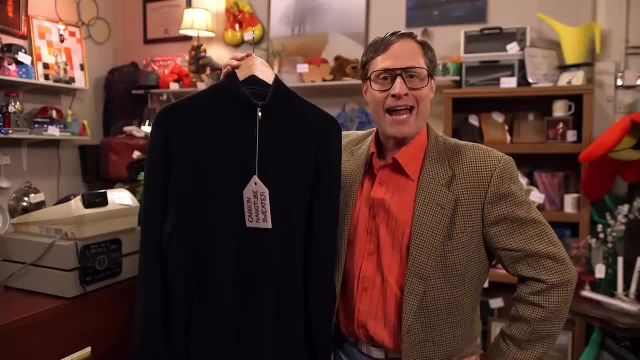 out of carbon nanotubes. I'm going to knit a carbon nanotube sweater. Well, first we have to make them cheaply enough to be affordable. There you go. One carbon nanotube sweater- $480,000.. 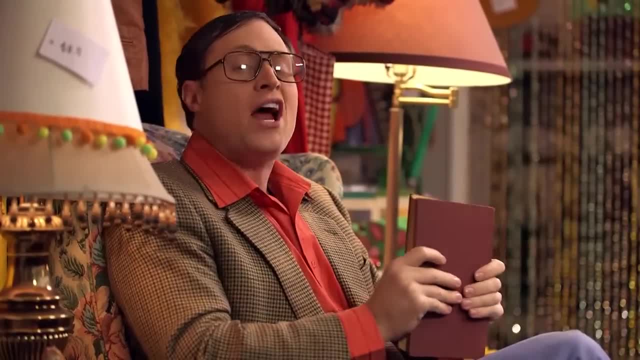 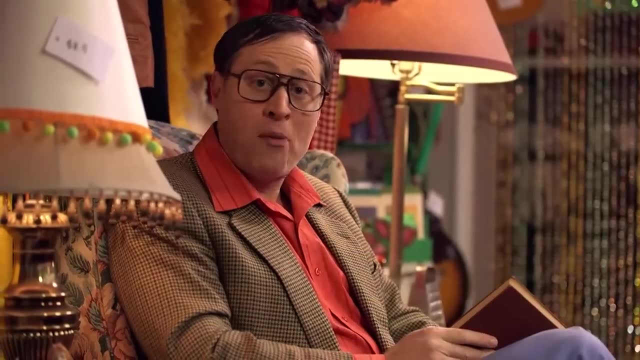 But material scientists all over the world are hard at work trying to find ways to make carbon nanotubes Faster and cheaper, And soon they'll be everywhere, And then spiders can go back to spinning their webs in peace. There you are, Gary. 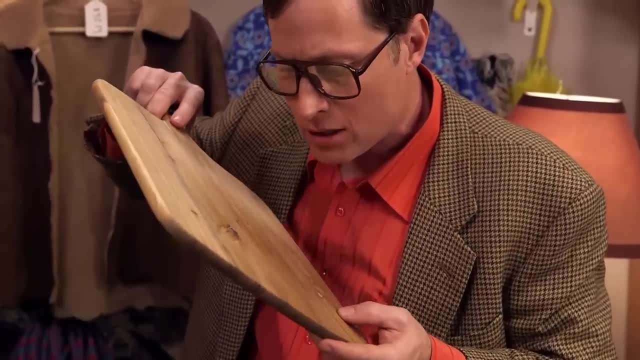 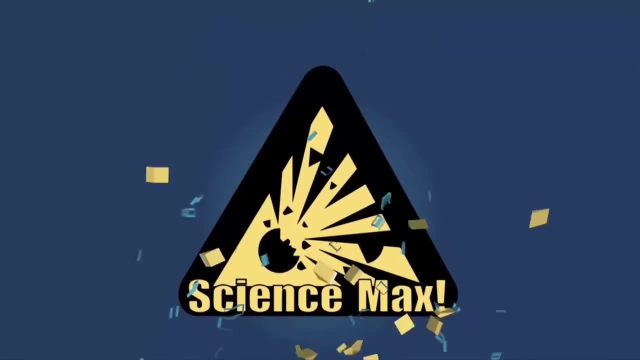 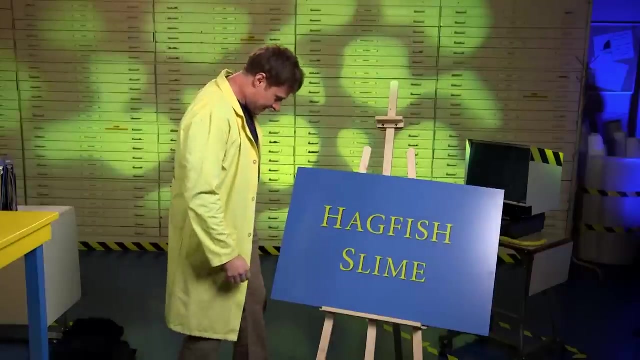 Where's everybody else? Petunia and Marco, and What do you mean? they're in my jacket. Now it is time to talk about an amazing natural polymer. It is hagfish slime. Ugh, Um, still well, hagfish. 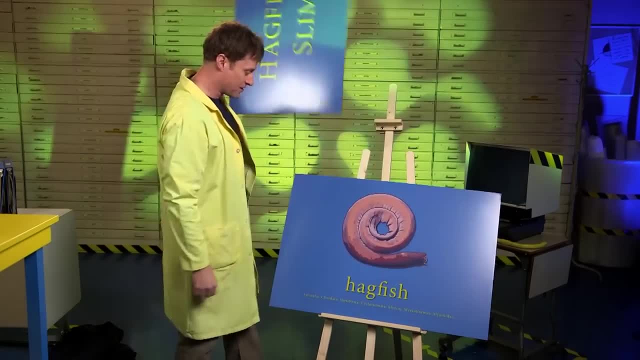 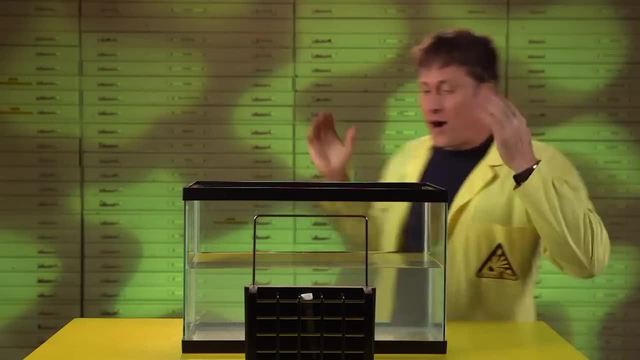 that's probably just an unfortunate name for the fish. I'm sure the fish itself doesn't Ugh. Okay, so hagfish makes slime, apparently When a hagfish is attacked by something that wants to eat it, like a shark or an eel. 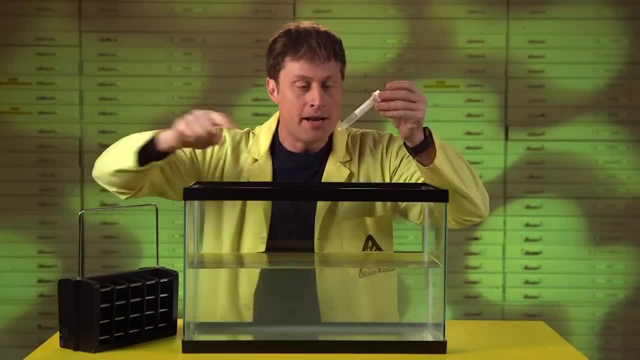 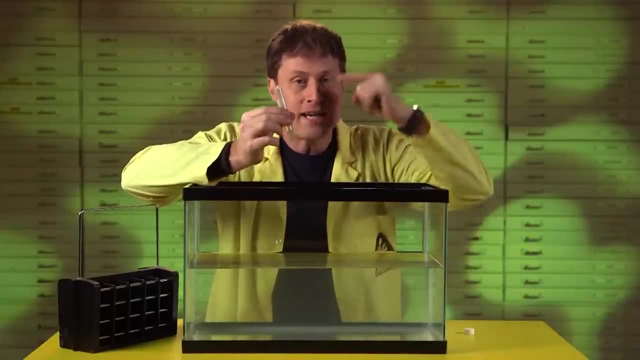 it secretes a tiny bit of a natural polymer. That's this little white bit right here at the end of this test tube. Now it doesn't look like much right now, but it reacts with seawater Watch. this Hagfish slime is very interesting to scientists. 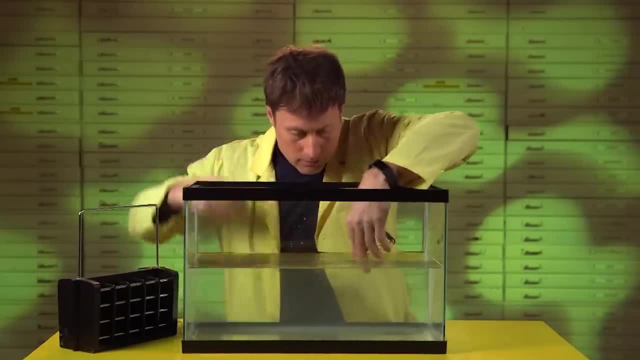 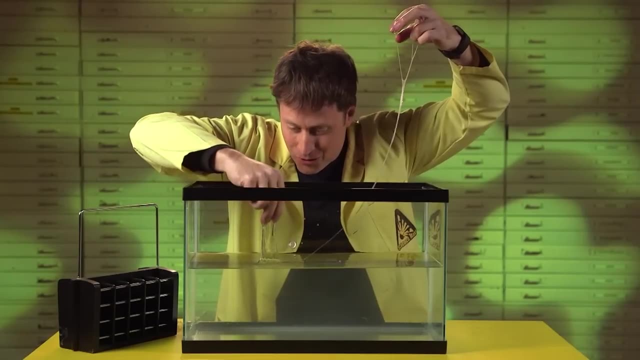 because you start with just a tiny little bit and add seawater and suddenly you have a lot of slime. Whoa, This stuff is actually pretty cool. Hagfish slime is a natural polymer. It's made just the same as the other polymers. 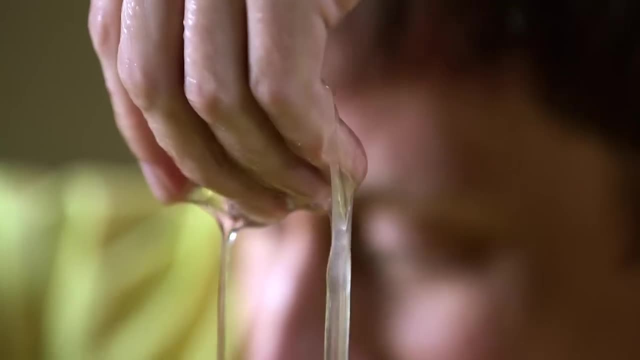 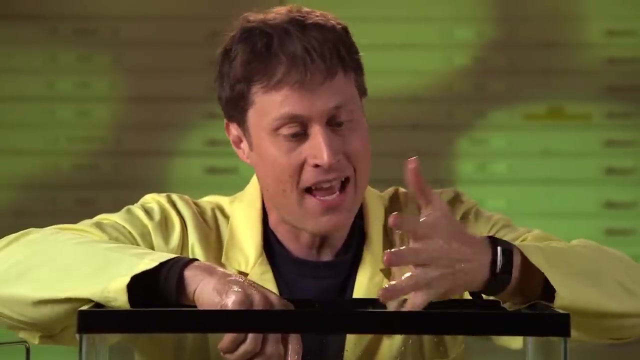 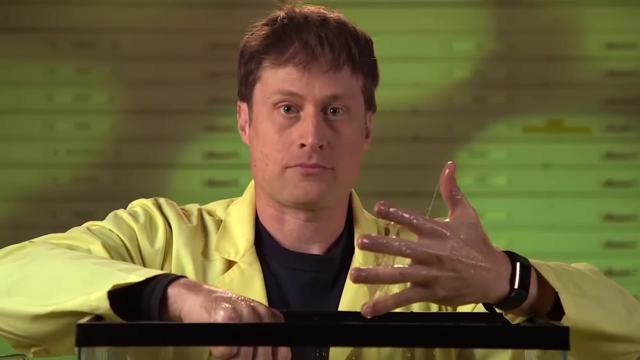 out of long chains of molecules, but it's naturally produced by a living organism. And because it's naturally produced, that means it's biodegradable. Hagfish slime- It's pretty cool, after all, Ha-ha Ugh Foam. 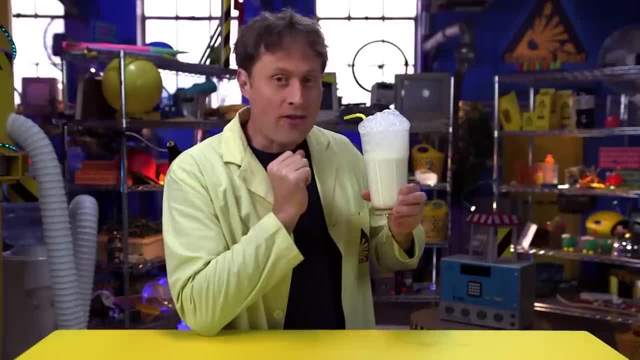 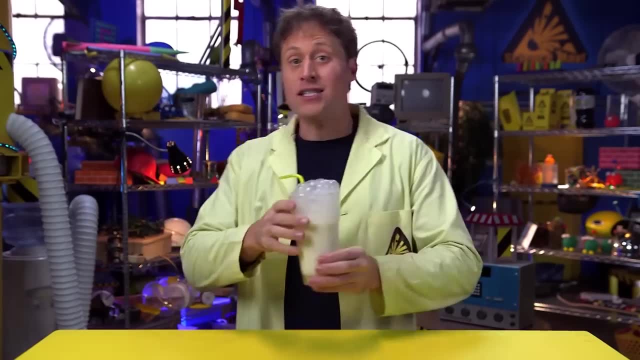 Foam, Foam. How can they all be foam? Well, foam usually means something to do with bubbles. There's all kinds of solid foams out there, and they can be squishy or not squishy, And they're usually light. 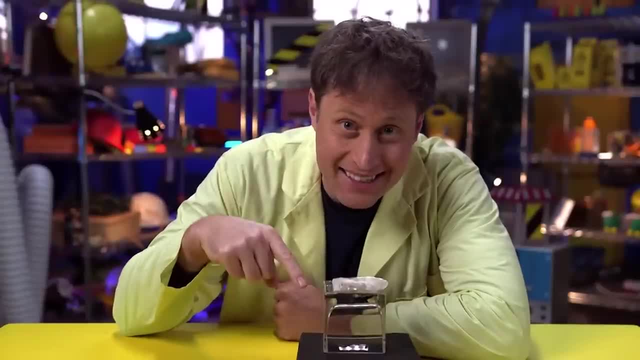 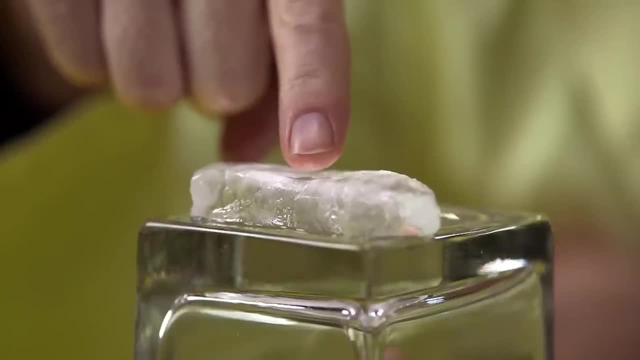 Air, Air, Air Air Air. It's an insulator. That means it does not conduct heat or cold. very well, You see, I cannot tell this ice is cold until I get my finger really close to it. Yeah, Yeah, there it is. 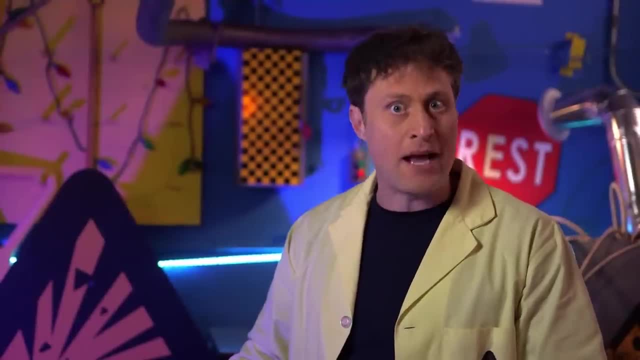 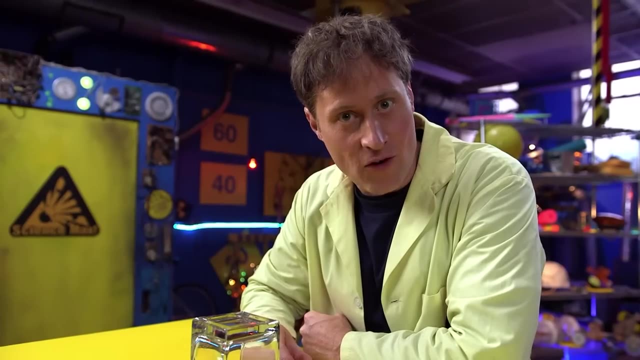 Uh-huh There, I feel it. And because foam is full of air bubbles, it makes a great insulator. That's why we make coolers out of foam. So what's the best, most advanced foam out there? It's this. It's called aerogel and it's 98.2% air. It is super light because it's mostly air, and it's a great insulator because it's mostly air. It's great to pack things in as well. 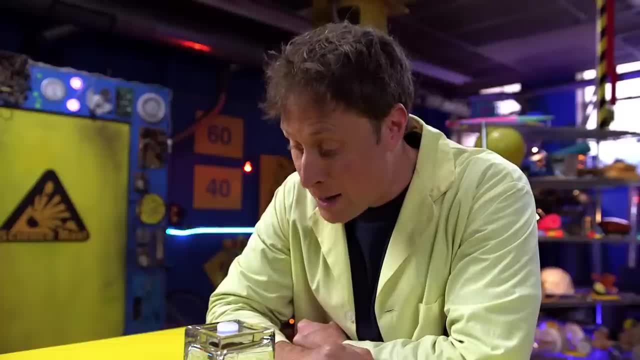 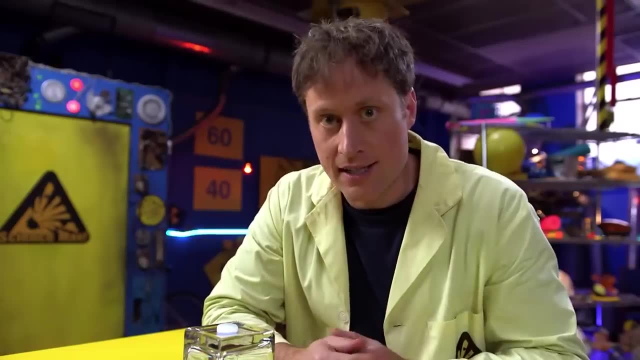 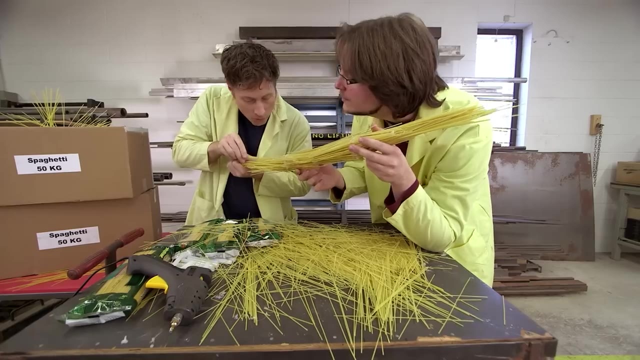 and NASA uses it on the Mars rover and in spacesuits because it's such a good insulator- Cool Or not cool, because you know it's an insulator, so it would protect from the cool. Our pasta bridge was going to take a long time. 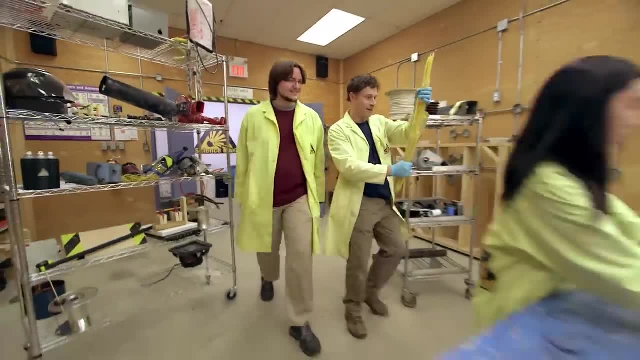 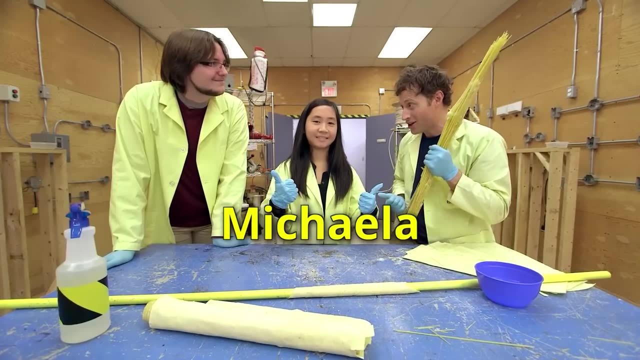 but it's time to build out of individual pieces. So we have a new plan. Hey Michaela, Hey Phil, How you doing? I'm great. How are you Good? This is Michaela. She's an undergrad in industrial engineering, right? 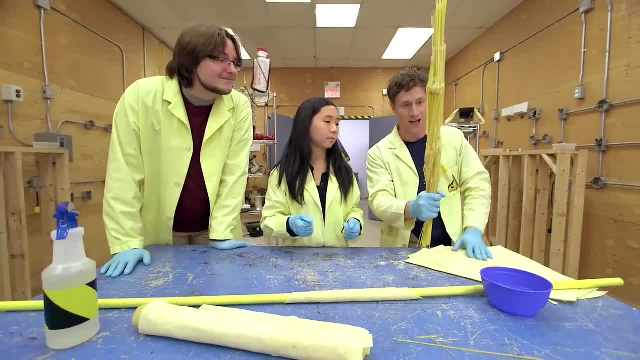 I am, And you and Kyle have a new plan for how we can build our pasta bridge. that's not going to look like this. Oh man, This is the best that Kyle and I could do with 20 minutes. Okay, Well, I have better. 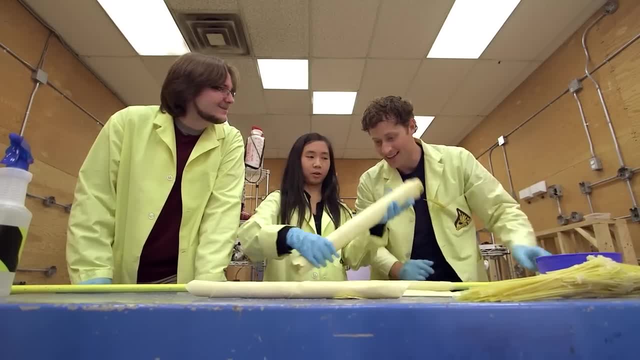 Good, I'm glad. How are we going to do it? So, instead of that, we're going to try something like this: Oh, okay, This is sort of like a giant burrito kind of thing, right, Yep, But we're going to build the bridge out of this. 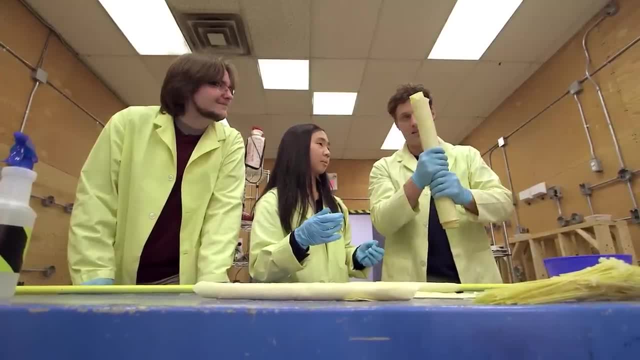 Exactly. Are we going to make it longer, though? Yep, We're going to make it eight feet long. We have this long pole right? Yep, And we have sheets of this pasta. We're going to put them on the diagonal. 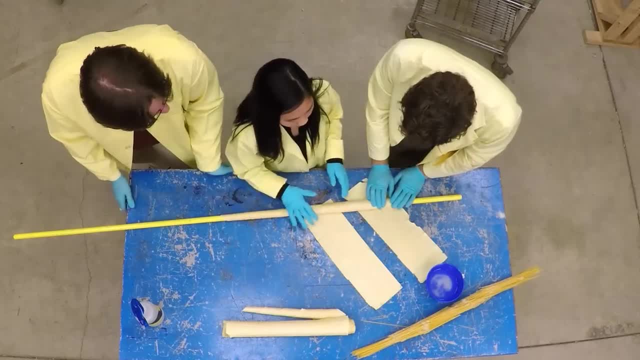 Okay, And we're going to roll it, but we're going to start from this corner and we're going to keep rolling, And don't forget to add water, And we've got to add water. I'll add the water, Okay. 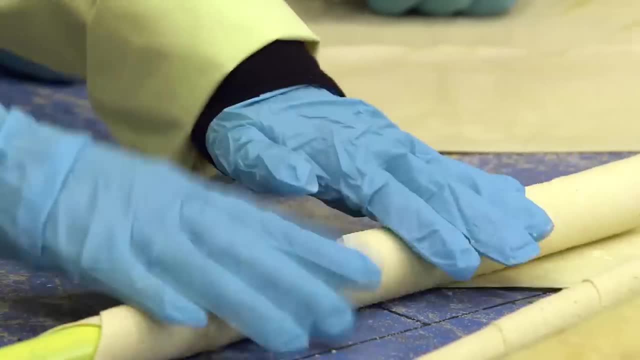 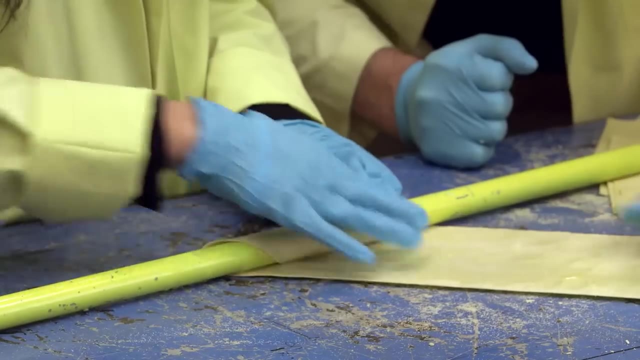 Adding water Just like this. Yeah, Yep, It helps the pasta to stick together, Okay, So now we're going to add water And we're going to add water. Okay, And we're going to add water. So as we're rolling, we're rolling, we're rolling. 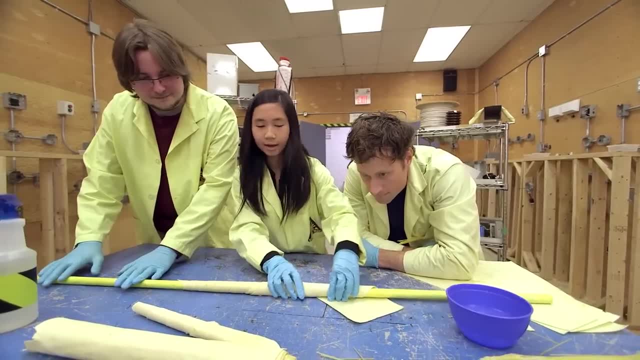 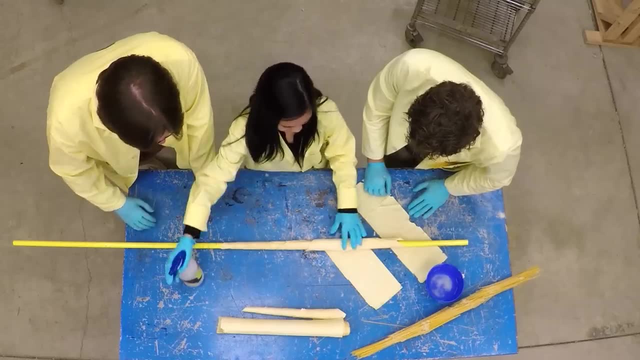 we're going to keep doing this with a bunch more sheets so that it gets really really long, like eight feet long, And when we're finally done rolling, we've got to spray it with some varnish, Yep, And so it all holds together. 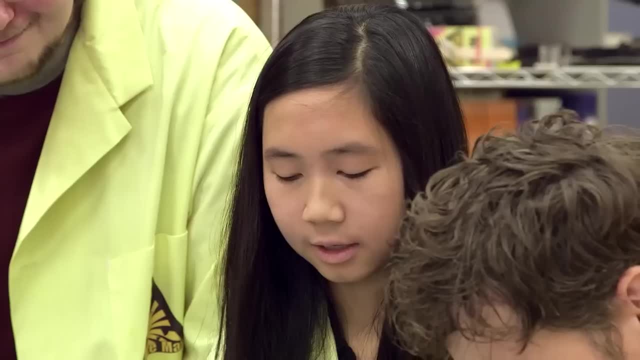 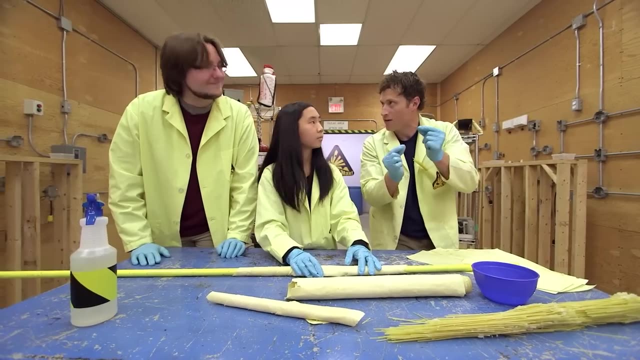 Great. And then it's going to be about this thick Yeah When we're finished with it. Exactly, This is going to be one of the parts of the deck of our bridge- Great. So each one of these large pieces is going to be like one single strand of pasta. 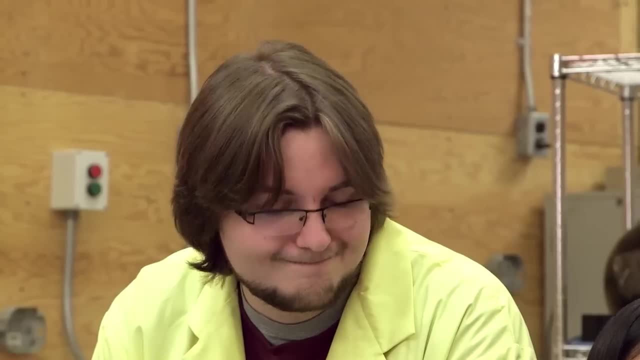 in the little bridge we made. Yeah, We need a lot of these, A lot, But still it's a lot faster than doing it piece by piece with just spaghetti. Aww, Every time I hold it up you make that noise. 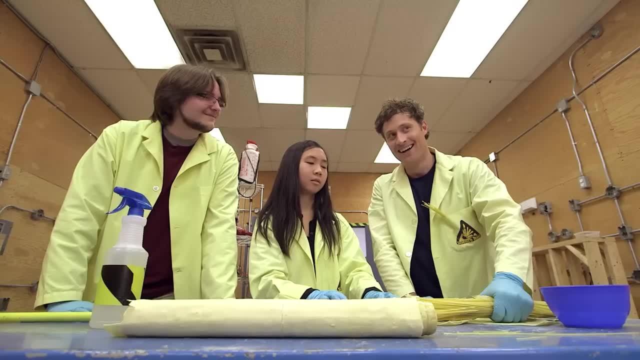 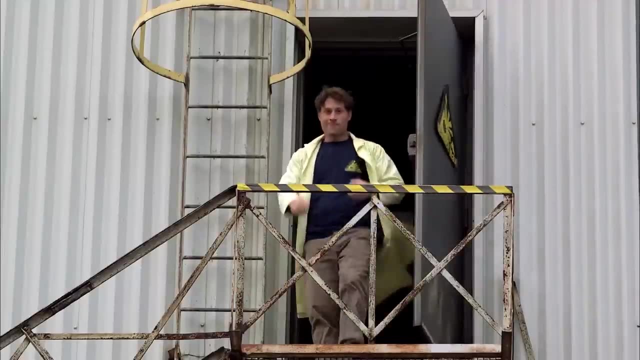 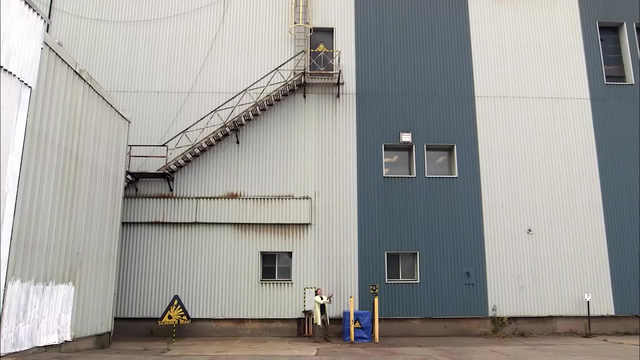 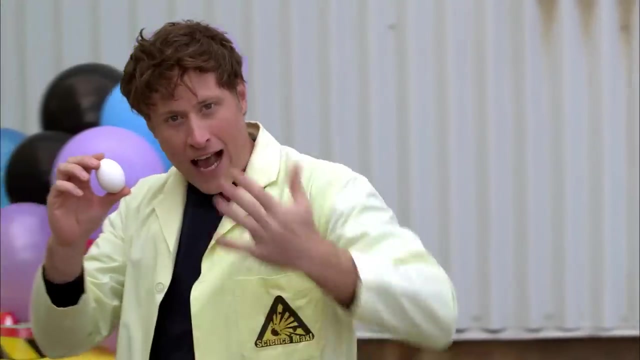 Aww, Aww, Aww, Awesome. This is an egg. Eggs do not like to be dropped. Oh, Fortunately, we can use the power of science to design something that'll keep the egg safe as it falls. Behold. 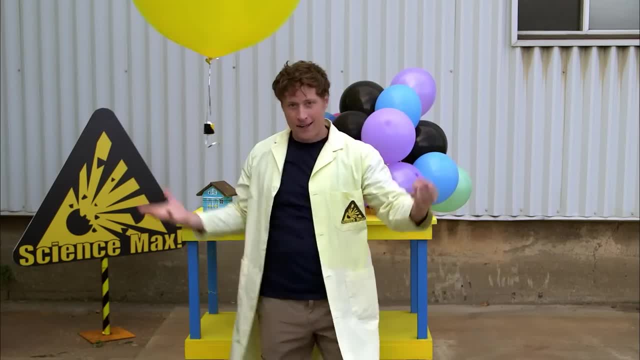 My egg drop contraptions. The thing I really like about this experiment is there's no wrong way to do this. You can come up with any design you want and see if it works. This one here is a bunch of helium balloons. This structure is just to keep the helium balloons on. 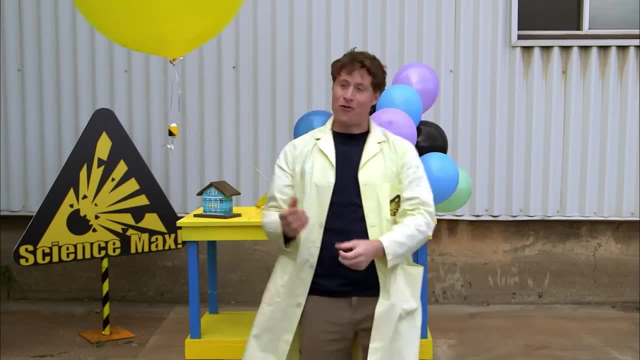 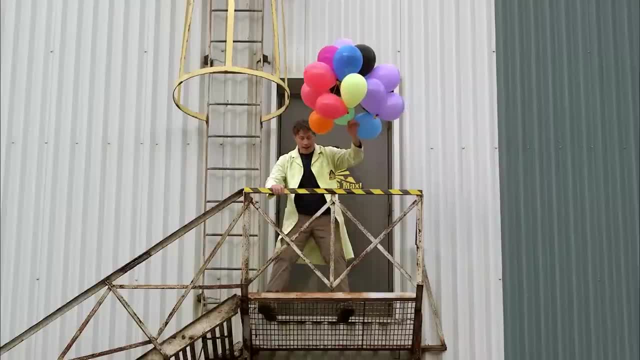 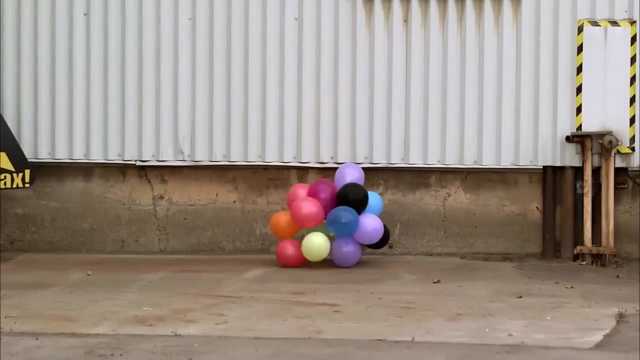 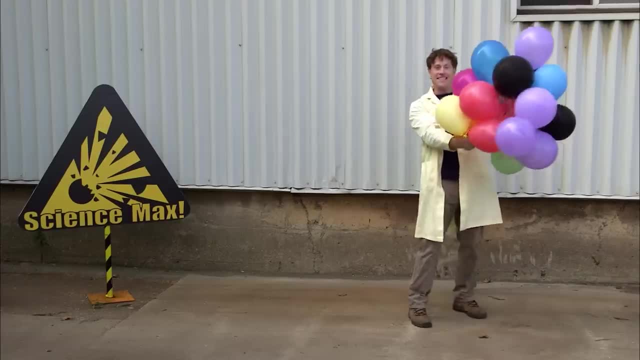 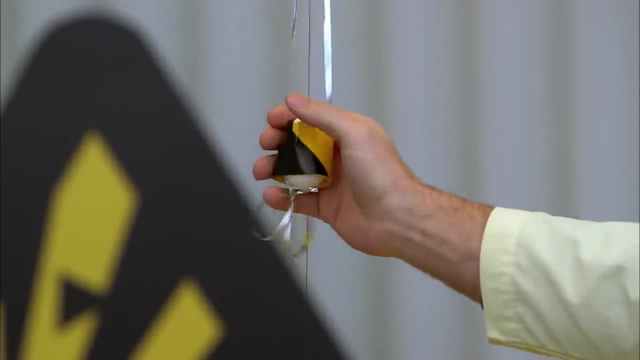 Miraculously sound. That one worked really well- Success. This is a giant helium balloon that I think will work pretty much the same way, Because I think this balloon will drop just slowly enough that the egg can actually just touch and nothing will happen. 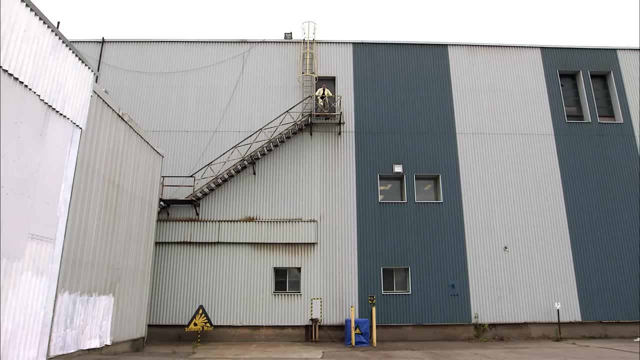 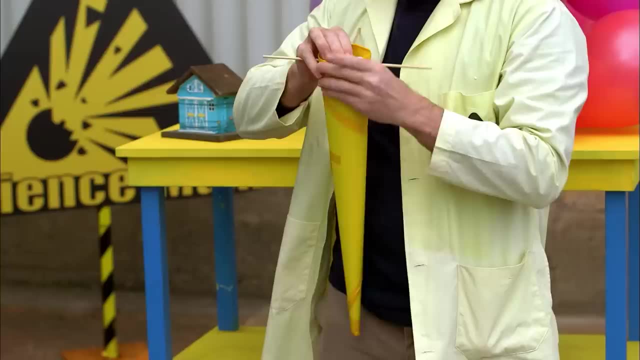 Um, so that didn't work. And then there's the balloon, And then there's this one, which has no slowing at all. It's all designed to just absorb the impact, And the idea is that the cone will crumple and absorb the force when it hits the bottom. 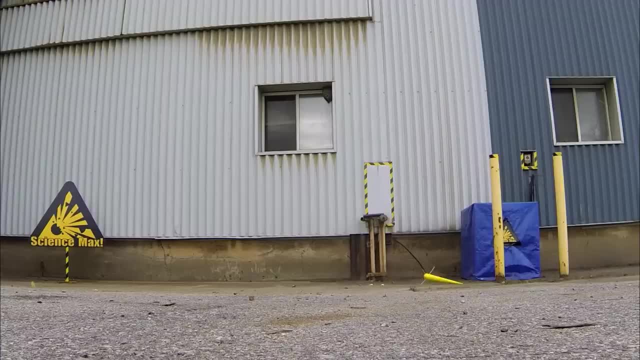 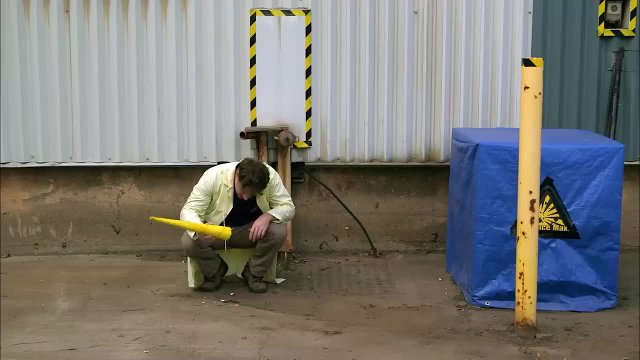 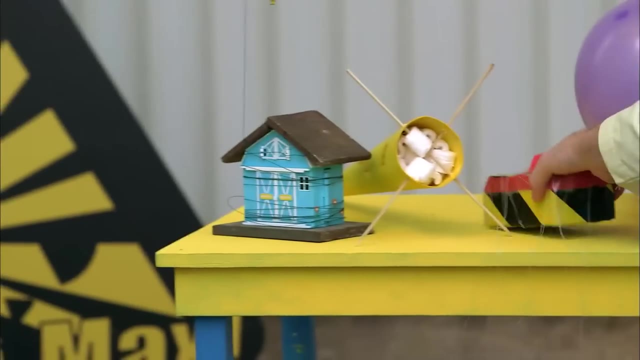 Oh no, Oh no. I think it would have worked if it hadn't turned in the air, but it did. And well, I guess the egg is completely broken. So I'd call that one a fail. This one is the parachute. 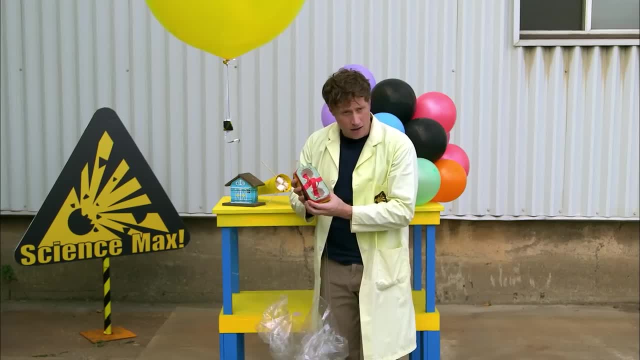 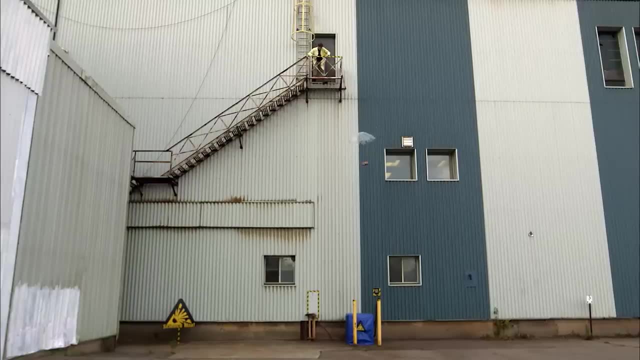 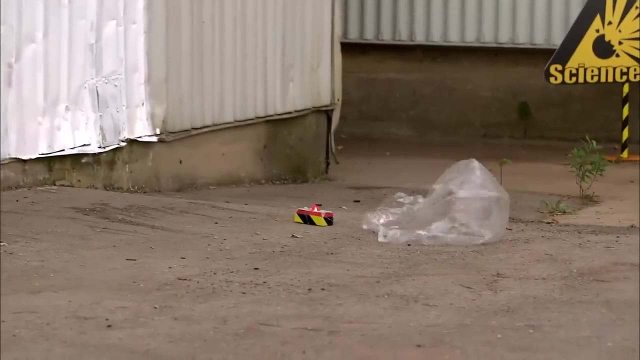 You see, the egg has been nestled into this foam container, And this is a parachute that will hopefully slow the egg down. Woo-hoo, Uh-oh, Whoa, Over, Over, Good, And That one seemed to work well. 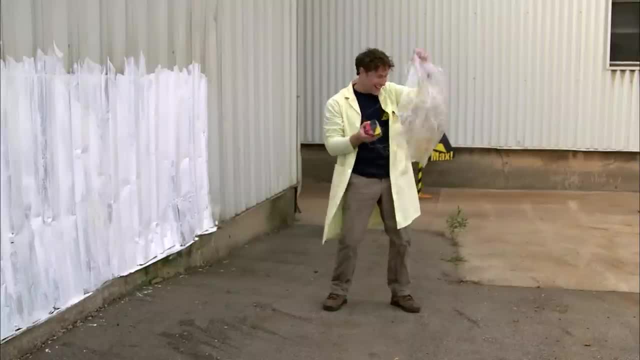 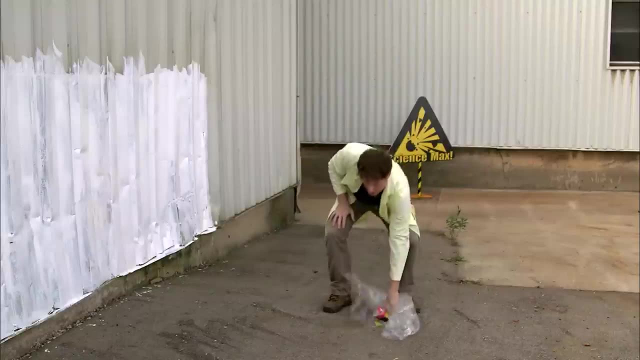 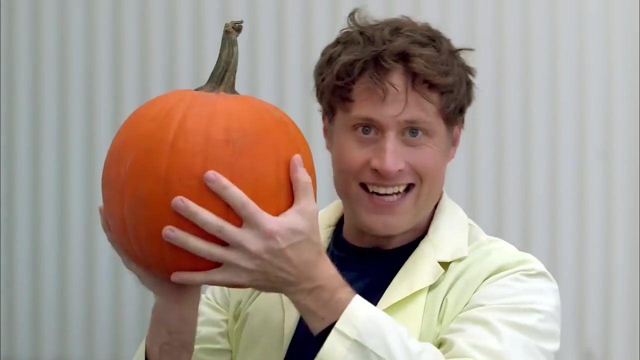 Yep, the egg is totally fine, The parachute worked All right. Egg drop experiment: totally fun experiment to do. But the question is: how do we max it out? And the answer is: pumpkin drop. Same thing, except with a pumpkin instead of an egg. 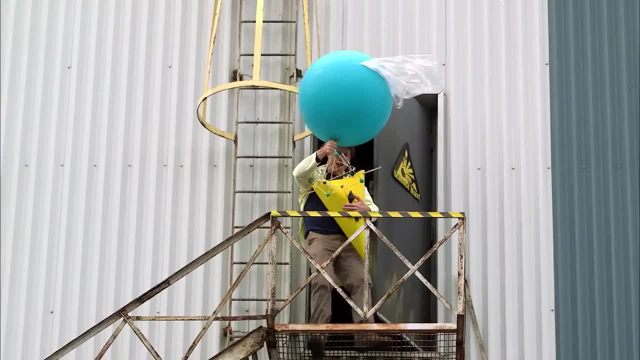 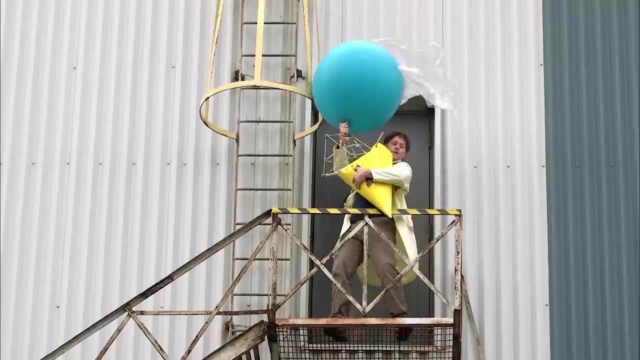 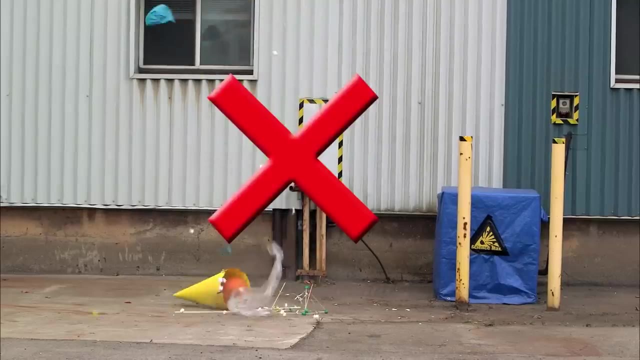 Come on, Okay, All right, Pumpkin drop with everything attached all at once. Okay, here we go, Ready: One, two, three. So what we've learned from this is: the heavier something is, the more force is acting on it from gravity. 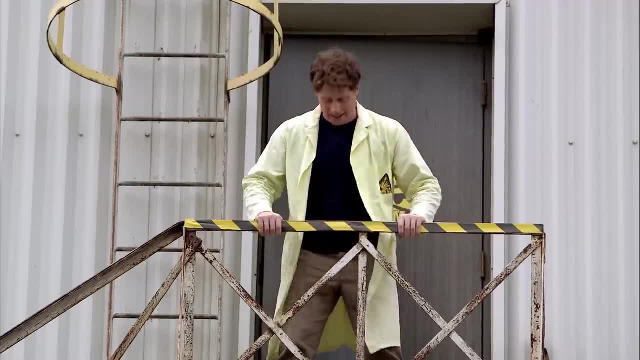 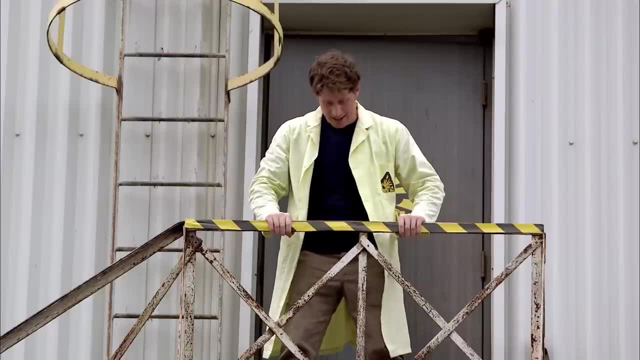 which means the harder it is to slow down when it's falling. Okay, Fair enough, You win this one gravity, But I'll beat you next time I'm. I'm going to get a broom Bills weight on two toilet paper rolls. 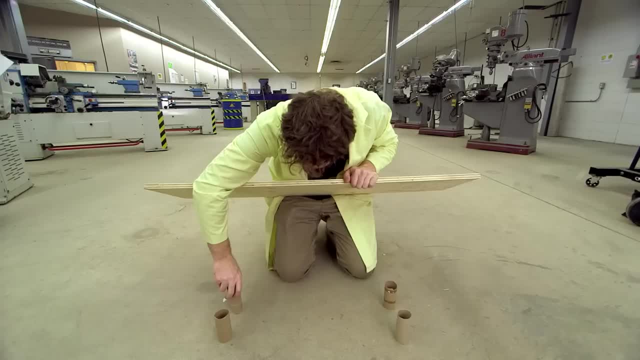 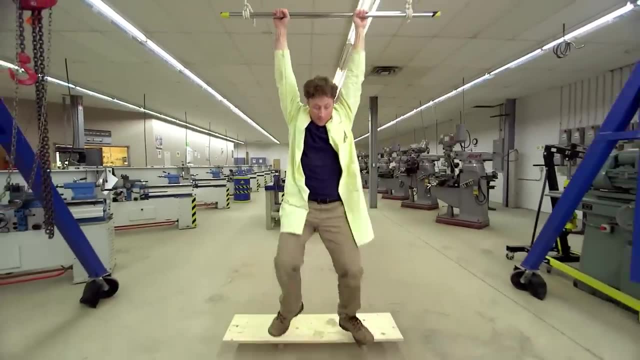 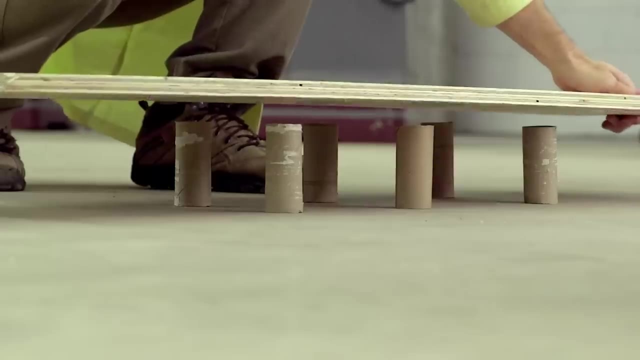 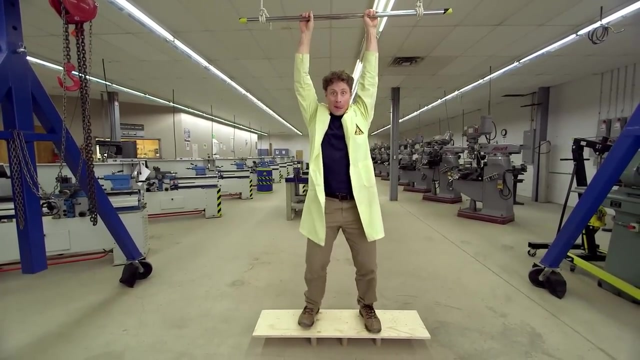 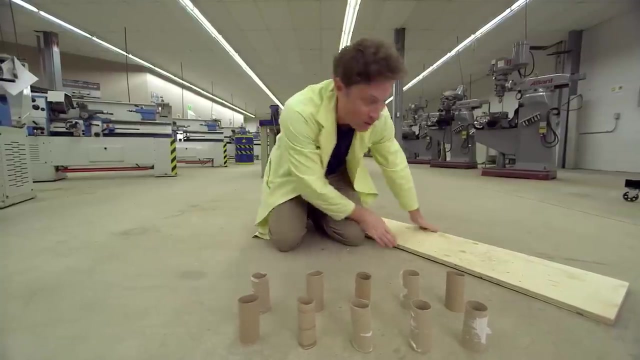 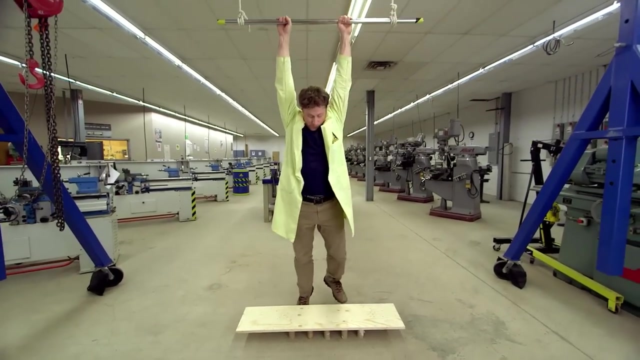 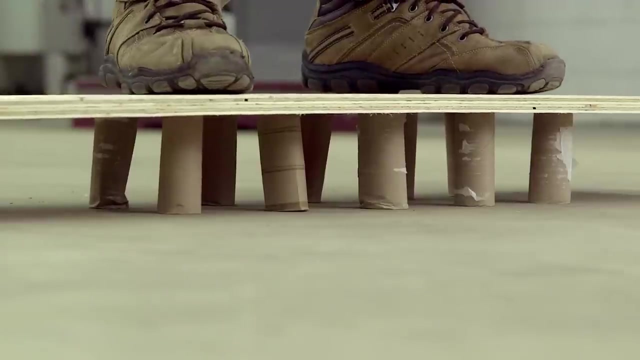 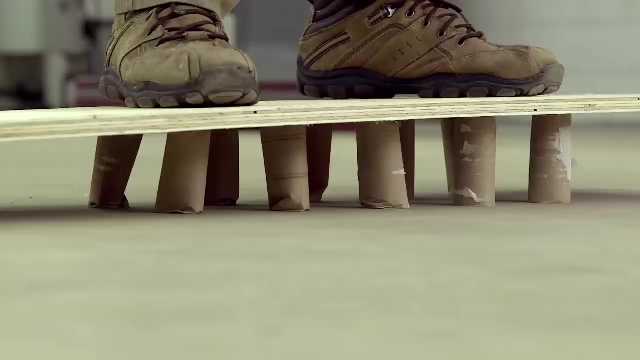 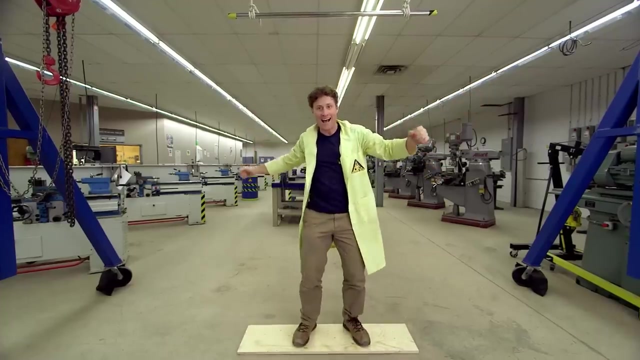 Hmm, Nope, Bills weight on four toilet paper rolls. Nope, Bills weight on six toilet paper rolls. Nope, Bills weight on ten toilet paper rolls. Nope, Nope, Nope, Nope, Nope. Phil's weight can be supported by ten toilet paper rolls. but what if Phil jumps? 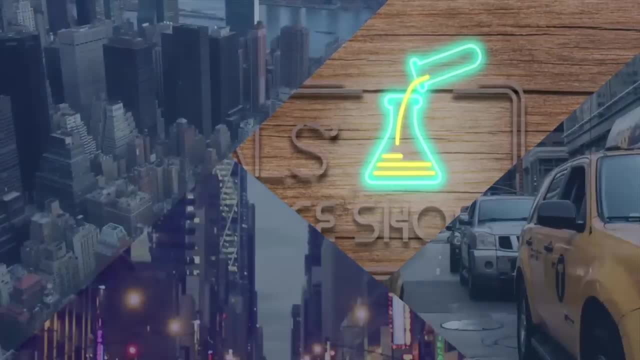 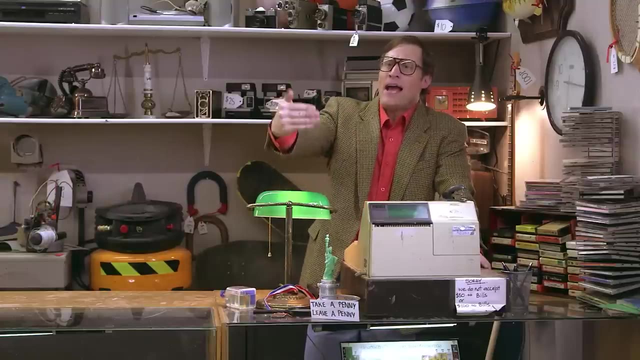 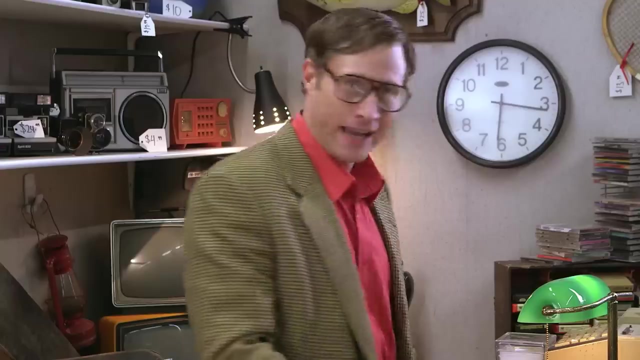 Didn't really work. That's good, Ramona. put it in the, put it in the background, put the sign in the background. Yeah, in the BG, I love the BG. Chemicals, Chemicals, Chemicals, Chemicals. 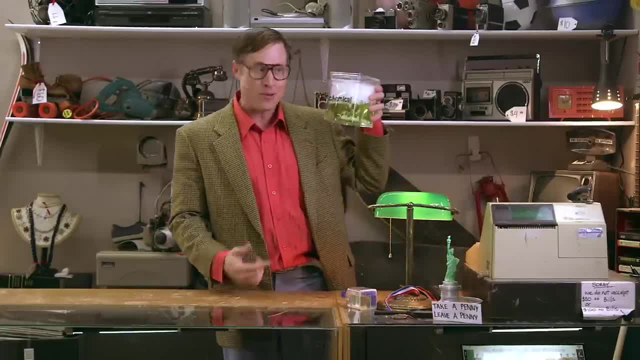 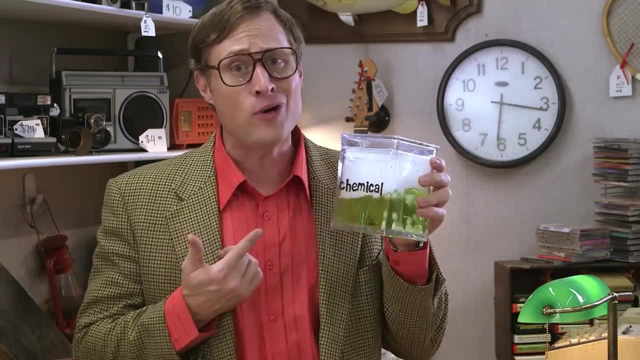 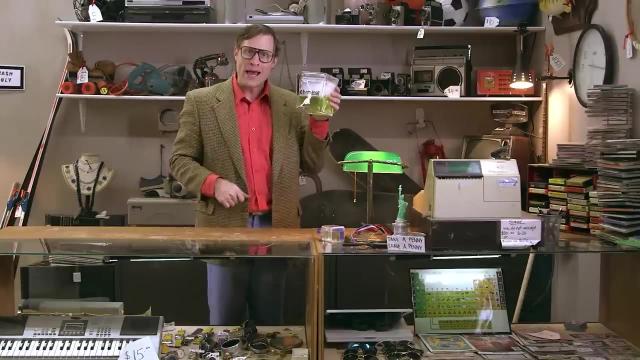 Chemicals. What are chemicals? Are they things you have in a lab, in a jar that say chemical on them? Well, yes, but if that's all you think chemicals are, then you need to know: Oh, you're chemicals. Turns out, the stuff in the jar is a chemical, but the jar itself also made of chemicals. 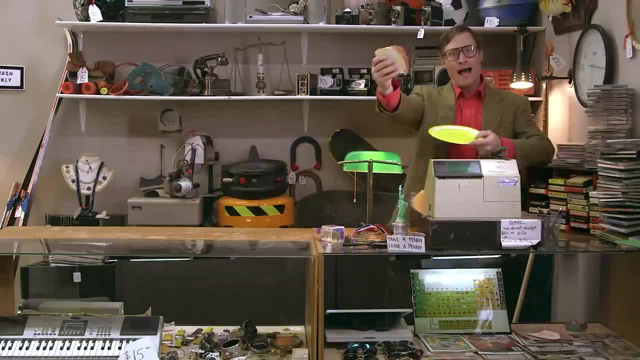 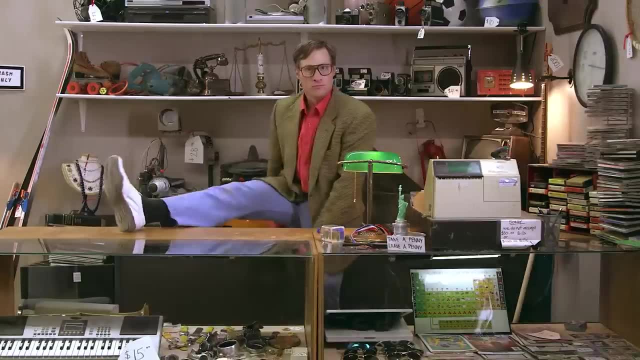 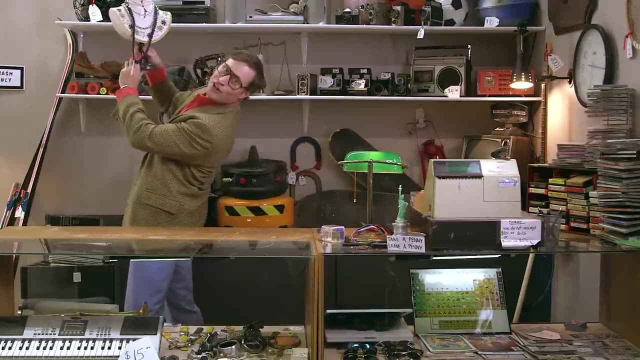 The table I'm putting it on made of chemicals: My lunch chemicals, Roller skate chemicals, My jacket chemicals, This guitar chemicals, My shoe chemicals, This watch chemicals, This fish chemicals, Chemicals, Chemicals. 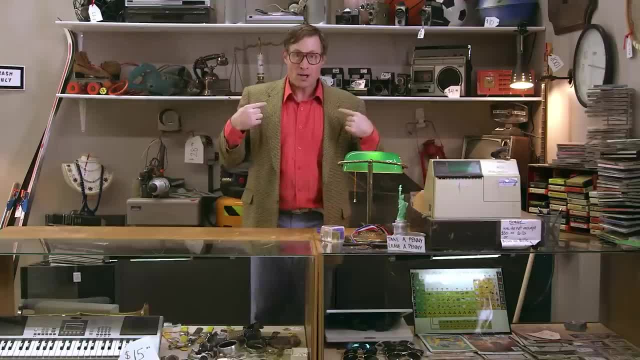 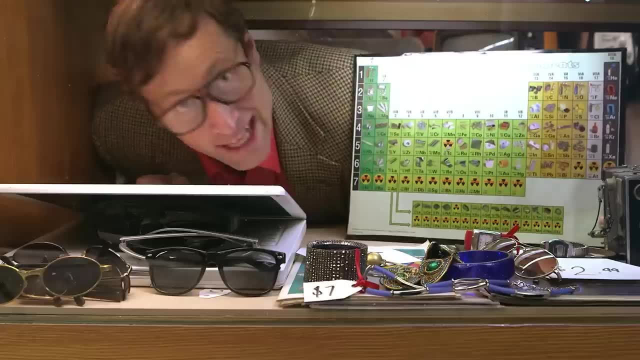 Chemicals, Chemicals, Me chemicals, You chemicals, Ramona, chemicals, Chemicals. No, I said you're chemicals, Chemicals, Never mind. This is it The periodic table of the elements. All matter in the universe is made up of these pure elements. 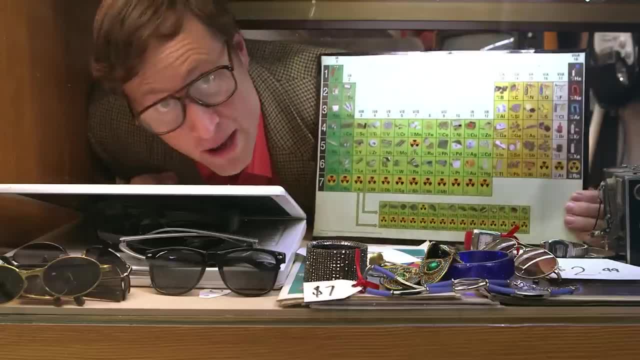 They go together in different ways to make up everything, All matter. Think of it like building blocks. These little atoms are some of the elements on this periodic table. You got one oxygen, two hydrogen Bam. You got a water molecule, One carbon, two oxygen. 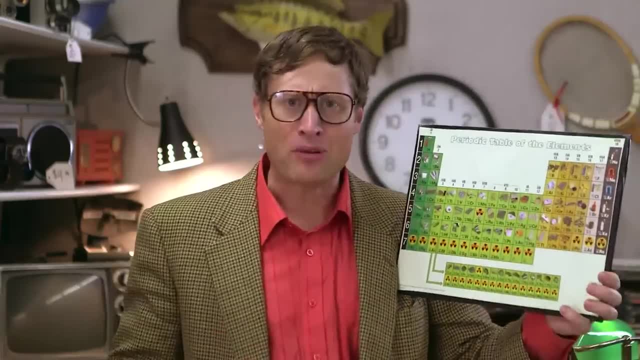 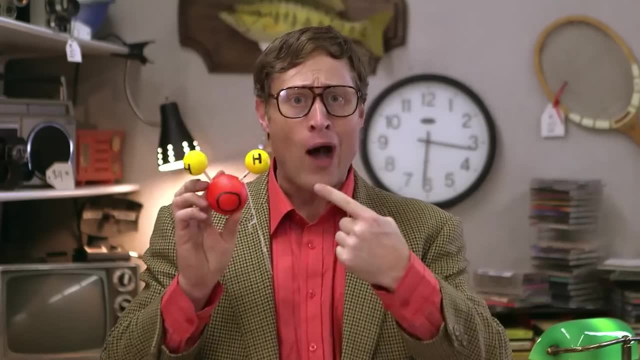 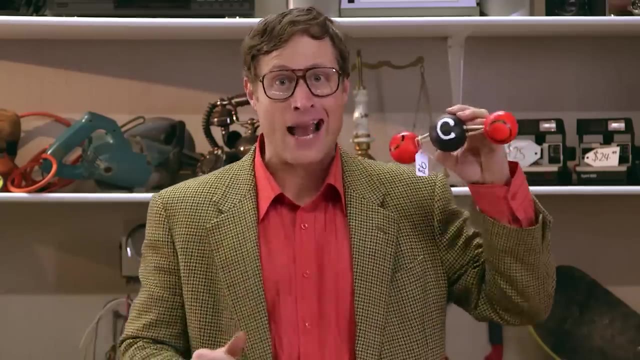 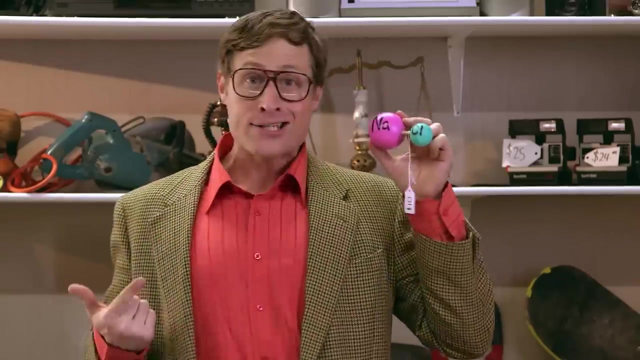 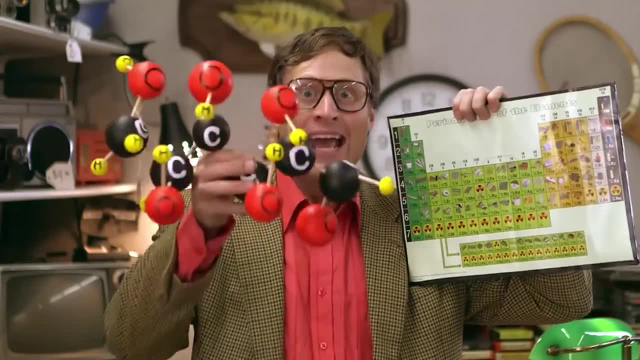 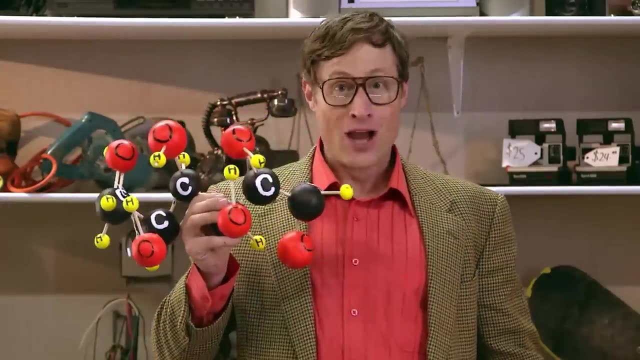 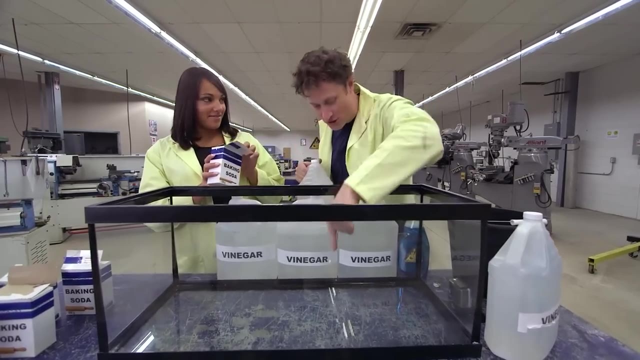 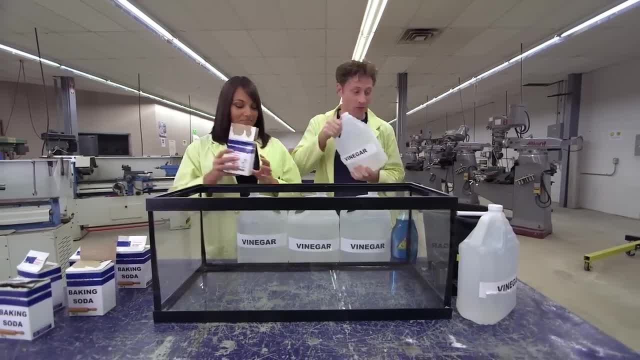 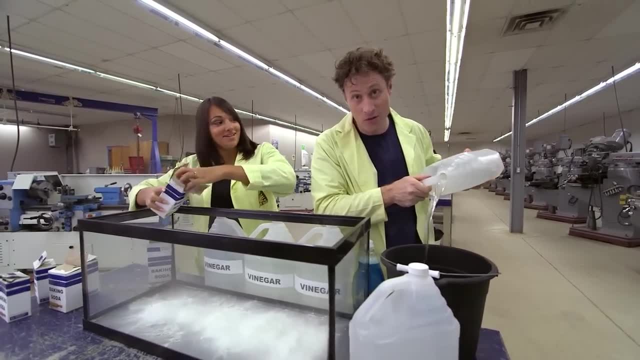 pour them together right away. Okay, you ready? Yep, Okay, go for it. When you're doing your PhD in chemistry, you get to do stuff like this. Yeah, Really, I get to do a lot of fun reactions in the lab. Oh, that's. 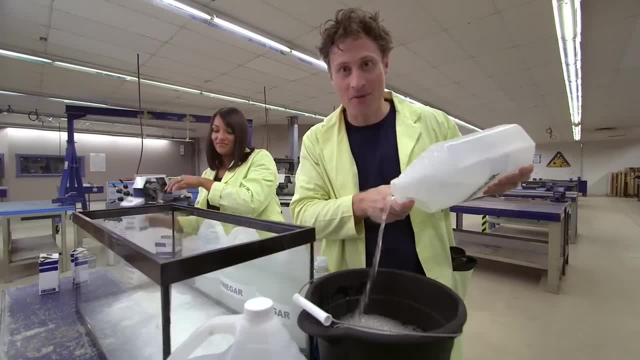 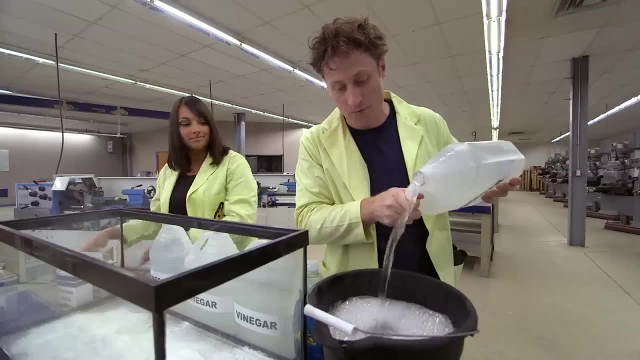 I'm jealous. Have you ever done this much vinegar in baking soda in one time? I can't say I ever have. There you go. That's what I like to hear. I already put the soap in the bucket so it would mix with the vinegar when I poured it in. 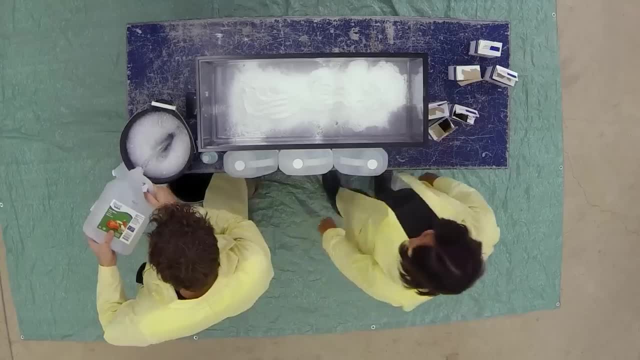 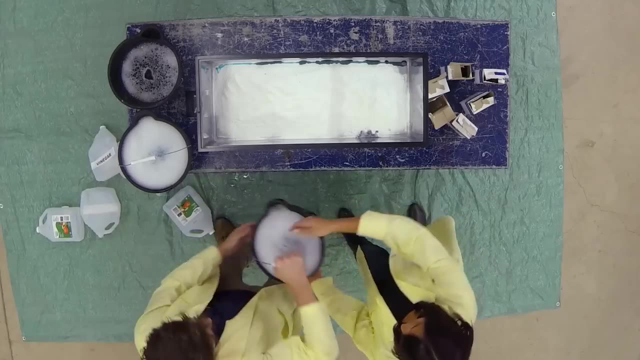 Are you done your baking soda? already I am, I'll pour faster, Oh faster. It smells vinegary, It smells vinegar. It makes me want french fries. Okay, Talena, you take this very full bucket of vinegar and dish soap. 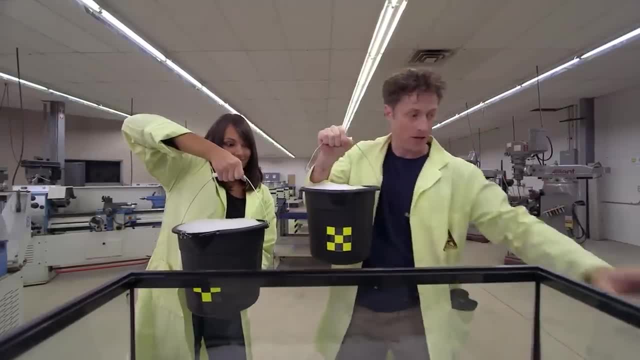 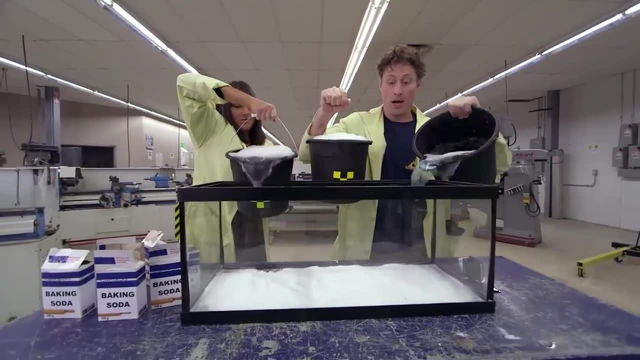 Thank you, I will take this one. Uh-oh, we still have our third bucket. Okay, I'm going to. I'll do these both at the same time. Okay, Ready On the count of three. One, two, three. 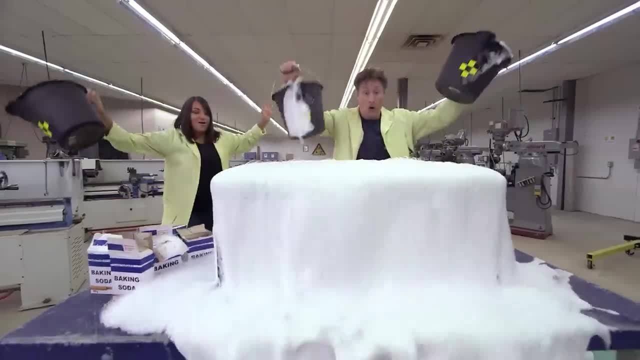 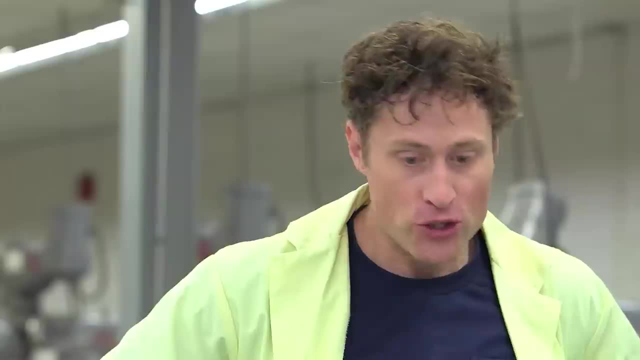 Whoa, Whoa, Whoa, Whoa, Whoa. Okay, That's awesome. So the one thing it didn't do: it didn't shoot up in the air, though Yeah, it's because the top is quite open. 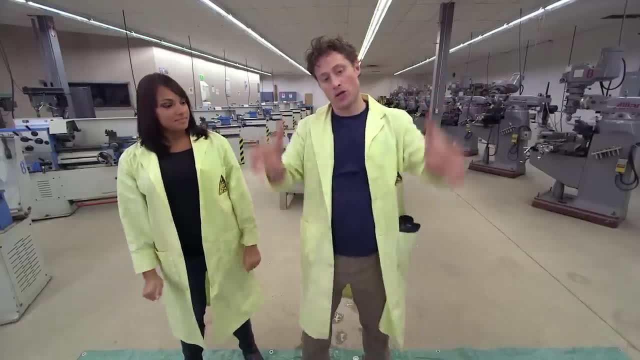 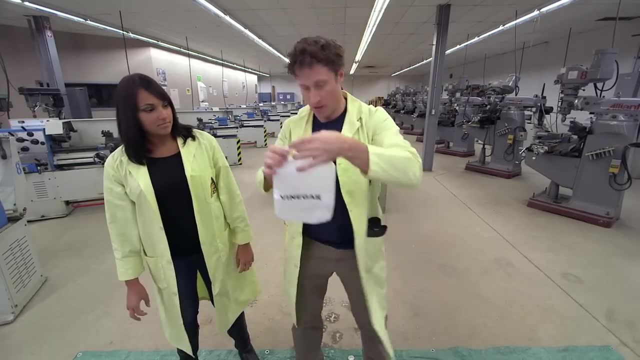 so you would need to constrict it to get it to shoot up. Oh yeah, because we're using just sort of a square, a rectangular prism container. We should get something that's maybe something more like our vinegar bottle, right Yeah? 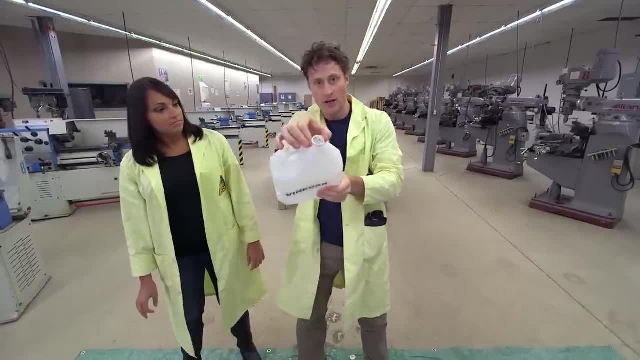 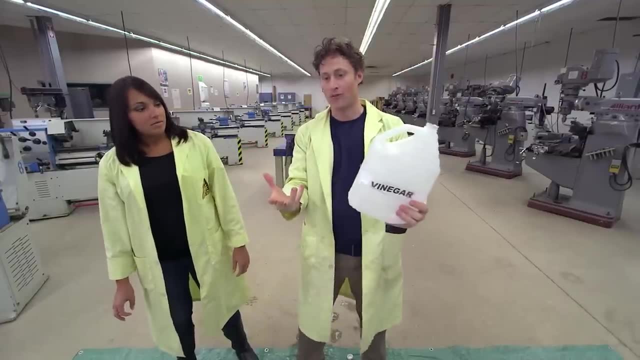 There's lots of space down here, but then it forces it in, So we're going to put it into a tighter opening at the top there, like a volcano. Yeah, And what else can we do to make it even more powerful?